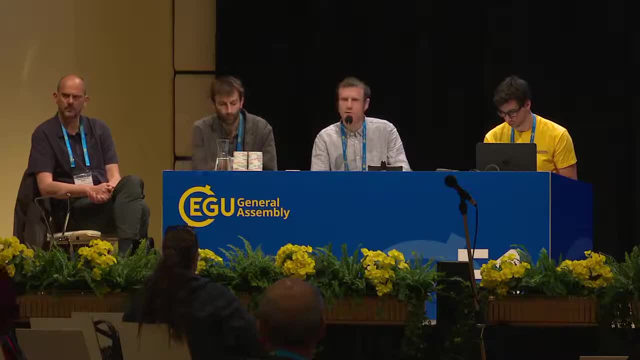 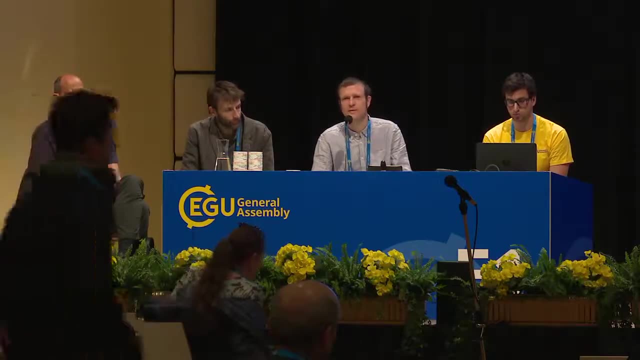 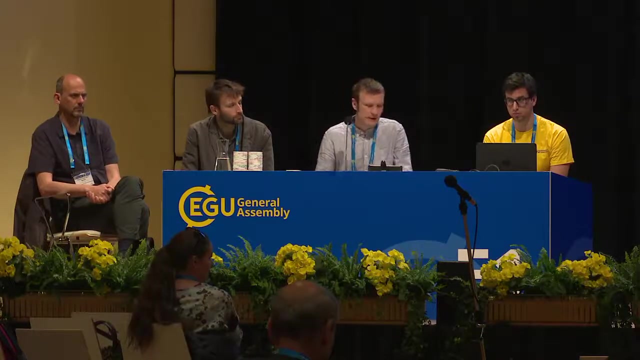 between the soliders, the hydrosphere, atmosphere and biosphere. So one could look at this session as a mere collection of unrelated topics, but I think it's much more than this and it's trying to find the bridges between all the spheres, And we're really happy because 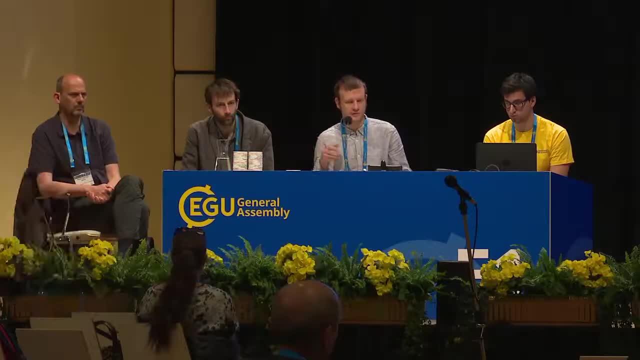 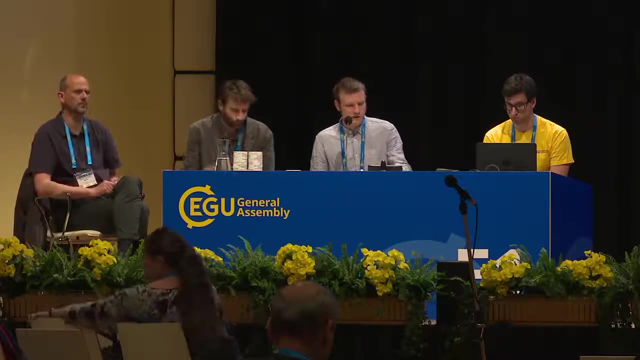 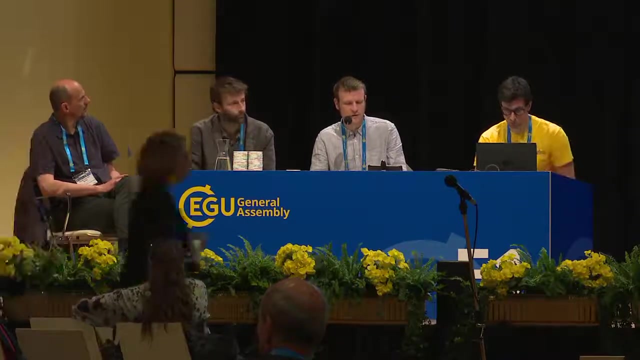 this session is going to encompass all the topics, ranging from soliders, ocean, atmosphere and even biosphere, So we're going to start by welcoming Jennifer McElwain, who's going to be talking about assessing biosphere feedbacks on Earth systems. 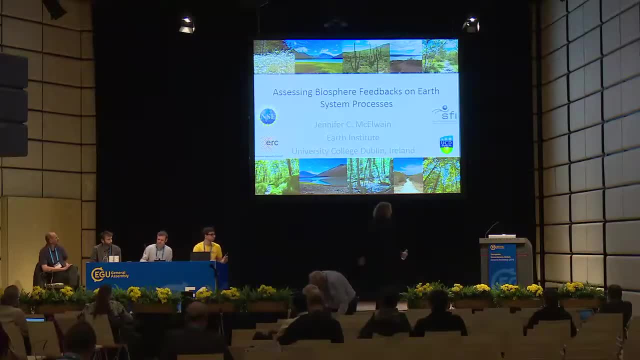 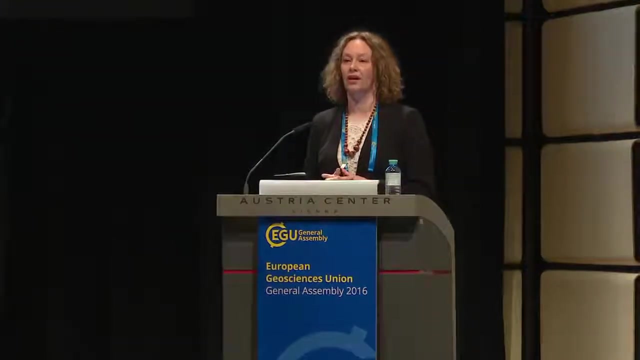 Earth system processes. So good morning and thank you for coming to this early talk. So what I'd like to look at today is the biosphere And I think if we look at Earth system processes- I suppose for my own bias being a paleobotanist- I think one of the biggest 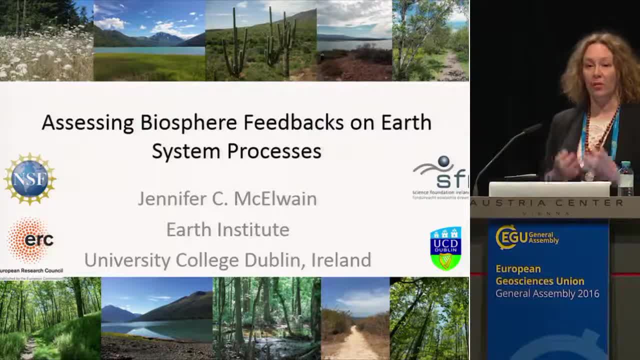 uncertainties is that we don't know what the biosphere is, And so I think we need to look at what the biosphere is, And I think one of the biggest uncertainties in Earth system processes is within the biosphere, And the biosphere is at the interface between the 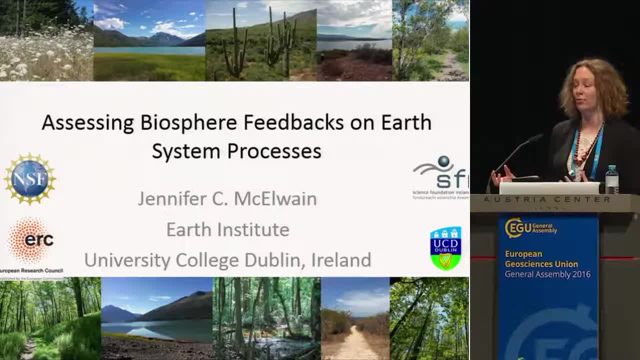 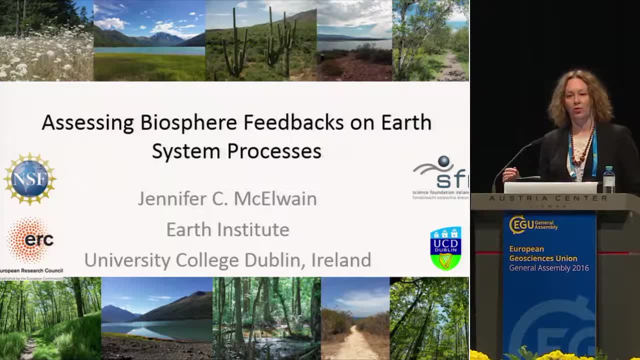 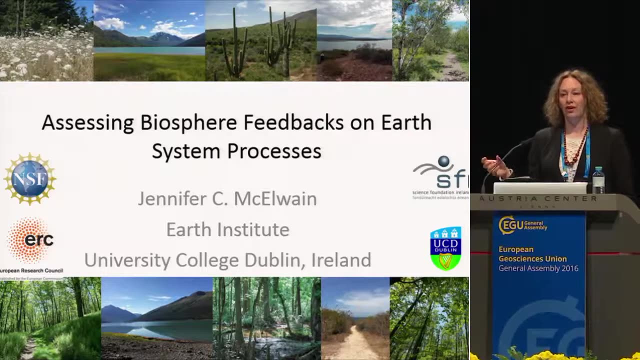 lithosphere, the hydrosphere, the atmosphere. So of course it's hugely important And I think what I'm going to do in my talk today is, rather than give you any answers, I'm hoping to provide some sort of a roadmap to show how we can use the paleo record to inform our understanding. 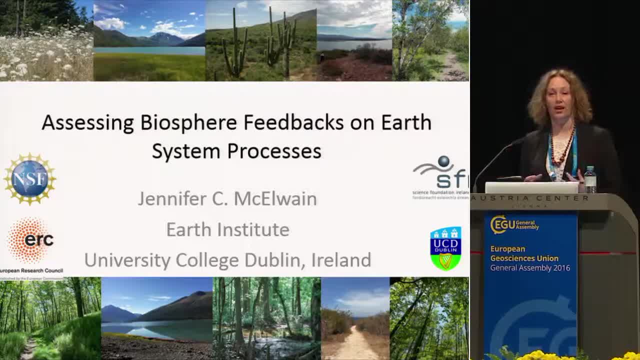 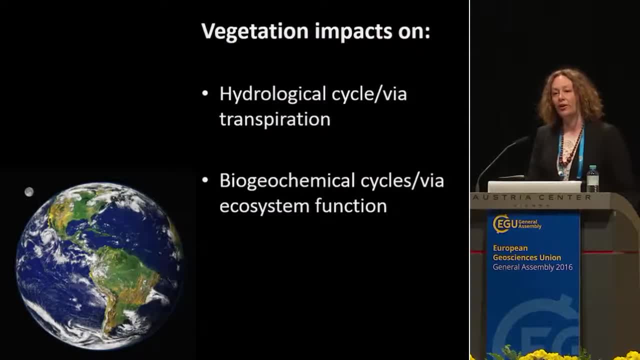 of biosphere processes which has relevance to today And has relevance to Earth system models. So what I want to particularly focus on are two aspects of the biosphere: Hydrological: the feedbacks of the biosphere on the hydrological cycle by looking at transpiration. 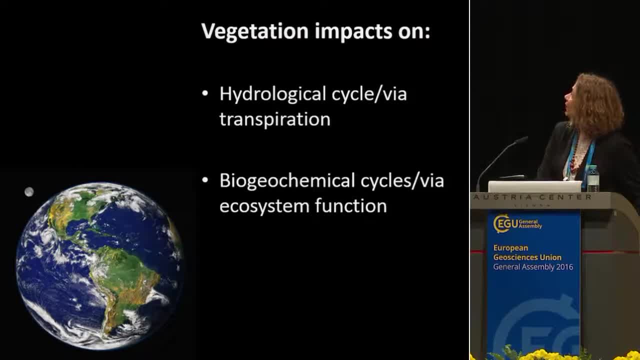 which is water loss from plant bodies. And if I have time- because I've rather too many slides- I want to also look at biogeochemical feedback. So how would changes in plant function influence biogeochemical cycling of nitrogen and carbon through the ecosystem? 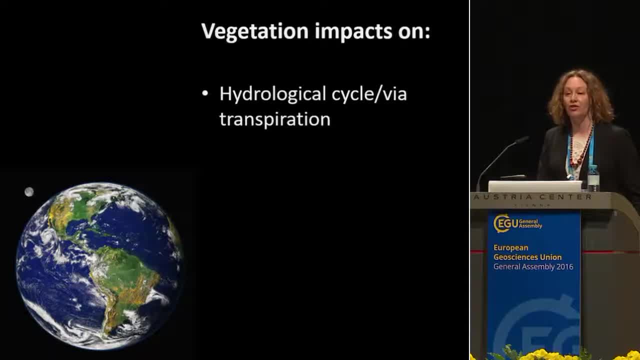 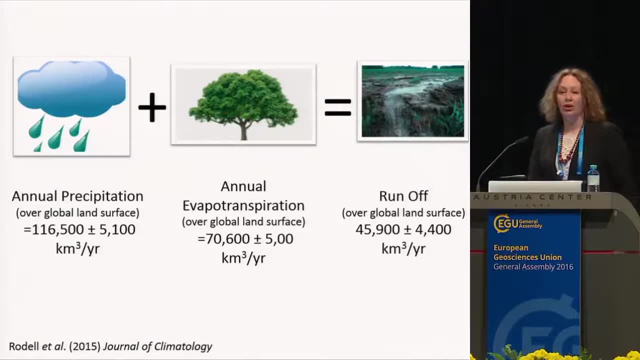 So looking at the effect of the biosphere, first on the hydrological cycle. to put it into context, if we look at this very simple bucket model of the global hydrological cycle, precipitation in annual evapotranspiration out equals runoff. So we can see here that the 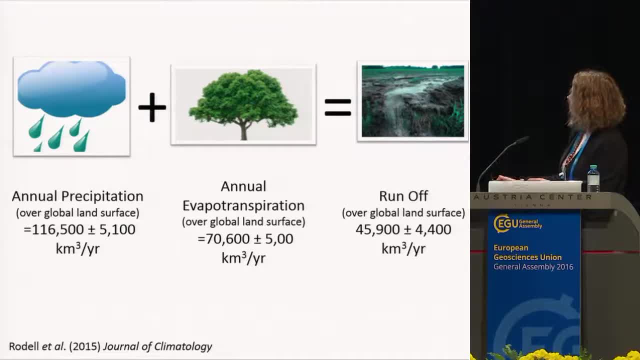 we can see here that, if I can use the pointer, how does this work? Sorry, Just press here. Okay, thanks. So you can see here that vegetation has a huge influence on the hydrological cycle via evapotranspiration, which is the combination of evaporation of water from land surfaces. 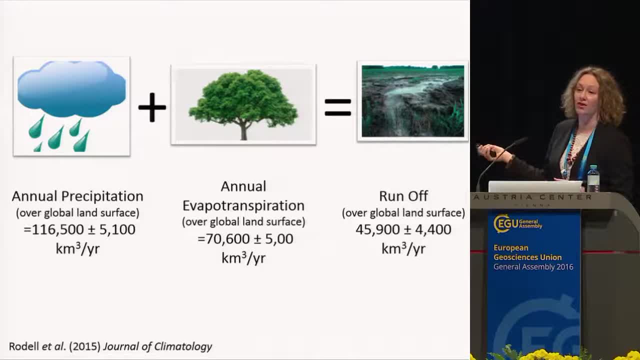 which is un-vegetated, and water loss from vegetative surfaces of the biosphere. So any change in the annual evapotranspiration budget is balanced by a change in runoff. So a decrease in this proportion, for example, would lead to an increase in runoff. 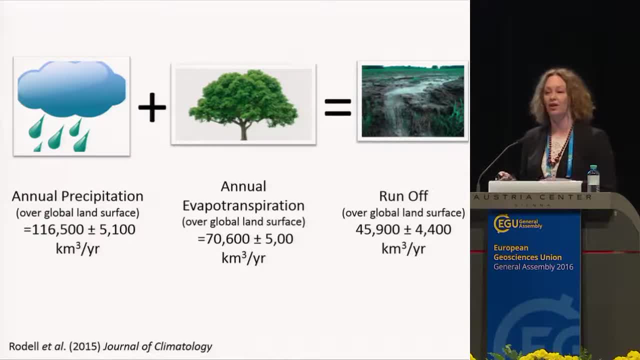 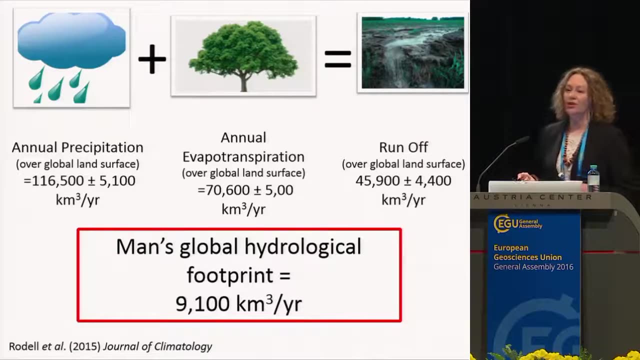 And runoff into the oceans has big impacts in terms of eutrophication. If we're looking on geological timescales, it can start having influence on organic carbon storage- black shales, oceanic anoxic events- So I want to put it into some sort of a context. 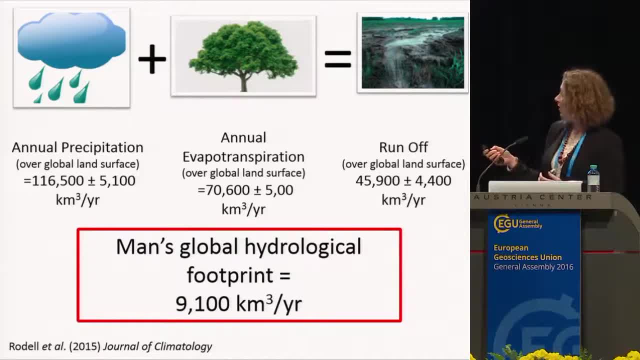 If you look at man's global hydrological footprint, it's 9,100 km3 per year. So even a 10% to 20% change in annual evapotranspiration is getting close to the magnitude of man's entire global footprint. 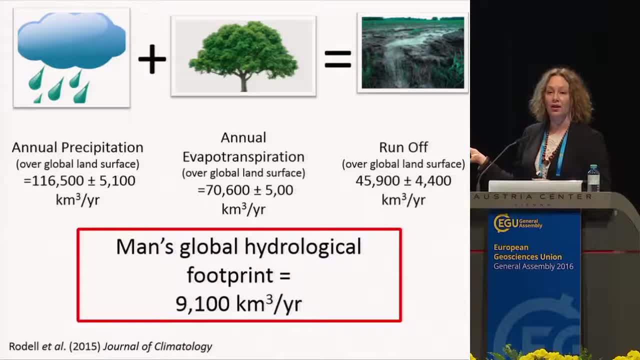 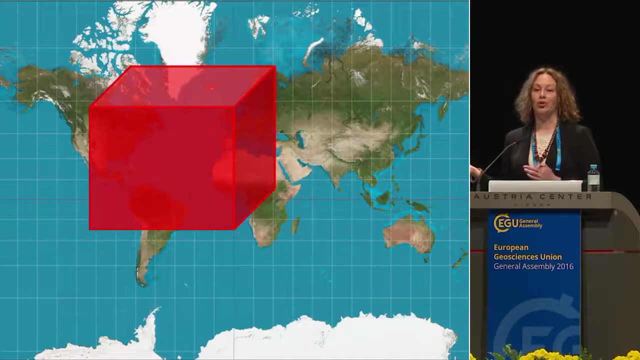 on the global hydrological cycle, So Plants are important. I wanted to try and visualise what this looks like, so I've done a horribly simple visualisation. That is a 9,000 km3 square on the global map. 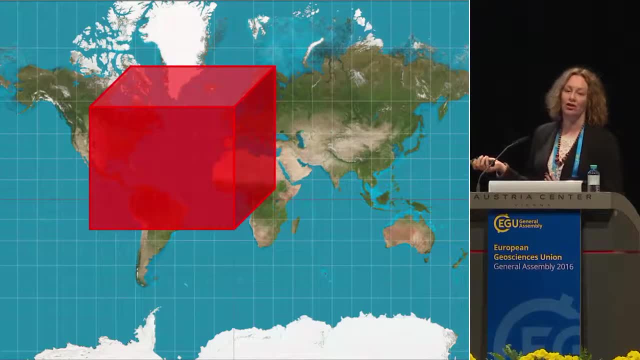 just to give you a sense of man's global footprint on the hydrological cycle. And what I'm suggesting from this model here is that a 10% to 20% decrease in transpiration of global vegetation, perhaps in response to increasing carbon dioxide. 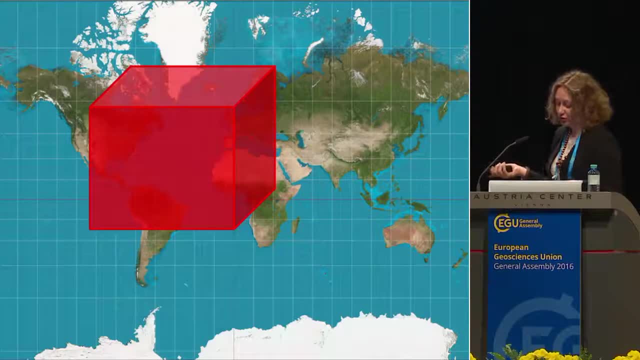 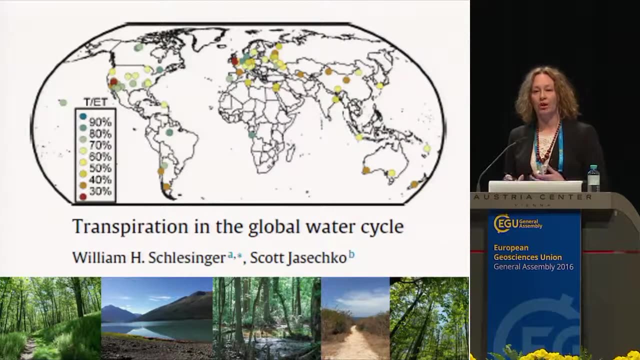 would have an equivalent effect on the whole transpiration cycle. So we have to consider: what role does transpiration play in this evapotranspiration budget- And this is recent data by Schlesinger and Giusecco- And what they've done is they've looked at different sites. 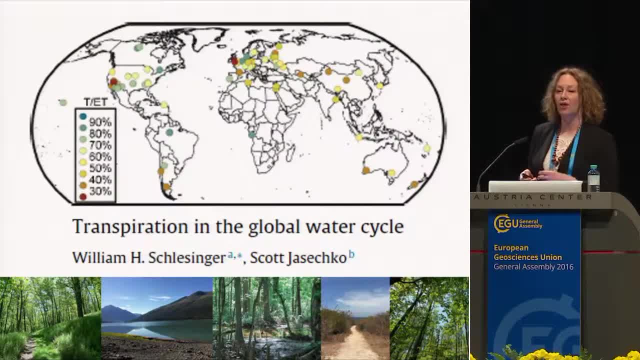 across the globe and tried to assess what proportion of the evapotranspiration budget is influenced by plants. Now, on average it's about 35%, But you can see that in some biomes, some vegetation types, 90% of the water coming from the whole evapotranspiration budget. 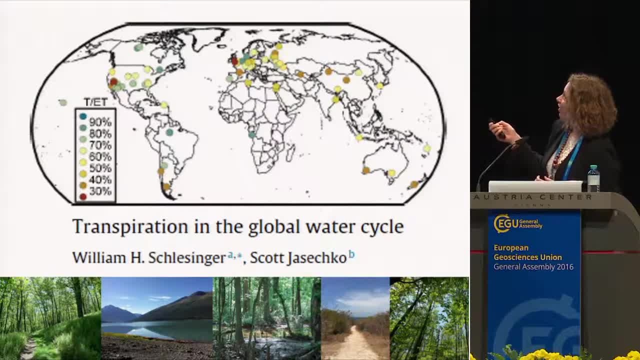 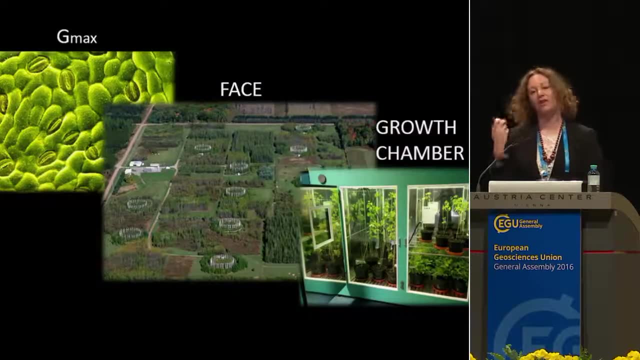 is coming from plants. So, depending on where you are in the world, plants can have a greater or lesser effect on the hydrological cycle and a greater or lesser effect at modulating the climate system. So how do we, How do we, assess biosphere feedbacks? 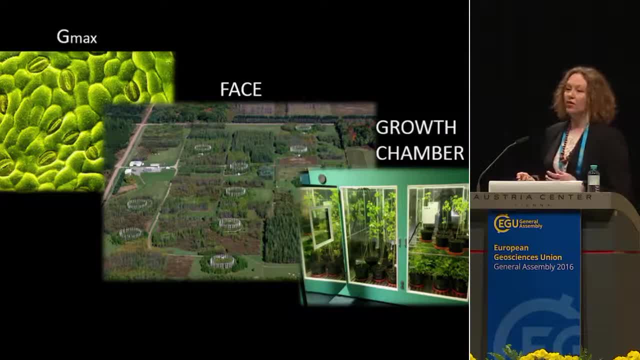 on Earth system processes And there are many different approaches And really my talk today has a lot of modern data sets rather than geological data sets. So we can grow plants in simulated atmospheric chambers, plant growth chambers where we alter the atmospheric composition. 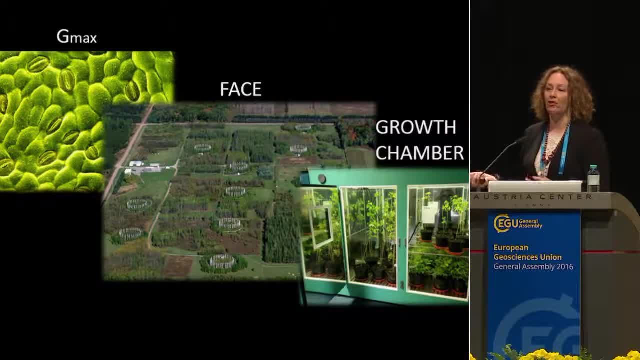 let's say, to double ambient CO2 or a mesozoic atmosphere or a paleozoic atmosphere. There's a lot of data already out there on face sites which are free air carbon dioxide enrichment And this looks at vegetation responses to a doubling of ambient CO2 concentration. 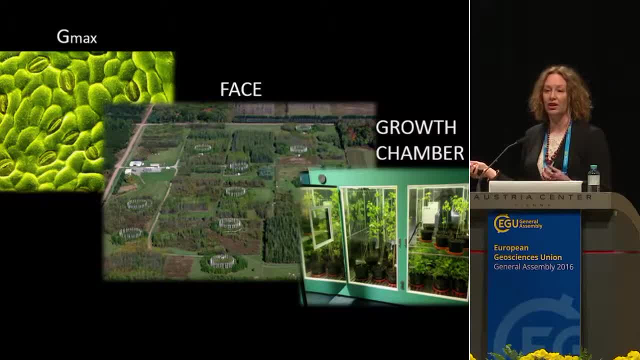 trying to assess: how do plants respond physiologically, how do plants respond in terms of water loss, and how will that influence the evapotranspiration budget? Another approach is developing paleo records And in the paleontological record, of course. 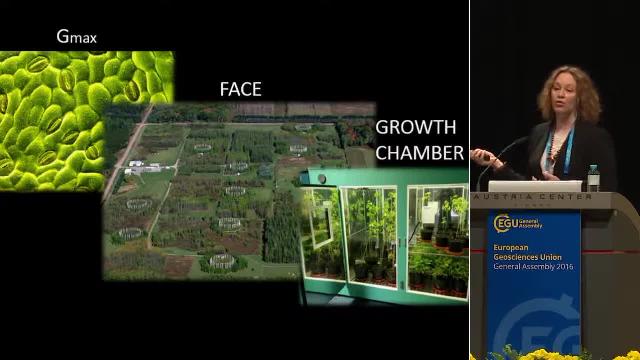 all we have is anatomy and chemistry, So we need to develop appropriate proxies, such as this proxy Gmax, which is theoretical maximum stomatal conductance. It's basically a measure of the maximum amount of water that can be released from a leaf surface. 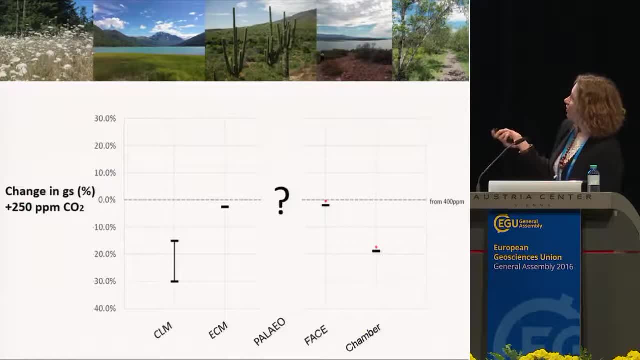 But there are a lot of uncertainties even in the modern data set. So this graph plots changes in stomatal conductance, GS, as a percentage, in response to a certain amount of water loss. So if you look at this graph you can see that there's about 250 ppm increase in CO2.. 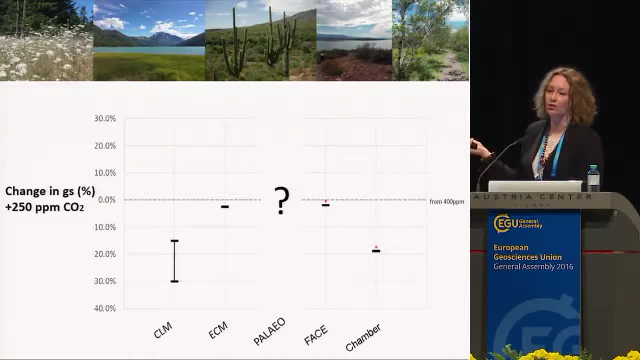 So that would be a simulation of the end of the century or 2050, depending on your climate scenario. If you look at vegetation in CLM responses. so the vegetation model in uncoupled mode, it suggests that globally vegetation could respond. 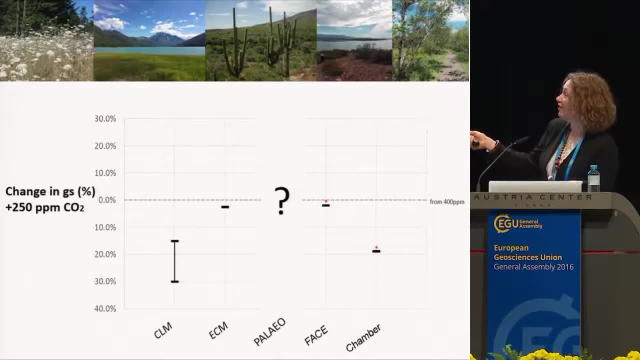 by decreasing stomatal conductance of between 20% to 30%. So if you remember back to the hydrological budget, this would have a huge potential impact on runoff And, if you think of it, on geological timescales. it could then start to influence the initiation. 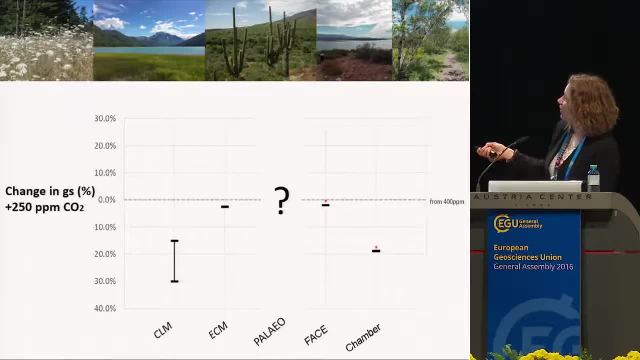 of oceanic anoxic events. However, if you look at Earth system models in fully coupled mode, where the vegetation is coupled to the atmosphere and ocean, it suggests a very modest response of global vegetation Phase studies, these big experiments where you're subjecting in situ forests. 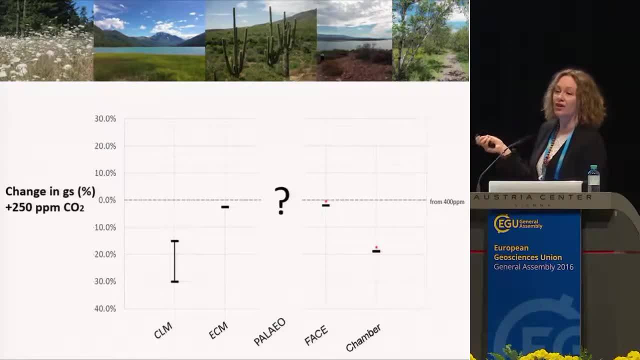 CO2 also suggest a modest response to increasing CO2.. So this would argue, the biosphere has very little impact on these big Earth system processes. However, if you look at chamber studies again, they're more in line with the vegetation model. 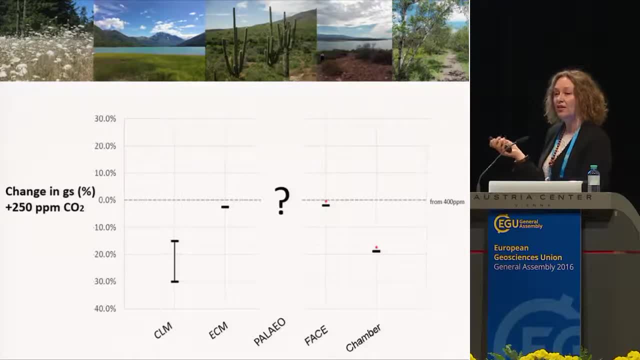 suggesting 20% reduction in stomatal conductance, the rate at which gas can be exchanged between the biosphere and atmosphere in response to CO2.. So there's huge uncertainty in the modeling data, the modern data, the experimental data And, I think, as a community. 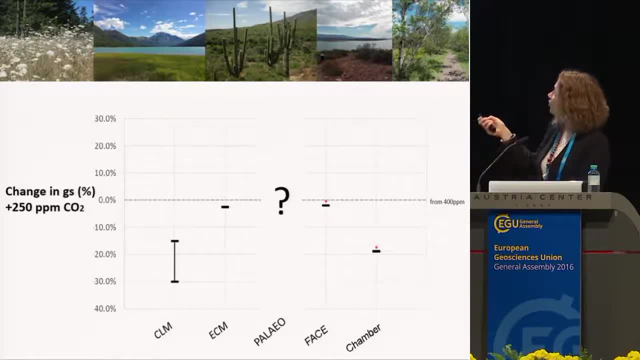 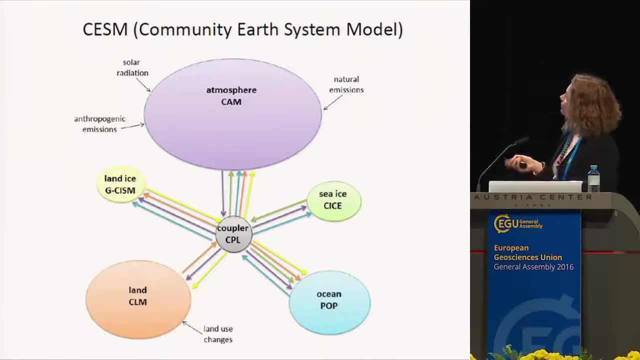 we have a lot to offer in terms of looking at paleo case studies to try and work out which of these is more likely. So we have a big project at the moment, which is a model data fusion project where we're working with climate modelers. 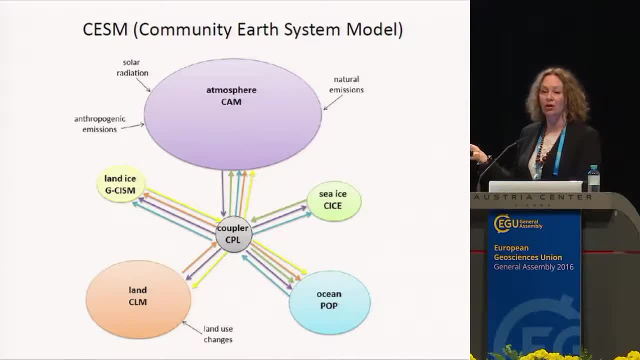 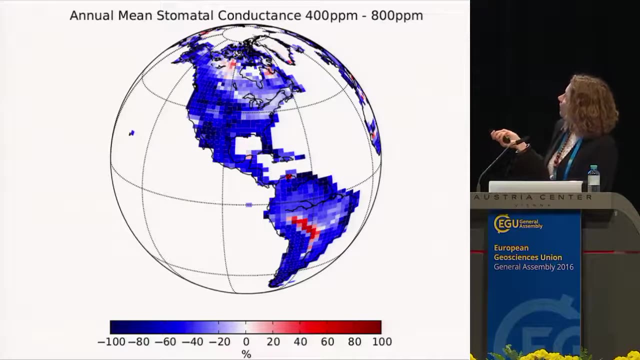 specifically asking: how well do the current vegetation models assess vegetation responses to increasing CO2? And is there a possible for physiological forcing of vegetation? This is output from the community lands model and CLM And you can see in response to an increase in stomatal conduct. 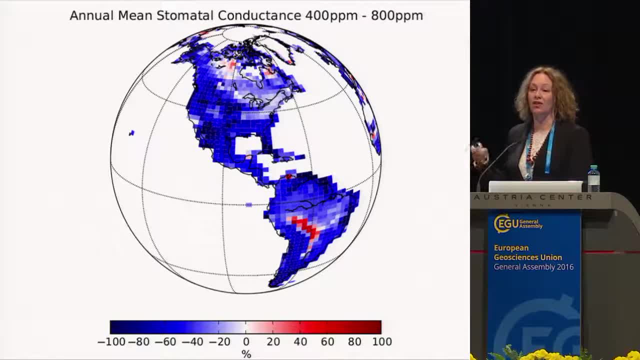 increase in CO2, let's say 700 ppm or 800 ppm increase in CO2, this plots the difference in stomatal conductance and you can see that it's a blue world And the model is suggesting that stomatal conductance in the future. 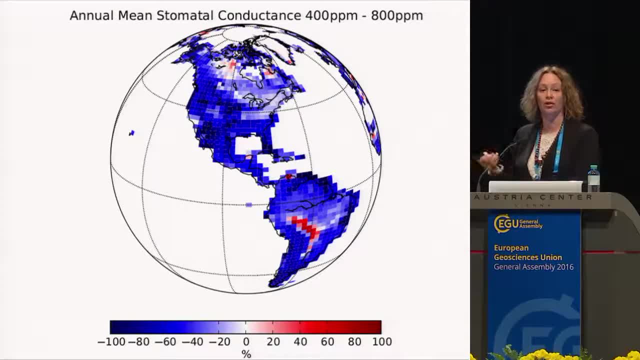 the rate at which the biosphere can lose water from the system is going to decrease dramatically. Now this isn't a new result. There are many climate models at Gedney and Betts who've proposed or have published on this type of response. 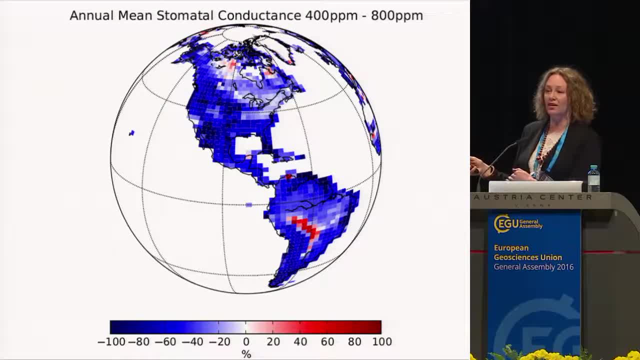 What we're doing with the modern data sets and a recent historical data set and the paleo studies is really trying to assess how robust this result is Because, in high CO2, if the biosphere can lose so much less water from the system. 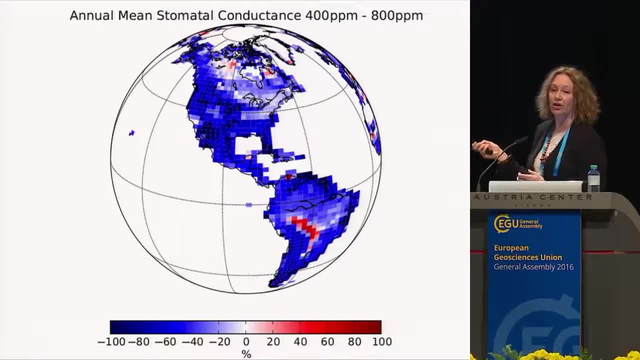 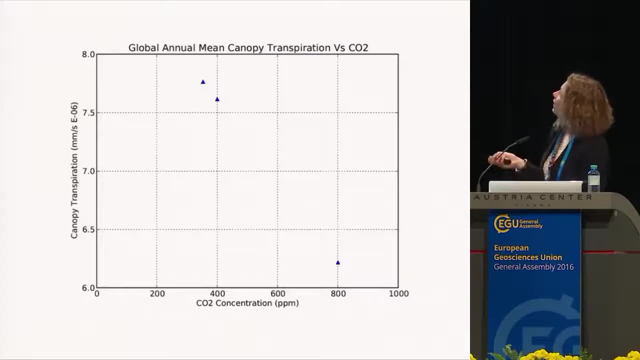 then this is going to have an absolutely huge impact on global runoff and loading of the oceans with particulates and nutrients, which can lead to other effects: eutrophication, increased organic carbon burial in the oceans. So what the model suggests is that 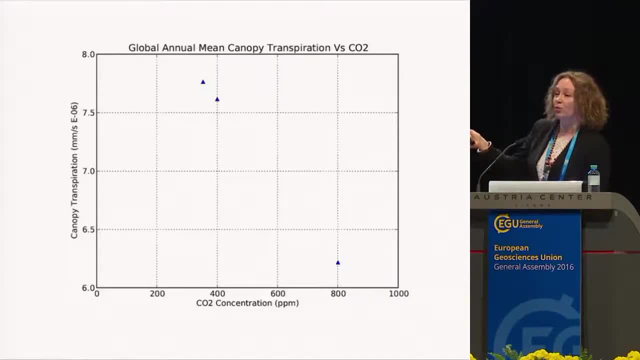 with increasing carbon dioxide concentration, transpiration, water loss from canopies decreases. Currently it's suggesting it's a very linear process, but we're trying to look at modern data sets and experimental data sets to see is it really a linear process? 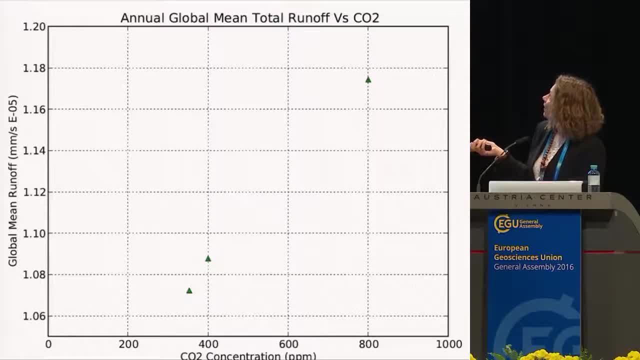 or is there nonlinearity in the system? The impact then on runoff is that with increasing CO2 concentration you would expect to see global runoff. So we've many paleo intervals, most paleo intervals in the geological past, where CO2 concentrations are much higher than present day. So these will serve as good analogues. 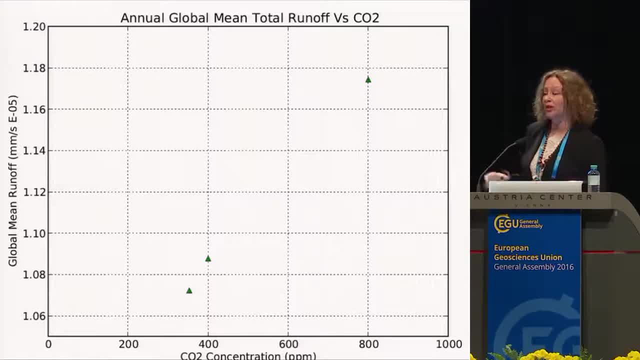 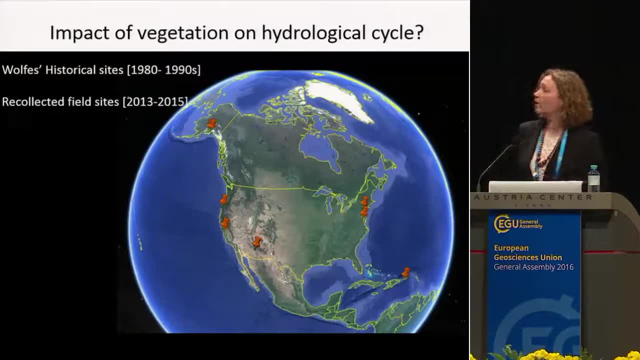 for understanding the processes and responses to help predict future runoff responses. So how are we going to try and improve the current vegetation models and improve our understanding of biosphere responses within the Earth system? Well, we're predominantly paleobotanists, so we're using as a starting point a famous historical collection of field. 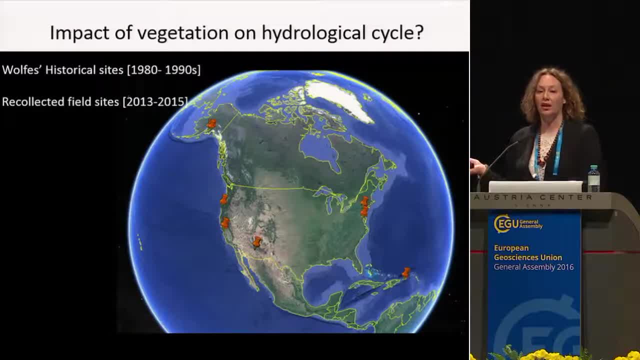 sites collected by Jack Wolf in the 1980s and 1990s And he was interested in developing proxies to look at paleoclimas. But he collected field sites- over 180 field sites from every vegetation type all across the world And he used the exact same collecting protocol. 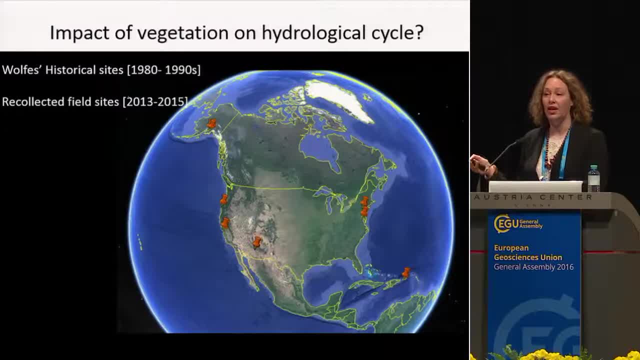 About 30 species of plants were collected from each site and all have been archived in the Smithsonian. So we set about between 2013 and 2015, collecting a subset of 22 of Jack Wolf's original field sites, And this gives us a contemporary climate change data set between 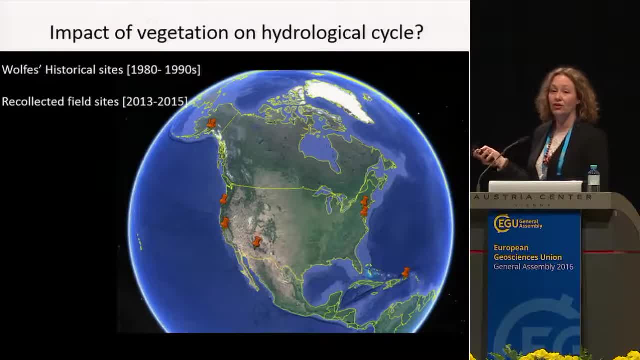 the 90s and the modern. This is 30 years of increasing CO2.. It's about 50 ppm And what we're trying to do is look at the vegetation and assess how is modern vegetation in each of the biomes responded in terms of stomatal conductance, a gas exchange? How has each biome influenced transpiration? 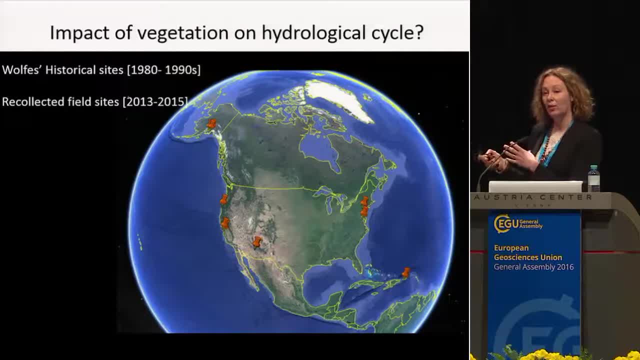 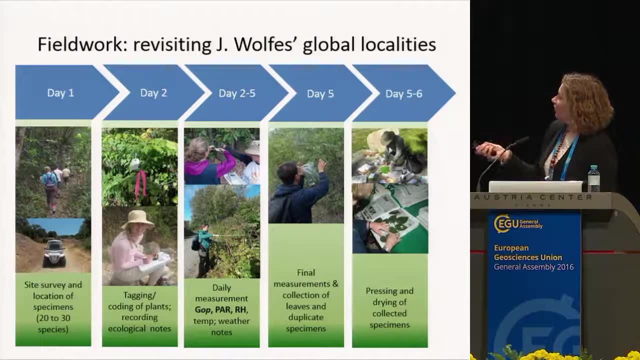 at the biome level And can we use that data set to improve existing models? So the data set— And what's unique about it is that we've gone out and collected physiological data- And physiological data is notoriously it's biological. it's notoriously noisy. 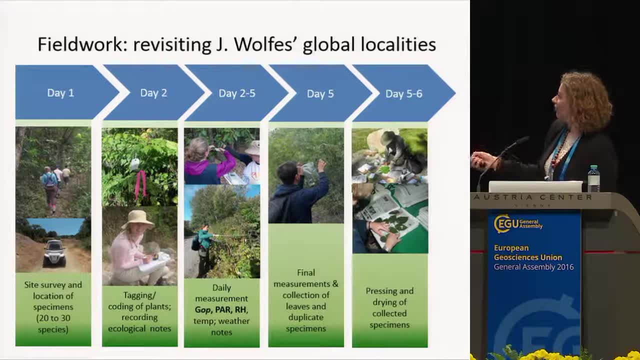 So once we find our field sites on our 20 to 30 species, we tag them and then track the physiological behaviour of that leaf, of that plant, replicated by individuals, by species, by size. And we track the behaviour of a leaf in response to light, relative humidity, temperature, vapour pressure deficit over about four to five days. 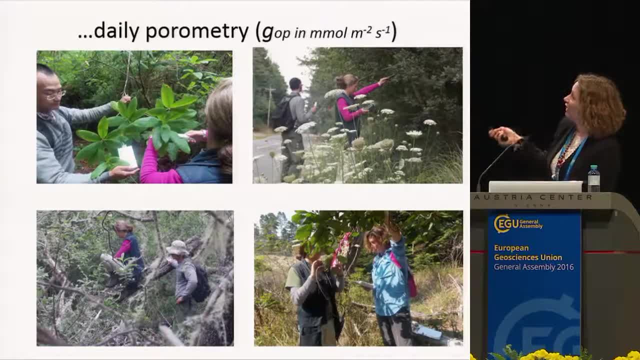 This data set and how are we measuring gas exchange? we're looking at pyrometry, So we're measuring the rate at which carbon dioxide is being taken up and the rate at which water is being lost from the leaf, And we use pyrometry or infrared gas analysis. 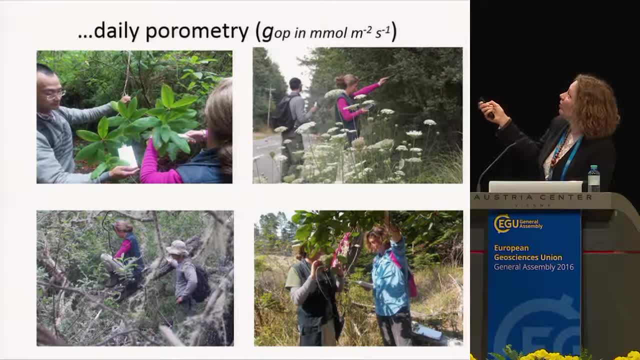 And our measure of interest is this here: GOP, operational stomatal conductance. So this is how species behave in different biome types, in different vegetation types And, looking at a huge global data set, how fast or slow do species lose water from the plant surface? 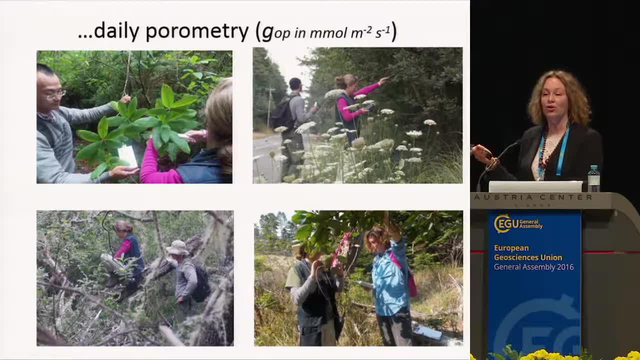 And the reason we're doing this big data set is in order to do the paleo work. we realised there isn't a global compilation of this type of data available in the modern, And the reason is most of the modern vegetation And most of the modern vegetation studies are based on crops or very derived angiosperms which just aren't of interest for the paleo record. 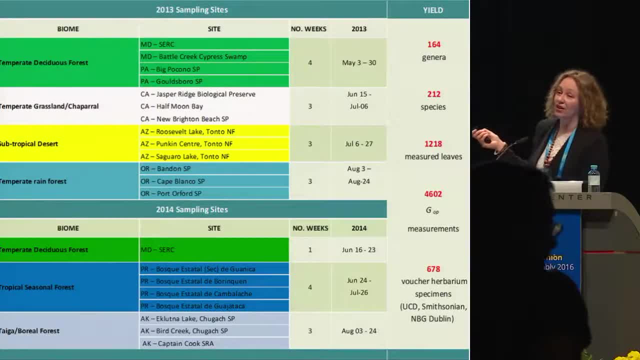 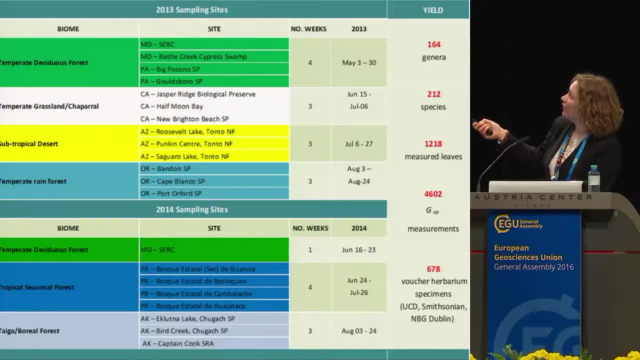 So the data set is now. the modern data set is now complete. We have sampled over 212 species from seven of the world's biomes. The only biome that we're missing is the full Arctic. We're focusing only on woody species. 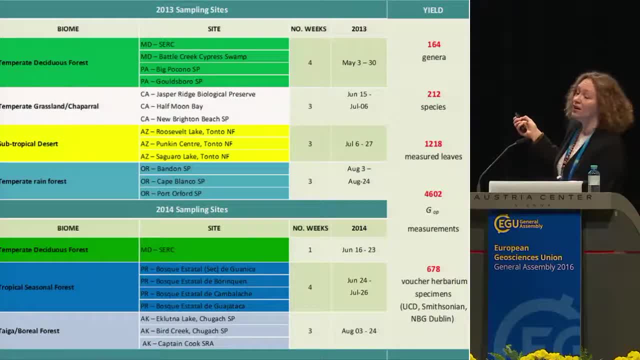 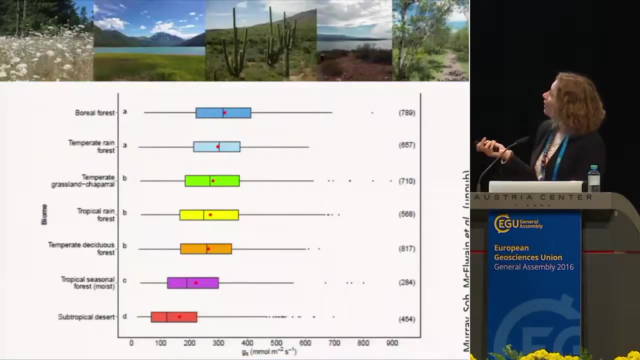 And woody angiosperms And the data set consists of nearly 5,000 unique measurements of plant behaviour in each of the biomes, How quickly this GOP measurement, how quickly the plants lose water or they exchange gas. So this is a result of a lot of work- about three years of field work by my team at University College Dublin. 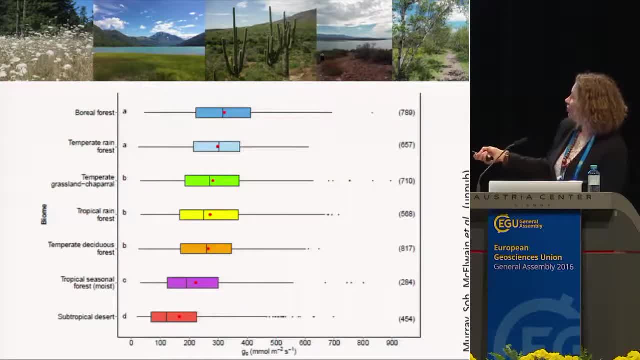 On the X-axis. On the X-axis, here I have GS, so the rate at which it's stomatal conductance and the unit is millimoles per meter squared per second. And what we've done is we've just grouped all the species, all the data, into biome types. 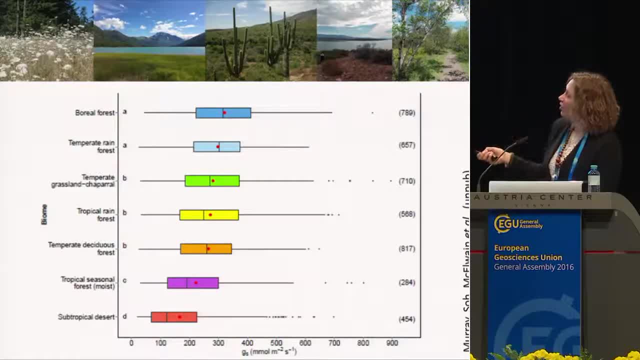 So you can see that there's a certain amount of conservatism between the different vegetation types, But this really is the first modern data set which describes the behaviour of different vegetation types around the world And why it's important for paleo, Because it allows us to put the paleo data into a modern context. 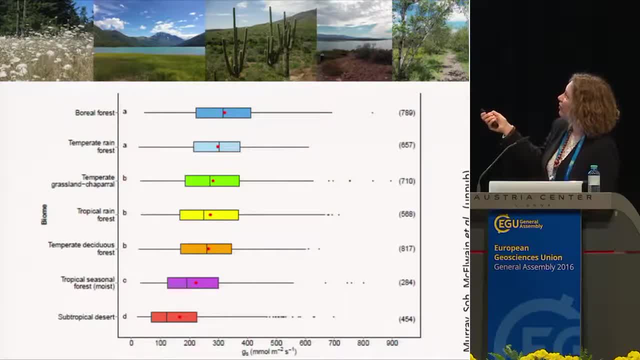 One surprising find is the boreal forest has a higher gas exchange rate in the summer than, for example, tropical rainforest. based on this data set, If I go back one, this is a modern data set which actually uses perimetry and gas exchange and infrared gas analysis to measure plant physiological behaviour. 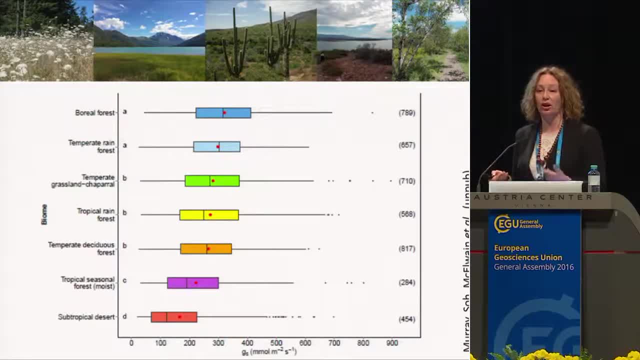 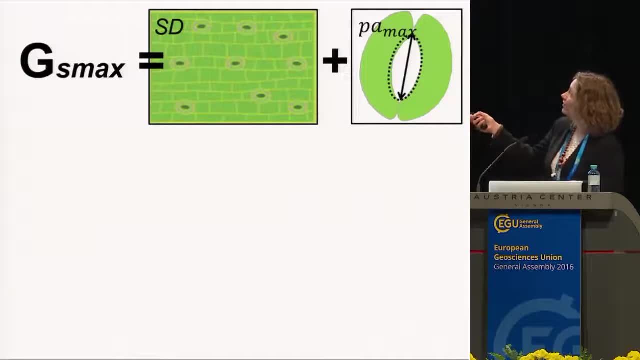 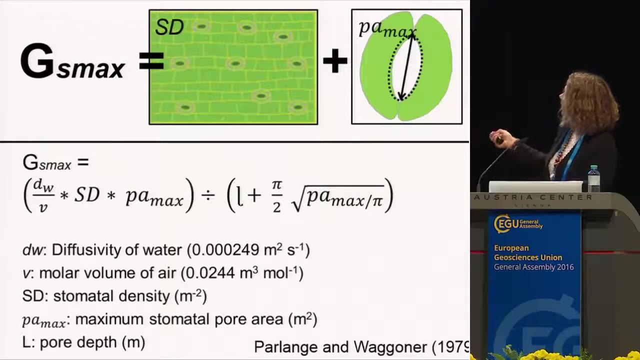 But of course in the physiological record we don't have access to actually measuring behaviour directly. So we need to develop proxies, And the proxy is Gmax, And this is basically a simple diffusion equation developed by Parlang and Wagoner back in the 70s. 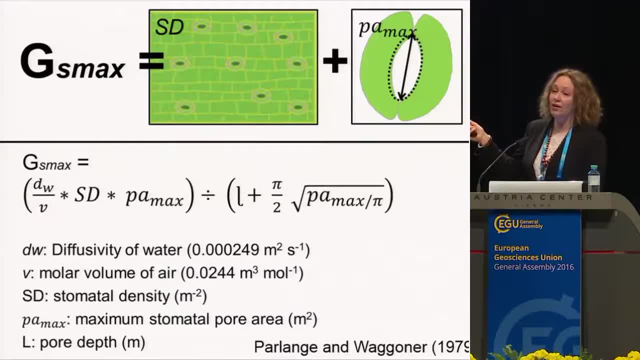 So the rate at which gas can be exchanged between the biosphere and the atmosphere at the leaf level is a function of the number of species, So the number of pores, stomata on the leaf surface and their size. And you put it into this diffusion equation and you get the theoretical maximum rate at which plants can exchange gases. 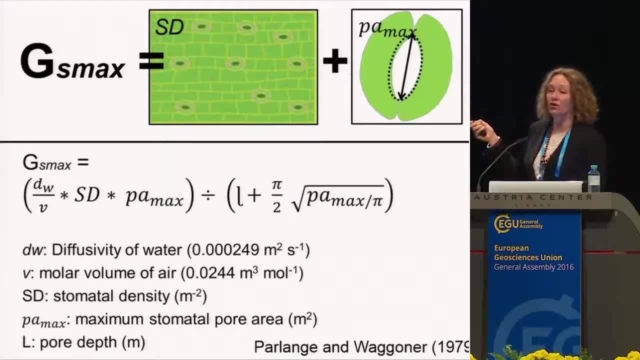 So we have plenty of fossil cuticles in the fossil record at which we can extract this anatomical data, plug it into this equation and get a theoretical rate, a maximum rate at which the biosphere in the past can exchange gas and influence the hydrological cycle. 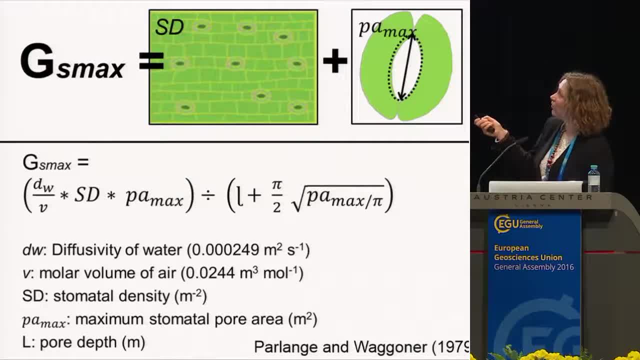 However, we needed to add one more step. This is a theoretical maximum, And field biologists know that plants rarely ever meet this theoretical maximum. You have to basically subject the plant to absolutely unique conditions for it to achieve this, to open stomata fully. 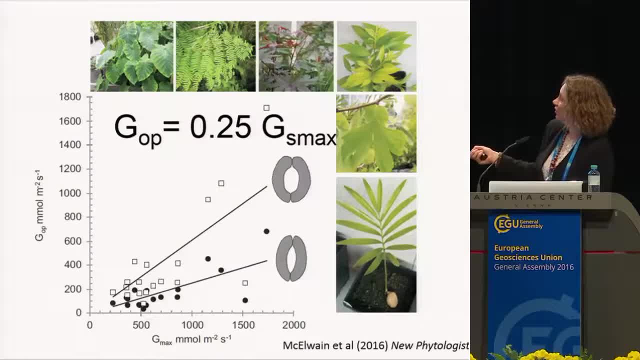 So, to apply this to the proxy record, we developed scaling relationships between theoretical maximum conductors and theoretical maximum conductors, And when we do this, it's a counter effect of the theoretical maximum conductors which we then apply to actual operating conductance in the field. 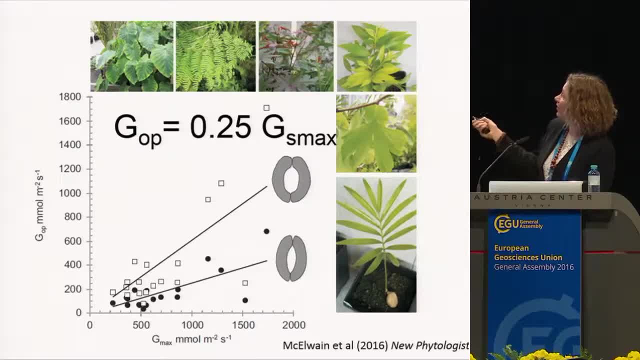 And just focusing on this bottom one here, typically plants partially open their stomata. They rarely fully open them And we've discovered for this subset of about 40 species that plants typically operate at 25% of their theoretical maximum. So if you have a fossil, you can look at the number of stomata on the leaf surface. you can measure the size of the pores to work out the theoretical maximum rate on a mass scale. 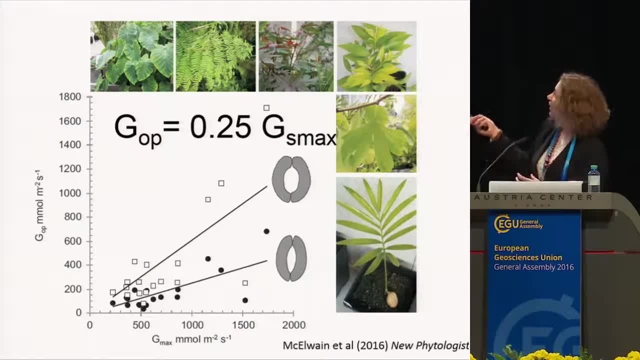 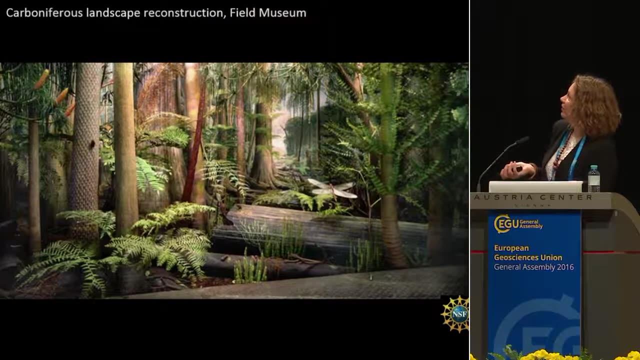 to work out Gmax and then apply this simple scaling relationship to work out paleo-operational conductance in the geological past. So I'm going to give you a case study right the way back in the Carboniferous and I'm going to 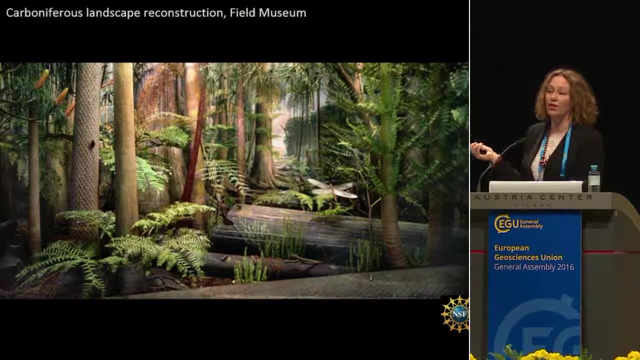 look particularly at this group of plants, the Medulosans. These are extinct, so we have no, we have no living analogue for these plants. but you could argue: if you're applying diffusion equations and applying a functional proxy, then you can apply this to any plant, whether it's 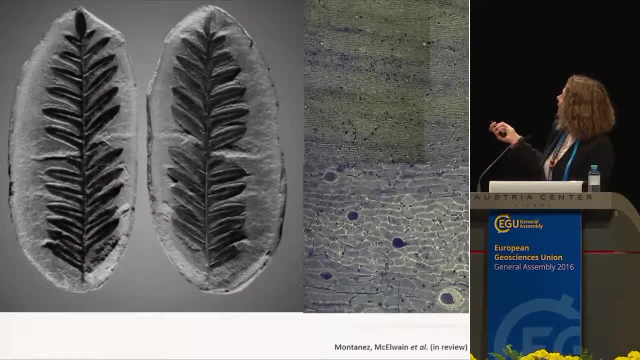 extinct or living. Here's a cuticle of Macro-Neuropterus, These tiny little things here are stomata. these are actual glands. This is Alethopterus, a cousin, just to show you what it looks like and you can see that it's a little bit of a cuticle and it's a little bit of a. 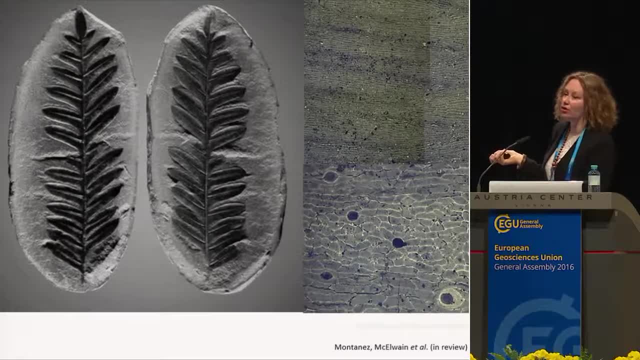 little bit of a cuticle and it's a little bit of a cuticle and it's a little bit of a cuticle. You can see here the veins going through this 300 million year old cuticle surface here. So what we've done is for about 50 of these species, spanning a 10 million year interval of the 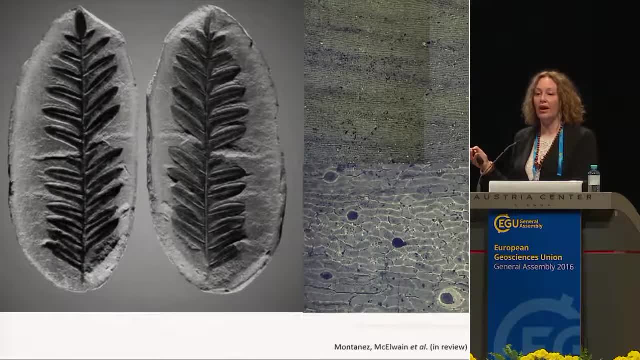 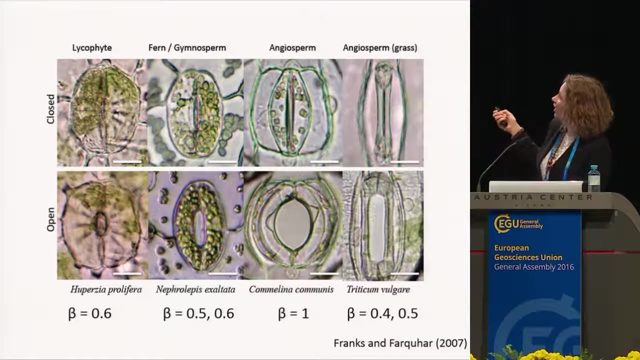 Pennsylvanian is. we've assessed the Gmax of these species. what is their maximum theoretical stomatal conductance and put it in context of the modern vegetation? You have to make a number of assumptions. These are different types of plants: stomata closed and stomata open. 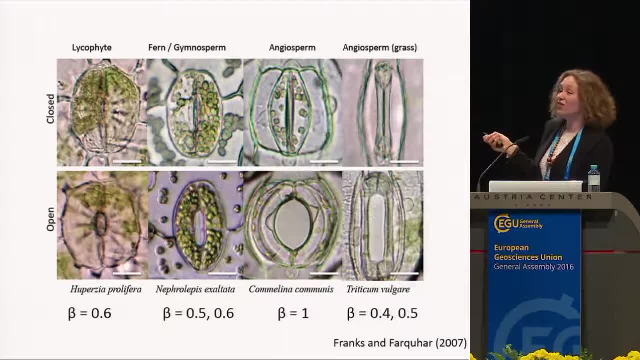 and you apply different scaling relationships, And because these plants are extinct, it's hard to know what to apply. so we've gone with the most conservative approach and assumed that stomata of these extinct plants only open their stomatal pores to half of a circle. 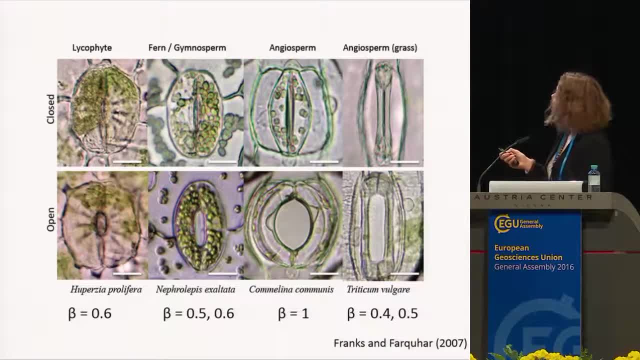 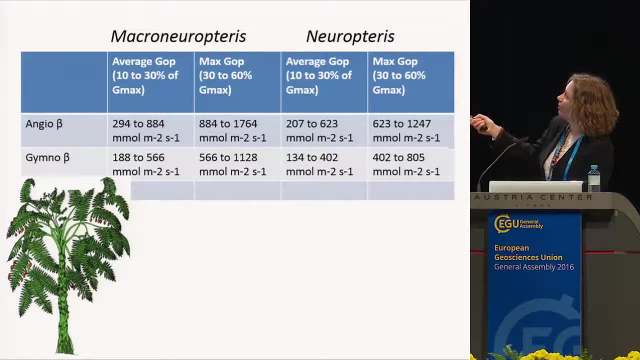 basically an ellipse rather than the angiosperm form. here We've got two genera and these are different scaling factors and I'm going to plus a data set, which is a data set of the stomata, and I'm going to plus a data set of the stomata and I'm 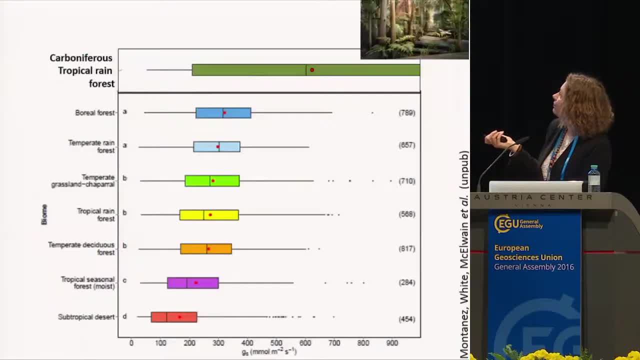 which applies the most conservative scaling factors. So here's the modern data set. This is modern vegetation and this is carboniferous vegetation, and this is really early data and it's unpublished. And this is of all of the key species present in a carboniferous ecosystem. 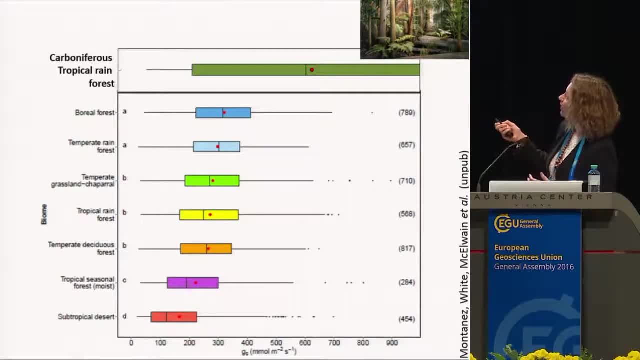 and I'm putting it up here in its raw form just to demonstrate that we are so often badly influenced by the modern And in the fossil record. I think as we begin to apply this type of approach, we're going to see lots of examples where the potential of paleovegetation to modulate 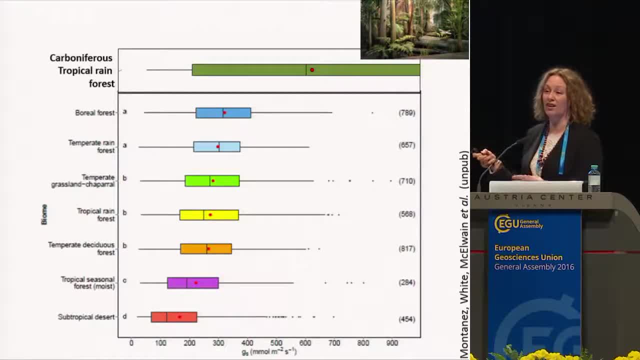 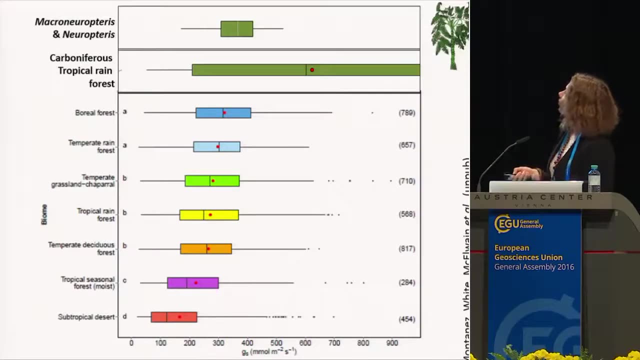 climate and to influence the global hydrological cycle is much greater than the modern, Because what this shows is that the rate at which carboniferous plants can exchange gas with the atmosphere is off the scale compared to all modern vegetation, If we just look at the macroneurocterous and neurocterous- and this is a much more robust data- 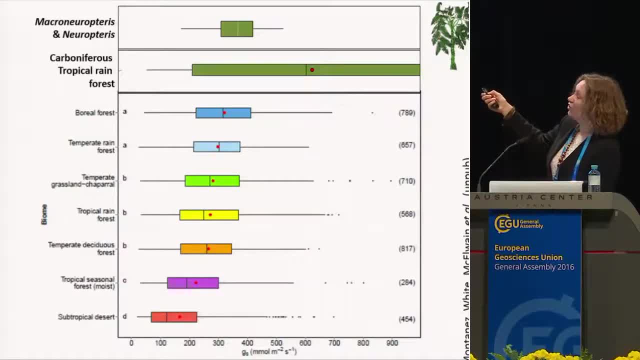 set, it's still much higher- has higher stomatal conductance rates than all of these modern biome types. So I think we've got enough proxies. now What we can begin to do is apply the paleobiosphere models, paleovegetation models, and assign a paleo function, rather than running a 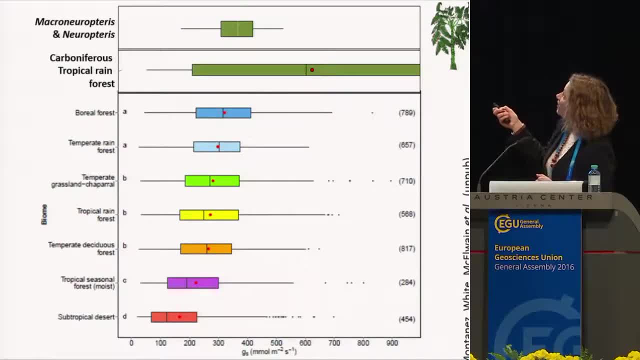 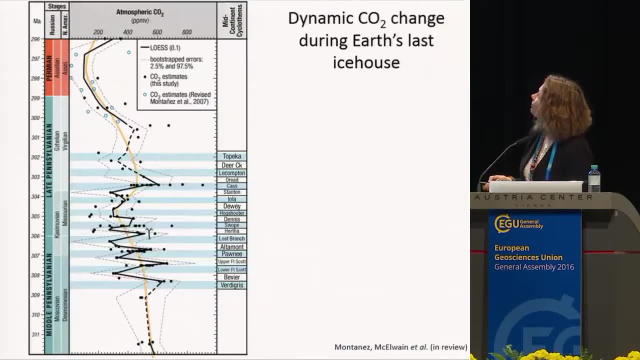 paleo model with a modern vegetation to really assess what rate the paleovegetation can influence atmospheric and climatic processes. We've reconstructed carbon dioxide levels through the carboniferous. So this is 10 million year CO2 record based on paleosol method and also the 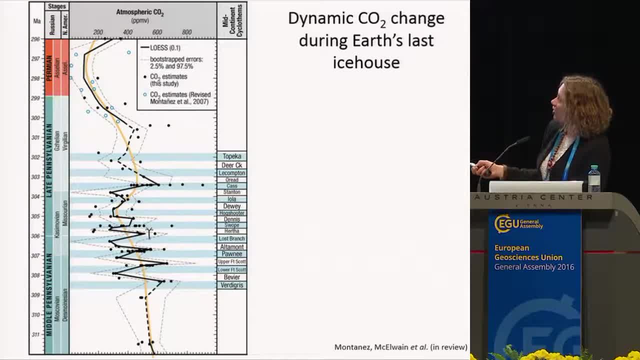 stomatal density proxy And it's a very exciting record. It shows these glacial interglacial transitions all the way through the carboniferous. And it's a very exciting record. It shows these glacial interglacial transitions all the way through the carboniferous, With CO2 lows of about 200,. 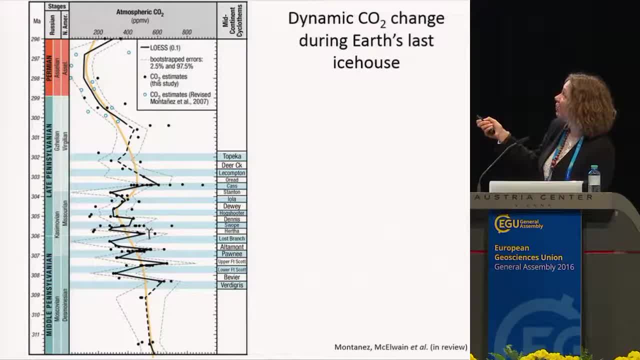 similar to the quaternary and CO2 highs much higher, up to 600 and 700 ppm. What we're now going to do is take our functional data sets through these glacial interglacial transition and assess at what rate could the tropical forests of the carboniferous have influenced the whole climate system through. 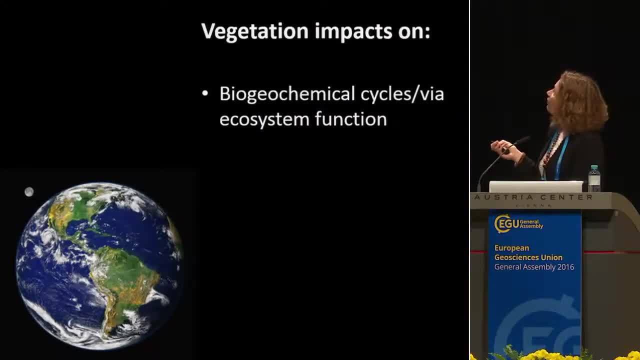 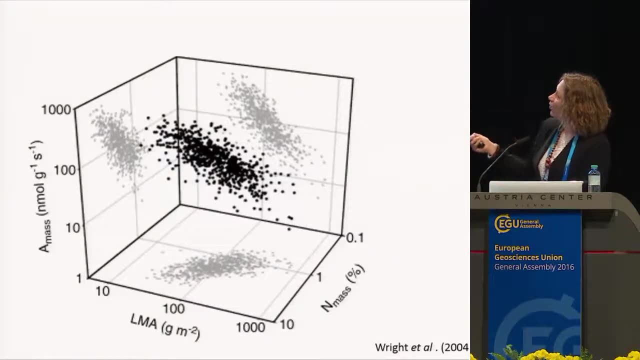 this interval. So what I want to finish on is looking at how vegetation impacts can influence biogeochemical cycles, And to do this we need proxies of ecosystem function in the past, And one of the best proxies we could develop would enable us to fit into this modern ecological 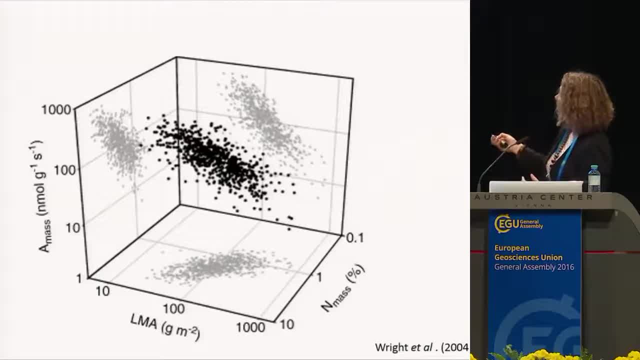 space, which is called the leaf economic spectrum, And this is a huge data set by Ian Wright in Australia. And what this graph plots here is photosynthetic rates, so any enzymatic biochemical process- And this is a huge data set by Ian Wright in Australia. And what this graph plots here is: 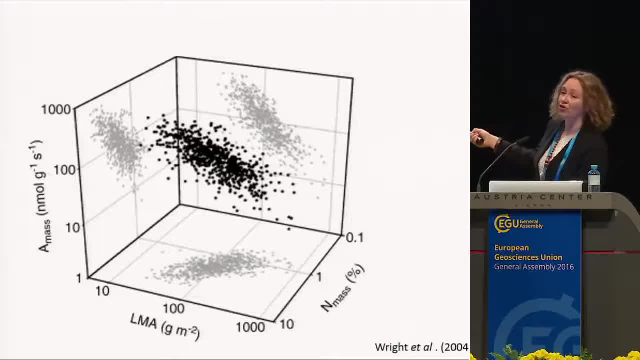 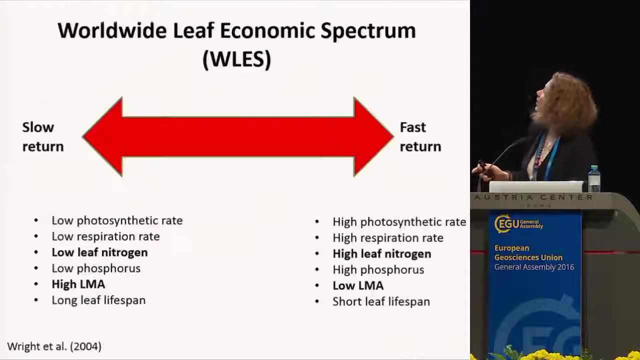 photosynthetic rates, so any enzymatic biochemical process, Against the proportion of nitrogen in plant tissue and against this parameter here, leaf mass per area. And this functional space can explain all species all across the globe. And if I explain it in a little bit more simple way, there's two. 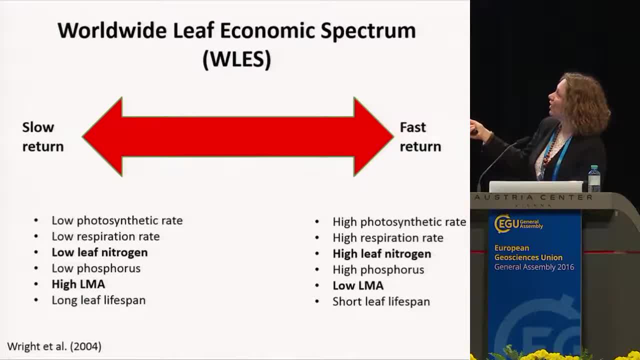 extreme ends of this leaf functional space. A slow return end- this is plants which have low biochemical rates, low photochemical rates. and a slow return end, which is plants which have low photosynthetic rates, low respiration rates, low nitrogen and they have high leaf mass per area. 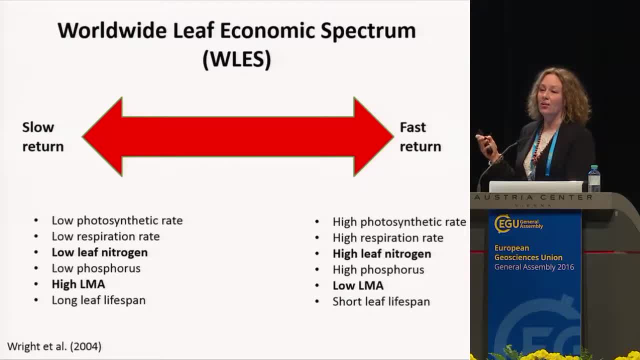 On the other return is the fast return end. These are basically live fast, die young. They have high biochemical rates, high photosynthetic rates, high respiration rates, high leaf nitrogen, which is quickly recycled back into the ecosystem, And they have low LMA. So if we can develop a 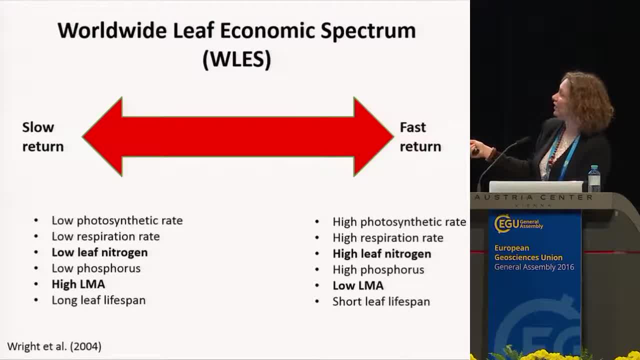 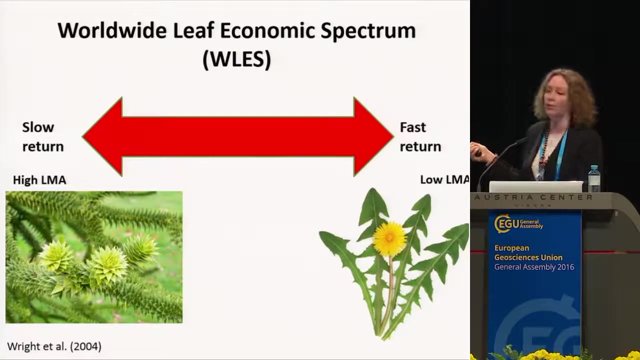 proxy for leaf mass per area, because we understand how leaf mass per area is interrelated and correlated with all of these other functional traits of the vegetation. then we have a proxy which will assess: is the recycling with the ecosystem slow or is the recycling with the ecosystem fast? So your archetypal slow return would be monkey. 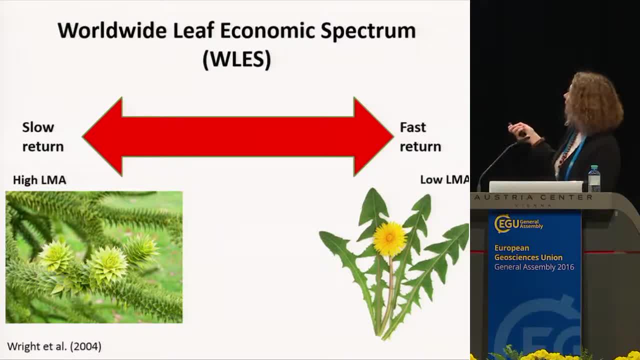 puzzle with a leaf lifespan of about 28 years and the archetypal low LMA plants. fast return would be dandelion, short-lived, high nitrogen. high photosynthetic- low photosynthetic rates- reproduces quickly, dies and sets seed And each of those recycle. 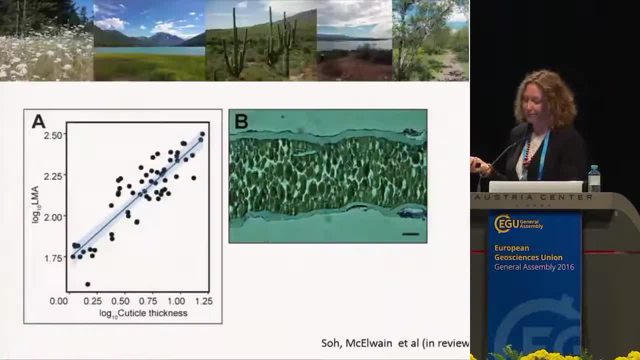 nitrogen at different rates within the ecosystem. So we've developed a new proxy for leaf mass per area, this important ecological trace that opens up all of this understanding of the functioning of the biosphere. And it's very simple: You take a cross-section of a fossil leaf. This is ginkgo. 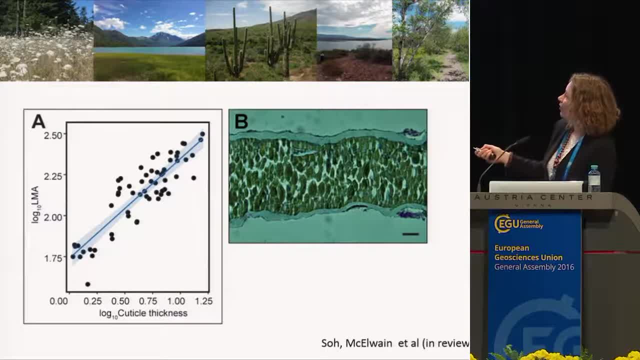 You measure the cuticle thickness And we found a very, very nice scaling relationship between cuticle thickness and LMA. As you increase cuticle thickness, we find that you increase LMA And that makes intuitive sense. A plant which invests. 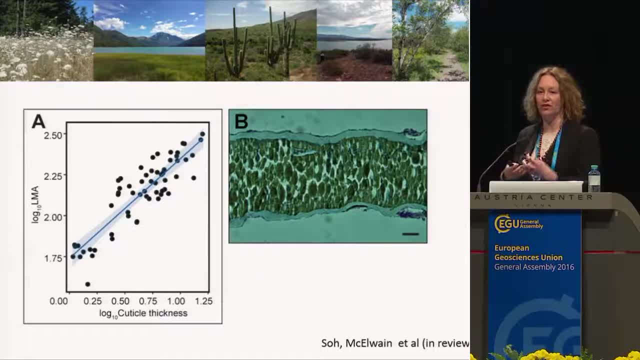 a high proportion of tissue which makes it resistant to decay and protected from the elements. thick cuticle is a high LMA plant And if you remember high LMA plants, these return nitrogen slowly to the ecosystem, Whereas low LMA plants are fast, quick and they recycle nitrogen quickly. 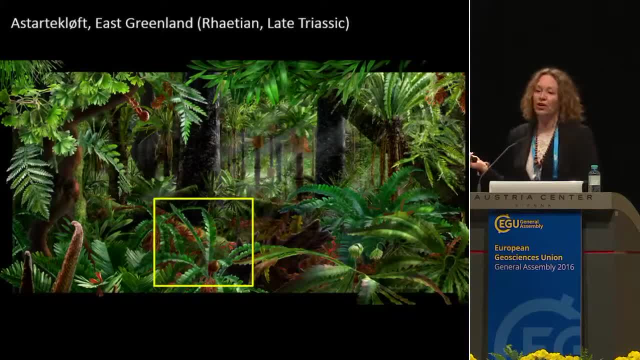 We've applied this proxy to a starter cluft in East Greenland, the Triassic-Jurassic boundary, And we've applied it to two different elements within these paleoecosystems: the Benetotales down here in this reconstruction and ginkgo ales. 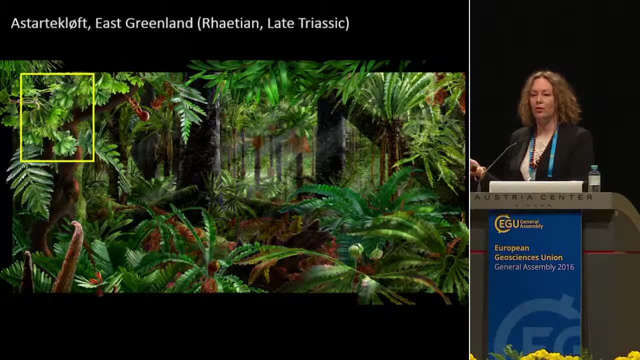 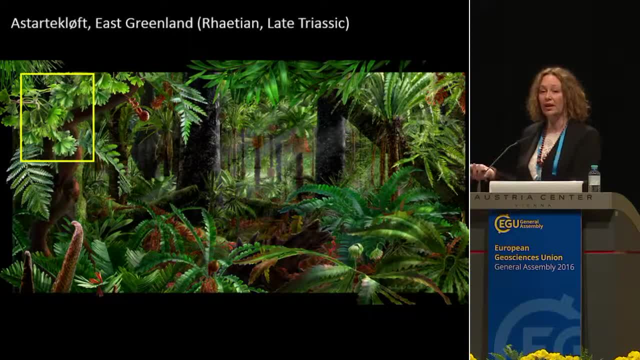 We've applied it to a lot of other plants And we've applied it to a lot of other plants in the vegetation. decreases in biodiversity in the vegetation. decreases in biodiversity in the vegetation. decreases in biodiversity- big ecological upheaval. 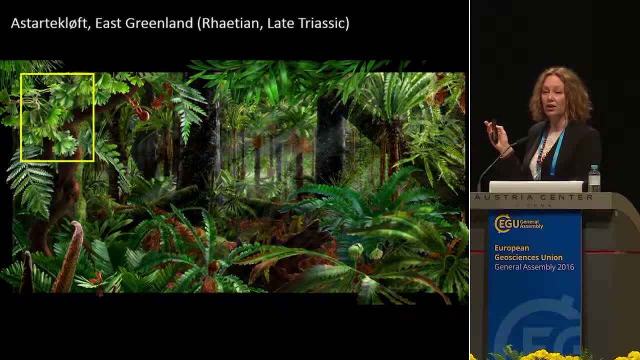 in the vegetation decreases in biodiversity- big ecological upheaval. in the vegetation decreases in biodiversity, big ecological upheaval. But what we've wanted to do, but what we've wanted to do, but what we've wanted to do is add on a functional understanding. 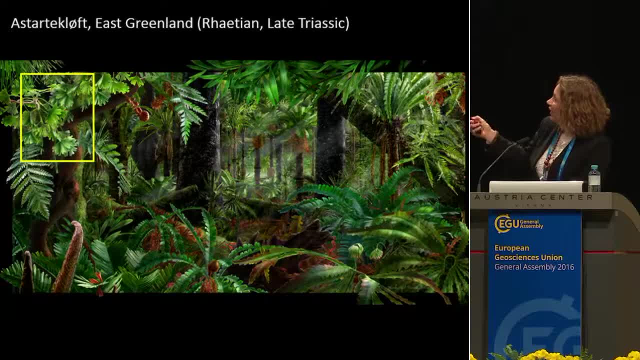 is add on a functional understanding, is add on a functional understanding to this data set, to this data set, to this data set. And we've done that by tracking, And we've done that by tracking, And we've done that by tracking changes in LMA leaf mass per area. 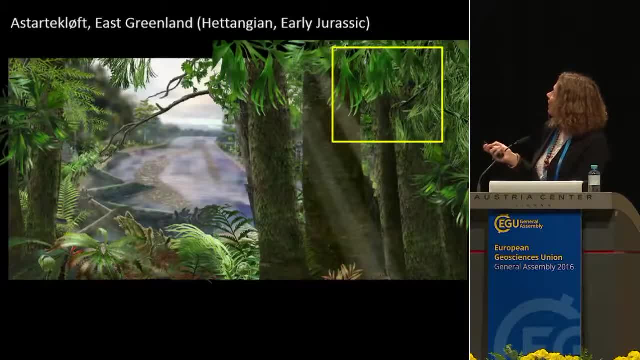 changes in LMA leaf mass per area. changes in LMA leaf mass per area for these plants and these plants, for these plants and these plants, for these plants and these plants In the early Jurassic. In the early Jurassic. 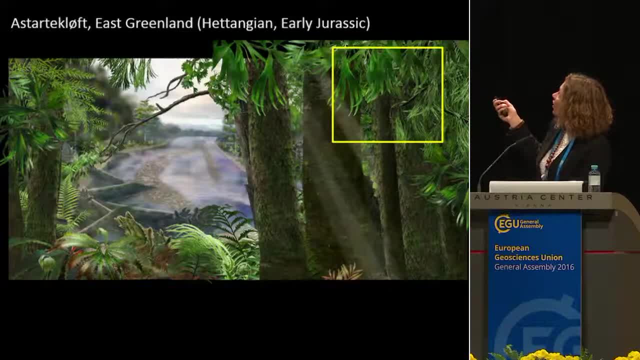 In the early Jurassic. you get a complete ecosystem change. you get a complete ecosystem change. you get a complete ecosystem change and ginkgo ales become the dominance and ginkgo ales become the dominance and ginkgo ales become the dominance, whereas in the latest Triassic. 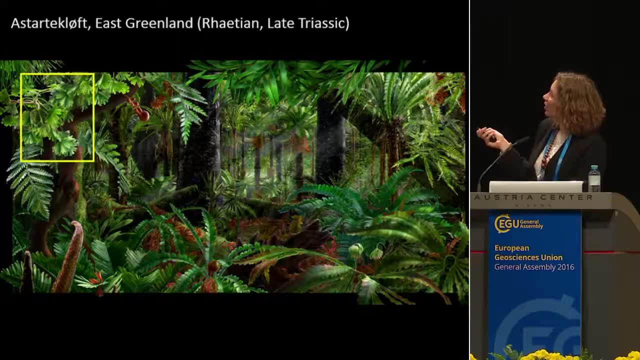 whereas in the latest Triassic, whereas in the latest Triassic, benetatales are the dominance, benetatales are the dominance, benetatales are the dominance. And you can look at a leaf. And you can look at a leaf. 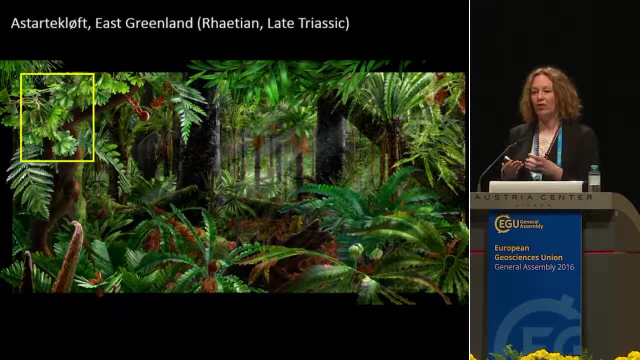 And you can look at a leaf and you can assess its transpiration and you can assess its transpiration and you can assess its transpiration. There's no way of measuring leaf mass. There's no way of measuring leaf mass. There's no way of measuring leaf mass per area, unless you take a cross. 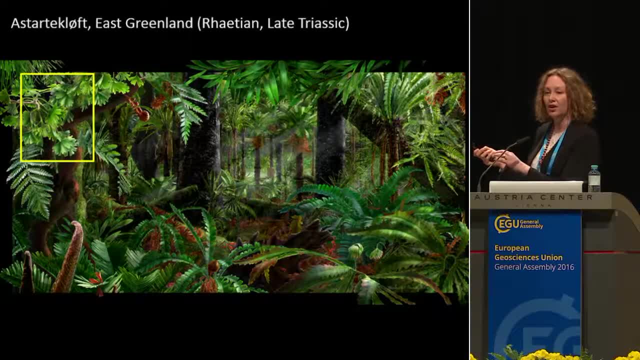 per area unless you take a cross per area, unless you take a cross section of the fossil leaves. section of the fossil leaves. section of the fossil leaves. Look at cuticle thickness and use Look at cuticle thickness and use. Look at cuticle thickness and use that as a proxy for leaf mass per. 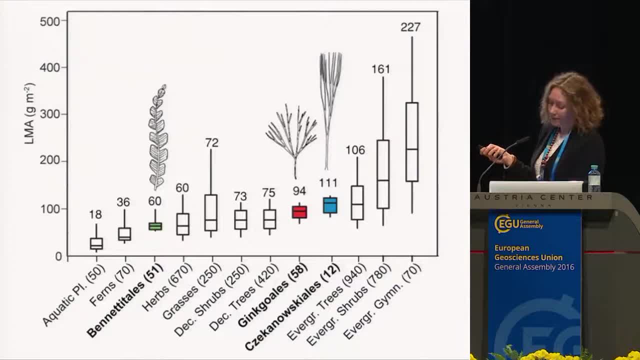 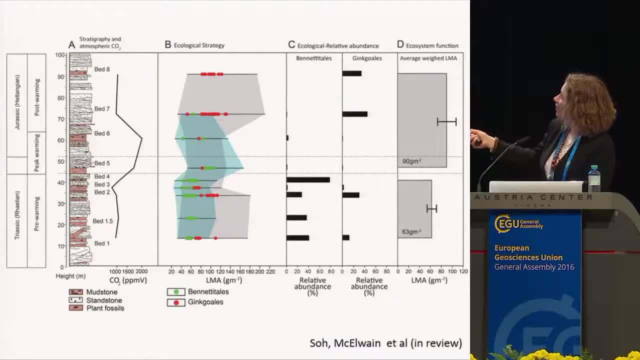 I'm going to skip to the final data set. I'm going to skip to the final data set. So here we have, So here we have. So here we have the Triassic-Jurassic boundary, the Triassic-Jurassic boundary, the Triassic-Jurassic boundary: Here's a CO2 reconstruction of 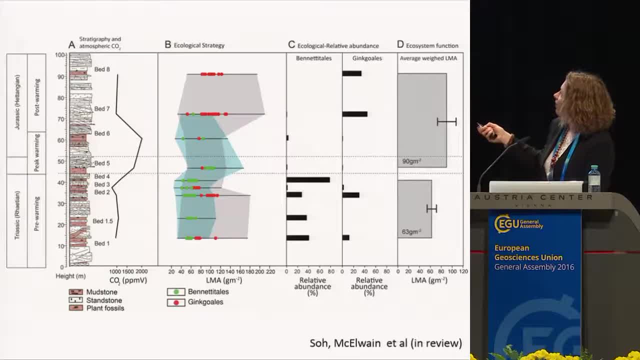 Here's a CO2 reconstruction of. Here's a CO2 reconstruction of Margaret Steinthorst-Dottir in the Margaret Steinthorst-Dottir in the Margaret Steinthorst-Dottir in the room room room. This tracks ecological strategy of. 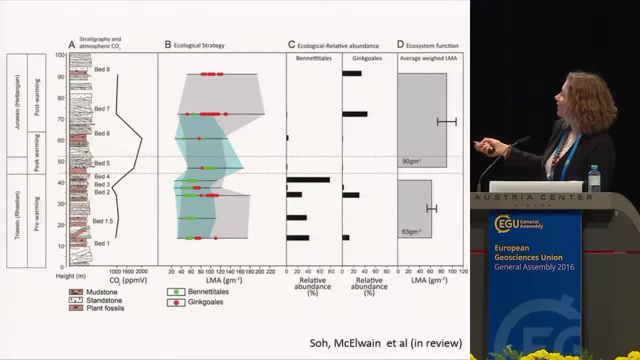 This tracks ecological strategy of. This tracks ecological strategy of those two key plant types: the those two key plant types. the those two key plant types: the Benetotales and Ginkoales. Benetotales and Ginkoales. 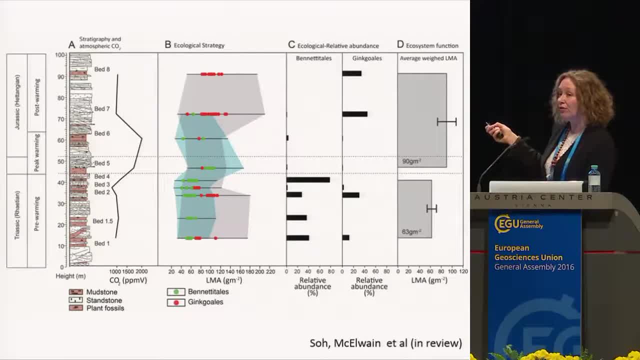 Benetotales and Ginkoales. We have relative abundance data. We have relative abundance data. We have relative abundance data based on macro fossils and also based on macro fossils and also based on macro fossils and also pollen of Luke Mander, who's in. 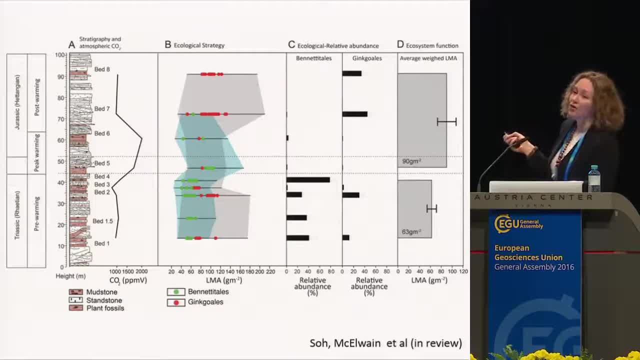 pollen of Luke Mander. who's in pollen of Luke Mander, who's in the audience, the audience, the audience, And here's the LMA data, And here's the LMA data, And here's the LMA data. So what we've done is we've looked. 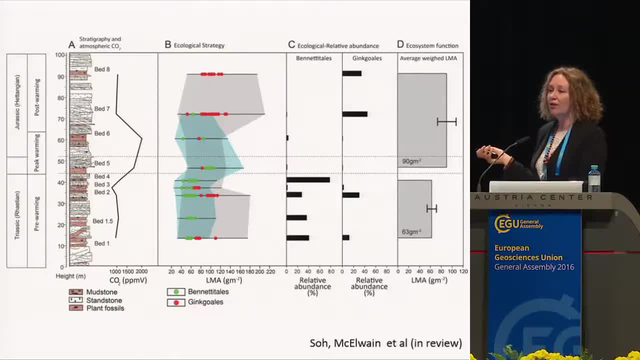 So what we've done is we've looked. So what we've done is we've looked at a community weighted leaf mass, at a community weighted leaf mass, at a community weighted leaf mass per area before and after the per area, before and after the per area before and after the Triassic-Jurassic boundary. 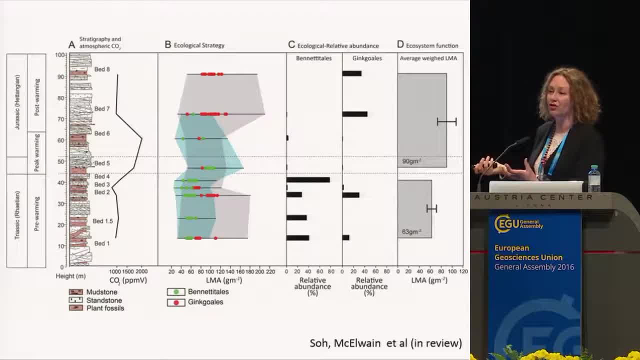 Triassic-Jurassic boundary, Triassic-Jurassic boundary. because we have all of the, because we have all of the, because we have all of the elements needed to assess, the elements needed to assess, the elements needed to assess the vegetation functionally. 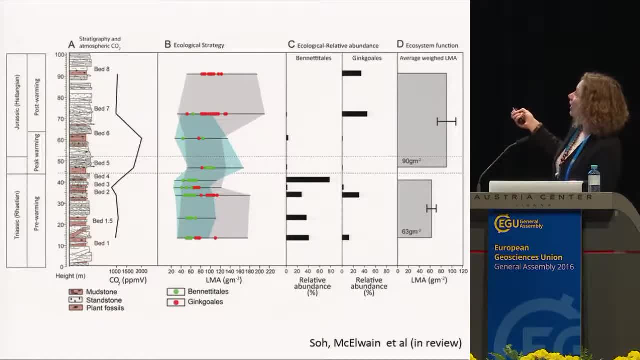 vegetation functionally. vegetation functionally And in a nutshell what it shows, And in a nutshell what it shows. And in a nutshell what it shows is that leaf mass per area of. is that leaf mass per area of? is that leaf mass per area of the vegetation before the? 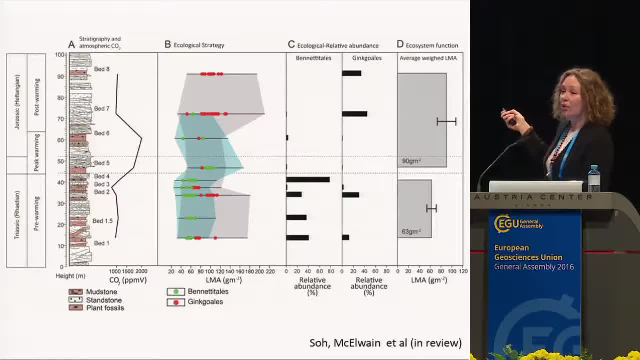 the vegetation before the. the vegetation before the boundary is very low. boundary is very low. boundary is very low. These are low LMA plants. These are low LMA plants. These are low LMA plants. They would have recycled nitrogen. They would have recycled nitrogen. They would have recycled nitrogen very fast through the ecosystem, very fast through the ecosystem, very fast through the ecosystem. They would have lost water at. They would have lost water at. They would have lost water at high rates, high rates, high rates. They would have had very rapid. 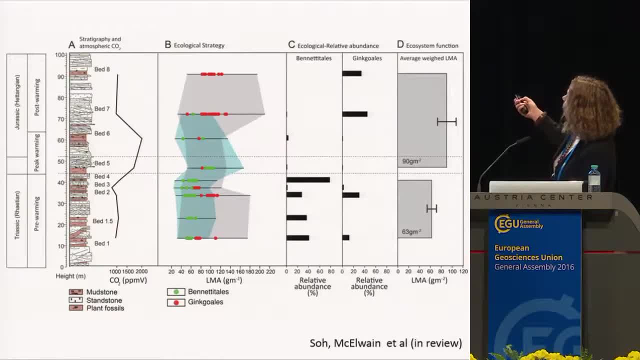 They would have had very rapid, They would have had very rapid photosynthetic rates, photosynthetic rates, photosynthetic rates. Whereas post-boundary we see this, Whereas post-boundary we see this, Whereas post-boundary we see this big increase in the LMA of the 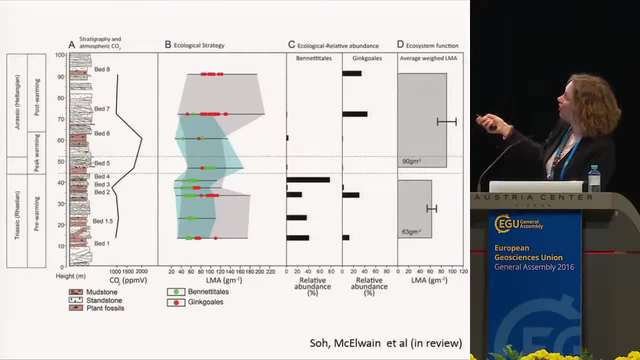 big increase in the LMA, of the big increase in the LMA of the ecosystem, ecosystem, ecosystem. So what this shows is that the. So what this shows is that the So what this shows is that the Triassic-Jurassic mass extinction- Triassic-Jurassic mass extinction. Triassic-Jurassic mass extinction boundary. not only did it cause boundary, not only did it cause boundary, not only did it cause extinction of species and extinction of species and extinction of species and individuals and result in individuals and result in individuals and result in ecological change, it also. ecological change. it also ecological change. it also fundamentally changed the fundamentally changed. the fundamentally changed the functioning of the ecosystems, functioning of the ecosystems, functioning of the ecosystems, So that post-boundary these, So that post-boundary these, So that post-boundary these would have been stress-tolerant. 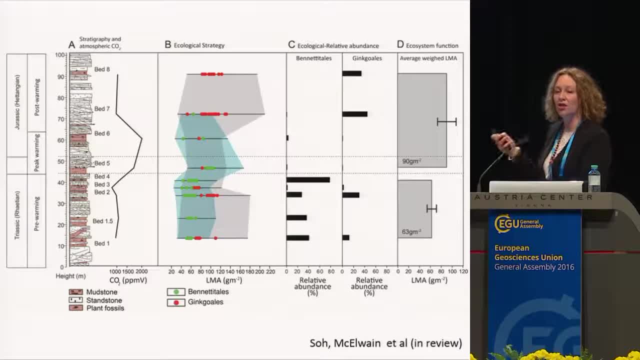 would have been stress-tolerant, would have been stress-tolerant long-leaf lifespan, the long-leaf lifespan, the long-leaf lifespan. the vegetation would have invested a vegetation would have invested a vegetation would have invested a lot into preserving the leaves. 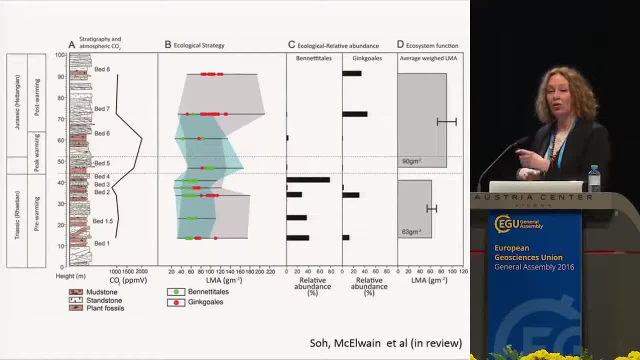 lot into preserving the leaves, lot into preserving the leaves for a long time, for a long time, for a long time, And, as a result, everything, all And, as a result, everything, all And as a result, everything, all elements would have been recycled. 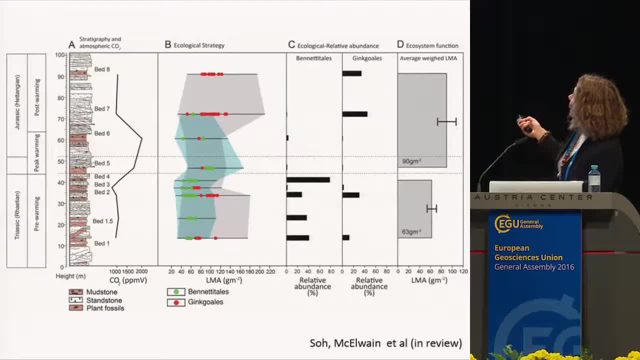 elements would have been recycled. elements would have been recycled very slowly through that system, very slowly through that system, very slowly through that system. So it's like going from a. So it's like going from a. So it's like going from a tropical, rainforest-type system. 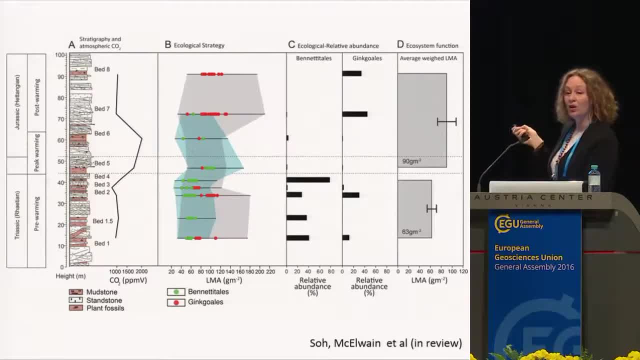 tropical rainforest-type system, tropical rainforest-type system to a boreal forest-type system, to a boreal forest-type system, to a boreal forest-type system. And we can only do that if you, And we can only do that if you, And we can only do that if you can apply these modern proxies to. 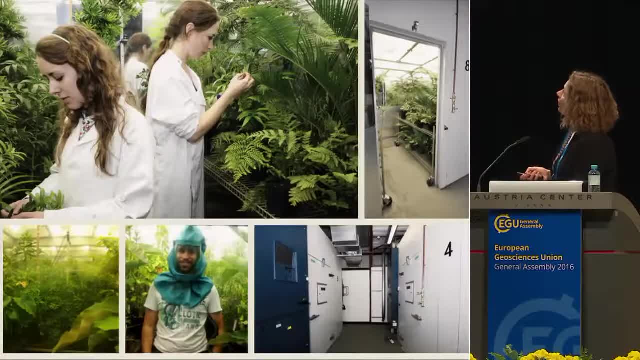 can apply these modern proxies to, can apply these modern proxies to the paleo data, the paleo data, the paleo data. So, does this stack up? if you So, does this stack up? if you So, does this stack up if you actually do, if you do experimental? 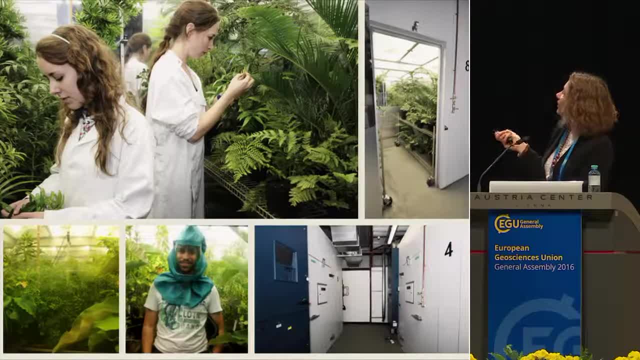 actually do, if you do experimental actually do, if you do experimental tests in plant growth chambers, tests in plant growth chambers, tests in plant growth chambers like we have in UCD and expose like we have in UCD and expose like we have in UCD and expose living plants to high CO2, low O2. living plants to high CO2, low O2. living plants to high CO2, low O2. atmospheres like we think we're atmospheres, like we think we're atmospheres like we think we're around at the Triassic-Jurassic- around at the Triassic-Jurassic. 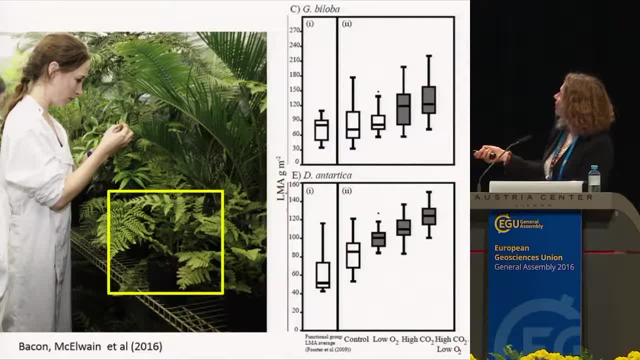 around at the Triassic-Jurassic boundary boundary boundary. This is work of Karen Bacon. This is work of Karen Bacon. This is work of Karen Bacon, who's also in the audience. who's also in the audience. who's also in the audience where she's looking at leaf mass. 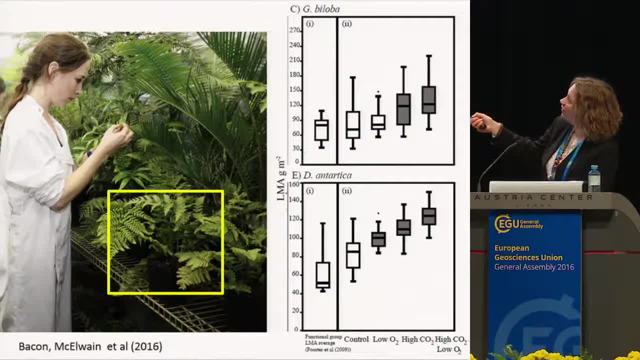 where she's looking at leaf mass, where she's looking at leaf mass per area of two different, per area of two different, per area of two different plants- Ginkgo, which is just here, plants Ginkgo, which is just here, plants Ginkgo, which is just here in the background, and Dixonia. 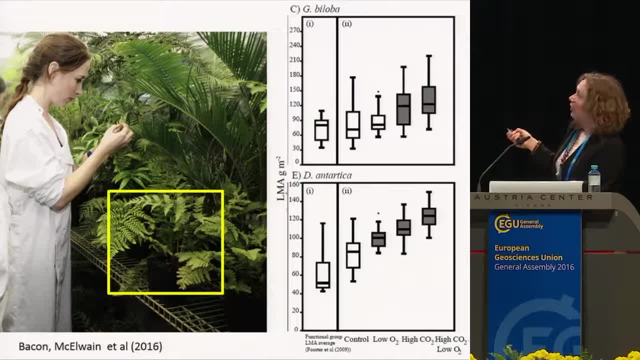 in the background and Dixonia in the background and Dixonia which is here, which is here, which is here. Plants growing in ambient Plants growing in ambient Plants growing in ambient atmospheres have low LMA atmospheres have low LMA. atmospheres have low LMA When you expose them experimentally. When you expose them experimentally, When you expose them experimentally to high CO2 atmospheres, they to high CO2 atmospheres, they to high CO2 atmospheres, they develop high LMA. 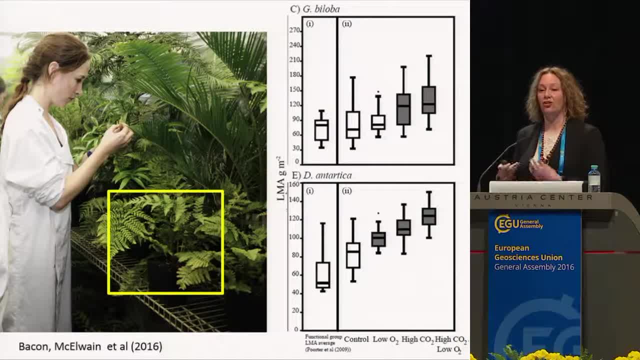 develop high LMA, develop high LMA. So not only do we see this in the, So not only do we see this in the, So not only do we see this in the paleo record, this change in paleo record, this change in. 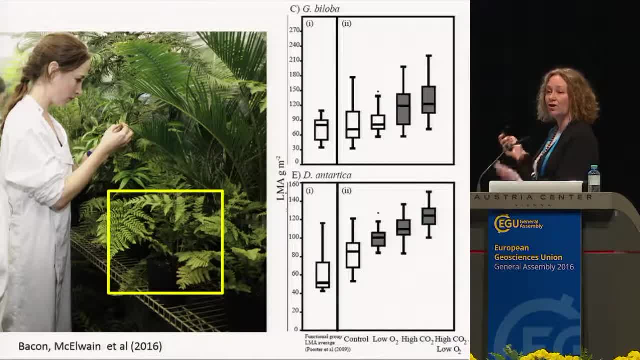 paleo record this change in functioning of vegetation, we functioning of vegetation, we functioning of vegetation. we can also support it through our can also support it through our can also support it through our experimental findings in plant, experimental findings in plant, experimental findings in plant growth chambers like these at 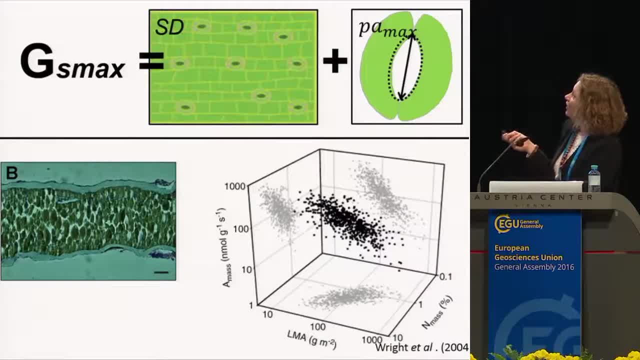 growth chambers like these at growth chambers like these at UCD, UCD, UCD. So, in conclusion, I think that the So in conclusion, I think that the So in conclusion, I think that the paleo community can add hugely. paleo community can add hugely. 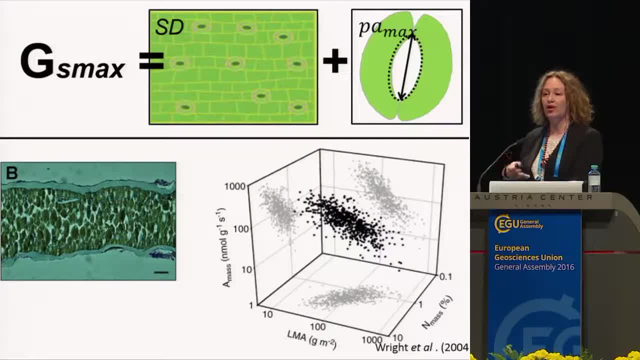 paleo community can add hugely to our understanding of how the to our understanding of how the to our understanding of how the biosphere can modulate climate, biosphere can modulate climate. biosphere can modulate climate and can influence Earth system and can influence Earth system. 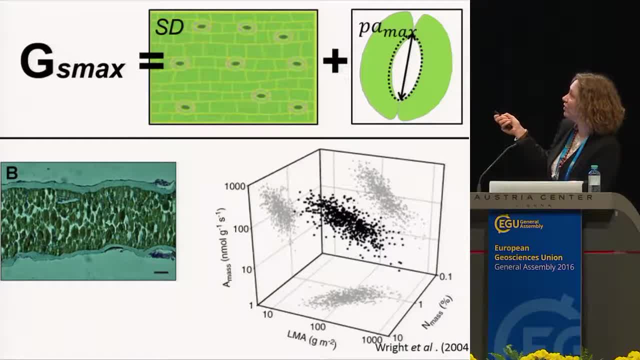 and can influence Earth system processes. by developing proxies processes. by developing proxies processes, by developing proxies that tell us about transpiration, that tell us about transpiration, that tell us about transpiration, proxies that tell us about proxies, that tell us about proxies, that tell us about ecosystem function. 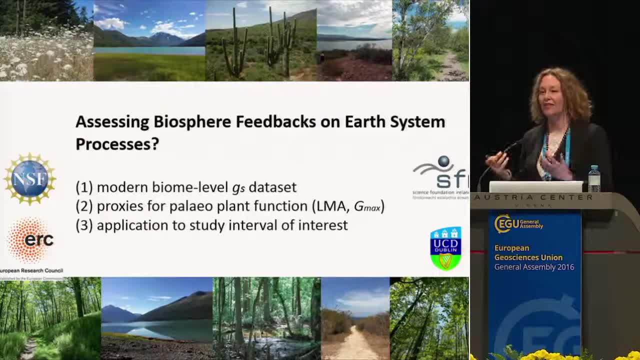 ecosystem function. ecosystem function. And although I think my talk has, And although I think my talk has, And although I think my talk has not provided any answers, I'm not provided any answers. I'm not provided any answers. I'm hoping that it has provided a. 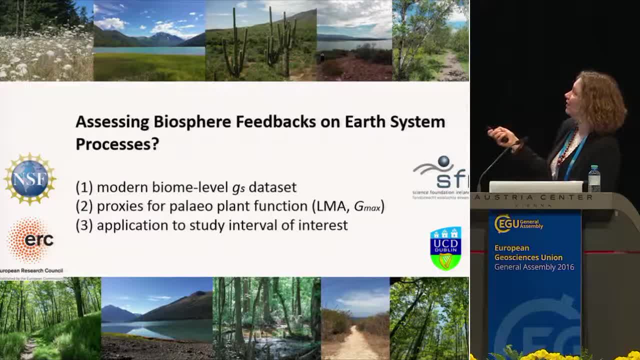 hoping that it has provided a, hoping that it has provided a road map, road map, road map. We need modern biome level data. We need modern biome level data. We need modern biome level data sets to put the paleo record sets to put the paleo record. 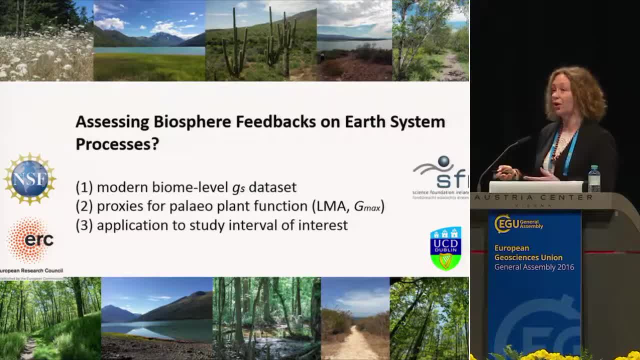 sets to put the paleo record into an Earth system process of into an Earth system process of into an Earth system process of the modern world, the modern world. the modern world We need to develop proxies for, We need to develop proxies for. We need to develop proxies for ecosystem function. in the past, 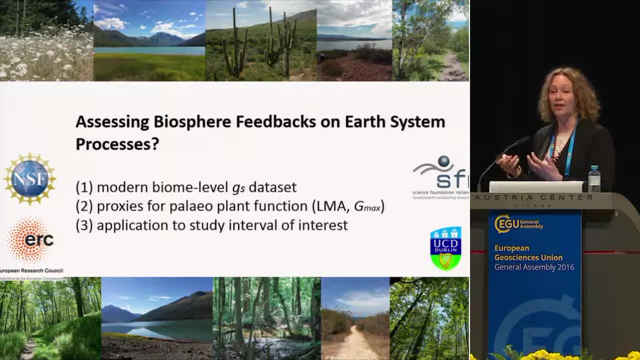 ecosystem function in the past, ecosystem function in the past And I think now that the fund, And I think now that the fund, And I think now that the fund can begin, we can begin to apply, can begin, we can begin to apply, can begin, we can begin to apply these to really well constrained 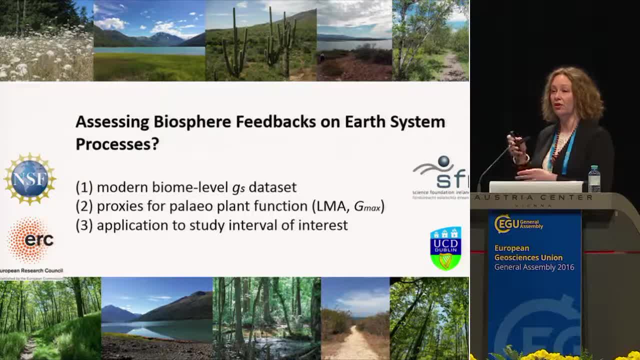 these to really well constrained, these to really well constrained intervals at high resolution intervals at high resolution intervals at high resolution, across mass extinction, across mass extinction, across mass extinction boundaries, across oceanic boundaries, across oceanic boundaries, across oceanic. anoxic events to understand. anoxic events to understand. 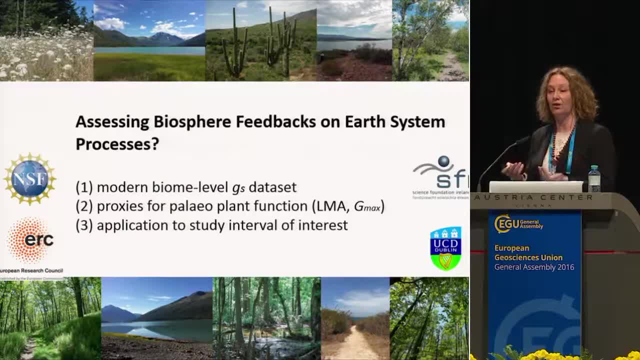 anoxic events to understand. did the biosphere have a greater? did the biosphere have a greater? did the biosphere have a greater influence or a lesser influence? influence or a lesser influence, influence or a lesser influence in terms of Earth system. in terms of Earth system. 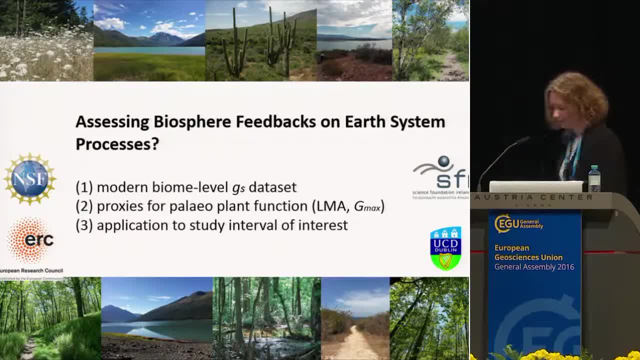 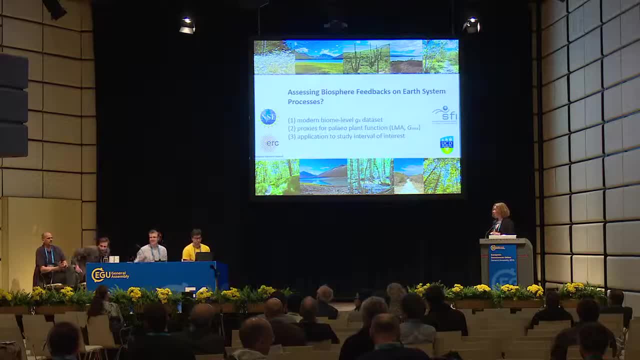 in terms of Earth system, processes at these key intervals, processes at these key intervals, processes at these key intervals in the geological past, in the geological past, in the geological past. Thank you, Thank you, Thank you. Forty-five seconds, Forty-five seconds. 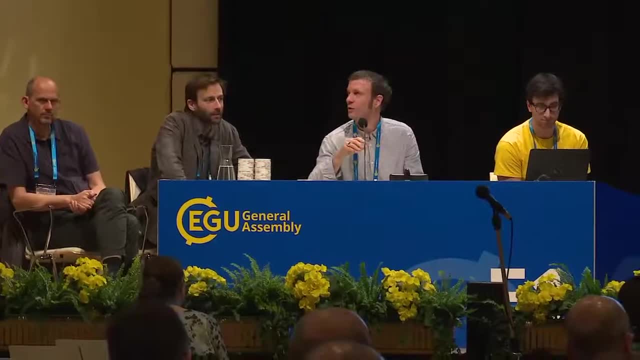 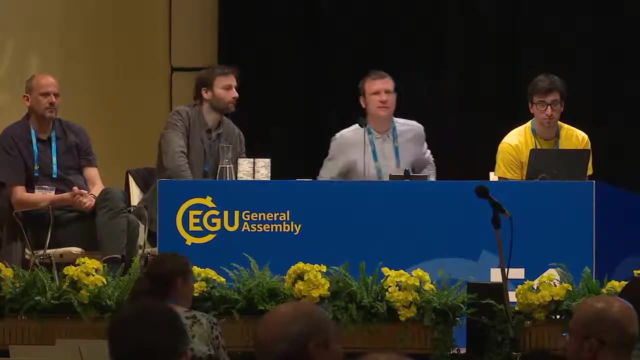 Forty-five seconds, All right, thank you very much. All right, thank you very much, All right. thank you very much, Jennifer, Jennifer, Jennifer, We have time for quick question. We have time for quick question. We have time for quick question. very quick, maybe. 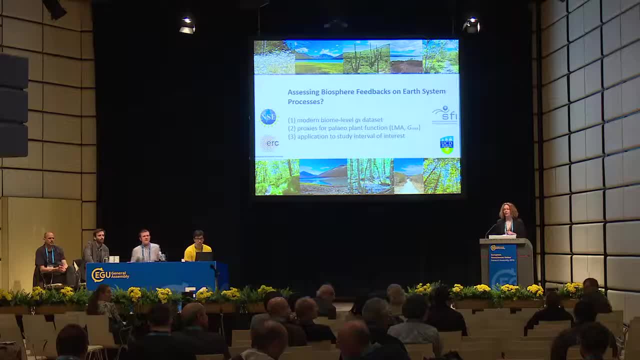 Excuse me. maybe this would be Excuse me, maybe this would be Excuse me, maybe this would be a question, but yesterday I a question, but yesterday I a question, but yesterday I heard that the most dominant heard that the most dominant. 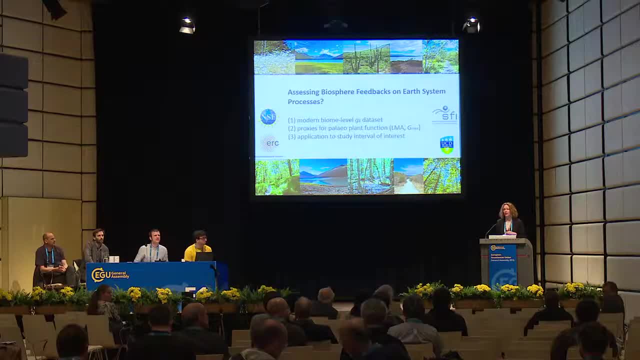 heard that the most dominant vegetation type of Earth today, vegetation type of Earth today, vegetation type of Earth today- is maize, is maize is maize. How would you put your study, How would you put your study, How would you put your study and your concept in this simple? 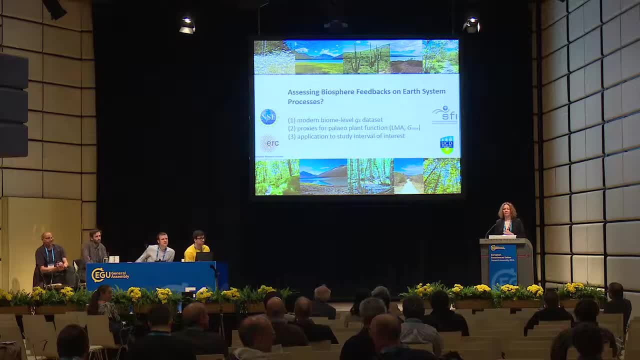 and your concept in this simple, and your concept in this simple practice, practice, practice. We don't have natural ecosystems, We don't have natural ecosystems. We don't have natural ecosystems that could be changed by us, that could be changed by us, that could be changed by us. So, yeah, that's a I would. 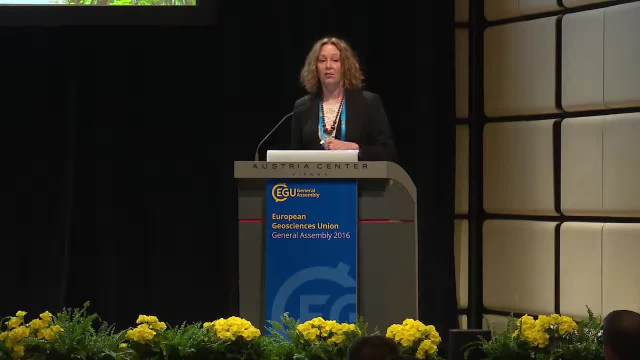 So, yeah, that's a I would. So yeah, that's a I would. yeah, maize is the dominant plant. yeah, maize is the dominant plant. yeah, maize is the dominant plant in crop systems, in crop systems. 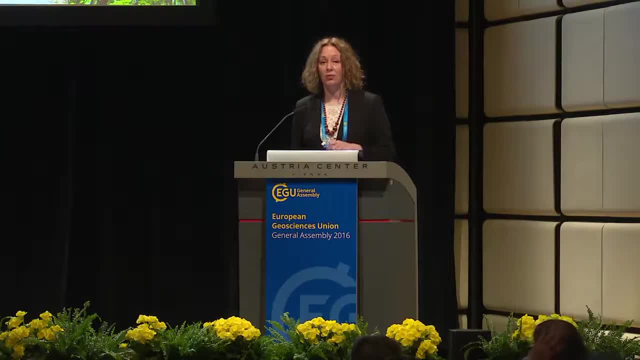 in crop systems. It would be a low LMA plant. It would be a low LMA plant. It would be a low LMA plant and it would have high, and it would have high, and it would have high photosynthetic rates. 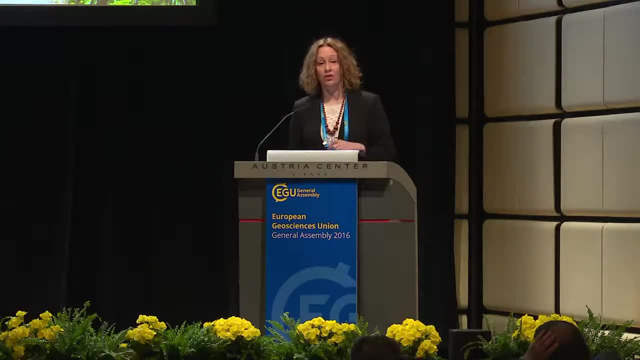 photosynthetic rates. photosynthetic rates, high transpiration rates, high transpiration rates, high transpiration rates, high gas exchange. high gas exchange, high gas exchange. All of our data, we have purposely, All of our data, we have purposely. 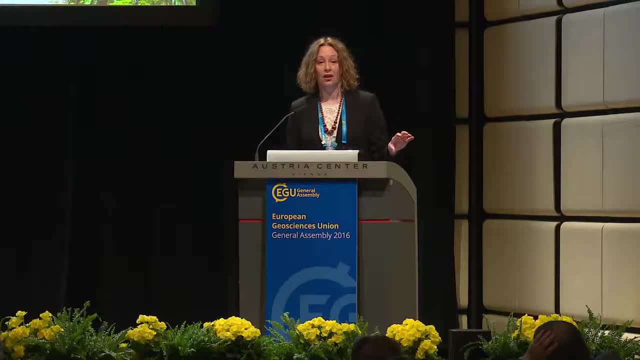 All of our data, we have purposely gone out to the wooded, gone out to the wooded, gone out to the wooded vegetation, vegetation, vegetation. I don't know whether, geographically, I don't know whether, geographically, I don't know whether geographically, perhaps geographically, it is the 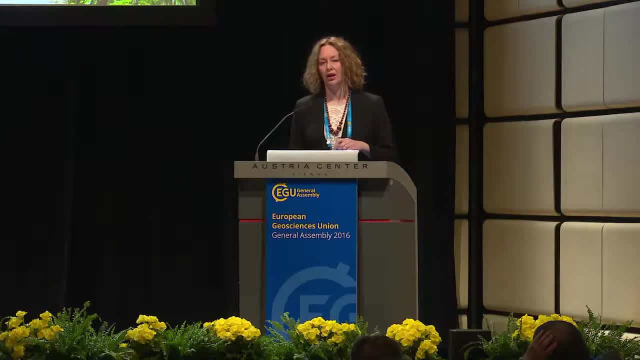 perhaps geographically it is the. perhaps geographically it is the dominant. I haven't looked at dominant. I haven't looked at dominant. I haven't looked at crops in particular, but you crops in particular, but you crops in particular. but you could easily take crop plants. could easily take crop plants, could easily take crop plants. They are assessed as a plant. They are assessed as a plant. They are assessed as a plant functional type, within the functional type, within the functional type, within the biosphere models, and they would biosphere models and they would 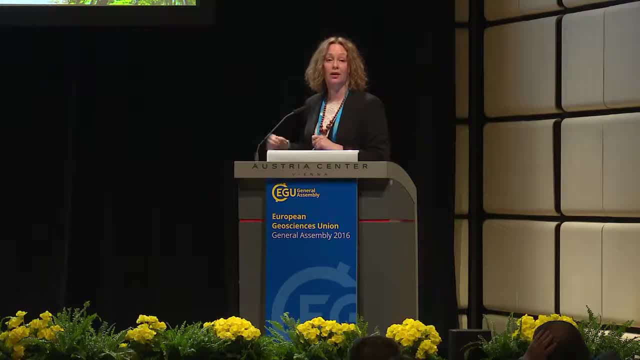 biosphere models and they would be at the extreme end of the be, at the extreme end of the be, at the extreme end of the function in terms of low LMA function, in terms of low LMA function, in terms of low LMA. I suppose, typically, I'm always 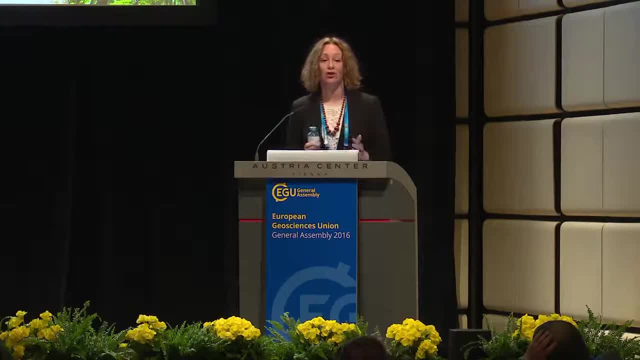 I suppose, typically I'm always, I suppose, typically I'm always wanting to apply these to the wanting to apply these to the wanting to apply these to the paleo records. so we have not paleo records, so we have not paleo records. so we have not looked at the crop plants at all. 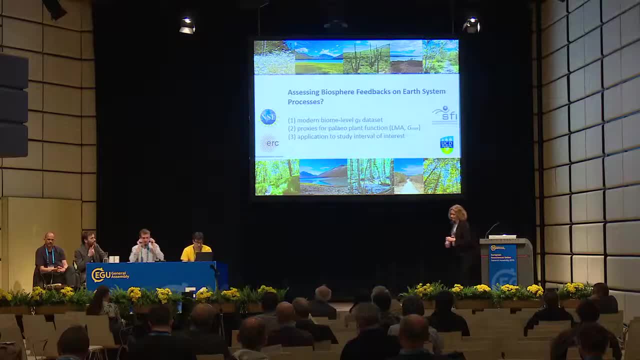 looked at the crop plants at all. looked at the crop plants at all. All right, thank you very much. All right, thank you very much. All right, thank you very much. So it's time to move on to the. So it's time to move on to the. 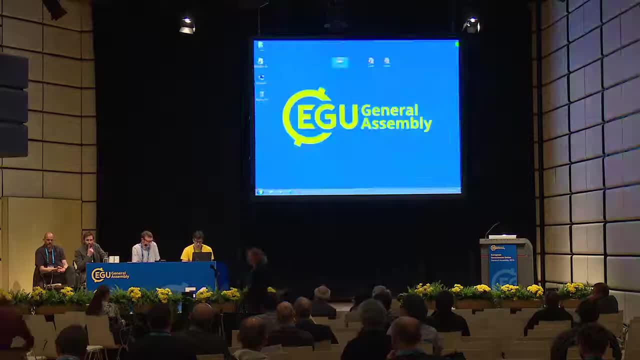 So it's time to move on to the next speaker. who is Carlos next speaker? who is Carlos next speaker? who is Carlos Jaramillo? who is going to talk Jaramillo? who is going to talk Jaramillo? who is going to talk about the evolution of the. 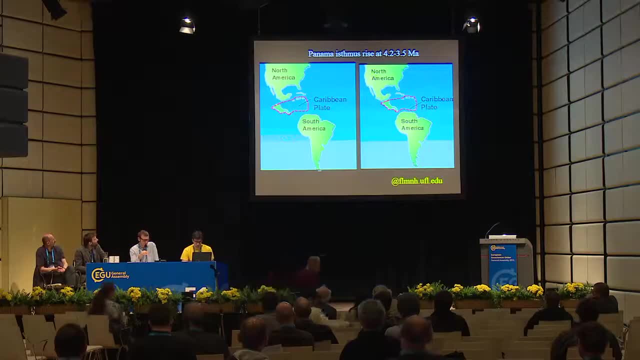 about the evolution of the. about the evolution of the isthmus of Panama. biological isthmus of Panama. biological isthmus of Panama: biological, paleoceanographic and paleoceanographic and paleoceanographic and paleoclimatological implications. 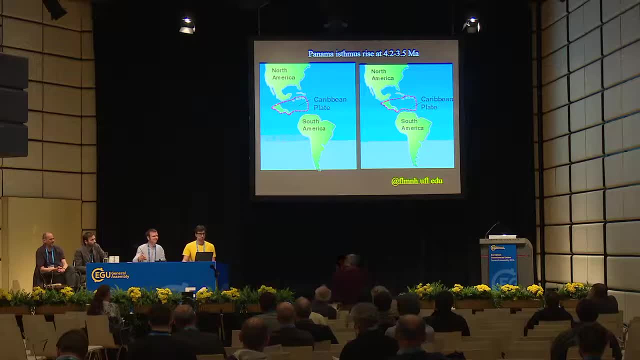 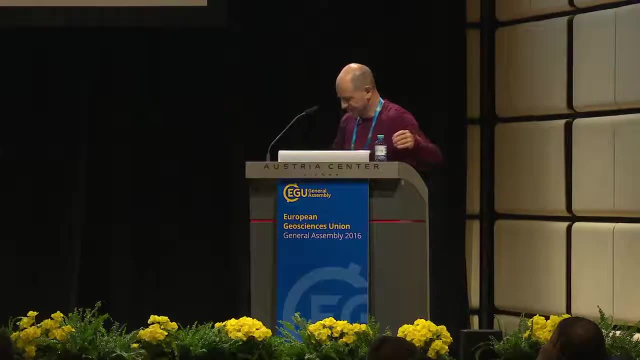 paleoclimatological implications. paleoclimatological implications. Carlos, Carlos, Carlos, Thank you, Thank you, Thank you. Well, I cannot. This is the rise of the isthmus of. This is the rise of the isthmus of. 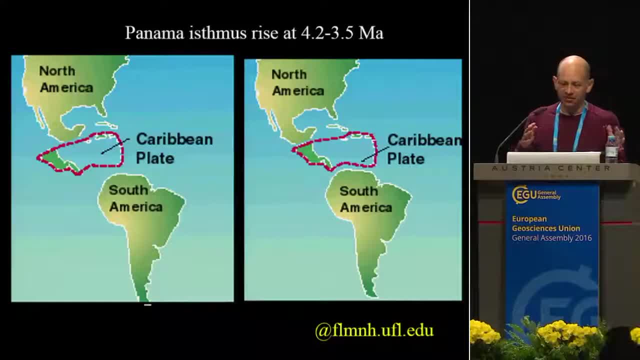 This is the rise of the isthmus of Panama. I think is a good Panama. I think is a good Panama. I think is a good example of where geology, example of where geology, example of where geology, biology and the oceans meet. 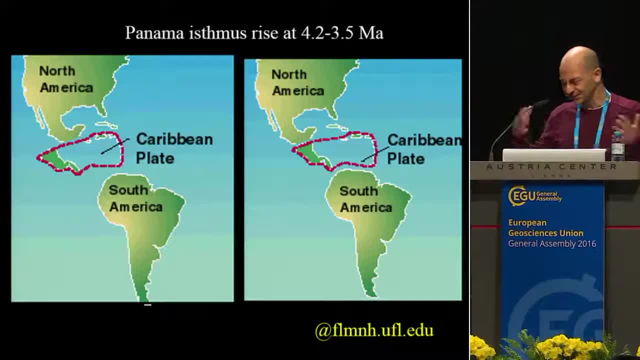 biology and the oceans meet. biology and the oceans meet together, together, together. And even though it's a small, And even though it's a small, And even though it's a small event in a geographical space, event in a geographical space event in a geographical space has, as I will show you, has. 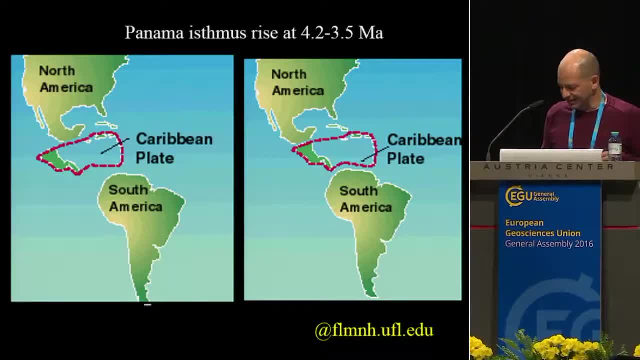 has, as I will show you, has, has, as I will show you, has profound implications in the profound implications in the profound implications in the history of our planet, history of our planet, history of our planet. So, the rise of the isthmus of 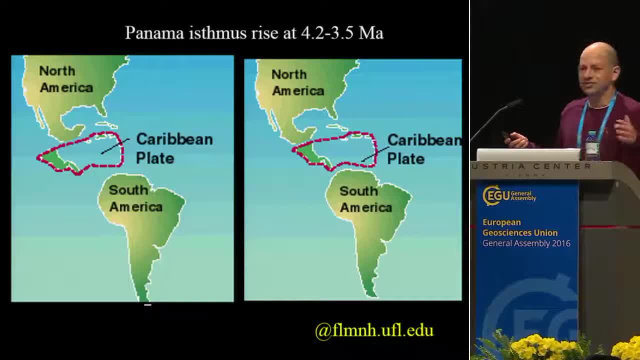 So the rise of the isthmus of, So the rise of the isthmus of Panama is a story that probably Panama is a story that probably Panama is a story that probably you even saw in, you even see in, you even saw in, you even see in. 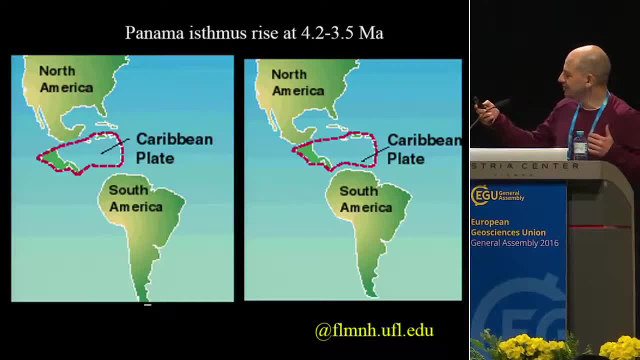 you even saw in, you even see in textbooks for high school, textbooks for high school, textbooks for high school- This geological event where the This geological event, where the This geological event where the rise of the isthmus of Panama, rise of the isthmus of Panama. 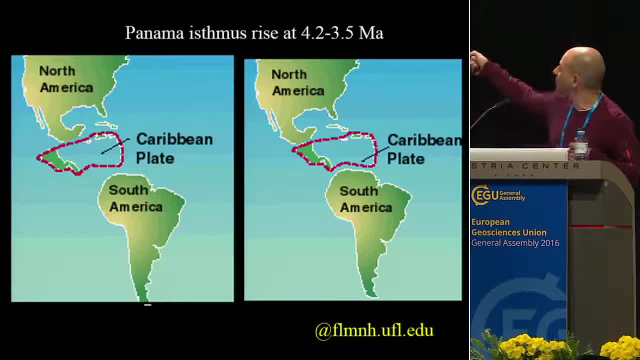 rise of the isthmus of Panama about 3.5 million years ago. about 3.5 million years ago, about 3.5 million years ago, connected two continents that connected two continents. that connected two continents that were isolated for a long time. 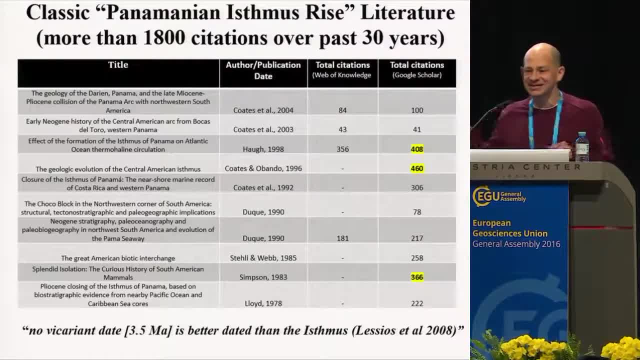 were isolated for a long time, were isolated for a long time And thousands of papers have, And thousands of papers have, And thousands of papers have really cited this idea of the really cited this idea of the really cited this idea of the rise of the isthmus at 3.5. 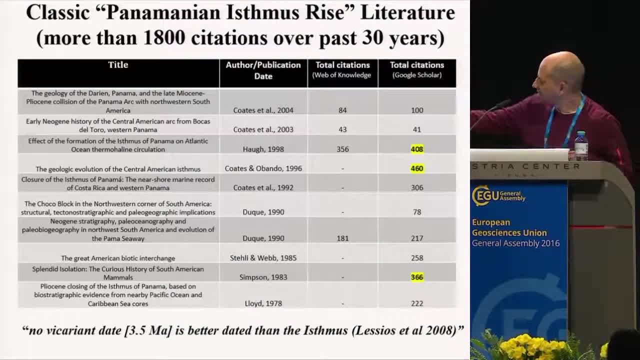 rise of the isthmus at 3.5, rise of the isthmus at 3.5 million years, million years, million years, Even, and you can summarize this, Even, and you can summarize this, Even, and you can summarize this with this quote by Iglesias: 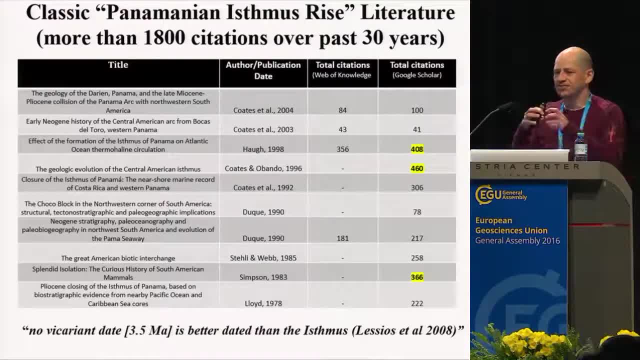 with this quote by Iglesias, with this quote by Iglesias many years ago, that there is many years ago, that there is many years ago that there is not a better example of two, not a better example of two, not a better example of two things getting together than the. 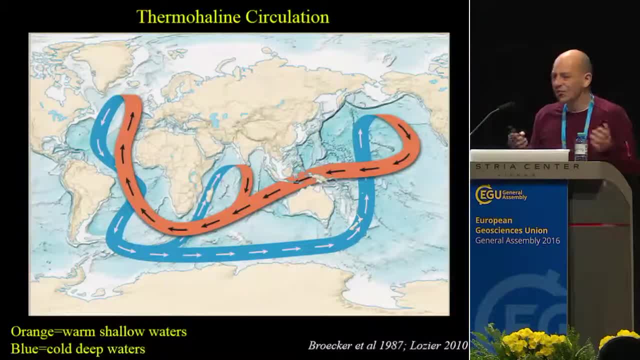 things getting together than the things getting together, than the rise of the isthmus of Panama. rise of the isthmus of Panama. rise of the isthmus of Panama, Even though it's in a geographical, Even though it's in a geographical. 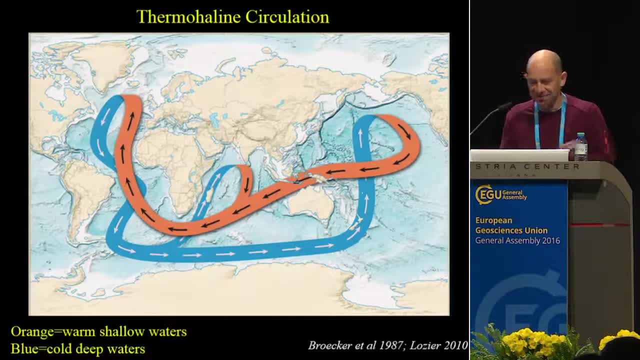 Even though it's in a geographical space, in a very close area, space in a very close area, space in a very close area. just Panama, just Panama, just Panama. Well, because the rise of the isthmus? Well, because the rise of the isthmus. 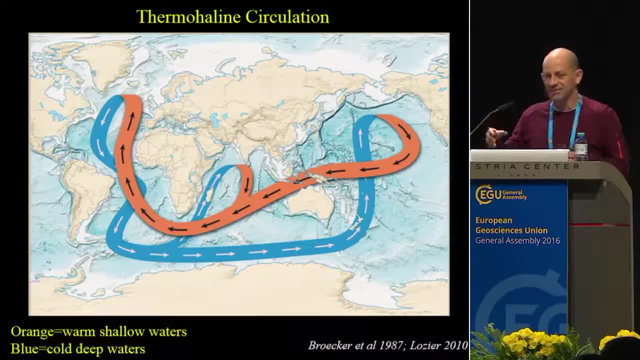 Well, because the rise of the isthmus is linked to four major, has been is linked to four major has been is linked to four major has been thought of being linked to four, thought of being linked to four, thought of being linked to four major events in Earth history. 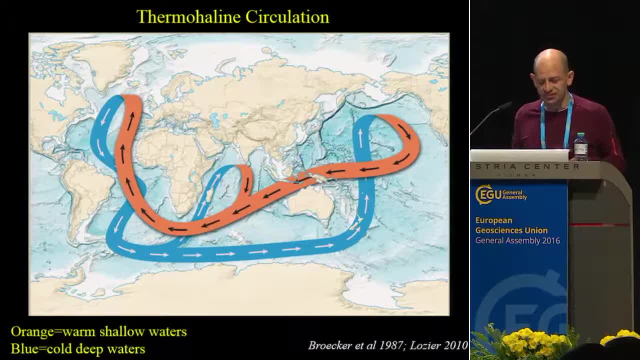 major events in Earth history. major events in Earth history. The first is that once the isthmus. The first is that once the isthmus. The first is that once the isthmus of Panama goes up, it triggers the of Panama goes up, it triggers the. 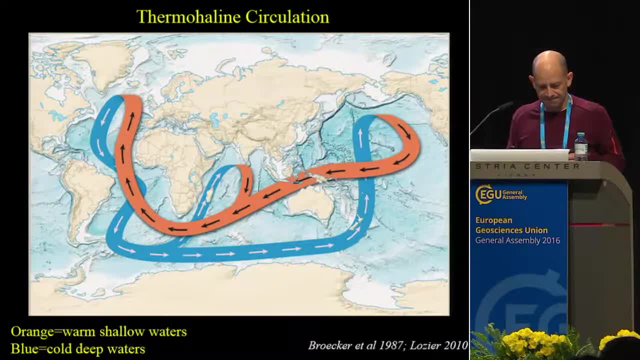 of Panama goes up, it triggers the onset of the thermohaline onset, of the thermohaline onset of the thermohaline circulation, circulation, circulation. The second is that, once the isthmus. The second is that once the isthmus. 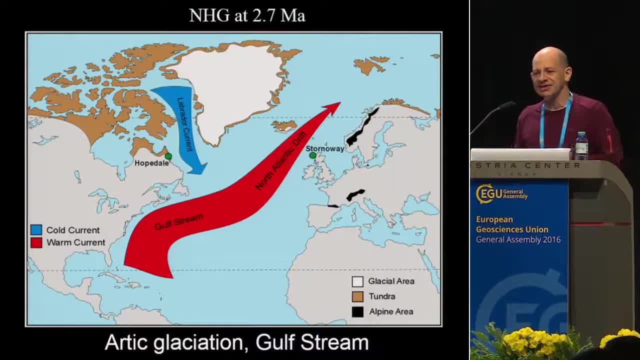 The second is that, once the isthmus goes up, that's the trigger for the goes up. that's the trigger for the goes up. that's the trigger for the beginning of the glaciations in the beginning of the glaciations, in the beginning of the glaciations in the Arctic, 2.7 million years ago. 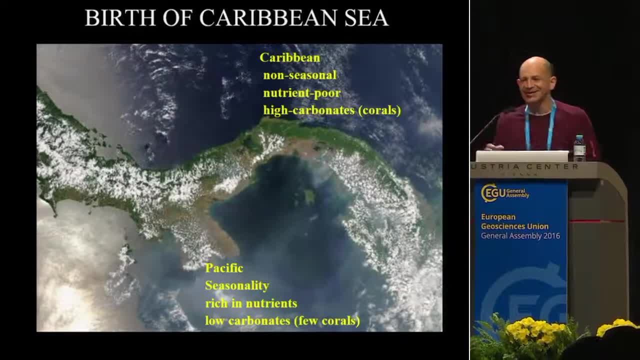 Arctic 2.7 million years ago. Arctic 2.7 million years ago. The third event is once the isthmus. The third event is once the isthmus. The third event is once the isthmus goes up the Caribbean Sea as we. 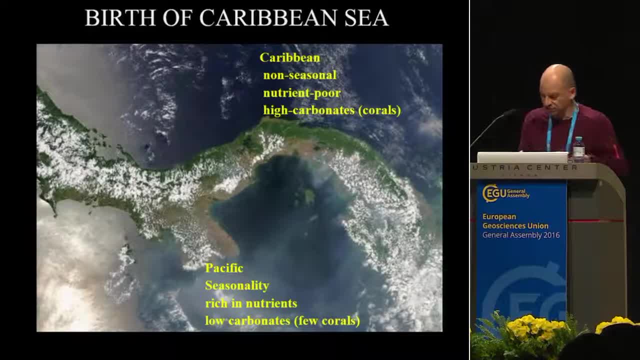 goes up the Caribbean Sea as we goes up the Caribbean Sea, as we know it today, is born. know it today is born. know it today is born. So, as you go to the Caribbean, you, So as you go to the Caribbean, you. 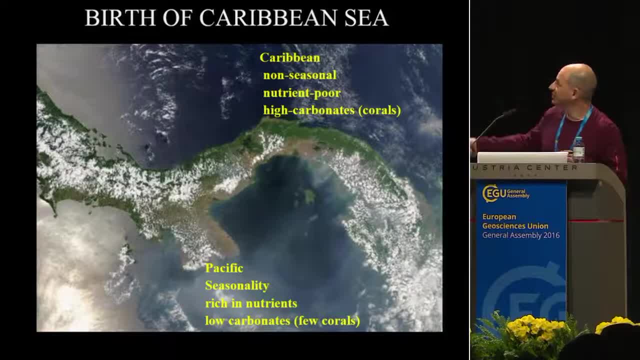 So, as you go to the Caribbean, you will see that it's very different, will see that it's very different, will see that it's very different from the tropical Pacific Ocean, from the tropical Pacific Ocean, from the tropical Pacific Ocean, While the Caribbean is putting 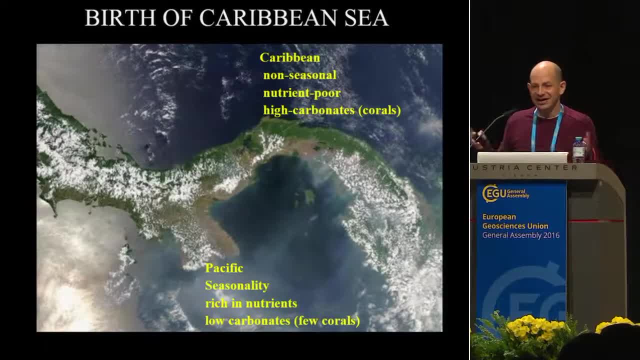 While the Caribbean is putting. While the Caribbean is putting nutrients, the temperature doesn't nutrients. the temperature doesn't nutrients. the temperature doesn't change throughout the year and it change throughout the year and it change throughout the year and it has a lot of carbonates and corals. 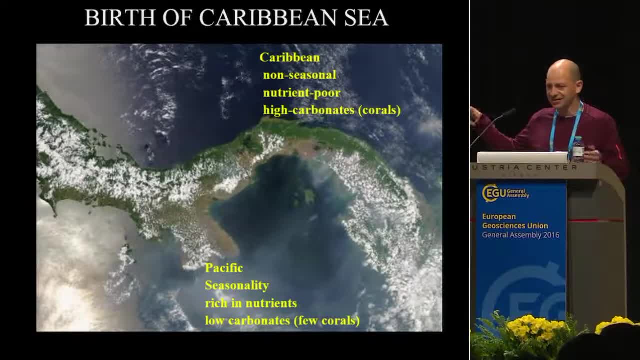 has a lot of carbonates and corals, has a lot of carbonates and corals. The Pacific is really different. The Pacific is really different. The Pacific is really different. It has a season- the temperature. It has a season- the temperature. 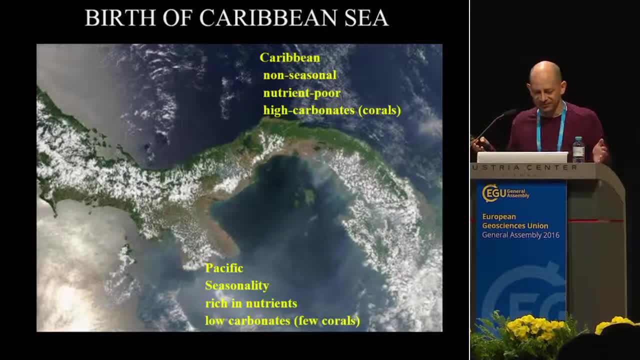 It has a season. the temperature changes throughout the year. it's changes throughout the year. it's changes throughout the year. it's very rich in nutrients and has very, very rich in nutrients, and has very, very rich in nutrients and has very few corals. 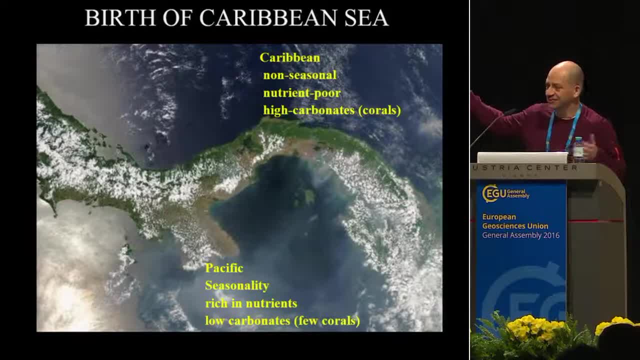 few corals, few corals. And the reason people have thought. And the reason people have thought, And the reason people have thought that the Caribbean is the way it, that the Caribbean is the way it, that the Caribbean is the way it is because, once the isthmus went, 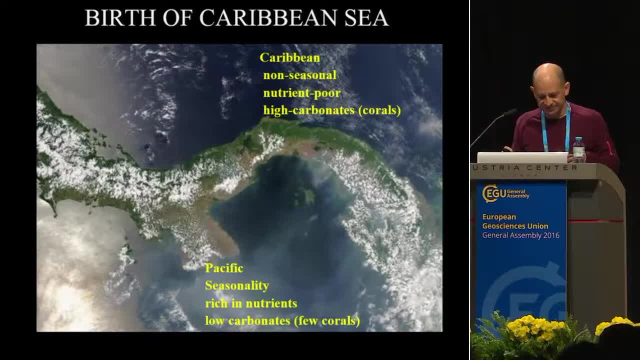 is because once the isthmus went, is because once the isthmus went up, it disconnected the Caribbean up, it disconnected the Caribbean up, it disconnected the Caribbean from the Pacific Ocean, from the Pacific Ocean, from the Pacific Ocean. And finally, the fourth thing, that 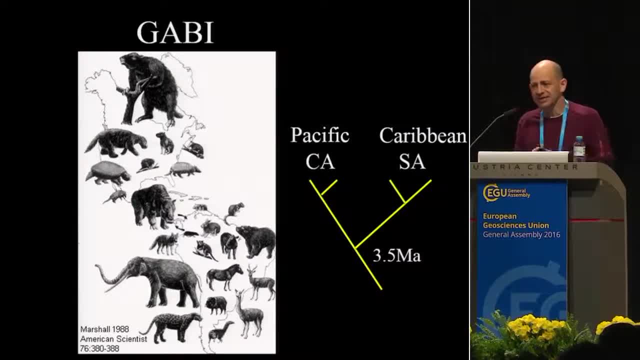 And finally, the fourth thing, that, And finally the fourth thing that has been linked to Panama, is what has been linked to Panama, is what has been linked to Panama, is what we call the Great American, we call the Great American, we call the Great American. Biotic Interchange, one of the 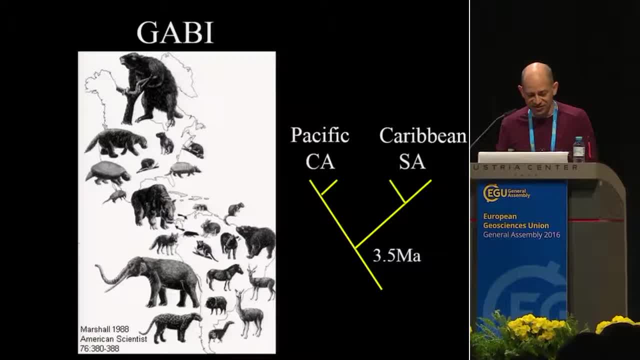 Biotic Interchange, one of the Biotic Interchange, one of the most amazing experiments, of most amazing experiments, of most amazing experiments of biological invasions. when these biological invasions, when these biological invasions, when these two continents that were, two continents that were. 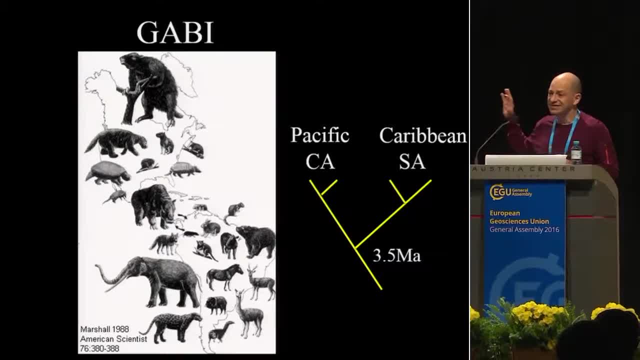 two continents that were separated got together. separated, got together, separated, got together. So, if you're a biologist, this is So. if you're a biologist, this is So. if you're a biologist, this is a fantastic experiment. a fantastic experiment. 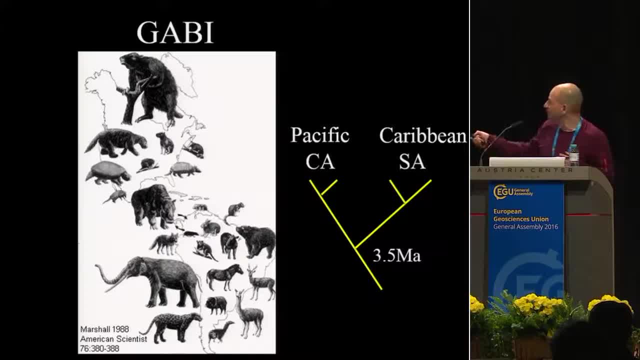 a fantastic experiment If you are a marine biologist, If you are a marine biologist, If you are a marine biologist, it's an experiment of what. it's an experiment of what. it's an experiment of what happened with two populations. happened with two populations. 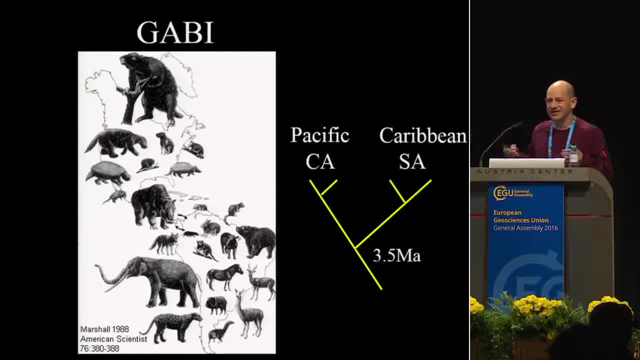 happened with two populations that were joined together in, that were joined together in, that were joined together in the Caribbean and the Pacific. the Caribbean and the Pacific. the Caribbean and the Pacific get split apart by the rise of get split apart by the rise of. 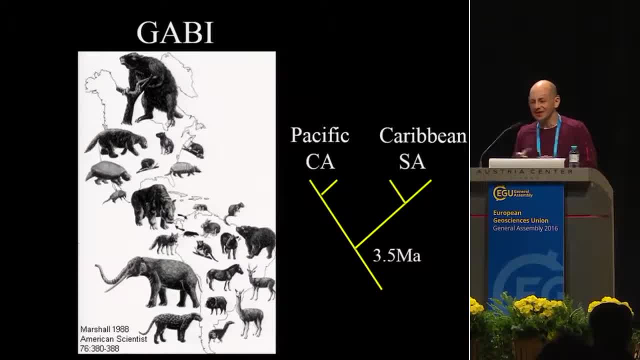 get split apart by the rise of the isthmus, the isthmus, the isthmus. And if you are in the continent, And if you are in the continent, And if you are in the continent, it's an experiment of what? 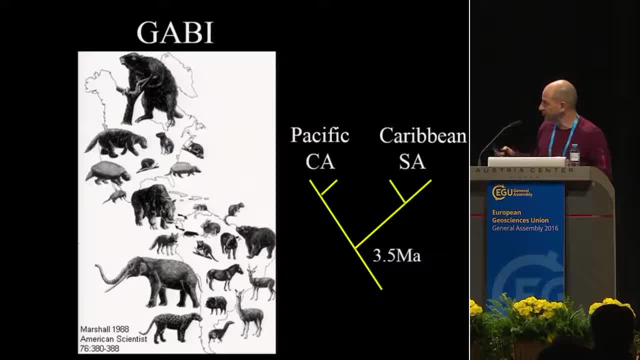 it's an experiment of what. it's an experiment of what happened with two things. that happened with two things. that happened with two things that were apart, are together, were apart, are together, were apart, are together. So you find migration of plants. So you find migration of plants. 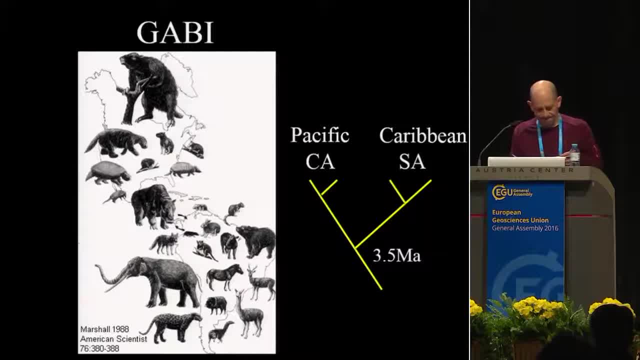 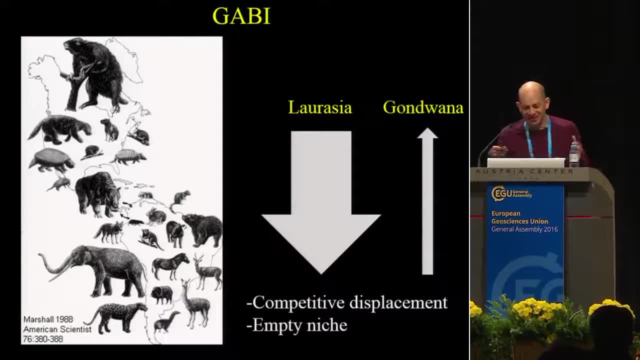 So you find migration of plants and animals going in both and animals going in both and animals going in both directions, And a common theme about this And a common theme about this And a common theme about this- Great American Biotic, Great American Biotic, Great American Biotic- Interchange is that it has been. 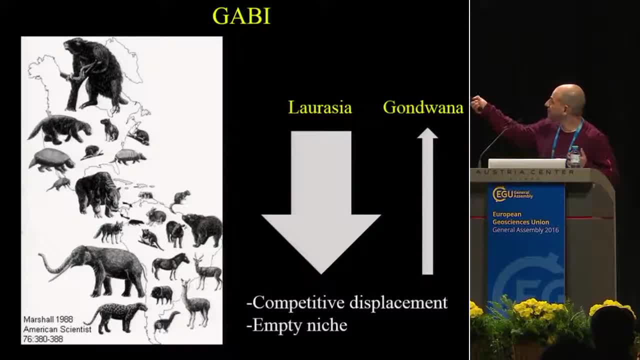 Interchange is that it has been. Interchange is that it has been asymmetrical, asymmetrical, asymmetrical. So, in general, most of the animals. So, in general, most of the animals, So, in general, most of the animals that we see here in South America. 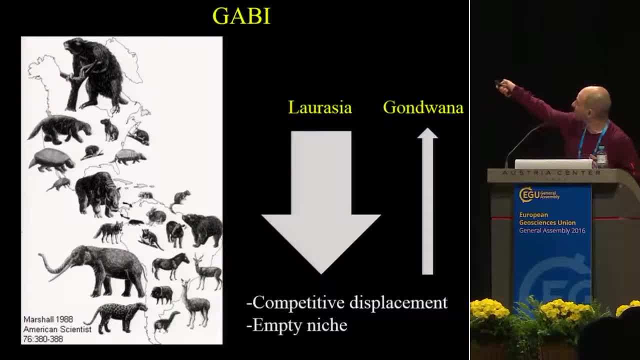 that we see here in South America, that we see here in South America, were derived from North America, were derived from North America, were derived from North America. So it's a big asymmetry. So it's a big asymmetry. So it's a big asymmetry. Most of the migration happened. 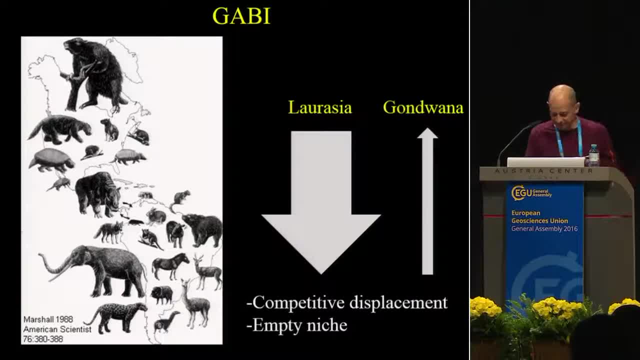 Most of the migration happened. Most of the migration happened from the north to the south, from the north to the south, from the north to the south, and then to the south to the north, and then to the south to the north, and then to the south to the north. About six years ago. 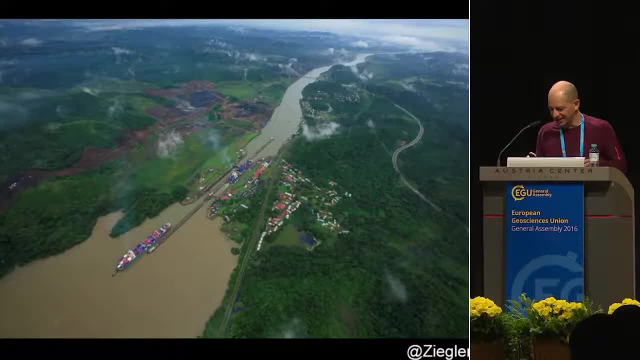 About six years ago, About six years ago, the country of Panama decided, the country of Panama decided, the country of Panama decided to expand the Panama Canal, to expand the Panama Canal, to expand the Panama Canal, And it was a major enterprise, And it was a major enterprise. 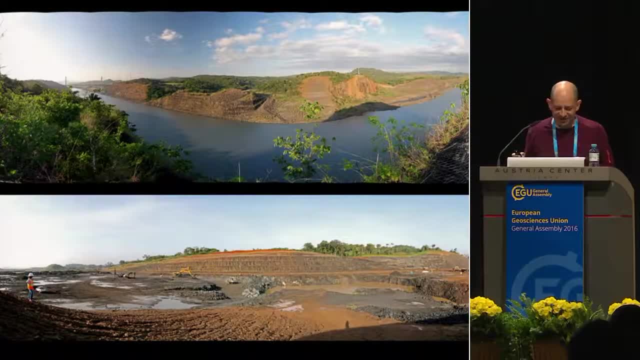 And it was a major enterprise for Panama, for Panama, for Panama. It's a small country, It's a small country. It's a small country, only 3.5 million people, only 3.5 million people, only 3.5 million people. And this was a big investment. 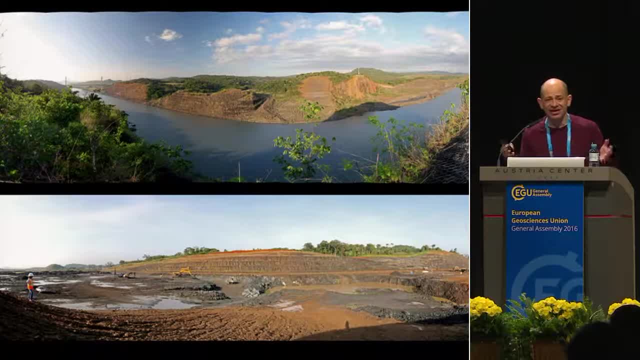 And this was a big investment, And this was a big investment about $5 billion, about $5 billion, about $5 billion. And you can tell how Panama And you can tell how Panama And you can tell how Panama really loves geology. 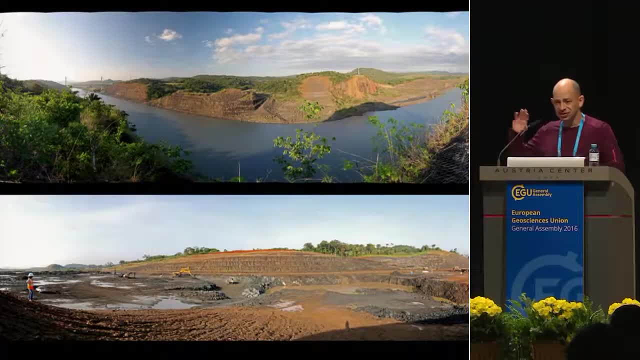 really loves geology, really loves geology because they decided to invest. because they decided to invest, because they decided to invest $5 billion in doing a geological $5 billion, in doing a geological $5 billion, in doing a geological cross-section from the Caribbean, cross-section from the Caribbean. 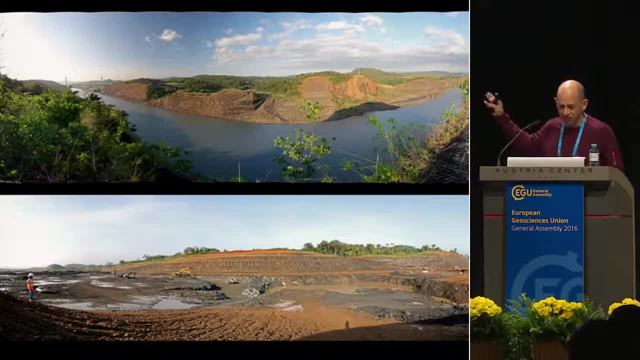 cross-section from the Caribbean to Panama to Panama, to Panama. So we put together a big team of So we put together a big team of So we put together a big team of geologists to go to the field, geologists to go to the field. 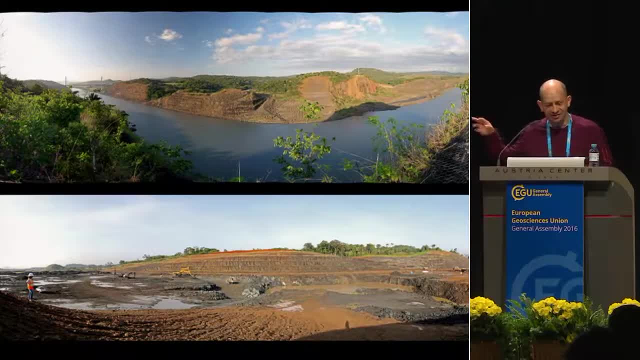 geologists to go to the field And most of these places that you And most of these places that you And most of these places that you see in the photo are gone- see in the photo- are gone- see in the photo- are gone either because the entire 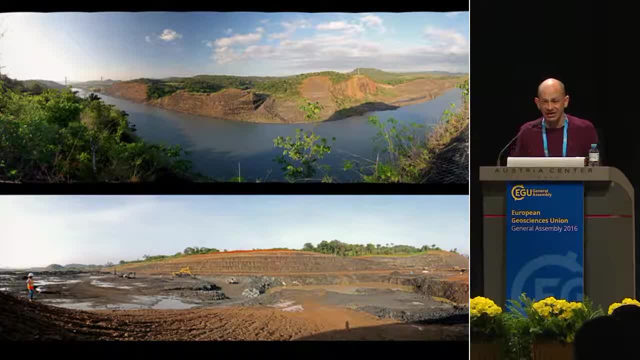 either because the entire, either because the entire mountains were taken away. mountains were taken away, mountains were taken away, and that's where the new locks and that's where the new locks and that's where the new locks of the canal are, or because 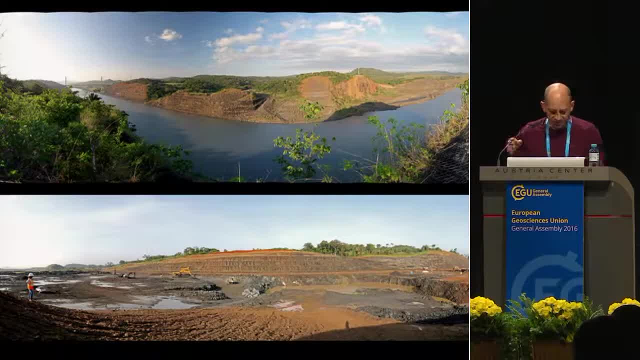 of the canal are, or because of the canal are, or because this is already covered with. this is already covered with, this is already covered with vegetation, vegetation, vegetation. So we have a small window to, So we have a small window to, So we have a small window to really use all this new. 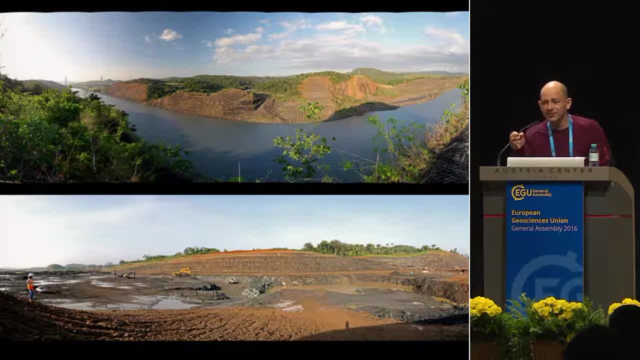 really use all this new. really use all this new information that was available, information that was available, information that was available to us, to us, to us, But of course, when we started, But of course, when we started, But of course, when we started this work five years ago, we 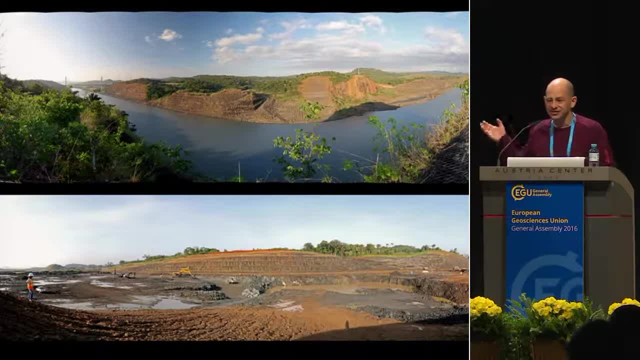 this work five years ago. we this work five years ago. we didn't want to focus on the rise, didn't want to focus on the rise, didn't want to focus on the rise of the Isthmus per se, because of the Isthmus per se, because. 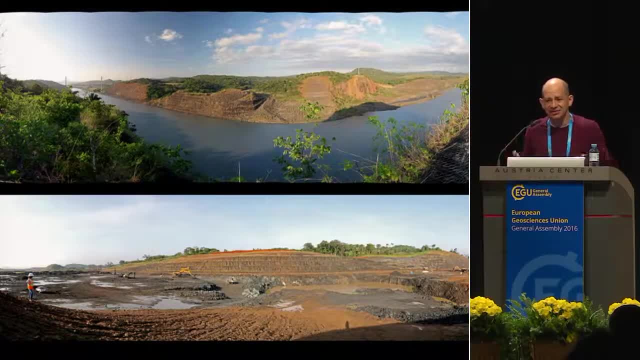 of the Isthmus per se, because when you have almost 2,000, when you have almost 2,000, when you have almost 2,000 papers citing that, the Isthmus papers citing that, the Isthmus papers citing that the Isthmus went up 3.5 million years ago. went up 3.5 million years ago. went up 3.5 million years ago. that's something that you don't. that's something that you don't. that's something that you don't want to do again. want to do again. 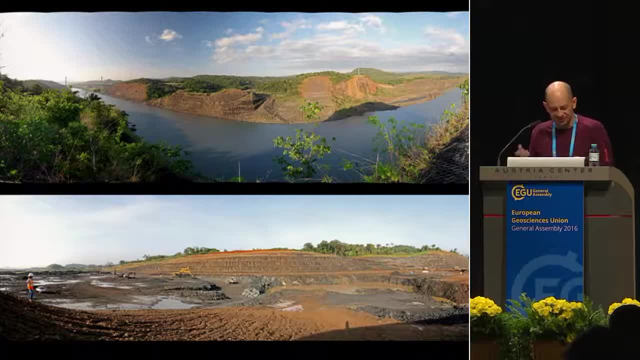 want to do again. So we decided to understand the. So we decided to understand the. So we decided to understand the early history of the Isthmus, early history of the Isthmus, early history of the Isthmus. rather than the actual final. rather than the actual final. 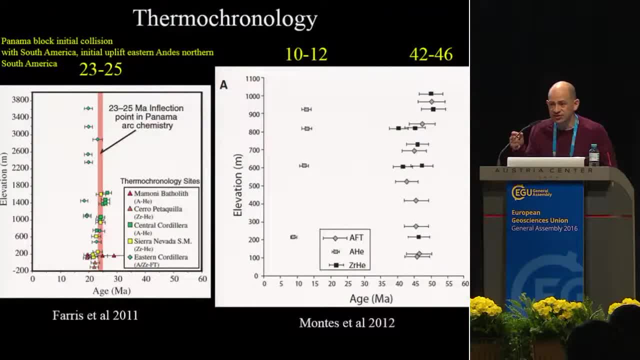 rather than the actual final uplift of the Isthmus, uplift of the Isthmus, uplift of the Isthmus. And we started to use a number. And we started to use a number, And we started to use a number of tools that geologists didn't. 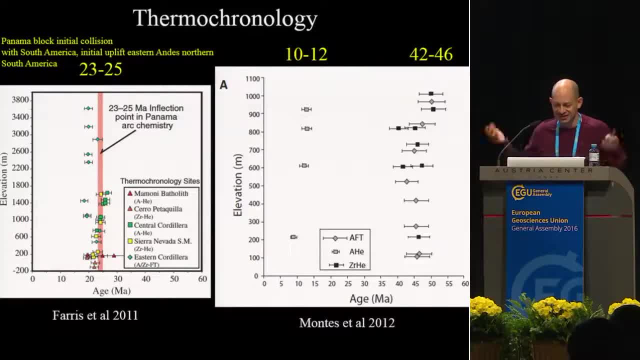 of tools that geologists didn't, of tools that geologists didn't have 20 years ago, when this idea have 20 years ago, when this idea have 20 years ago when this idea of the Isthmus was developed, of the Isthmus was developed. 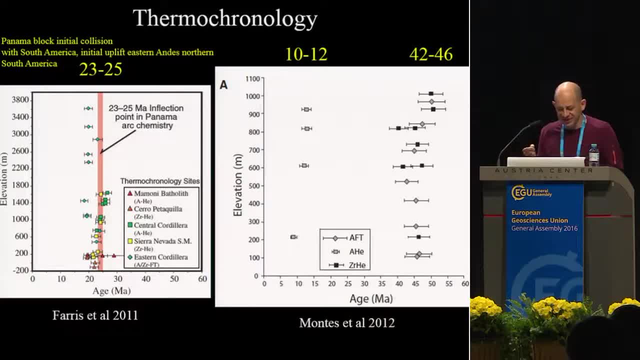 of the Isthmus was developed also by the Smithsonian in Panama, also by the Smithsonian in Panama, also by the Smithsonian in Panama, And one of the first techniques And one of the first techniques And one of the first techniques we used was thermochronology. 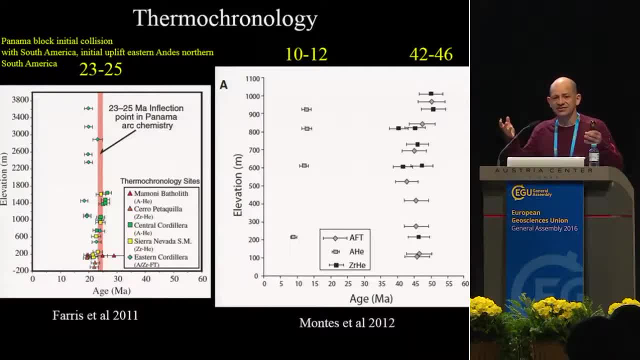 we used was thermochronology. we used was thermochronology, and this is using, and this is using, and this is using: circum-crystal today, circum-crystal today, circum-crystal today: the exhumation of the rock. 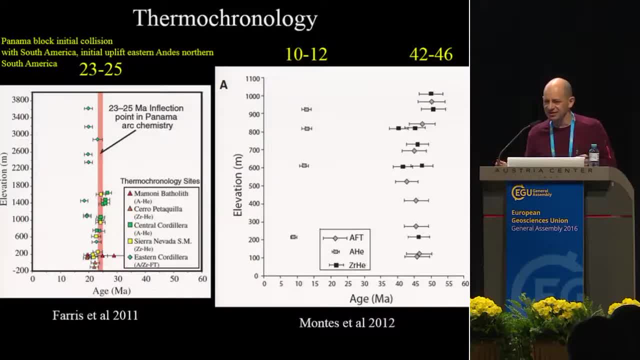 the exhumation of the rock. the exhumation of the rock when the particular block of rock, when the particular block of rock, when the particular block of rock goes up to the surface, goes up to the surface, goes up to the surface, And we did that all over Panama. 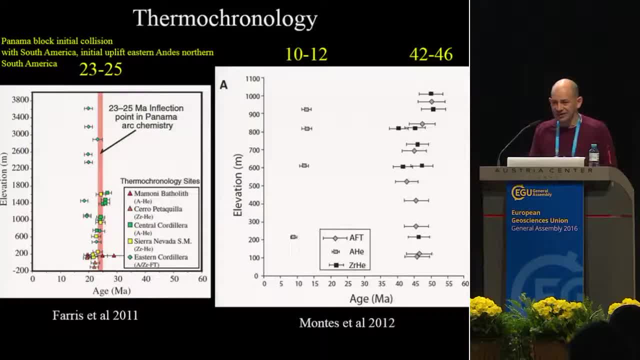 And we did that all over Panama, And we did that all over Panama, especially in the canal, especially in the canal, especially in the canal. And the first thing that we found, And the first thing that we found, And the first thing that we found that you can see here, is that 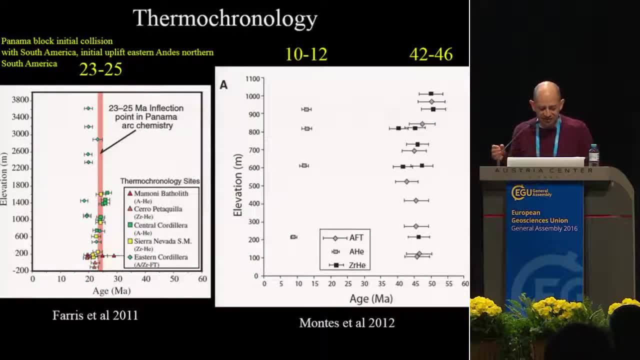 that you can see here is that that you can see here is that we didn't see a strong signal. we didn't see a strong signal. we didn't see a strong signal 3.5 million years ago. 3.5 million years ago. 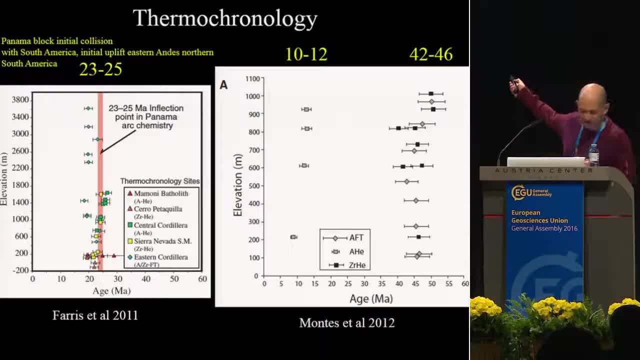 3.5 million years ago. So we saw a big exhumation event. So we saw a big exhumation event. So we saw a big exhumation event at 42 million years. at 42 million years. at 42 million years, 23 million years. 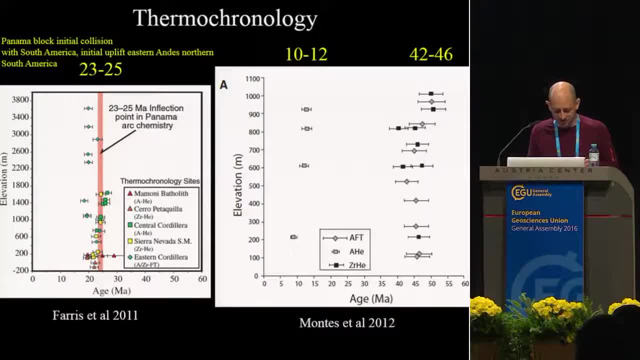 23 million years, 23 million years and 10 million years, and 10 million years and 10 million years, But we didn't see anything, But we didn't see anything, But we didn't see anything at 3.5 million years. 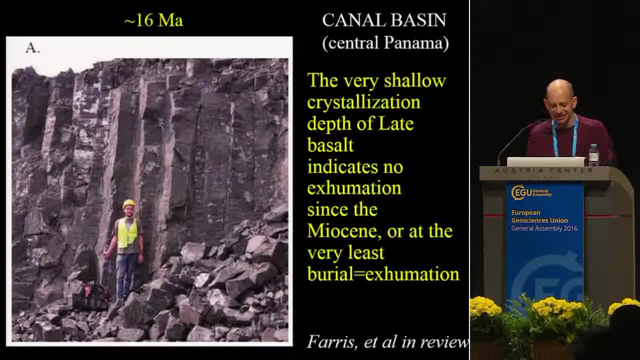 at 3.5 million years. at 3.5 million years, We also analyzed the geology. We also analyzed the geology. We also analyzed the geology of the volcanoes we see of the volcanoes we see of the volcanoes we see in central Panama. 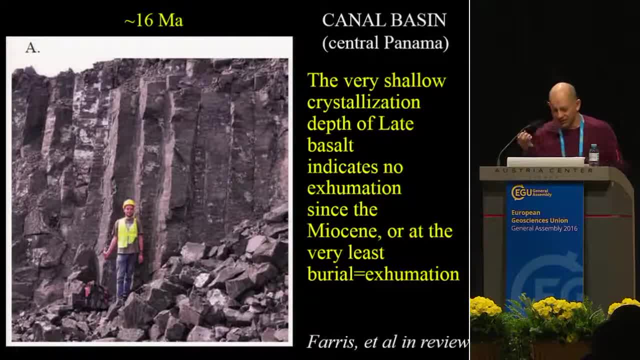 in central Panama. in central Panama, like the one you see in the photo, like the one you see in the photo, like the one you see in the photo. And the geology, the chemistry, And the geology, the chemistry. 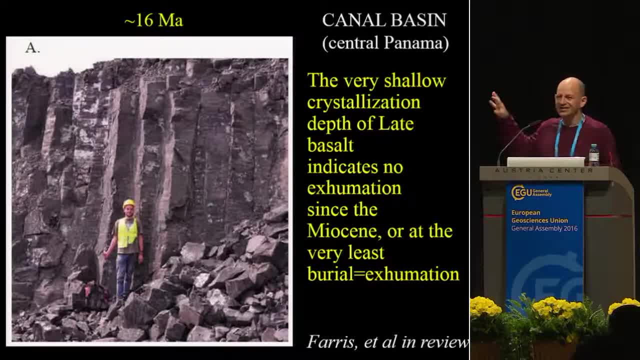 And the geology, the chemistry and the petrography of the rocks and the petrography of the rocks and the petrography of the rocks themselves show that these themselves show that these themselves show that these deposits, these volcanoes that were, 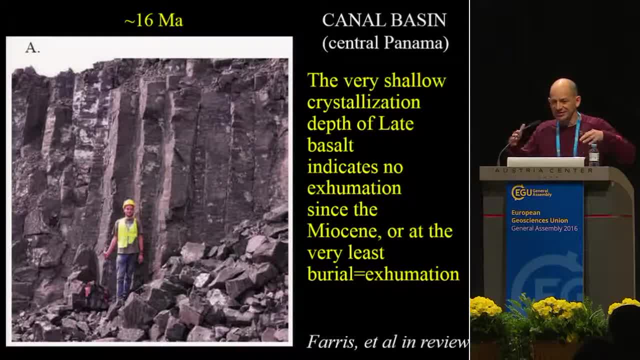 deposits, these volcanoes that were deposits, these volcanoes that were 16 million years old, were 16 million years old, were 16 million years old, were subaerial, subaerial, subaerial, So they were not in a submarine. 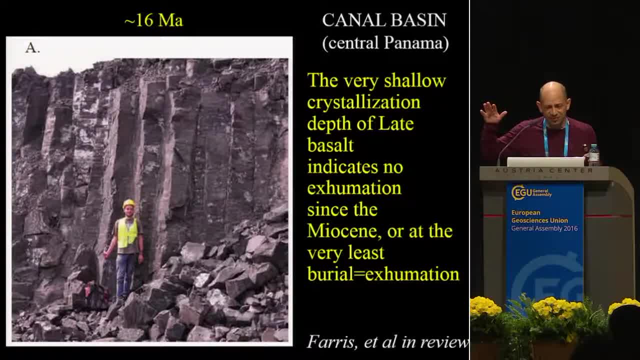 So they were not in a submarine, So they were not in a submarine. volcano that then went up, volcano that then went up, volcano that then went up. but it was a volcano that probably. but it was a volcano that probably, but it was a volcano that probably was very similar outside the 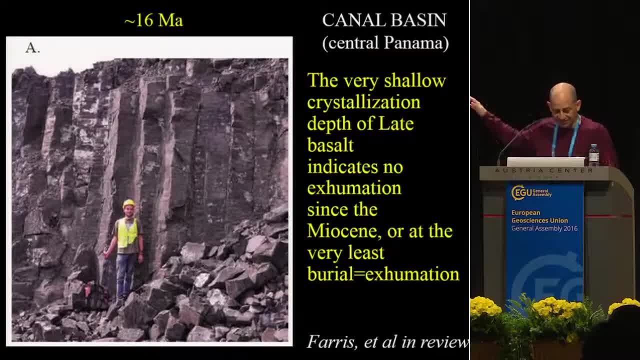 was very similar outside. the was very similar outside the landscape as we see today, landscape as we see today, landscape as we see today- And this is already in the early, And this is already in the early, And this is already in the early 16 million years ago. 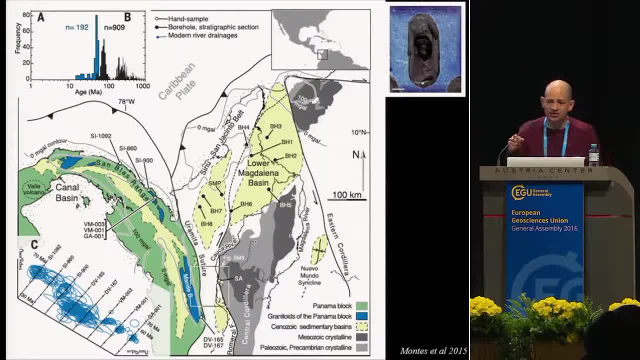 16 million years ago, 16 million years ago. Now we use a technique called Now we use a technique called Now, we use a technique called provenance analysis, provenance analysis, provenance analysis. So you take also a circon crystal, So you take also a circon crystal. 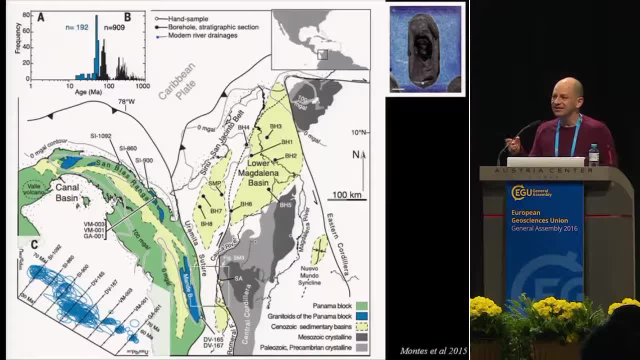 So you take also a circon crystal from a sedimentary rock and by from a sedimentary rock and by from a sedimentary rock and by dating the crystal you can tell dating the crystal. you can tell dating the crystal, you can tell where this circon was derived. 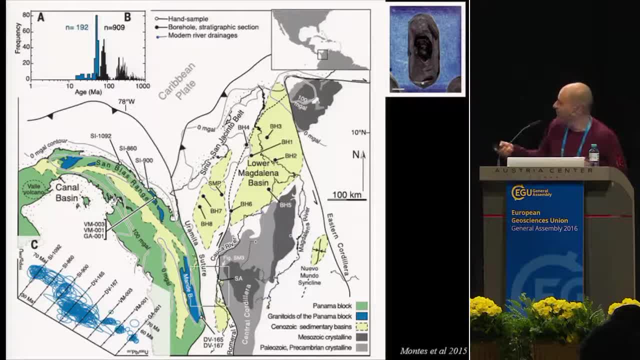 where this circon was derived, where this circon was derived from, and we went to different from, and we went to different from and we went to different places in Colombia and Panama: places in Colombia and Panama, places in Colombia and Panama. And this line that you can see. 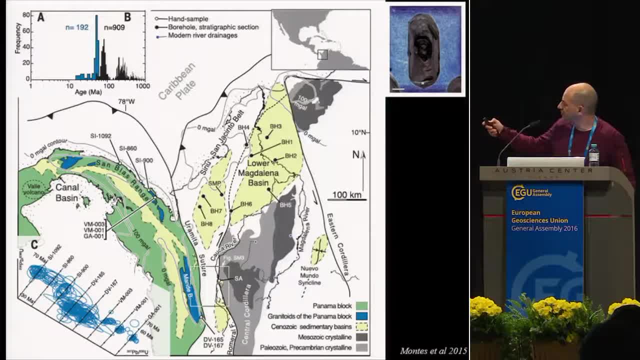 And this line that you can see, And this line that you can see, here is the actual tectonic, here is the actual tectonic, here is the actual tectonic boundary between the Caribbean boundary, between the Caribbean boundary, between the Caribbean plate and Panama and the South. 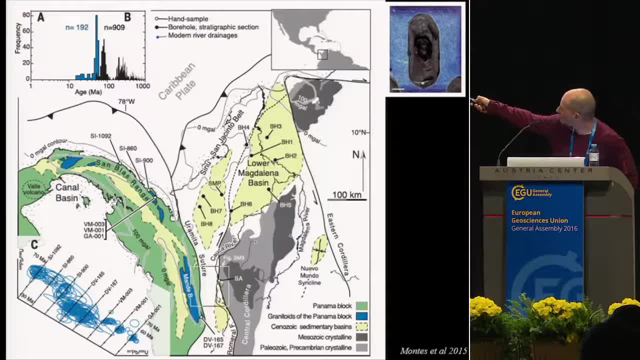 plate and Panama and the South plate and Panama and the South American plate, American plate, American plate. So the actual collision of Panama, So the actual collision of Panama, So the actual collision of Panama with Colombia is within Colombia, with Colombia is within Colombia. 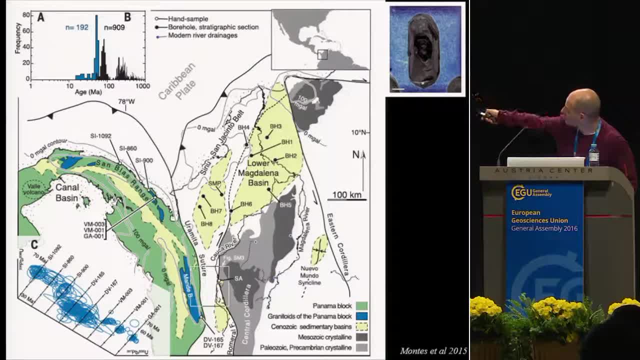 with Colombia is within Colombia. So we went to places here and also, So we went to places here and also, So we went to places here and also places here, and we used this places here and we used this places here and we used this provenance analysis. 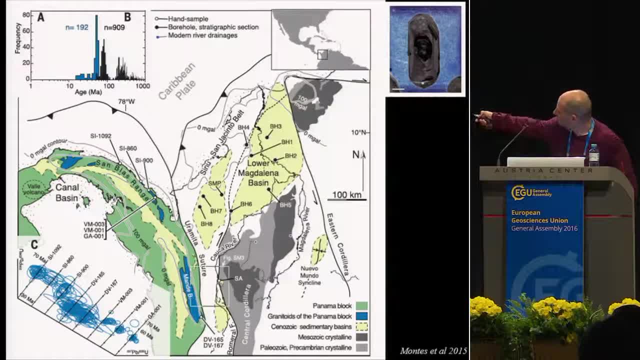 provenance analysis. provenance analysis: What we found is that we found here What we found is that we found here. What we found is that we found here fluvial rocks on the Colombian fluvial rocks on the Colombian fluvial rocks on the Colombian side that had circons, that only 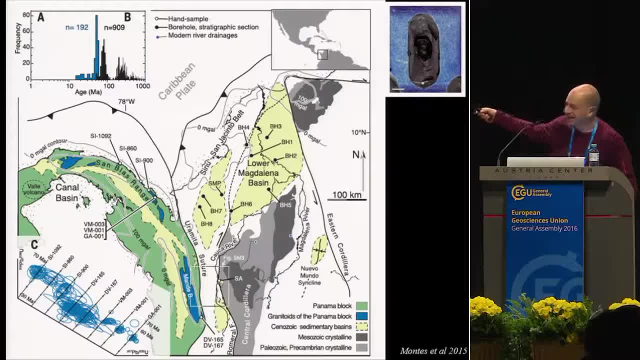 side that had circons, that only side that had circons, that only could come from the Panamanian, could come from the Panamanian, could come from the Panamanian Volcanica, Volcanica, Volcanica, And when we date these sedimentary, 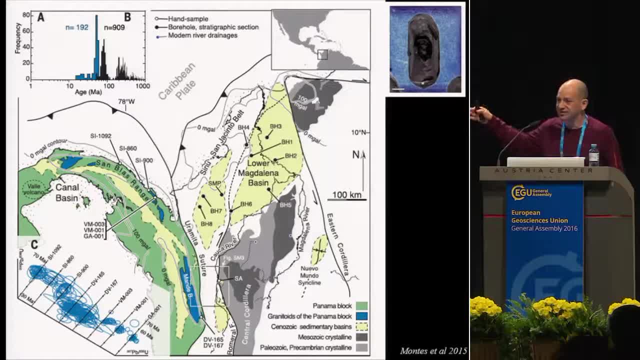 And when we date these sedimentary And when we date these sedimentary rocks, we realized that there were rocks. we realized that there were rocks, we realized that there were middle miocene about 12 to 13. middle miocene about 12 to 13. 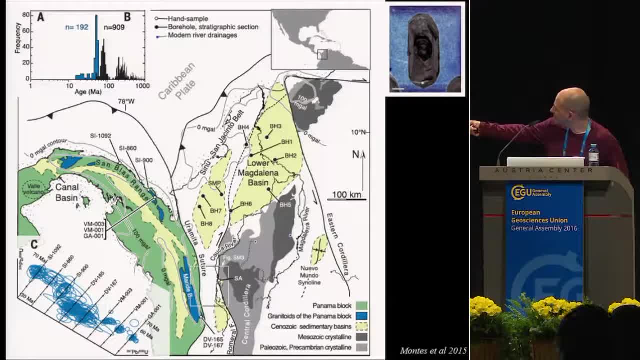 middle miocene, about 12 to 13 million years old. showing that million years old. showing that million years old. showing that by that time this collision had, by that time this collision had, by that time this collision had already happened and there were. 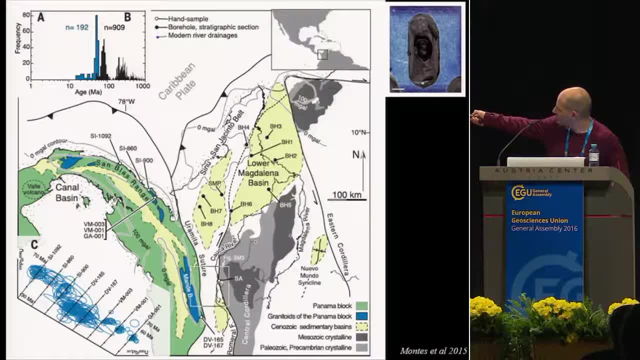 already happened and there were already happened and there were sediments that were coming from, sediments that were coming from, sediments that were coming from Panama into the South American Panama, into the South American Panama, into the South American plate plate plate And this boundary, that was the 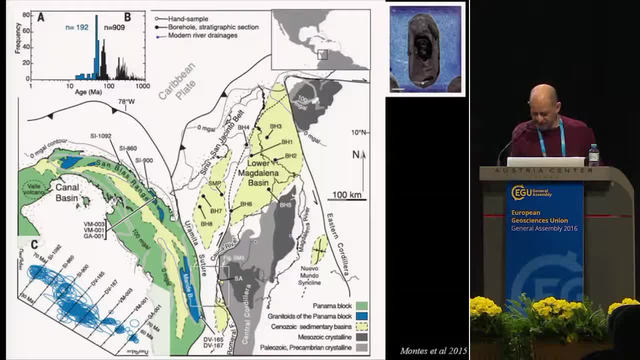 And this boundary, that was the, And this boundary, that was the ocean that was connecting the ocean, that was connecting the ocean, that was connecting the Caribbean with the Pacific, was Caribbean with the Pacific, was Caribbean with the Pacific, was already closed, already closed, already closed. So we think this is how Panama and 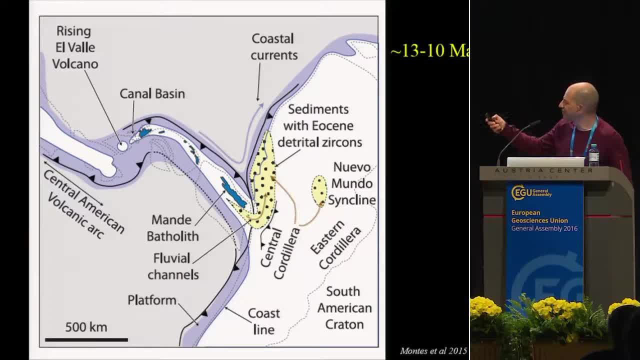 So we think this is how Panama, and So we think this is how Panama and the connection will look about. the connection will look about the connection will look about between 13 and 10 million years, between 13 and 10 million years, between 13 and 10 million years ago. 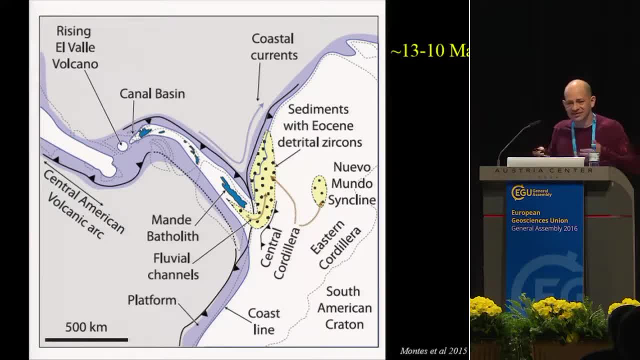 ago ago. So this Central American seaway, the. So this Central American seaway, the. So this Central American seaway, the deep seaway along the tectonic deep seaway, along the tectonic deep seaway along the tectonic boundary between South America. 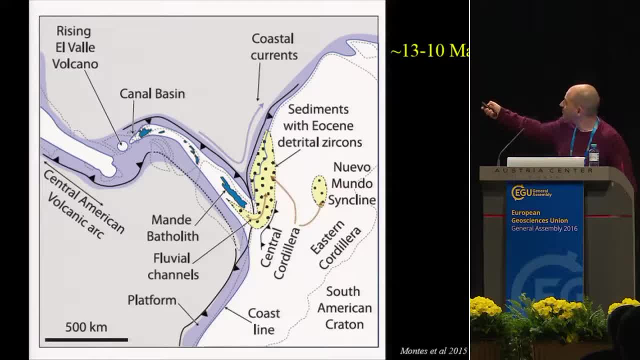 boundary between South America, boundary between South America and the Caribbean, was already and the Caribbean was already and the Caribbean was already closed by 10 million years, closed by 10 million years, closed by 10 million years, And you only have shallow water And you only have shallow water. 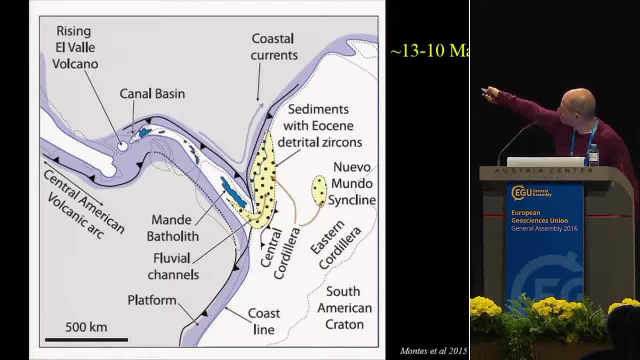 And you only have shallow water, connections in some other places, connections in some other places, connections in some other places, but this deep ocean was gone by. but this deep ocean was gone by. but this deep ocean was gone by 10 million years, 10 million years. 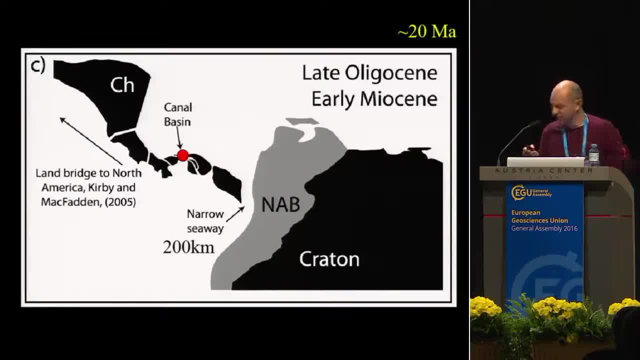 10 million years. Now I'm going to show you what the Now I'm going to show you what the Now I'm going to show you what the fossil record, the actual fossil fossil record, the actual fossil fossil record, the actual fossil record of Panama tell us about. record of Panama. tell us about record of Panama. tell us about the rise of the isthmus. the rise of the isthmus, the rise of the isthmus. So all the fossils I'm going to show. So all the fossils I'm going to show. 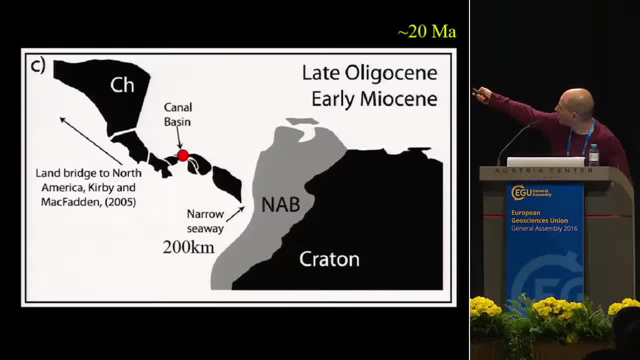 So all the fossils I'm going to show you in the next slides, come here, you in the next slides. come here, you in the next slides. come here from the canal base, from the canal base, from the canal base And, as you can see here, this is part. 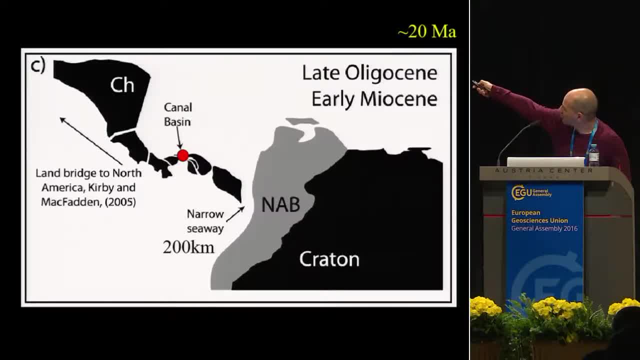 And, as you can see here, this is part, And, as you can see here, this is part of the scent of the Caribbean plate, of the scent of the Caribbean plate, of the scent of the Caribbean plate, and it will be part of pretty and it will be part of pretty. 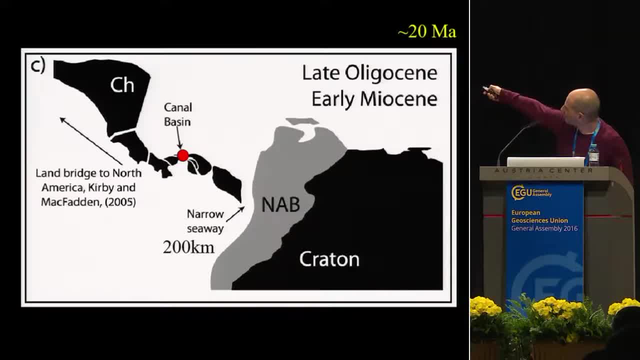 and it will be part of pretty North America, North America, North America. So this is the Panamanian seaway. So this is the Panamanian seaway. So this is the Panamanian seaway, the deep ocean and this is South. 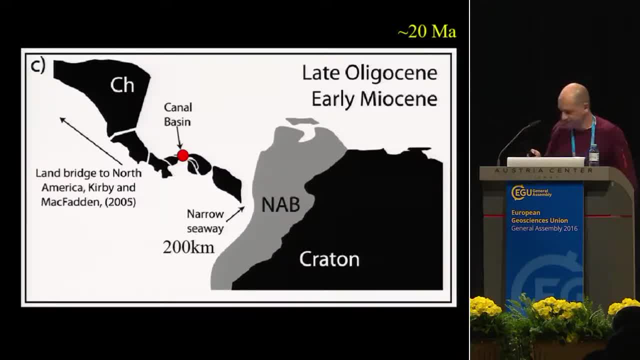 the deep ocean, and this is South the deep ocean, and this is South America, America, America, And so we'll be looking here about, And so we'll be looking here about, And so we'll be looking here about 20 million years ago. 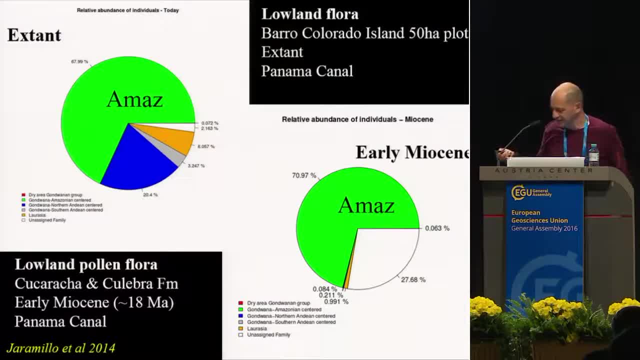 20 million years ago. 20 million years ago Now, when we look at the plants, Now when we look at the plants, Now when we look at the plants that we find in the Miocene of that, we find in the Miocene of that, we find in the Miocene of Panama, and compared to the plants, 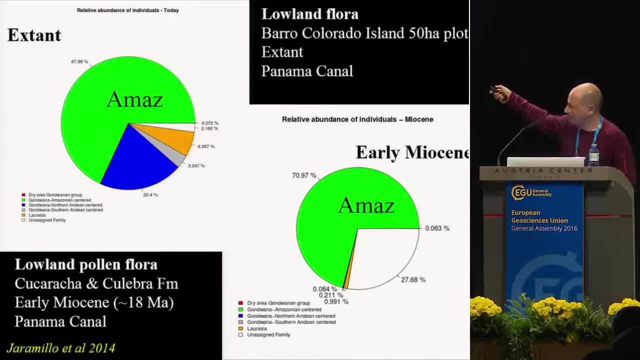 Panama and compared to the plants Panama, and compared to the plants that we find today also in Panama, that we find today also in Panama, that we find today also in Panama, and this is by looking at the and this is by looking at the. 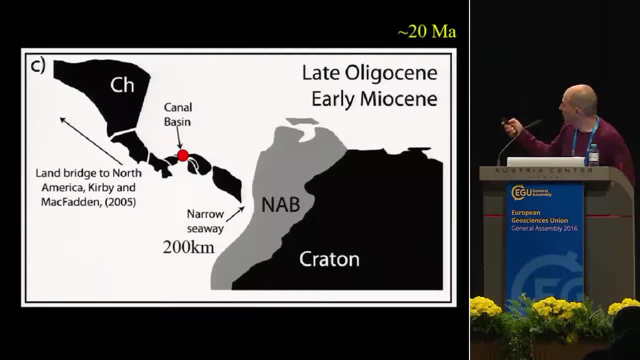 and this is by looking at the pollen record. we see that even pollen record, we see that even pollen record, we see that, even though there were a deep ocean, though there were a deep ocean, though there were a deep ocean disconnecting these two areas, 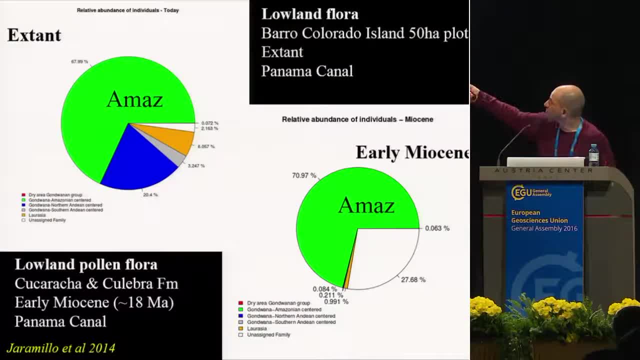 disconnecting these two areas. disconnecting these two areas, the plants had already been able. the plants had already been able, the plants had already been able to cross to Panama, to cross to Panama, to cross to Panama. So most of the plants in the 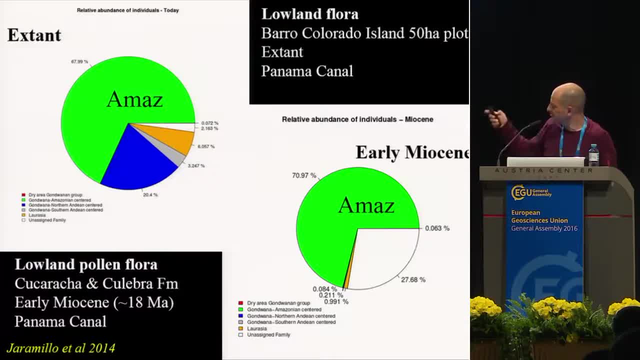 So most of the plants in the, So most of the plants in the Miocene of Panama already came Miocene of Panama, already came Miocene of Panama, already came from Amazonia, as you can see from Amazonia, as you can see from Amazonia, as you can see here. 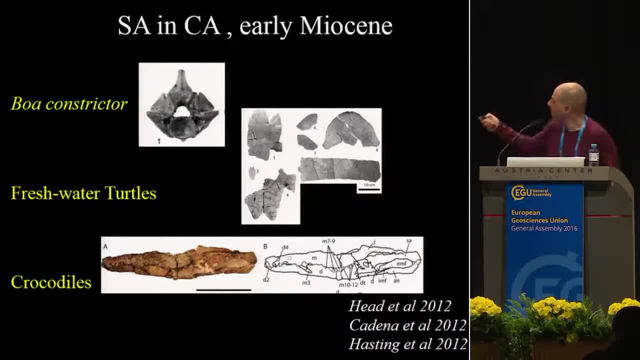 here, here, When we look at the vertebrates, When we look at the vertebrates, When we look at the vertebrates, like boas, freshwater turtles, like boas, freshwater turtles, like boas, freshwater turtles. and crocodiles, many of those. 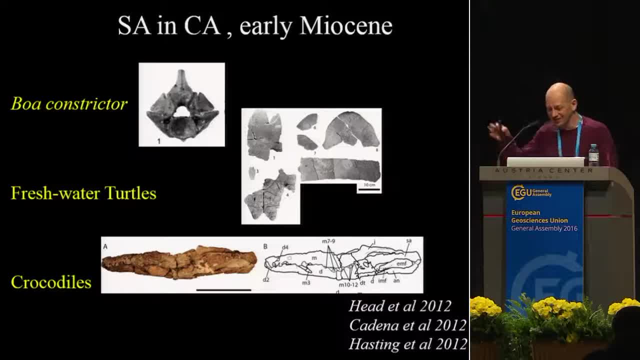 and crocodiles, many of those and crocodiles, many of those suggested that they came from, suggested that they came from, suggested that they came from South America, South America, South America. So they were already able to cross, So they were already able to cross. 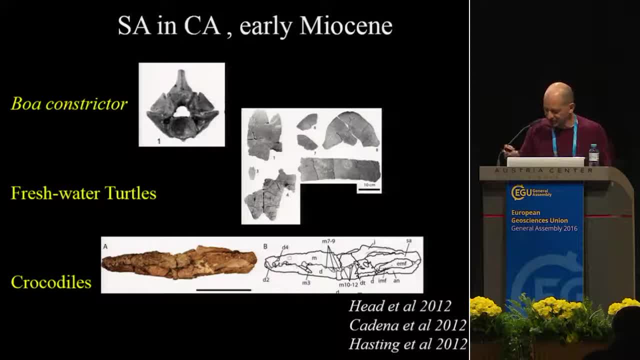 So they were already able to cross this Central American seaway, this Central American seaway, this Central American seaway in the early Miocene, in the early Miocene, in the early Miocene. Now, the only group that really, Now the only group that really. 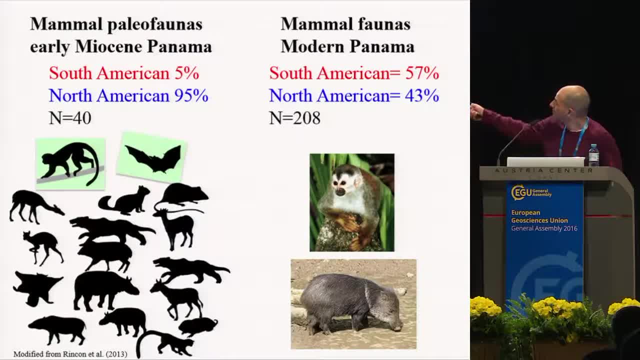 Now the only group that really doesn't show that are the, doesn't show that are the, doesn't show that are the mammals, mammals, mammals. So when we compare the mammals of, So, when we compare the mammals of, So, when we compare the mammals of the Miocene of Panama, as we can, 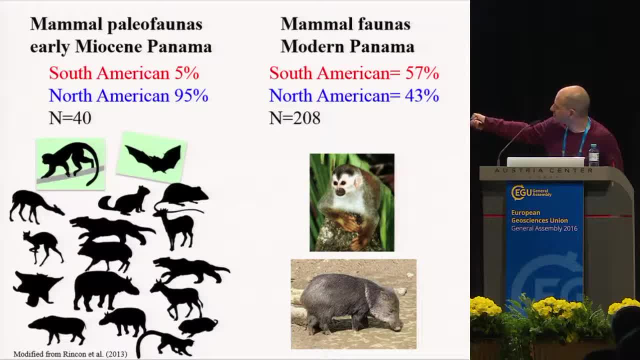 the Miocene of Panama, as we can, the Miocene of Panama as we can see here. so we have found, see here, so we have found, see here, so we have found rhinoceros horses, camels. rhinoceros horses, camels. 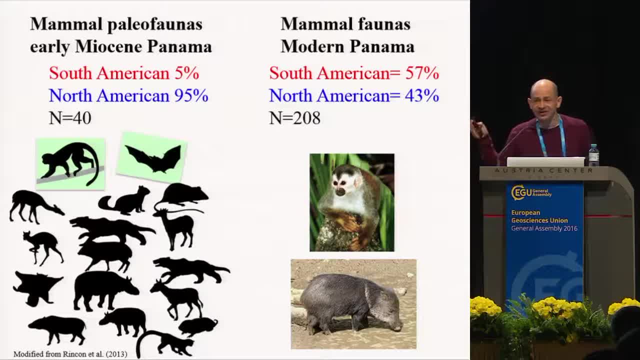 rhinoceros, horses, camels. everything that you see here come. everything that you see here come. everything that you see here come from North America in the Miocene, from North America in the Miocene, from North America in the Miocene of Panama. 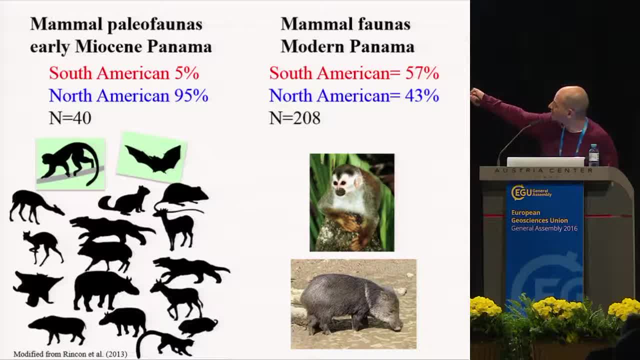 of Panama, of Panama. The only two things that are from, The only two things that are from, The only two things that are from South America are a bat and a South America are a bat and a South America are a bat and a monkey monkey. 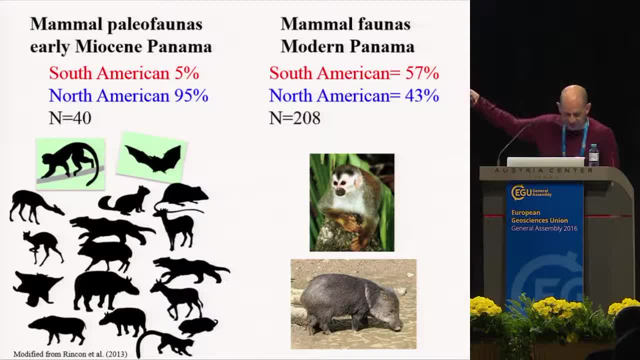 monkey, And this monkey is being published, And this monkey is being published, And this monkey is being published this Friday, this Friday, this Friday, And this monkey came from South And this monkey came from South And this monkey came from South America to Colombia. 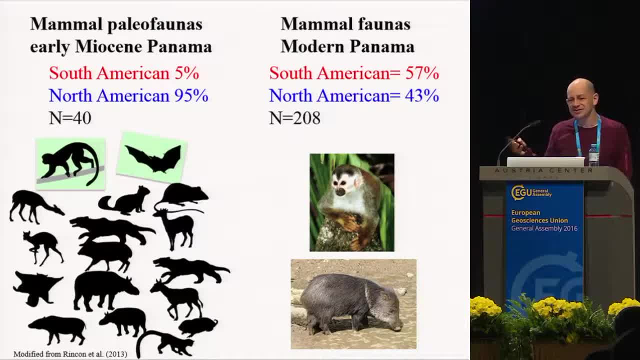 America to Colombia, America to Colombia. So in proportion, only 5% of the So in proportion, only 5% of the So in proportion, only 5% of the mammals from South America were mammals from South America were mammals from South America were here in the early Miocene of. 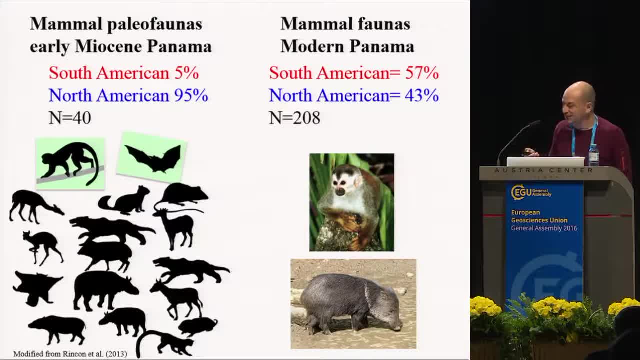 here in the early Miocene of, here in the early Miocene of Panama, Panama, Panama. If you compare it with the, If you compare it with the, If you compare it with the faunas of today, the mammals. faunas of today, the mammals. 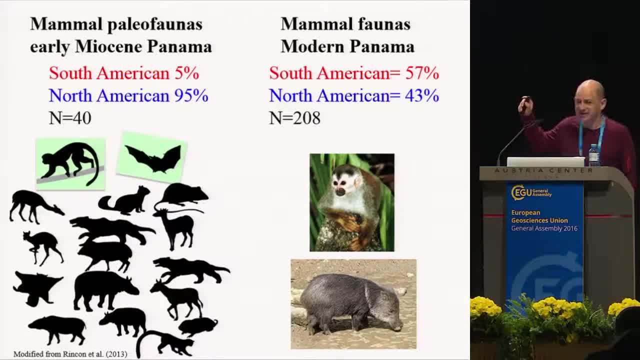 faunas of today, the mammals. faunas of modern Panama. the faunas of modern Panama, the faunas of modern Panama, the South American represent almost South American, represent almost South American, represent almost 60% of the fauna, 60% of the fauna. 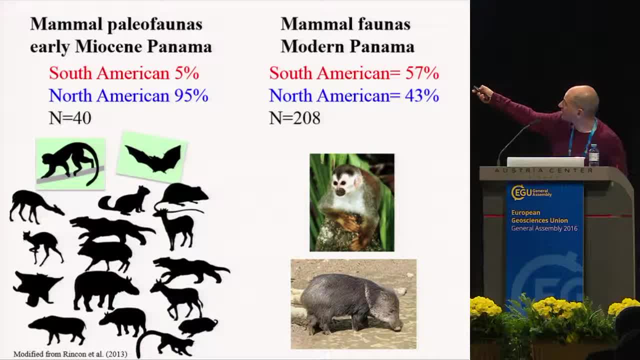 60% of the fauna. So you already see a big. So you already see a big. So you already see a big asymmetry of what happened in, asymmetry of what happened in, asymmetry of what happened in the early Miocene compared to the early Miocene compared to. 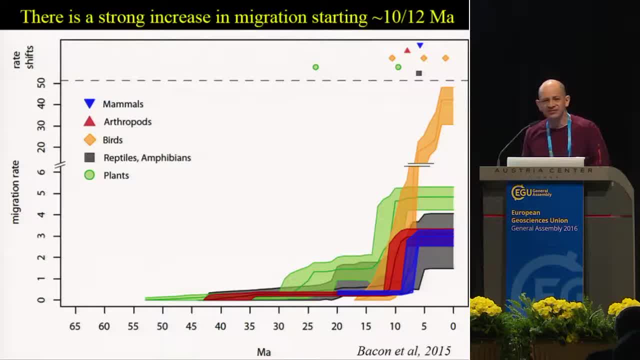 the early Miocene, compared to today, today, today, Now, there are many things that Now there are many things that Now there are many things that don't fossilize like frogs and don't fossilize like frogs and don't fossilize like frogs and lizards. 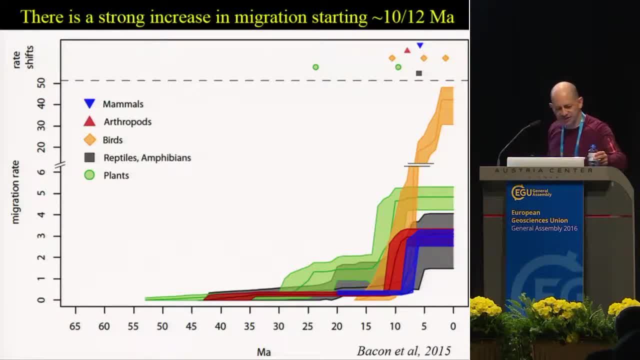 lizards, lizards. So we decide to use the genetic, So we decide to use the genetic, So we decide to use the genetic record and we did a meta-analysis record, and we did a meta-analysis record and we did a meta-analysis of almost 400 phylogenetic. 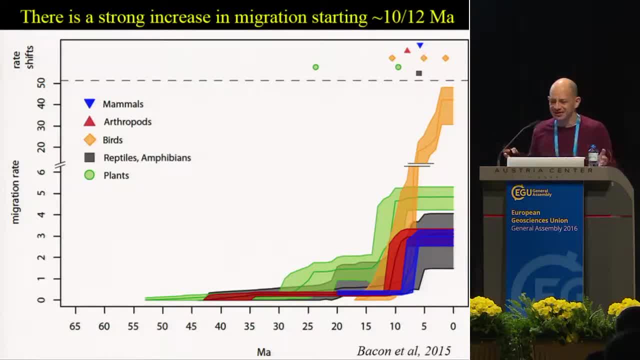 of almost 400 phylogenetic of almost 400 phylogenetic sequences of plants and animals. sequences of plants and animals. sequences of plants and animals, both in the oceans and in the, both in the oceans and in the, both in the oceans and in the land, to see when we will see an. 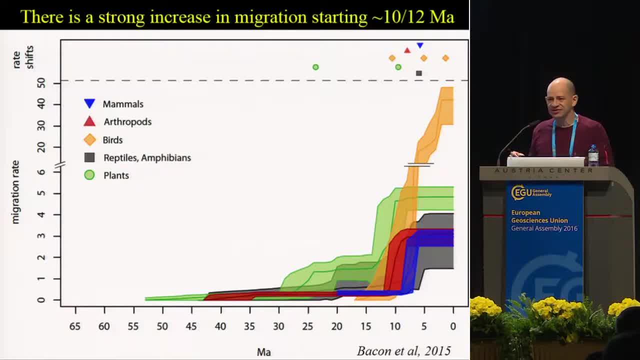 land, to see when we will see an land, to see when we will see an increase in the migration rate, increase in the migration rate, increase in the migration rate if you are in terrestrial, if you are in terrestrial, if you are in terrestrial continents or you see a. 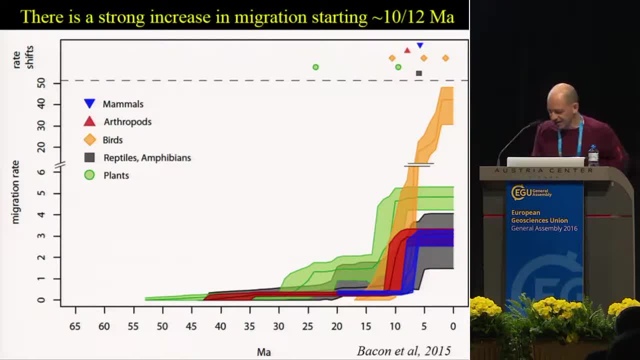 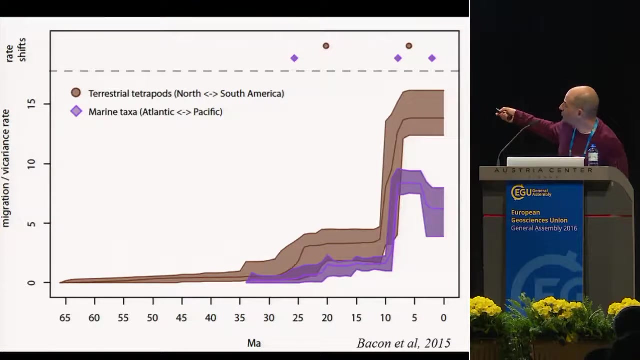 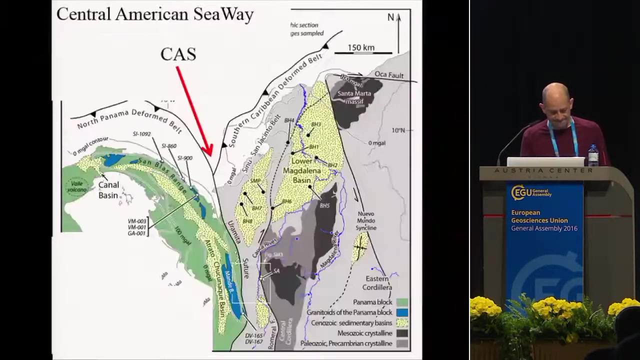 continents- or you see a continents or you see a of vicarious about 10 million years ago as you, as similar as to the terrestrial taxa. now, once again, just want to remind you that the Central American seaway, so this deep ocean that connected with the Caribbean, with the Pacific, is along. 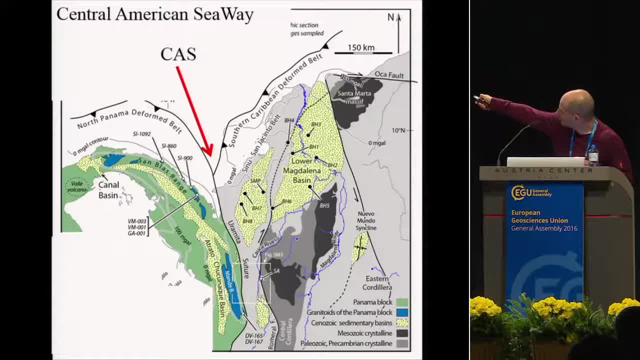 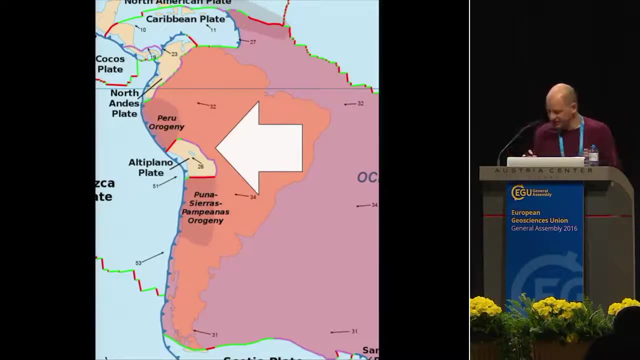 this line that you can see here between the green and the gray. so that's the actual tectonic boundary between South America and the Caribbean plate and Panama, and the history of this collision is really linked to the entire history of South America, how South America has been moving toward the West and is 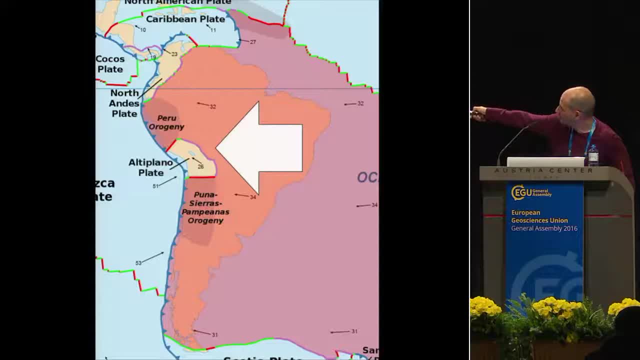 colliding with the plates that you see, you, you see here in the Pacific, the only difference that, because Panama is, is there in the transition between the Pacific and the South America and the Caribbean, and the alienation of the Caribbean plate, and the Caribbean plate is so thick all the. 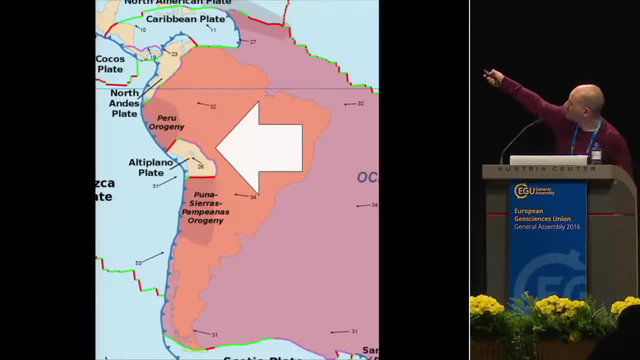 collisions that happen here along this boundary are registered in the rock themselves. well, if you go down here in the past, in all the plates that are here- because all those specific place goals underneath South America- the evidence of the collisions are gone. so everything, all the events that you see here are 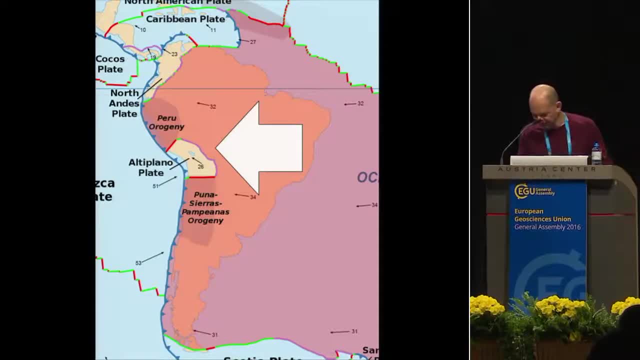 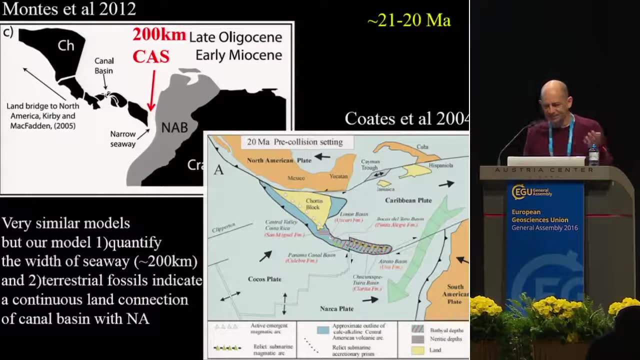 also seen in the entire South America at the same time. so in general, I can summarize the geological history of the 시�nus by three major event. one that happened 46 million years ago, but this one, 21, is when really you start to develop the landscape of Central America. so this 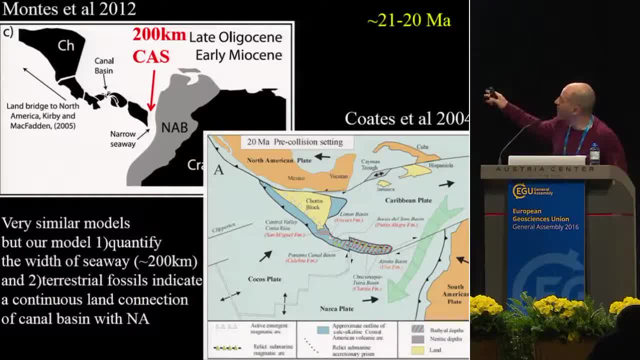 would be the biodeưởngographic situation of the Commission twenty million years ago. when we see extensive land being produced in Central America, so extensive that all the mammals we have here are yo Bereicer Terrae, what we see is Coxschilsalem. 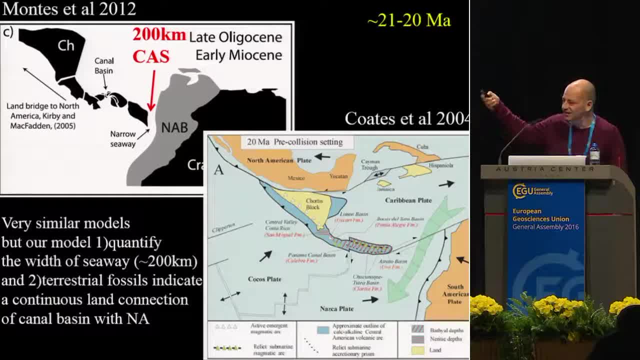 are sometimes the same species that you find in central in Montana, Florida, Texas. So by 20 million years ago you could walk from here to Texas and Florida. The Central American seaway was about 200 kilometers wide And as you compare it with the modeling that had done before, 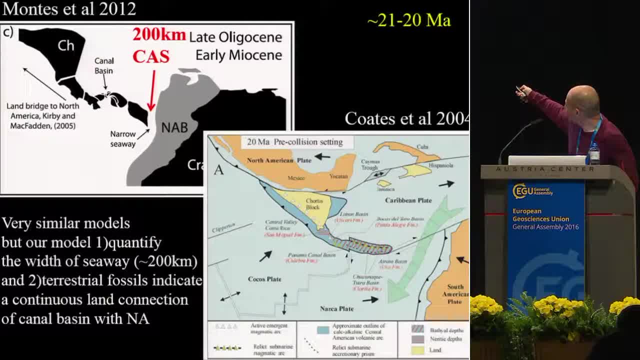 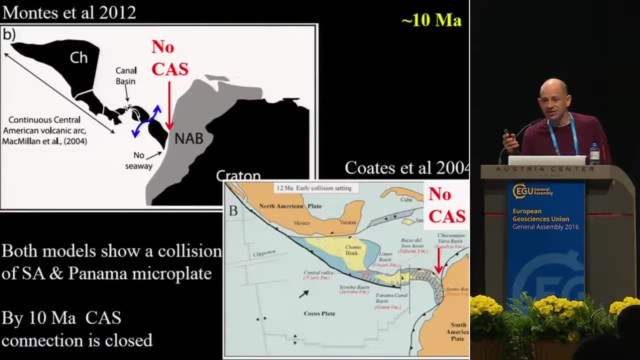 you could see that it was very similar, Basically the same situation, only that we put a really distance along the Central American seaway, Only 200 kilometers separated those 20 million years ago. Now, 10 million years ago, the second major event. 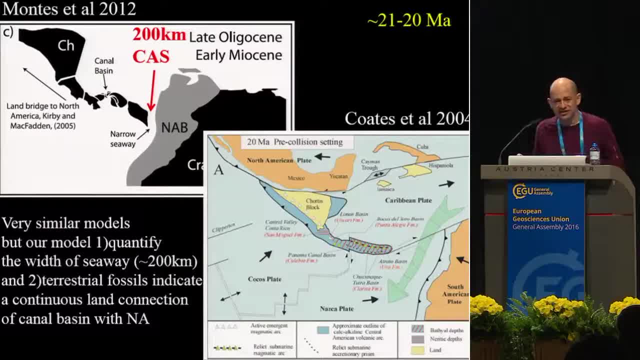 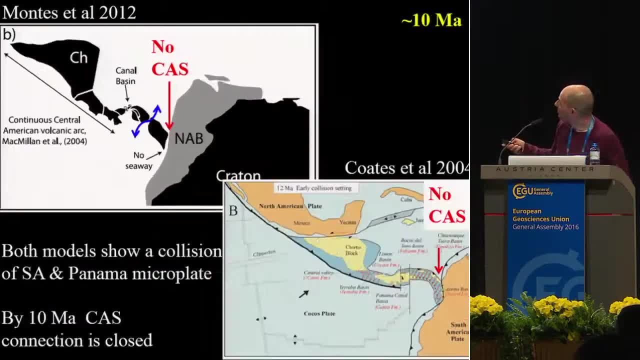 and something I forgot to tell you- that 20 million years ago, when you see the first major uplift of the Andes from Colombia down to Patagonia, The second major event happened 10 million years ago And once again you see the same thing all along the Andes. 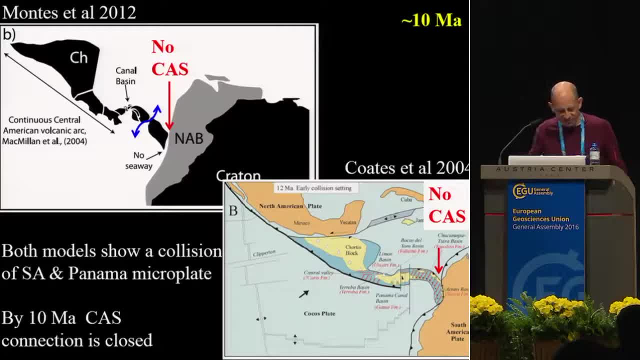 A major uplift of the Andes all across South America, And by 10 million years ago we think that the Central American seaway had already gone. So this collision happened about that time And you only have circulation of shallow water between both the oceans since then. 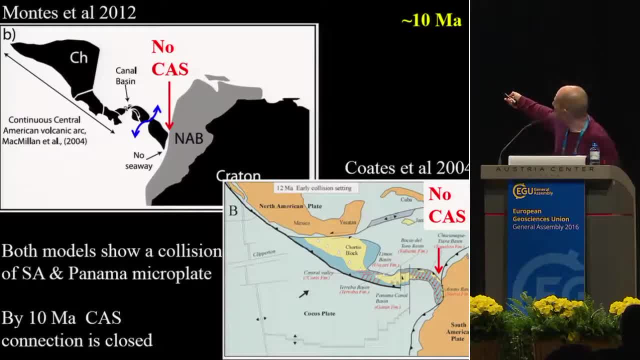 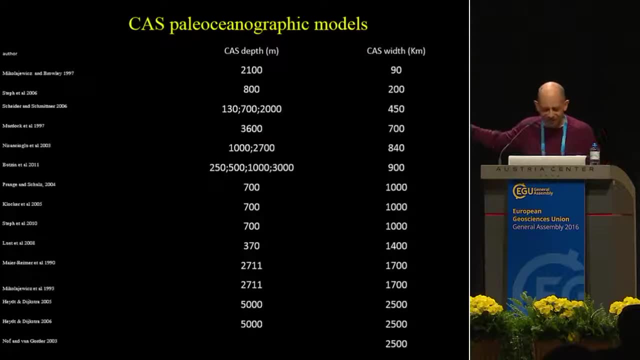 Okay, And it's really the same situation you see in the geography that had been proposed before, that the collision had already happened 10 million years ago. Now, if you are a paleoclimatologist, I think if you haven't done a model on the rise of the isthmus of Panama, 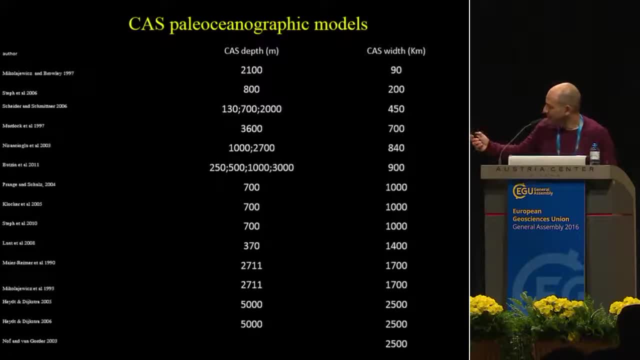 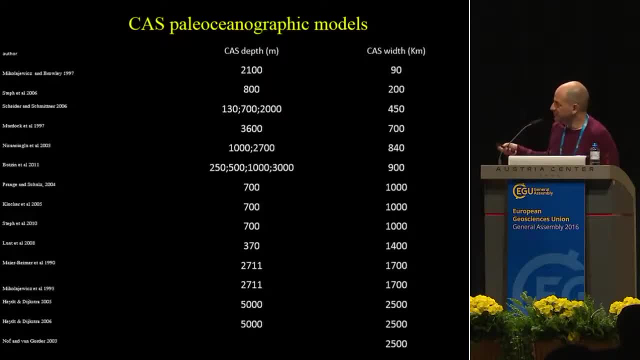 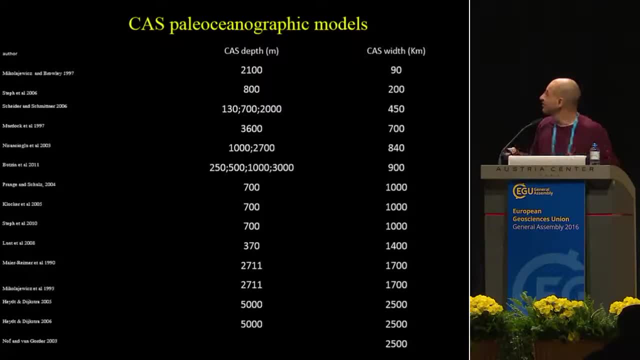 in the model itself. So you go from 5,000 kilometers of water depth to 130 meters, And also you go from 90 kilometers wide to 2,500.. So you can go from 1,000 kilometers wide to 200 kilometers wide. 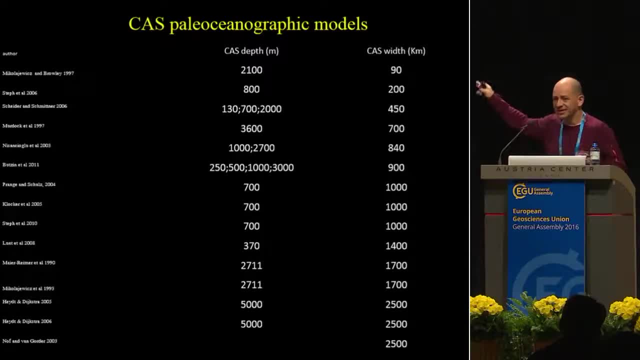 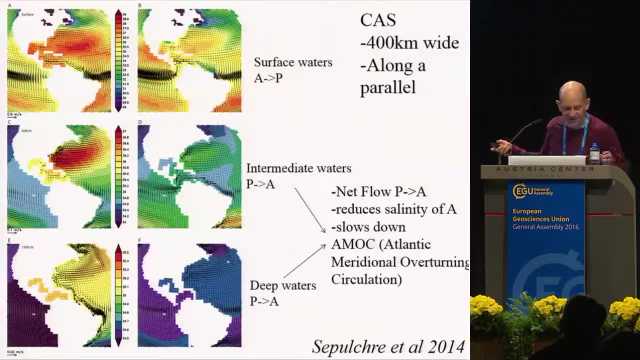 And this always has been assumed to be- 3.5 million years ago, Of course, with a model, and we did our own modeling and show the same result as many models have shown before, Once the isthmus of Panama is up, as you can see here today, versus what happened with 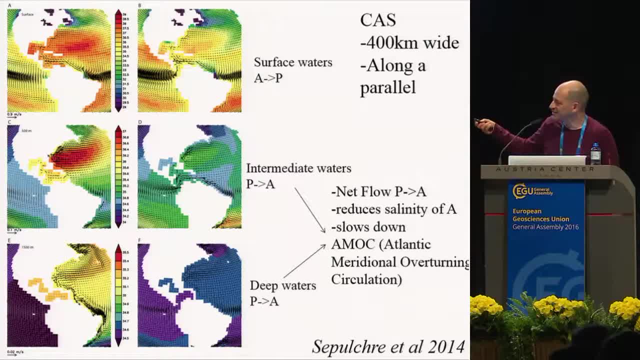 the isthmus is gone, The salinity of the Atlantic, especially in the deep bottom of Latin America, is fired, deep water and the intermediate water changes And once that happens, the thermohaline circulation that we have today is basically gone And every model 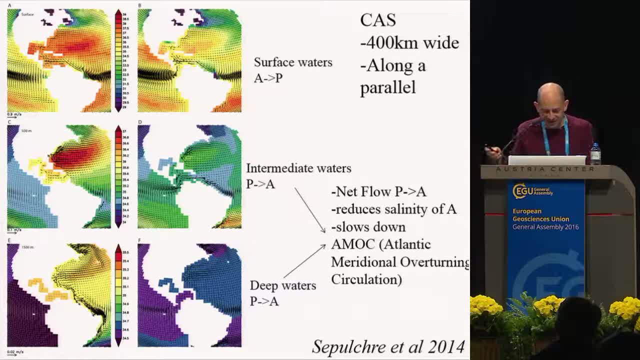 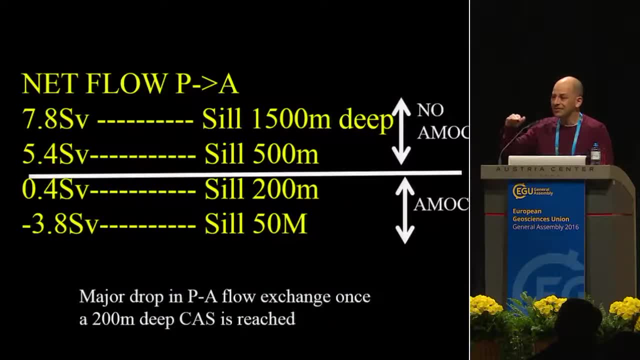 that has been published shows more or less the same thing. Something that we did differently here is that we explored the depth of the Central American seaway. What happens if the seaway goes from 1,000 meters of depth to 50 meters? 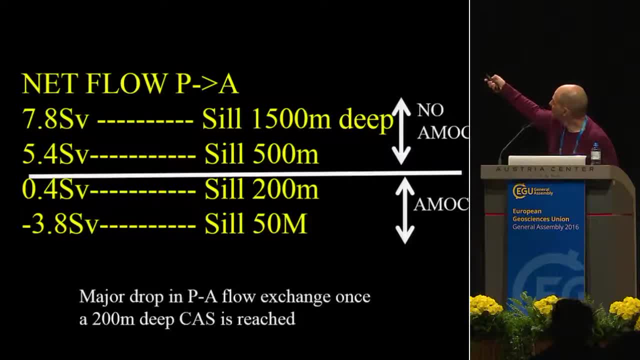 And Pierre showed in his model that once you cross this, you go from 500 to 200 meters of water depth. that in paleo-geographical terms is similar to the rise of the isthmus of Panama. So once you go to shallow waters, the exchange of water. 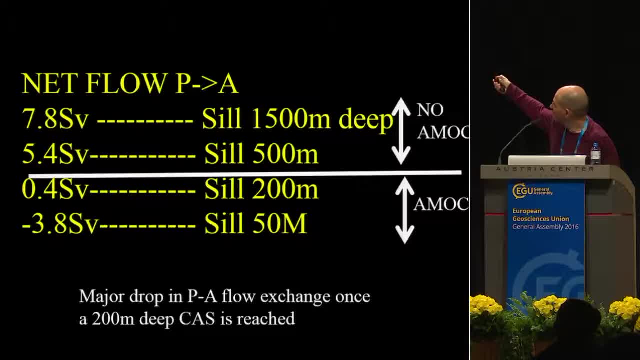 between the Caribbean and the Pacific is not enough to affect the thermohaline circulation. So in other words, if the seaway is deep, you don't have thermohaline circulation. If the Central American seaway is shallow, you have thermohaline circulation. Now how? 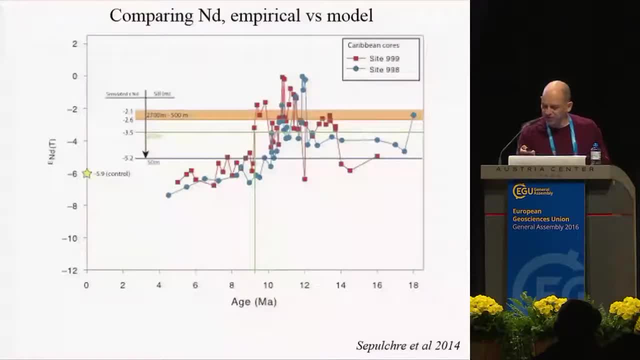 do you test that in the actual empirical record? So we use neodymium. That is a good tracer to see if you have waters coming from the Atlantic or coming from the Pacific, because the Pacific is surrounded by volcanoes, has a lot of neodymium, while the Atlantic doesn't. 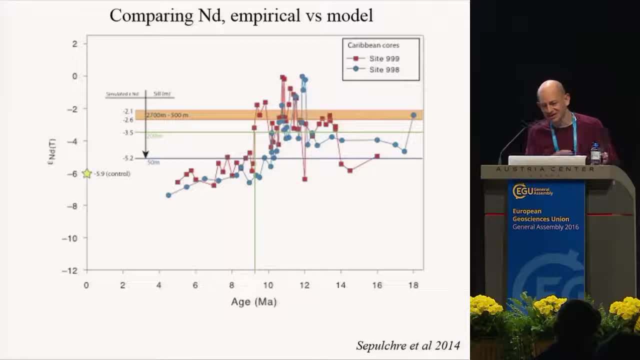 So it's a good tracer of if the waters are coming either from the Atlantic or the Pacific. And here we went to the Caribbean Ocean, to one of the ODP drillings in the middle of the Columbia Basin, And this line that you can see here is: 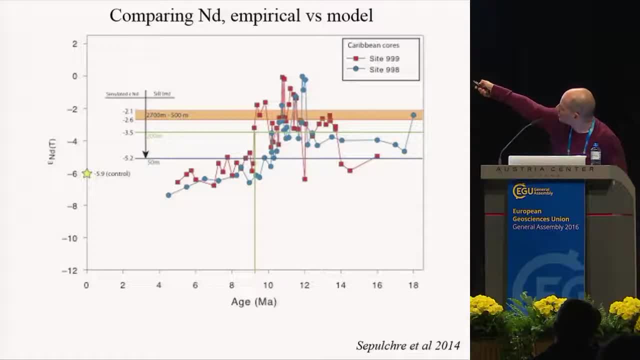 the neodymium values. And if the neodymiums are in this region, it's because the waters are from the Pacific, And if the neodymiums are in these values, it's because the waters are, let's say, from the Atlantic. And, as you can see, 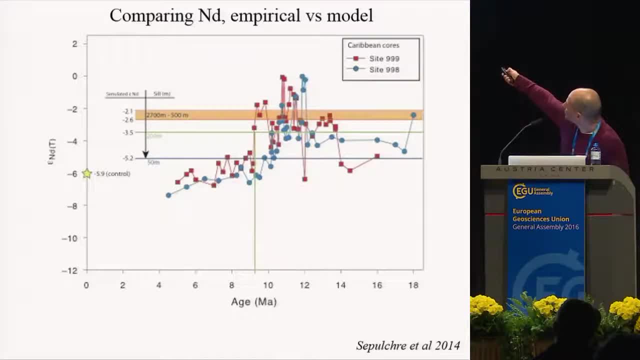 it's the same thing we have seen with the other data. Once you go from 12 million years to 10 million years, the water starts to be derived from the Pacific towards being waters derived from the Atlantic. And the same thing we have shown with the geology and also with the. 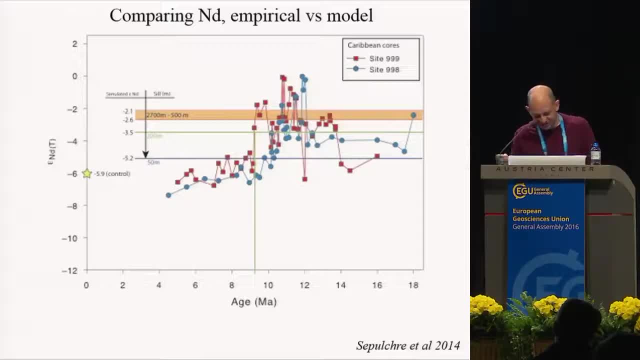 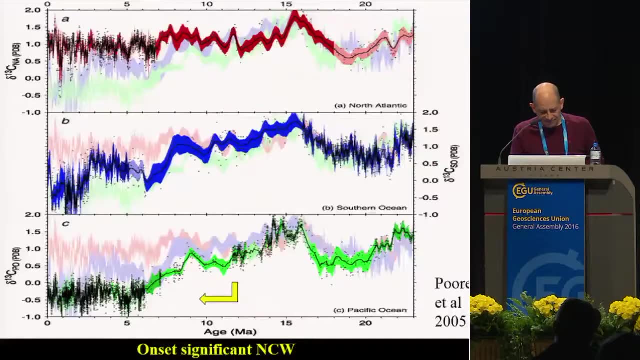 genetic data. But the 10 million years is really the trigger to the rise of the Isthmus, the real rise of the Isthmus of Panama, And when you compare with the evidence that we have of when the thermohaline circulation, 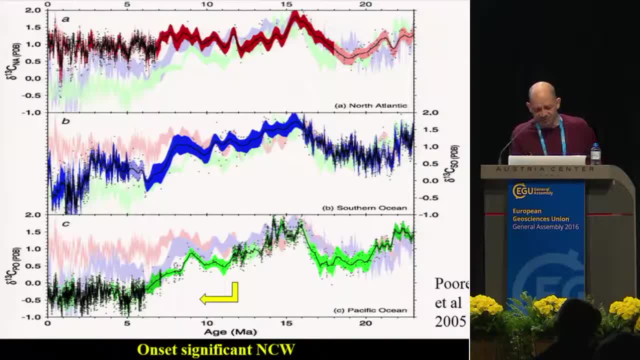 has been since when the thermohaline circulation has been operated. I think the two data sets match very well, Because there are many evidences that the thermohaline has been going on at least for the last 10 million years, And there was always. 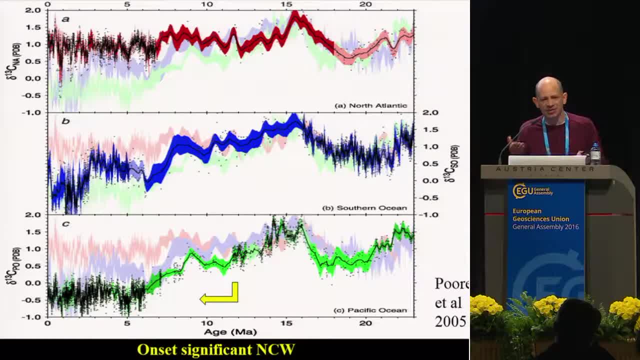 this connection. How come the Isthmus of Panama went 3.5 million years? Every model has been done as it indicates that once the Isthmus goes up, you have a thermohaline circulation. However, the empirical data from the thermohaline circulation show: 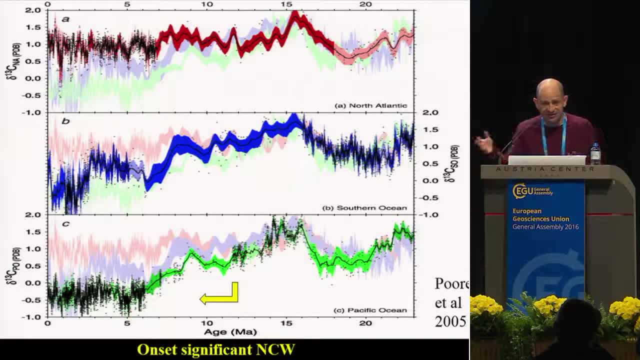 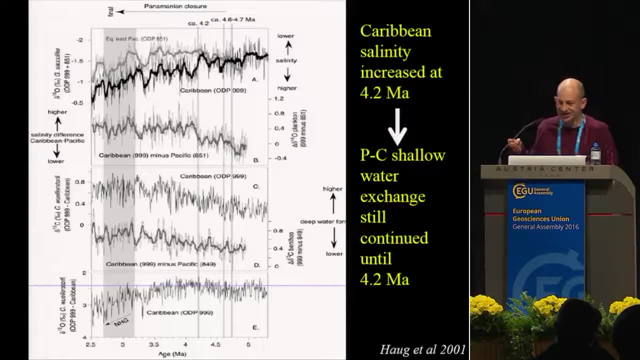 that it has been going at least for the last 10 million years, So I think the connection between the two events are really linked to each other. However, there are still a lot of evidences that the salinity of the Caribbean increased about 4.2 million years ago. 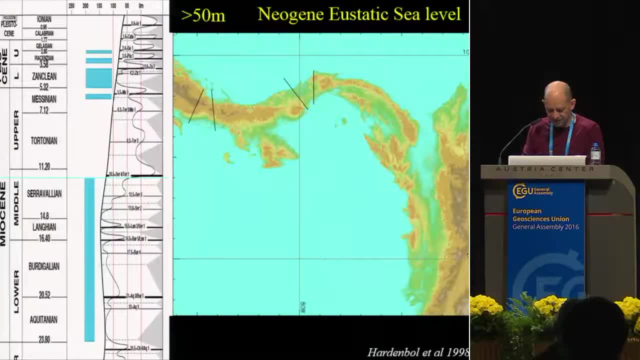 And I think you could explain that this simple geostatic sea level changes during the Neogene. So we think that between 10 and 3.5 million years, just the simple variation of sea levels going up and down and the small tectonic. 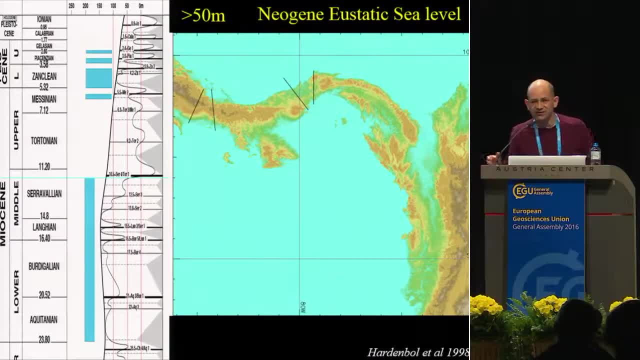 movements of Panama by 10, 15 meters will be enough to connect and disconnect the Caribbean with the Pacific over this period of time, But only shallow water and not a lot of water being exchanged between the two oceans. All of the 2.5 kilometers that many models have been assumed for. 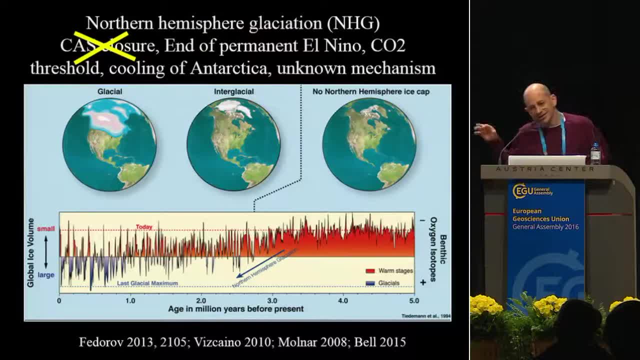 3.5 million years ago. If that's the case, we don't see any connections between the rise of the Isthmus of Panama and the initiation of the glaciations in the Arctic, And we are not the first ones saying that all of these papers over the past seven, eight years have shown. 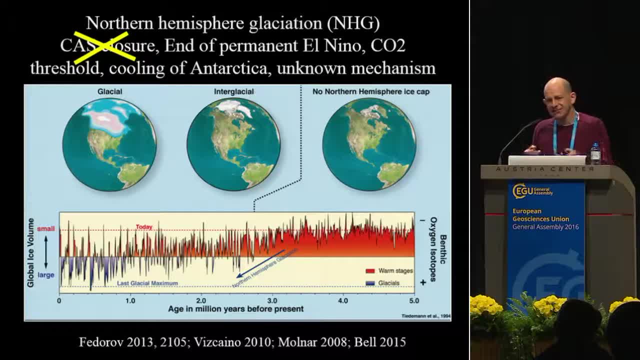 the same thing using different approaches. The rise of the Isthmus doesn't have to do a lot with the initiation of the glaciation in the Arctic, And the rise of the Isthmus was probably the best candidate. we have to explain why we have the climate. 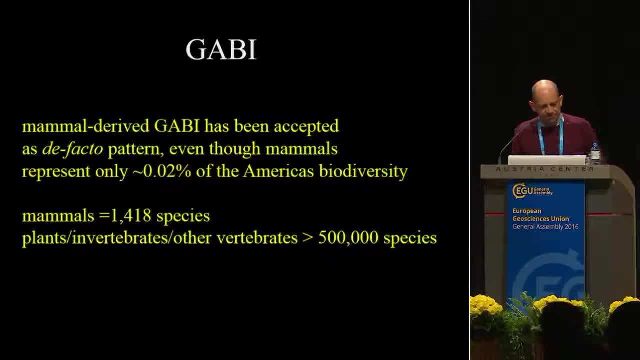 that we have today. Now, the last link, as I told you at the beginning, between the rise of the Isthmus is the great American biotic interchange. But really, when you look at the literature, this gap has been derived from the mammals themselves, And the mammals is only about 0.02%. 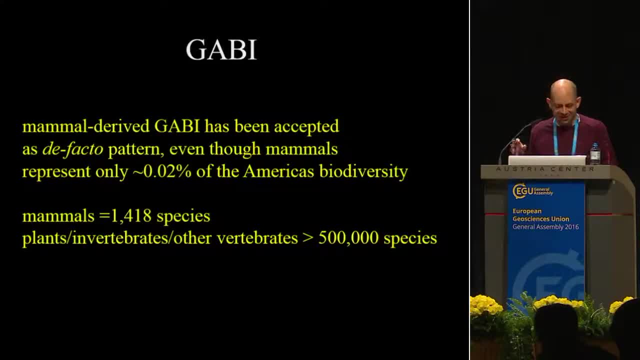 of all the species that live in the Americas today, Only 1,400 species out of half a million species of vertebrates we see in America. So the pattern of this great American biotic interchange is really a mammal pattern. As you remember, from the beginning the idea, 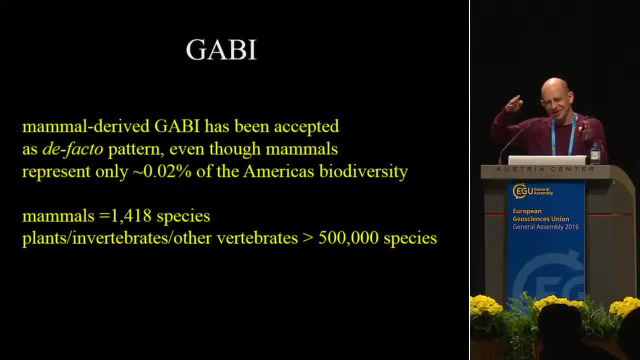 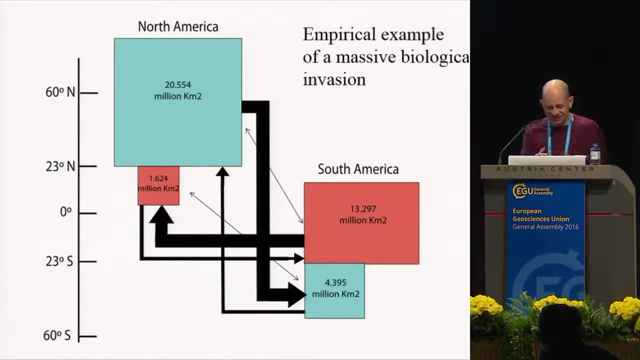 is that the North American mammals migrate faster and dominate the South American taxa, And this was because of the rise of the Isthmus. But if you think about what really happened when these two continents got together, it's really an example of what happened when you connect similar biomes. 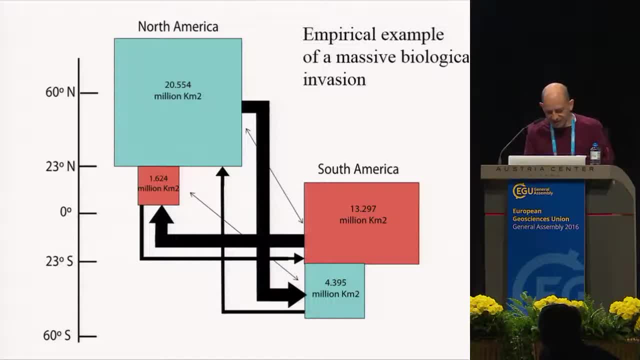 but with different sizes together. So if you are living in a North American temperate biome, you will see that before the collision the North American biome is really huge- All the savannas and temperate forests in North America compared to the temperate biome in South America. that is. 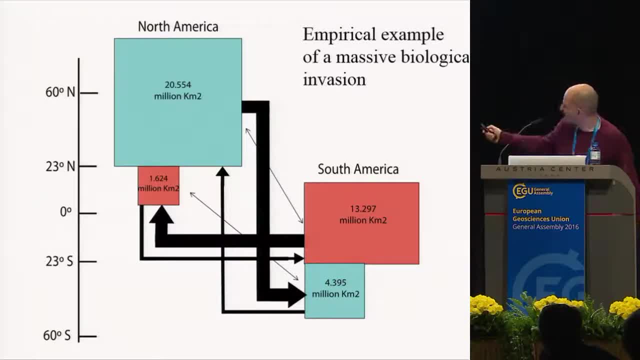 Patagonia and this other tip of South America that is really tiny in comparison to the area of North America. The opposite happens if you compare the tropics. The tropics of South America are a huge area compared to the tropics of North America. that would be between Panama and Mexico. 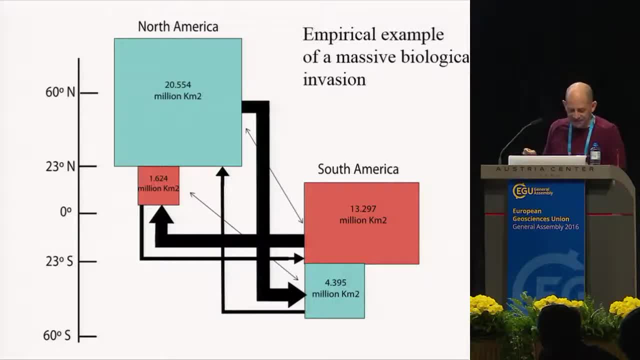 the Central American Isthmus, A very tiny area. So if you just join these biomes together just by simple population size, because the more number of individuals, the higher the ability to migrate to another place and they decrease the probability of extinction. 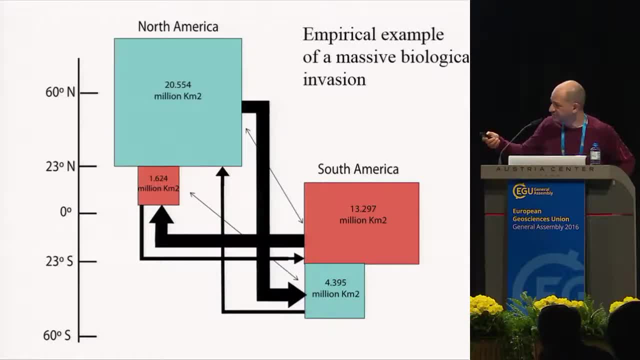 If you put these four biomes together, the prediction would be that the South American taxa will dominate the North American taxa in the tropics and the temperate mammals will dominate the temperate mammals of South America because of the difference in biome size. And this is in fact what happened. 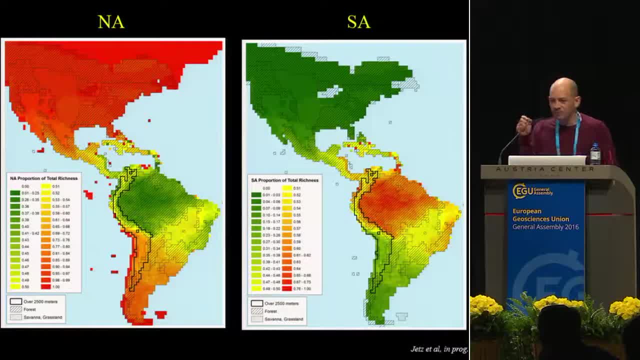 So in these two panels, what you see is the proportion of mammals today, The mammals that are living in the Americas today, that are separated by either coming from North America or coming from South America. So each of these is a pixel that represents a proportion. 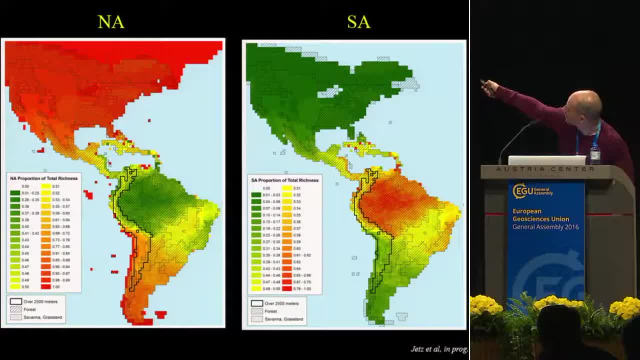 And here in this panel are the South American proportions and here are the North American proportions. So if the color is red, red is because the proportion is very high. If the color is green, it's because the proportion is very low. As you can see here, the mammals of the tropical taxa. 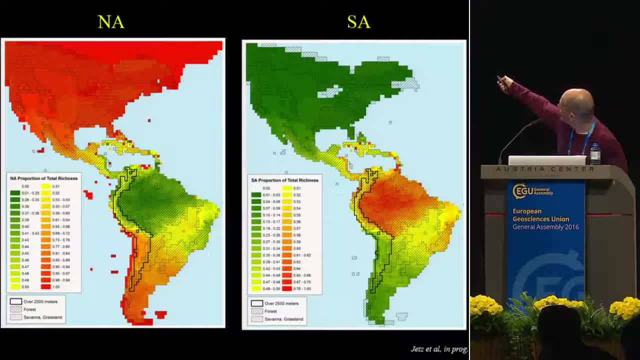 are really dominated by South American taxa, while the temperate taxa are really dominated by North American taxa here in North America and in Patagonia. So it shows you that if you think about the mammals again, if you think about the temperate mammals, 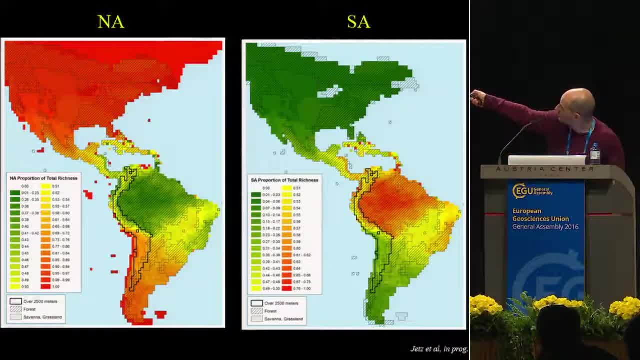 indeed, the direction of migration was from the North to the South, But if you think about the tropical mammals, the direction was the opposite, It was from the South to the North, Showing that, really, the size of the biome is one of the major drivers of this biological 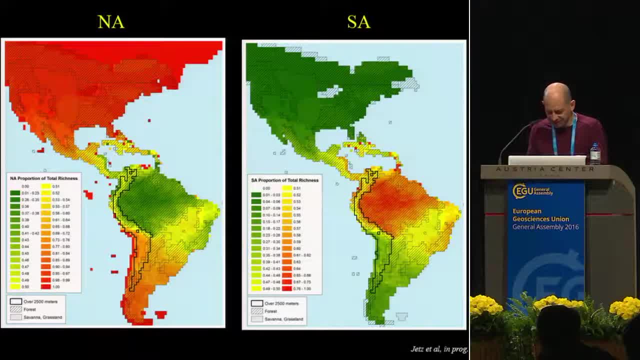 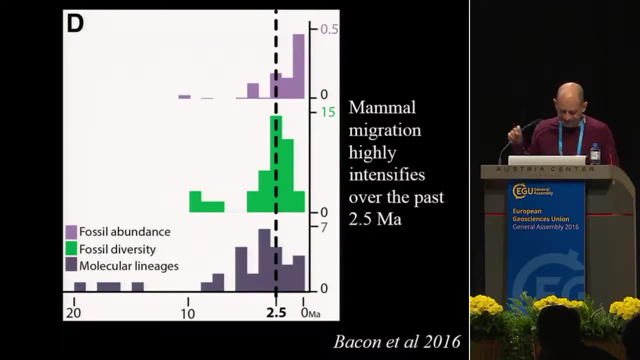 exchange rather than just the rise of the isthmus of Panama and the North American taxa being more competitive than the South American taxa. And also when you see when the actual migration happened, you see that the fossil record shows that it's not really at 3.5 million years but at 2.5 million years. 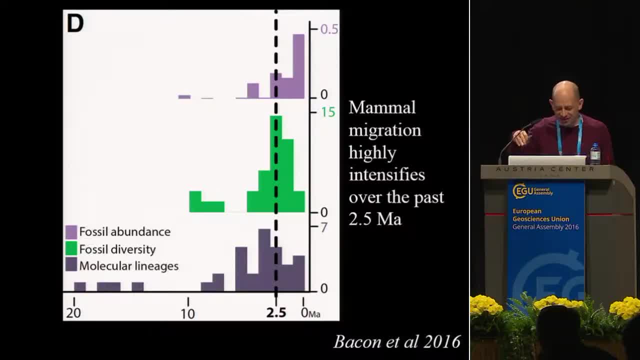 almost 1 million years later, There's a paper that is being published- I think it was published last week- and it shows how. so here are all the mammals, the proportion of the mammals that had migrated in both directions And, as you can see here, 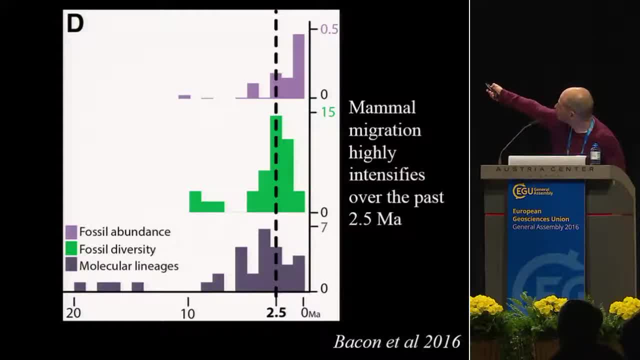 the actual migration, the onset of the migration. the fastest migration happened at 2.5 million years, Not before, Even though you still had the ability to migrate, at least for the past 10 million years, but the mammals didn't. So we think that the actual drivers of 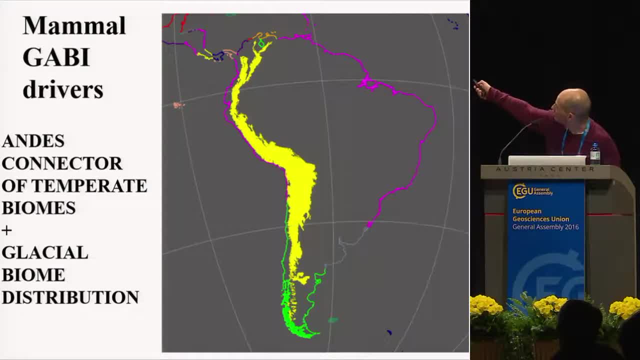 the migration itself rather than the rise of the isthmus of Panama are the combination of two elements: The Andes that act as a corridor for all the temperate taxa of North America to reach temperate areas of South America, And also by the changes in 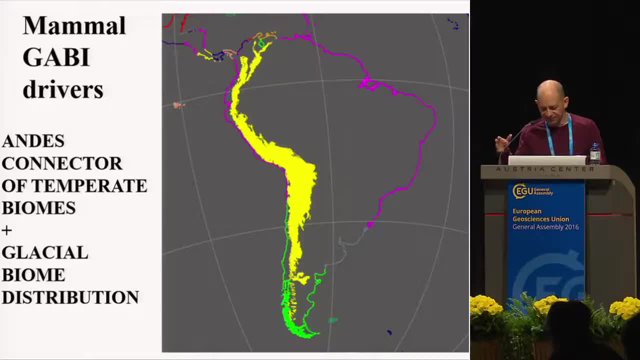 biome distribution during the last 2.7 million years, the glacial, interglacial cycles. Perhaps during glacial times, the spread of grassland vegetation or scrubland or dry forest increases, allowing this North American taxa that were not adapted to tropical rainforest to move toward the southern. 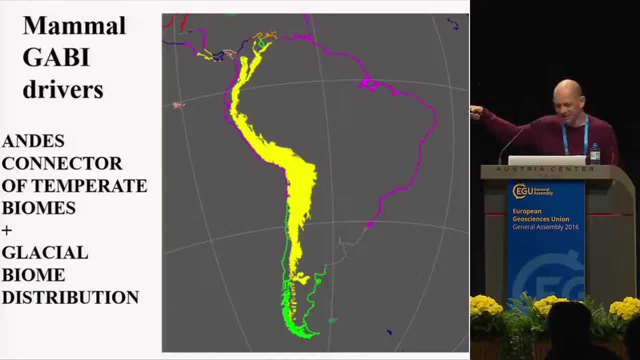 tip of South America And during interglacial times, the rainforest taxa moving into Central America. So the combination of the Andes plus biome is the actual driver of this great American biotic interchange in the Americas, rather than the actual rise of the isthmus itself. 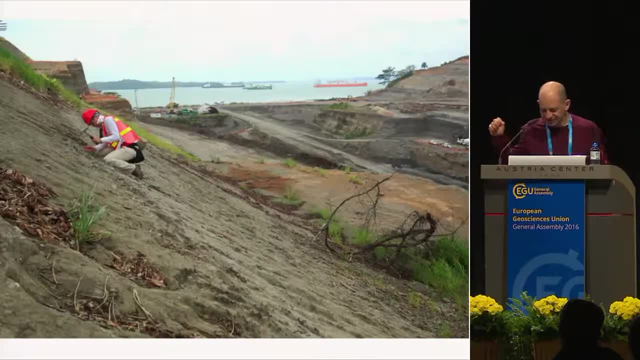 And finally, I think this example illustrates that every time you have the ability to collect new data, especially using this fantastic engineered work of the expansion of the Panama Canal, you have to do it, Even though this 3.5 million year idea has been. 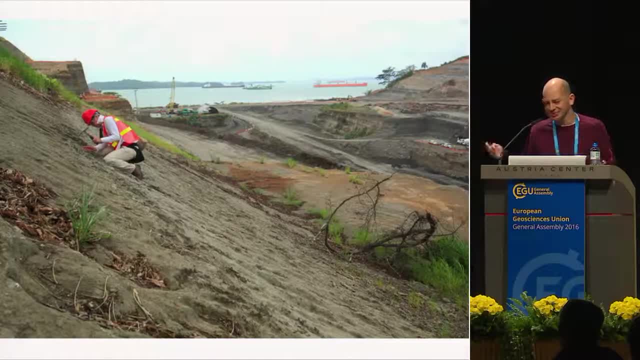 used for so many times for so many people during almost 25 years. the new evidence shows that probably that's not the case And we really need to re-evaluate many of these. many hundreds of papers have been using this as a priority. 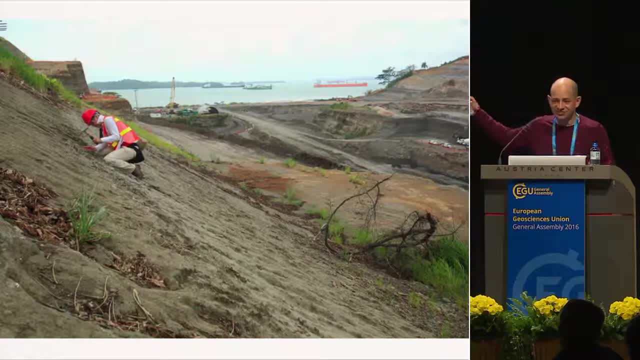 assumption that probably is not sustained by the geological data we have in Panama. So even people thatyou don't really need to work in Panama to have used this 3.5 million years. Just to finish, imagine you are working on a group of butterflies in Asia. 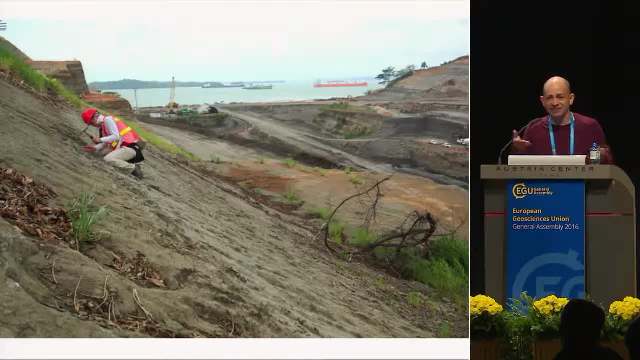 And because the fossil record of butterflies is almost non-existent, you will have to calibrate your phylogeny- if you are a biologist, using any calibration points, And so then you will use the calibration point of Panama. You have a butterfly in Panama. 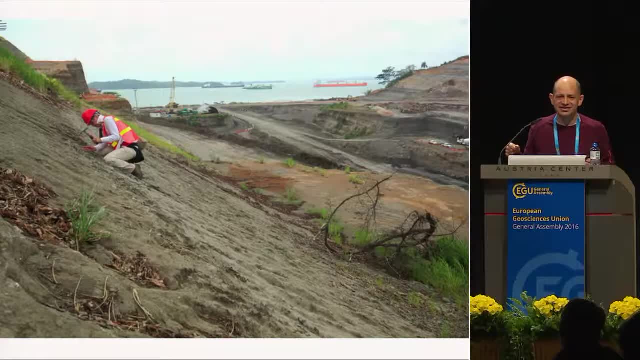 another in Colombia. You know that they split 3.5 million years ago, And then you will use the rate of molecular change in your group in Asia And that's how this 3.5 million year has been replicated worldwide. And, as I told you that we have to think, 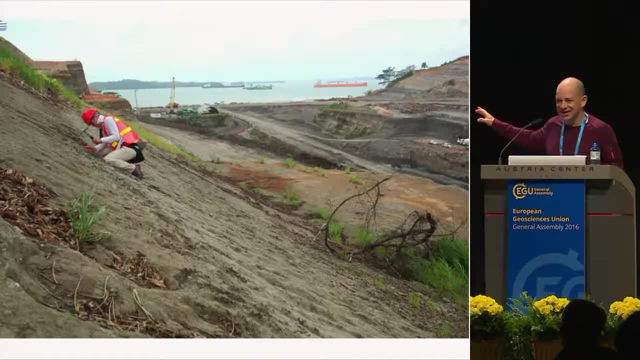 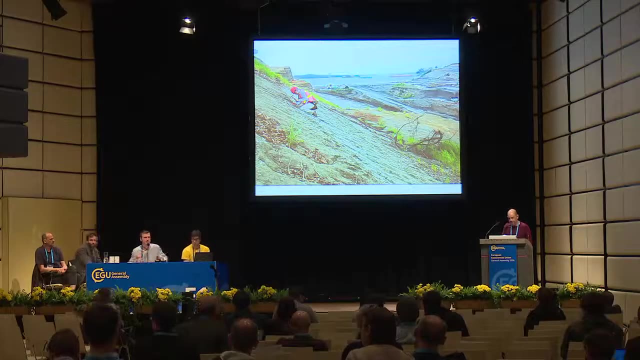 about that again And once again, show you the power of fieldwork, Something that we will never go away. Thank you very much for your time. Thank you very much, Carlos. Any questions from this inspiring talk? Yes, please, Hi, Fascinating talk. 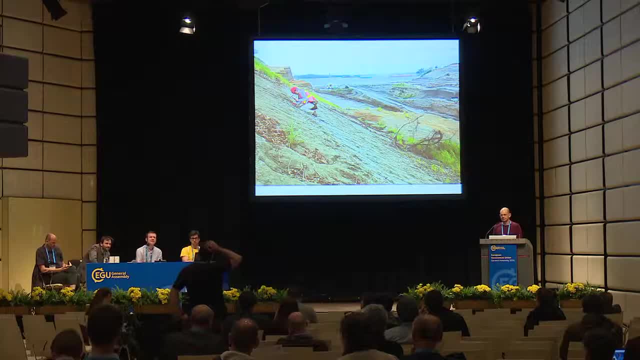 from University of Bergen. You maybe mentioned it, but it's still a bit unclear to me. So the isthmus shoaled about 10 million years ago, but the interchange didn't occur before about 2.5 million years ago. And what's the reason for that? And also in terms of other type of exchanges. 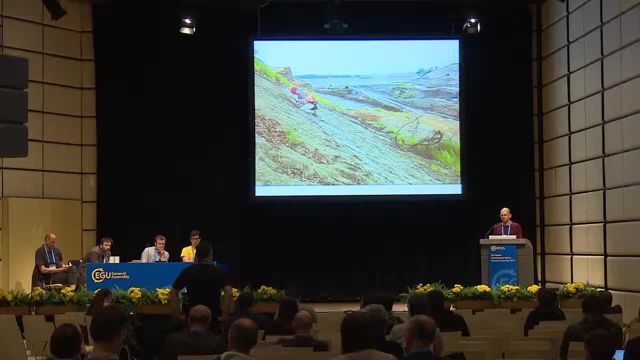 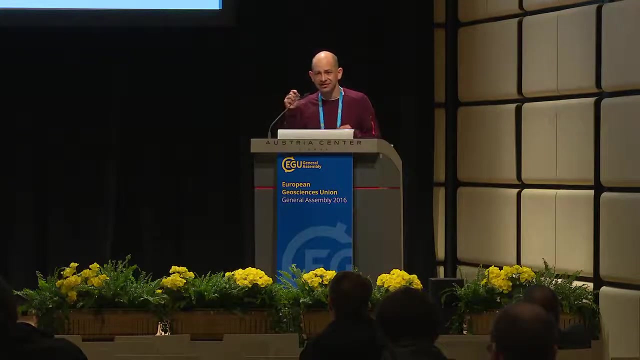 and more related to ocean and ventilation. there must have been large changes also before that that maybe would be nice to hear a little bit more about. Yeah, so for the mammals is when we see that the interchange start 2.5 million years ago, But for many other groups since 10 million. 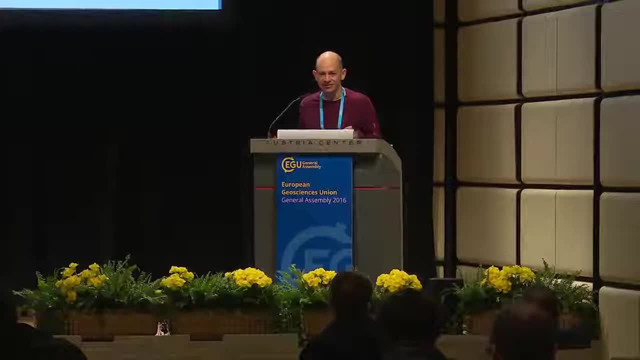 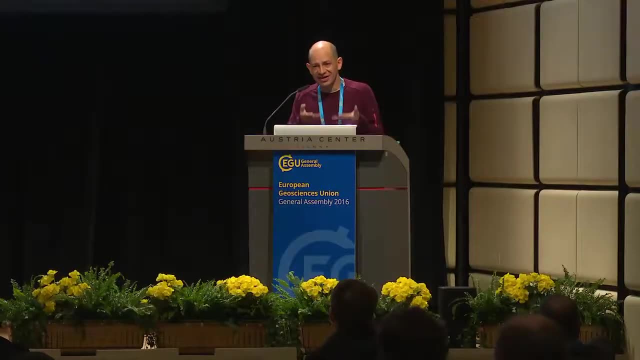 years. you see them going, coming, going back and forth. So this 2.5 million years is only for the mammals And, as I showed you, it's really driven not by the rice themselves but, I think, by the beginning of the glaciation interglaciation cycles. 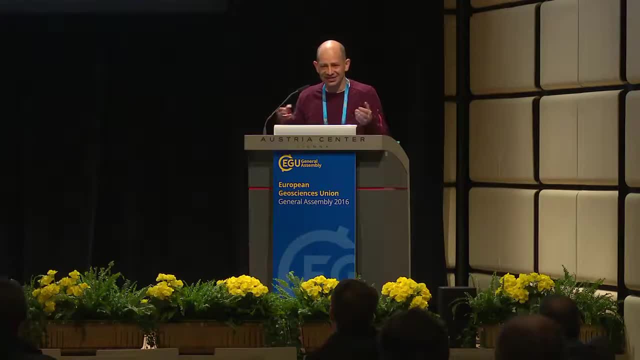 It's really a plasticine phenomena linked to glaciation interglaciations, And so between 10 and 3.5, we still think there are shallow water connections. Sometimes it will be disconnected as sea level goes up, as sea level goes down, And sometimes you will see connection as sea level goes up. or there is a new fault and you will have a 20 kilometer wide channel connecting the Caribbean with the Pacific. But I think, in terms of volume of water, at least the deep and intermediate water connection is gone by 10 million years. And the third question I forgot already. 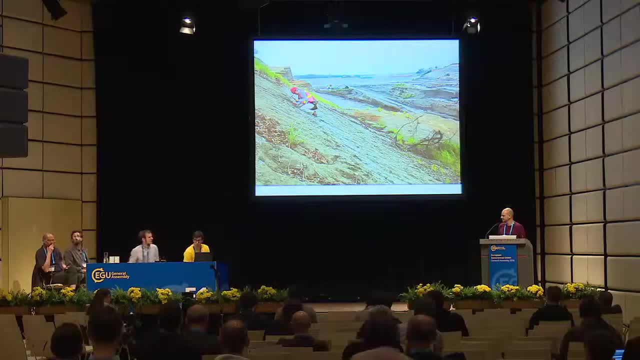 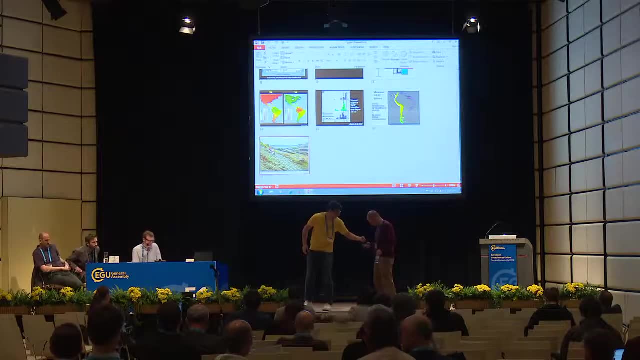 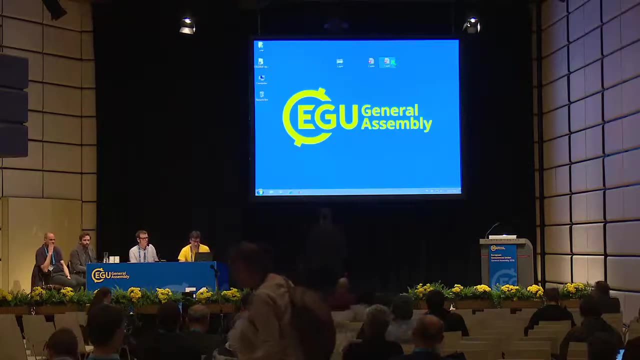 All right, Thank you. Unfortunately, it's time to move on to the next speaker. Thanks very much again, Carlos. The next speaker is going to be Henrik Sensen, and co-authors on the role of igneous and metamorphic processes in triggering mass extensions and earth creases. 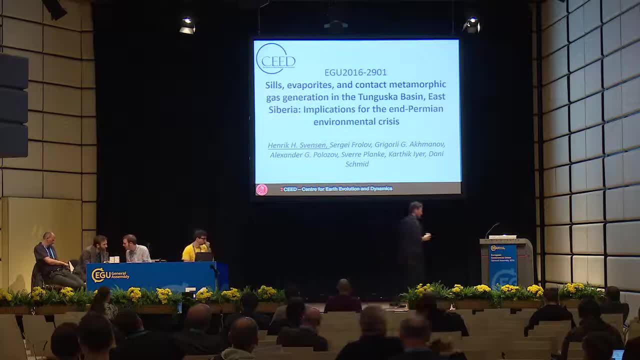 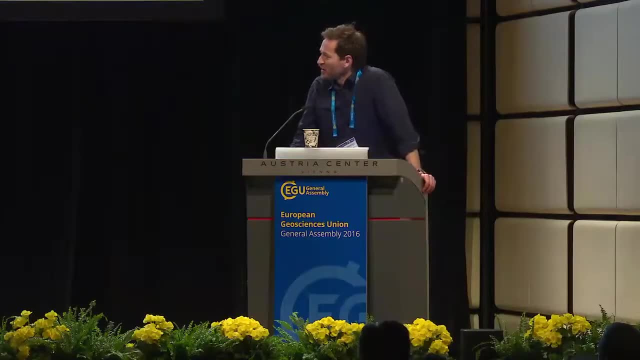 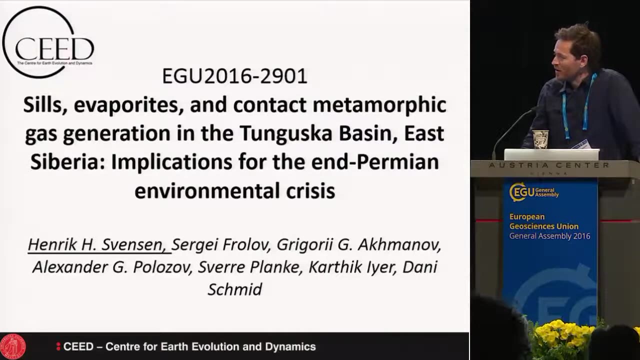 Good morning. Thanks for the invitation to give this presentation. Thanks for you for coming. I actually reorganized my slides last night, kind of late last night. I probably shouldn't have done that, because I've swapped my title page with a talk I'm giving after lunch today. 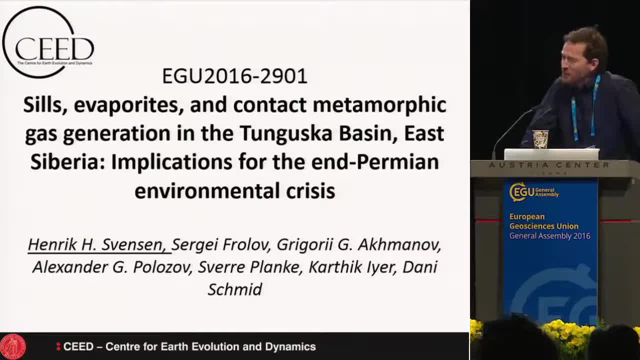 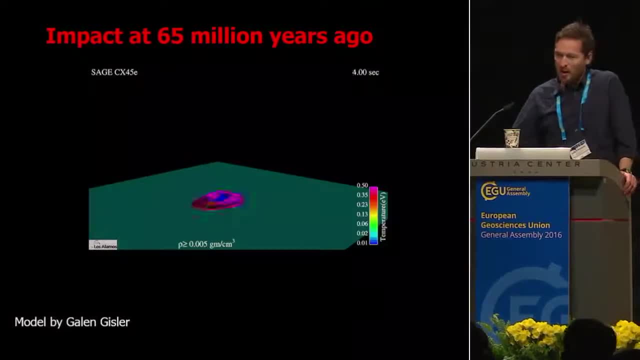 Of course, this is the only slide that shouldn't be here, But the topic is still the effect of solid earth degassing on mass extinctions and rapid environmental changes. Okay, This is one of my favorite animations. It was made by a former colleague, Galen Giesler. 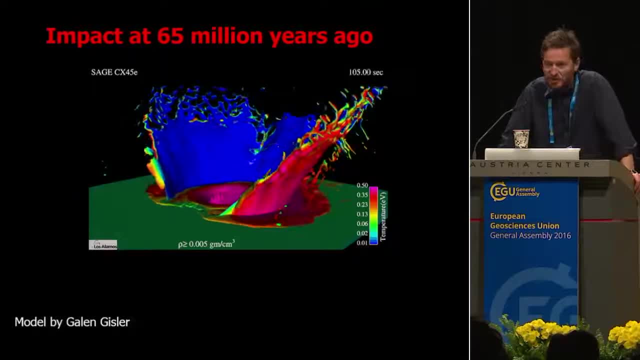 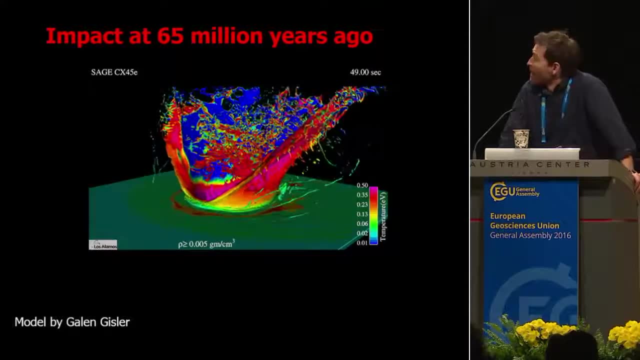 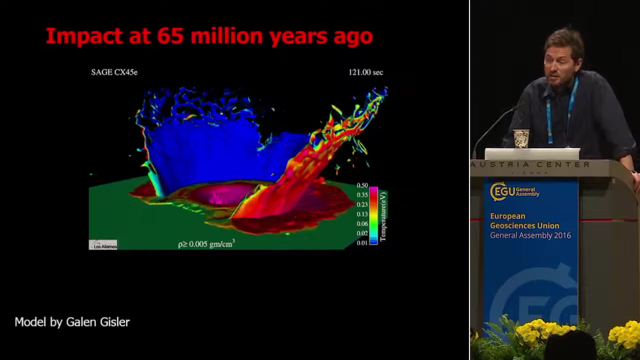 And it shows the kind of consequences or the impact of forming the Csikszentmihalyi structure in Mexico about 65 to 66 million years ago. When this story was first published by the Alvarez group in 1980, it changed quite a few things when it comes to understanding of mass extinctions. 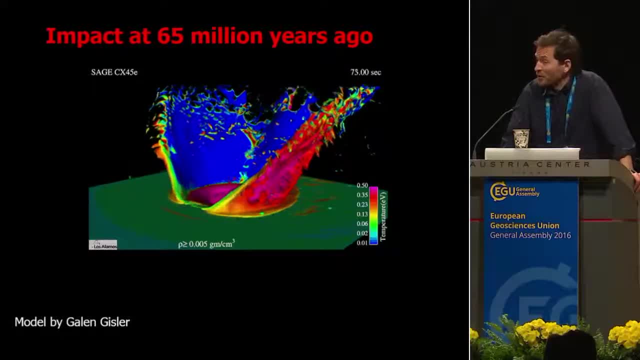 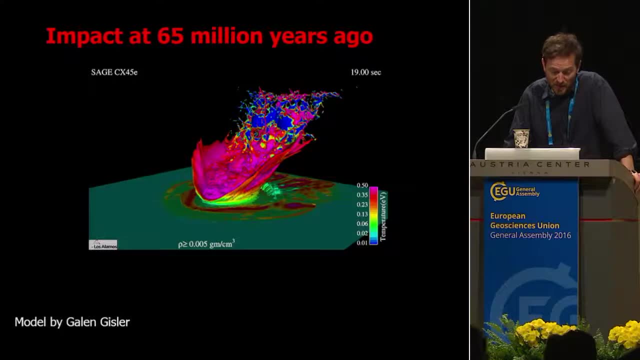 The public all of a sudden got interested in mass extinctions and also a lot of researchers got interested in extinctions, And then, of course, impact became a really really big thing. But there's another really really big thing when it comes to mass extinctions. 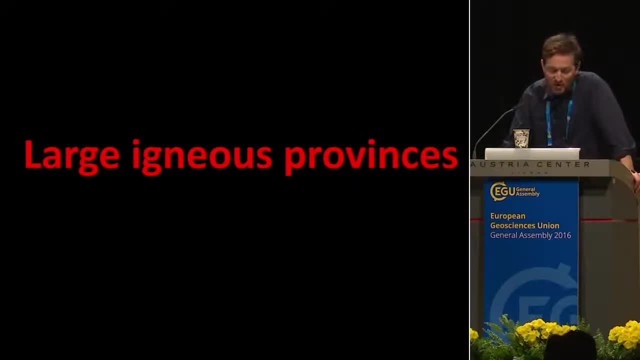 and that's large igneous provinces. And these large igneous provinces, or LIPs which we call them, have been associated with extinctions since the early 70s. But then when the Alvarez group arrived with the impact theory, it kind of swapped away all the foundations for linking extinctions. 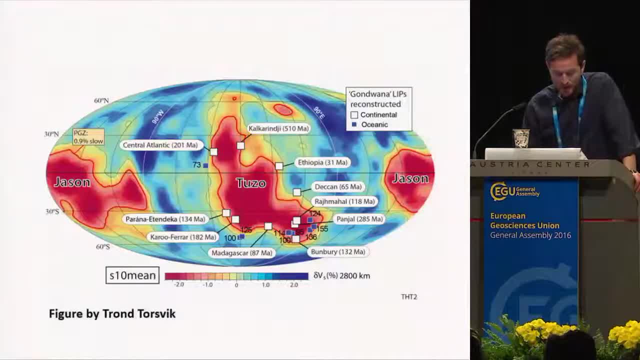 to large igneous provinces. A little bit about LIPs. This is a figure by Trond Torsvik. He's a colleague at the Center of Earth Evolution and Dynamics at the University of Oslo. He's linking LIPs to processes occurring at the core mantle boundary. 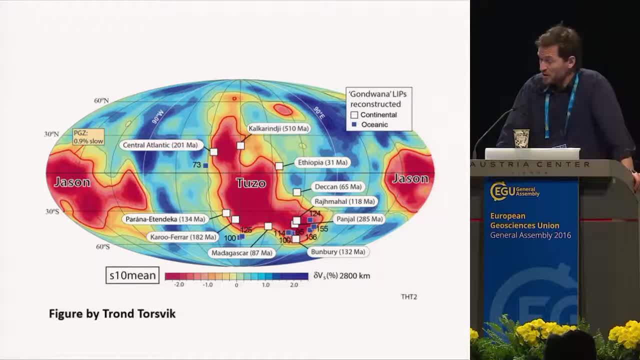 And this figure is a reconstruction showing the positions of LIPs related to Gondwana and also the positions of low shear velocity zones at the core mantle boundary, And it seems to be a fairly good agreement between these two. So the idea with the large igneous provinces is that they are sourced. 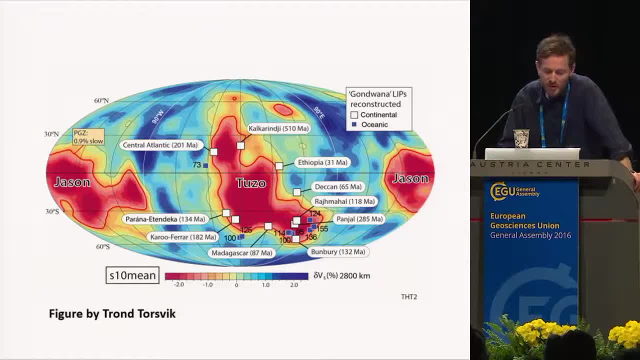 from the core mantle boundary and that plumes are connecting these deep structures with the surface. And, of course, when these magmas enter the surface, they enter the crust, forming sills and dikes, and then lavas and pyroclastic deposits at the surface. 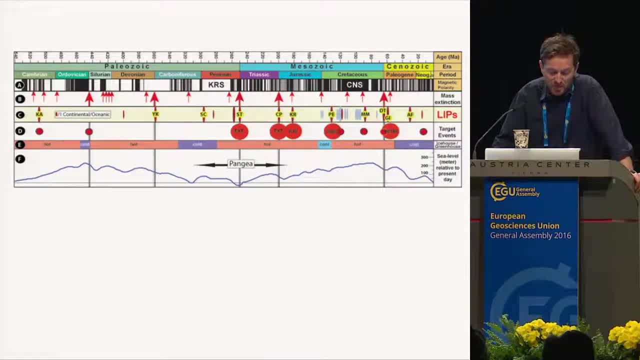 So, when it comes to extinctions, large igneous provinces and impacts, what does the record tell us about? Well, we have the big structures, We have the time scale. We have the Paleozoic, the Mesozoic and we have the periods with the Permian Jurassic and so on. 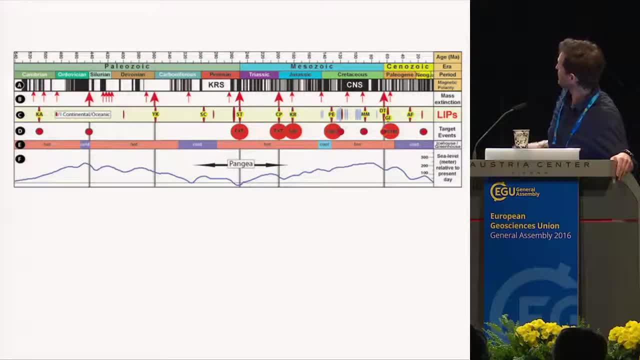 that you all know about And, of course, all the boundaries, the major boundaries are defined by these big events, with extinctions, with global warming episodes and so on, And really the big question is: what is the trigger? 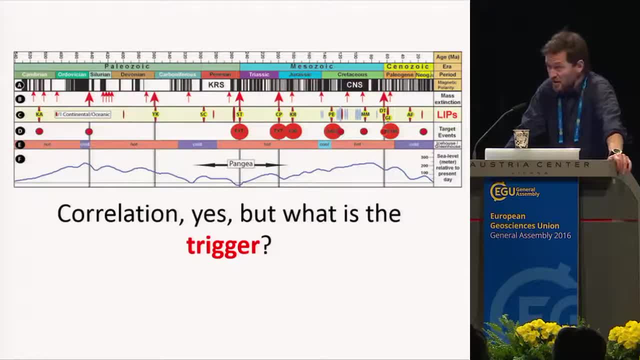 What is the link between these major episodes and changes in Earth history and the triggers, geologically speaking? Also interestingly, of course, is that, when it comes to impacts, it's only the K-T boundary that is currently associated with impacts. 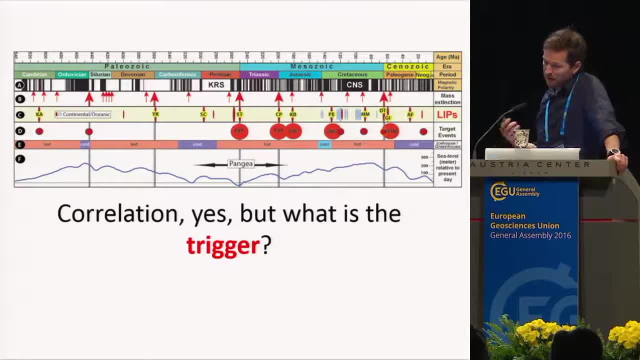 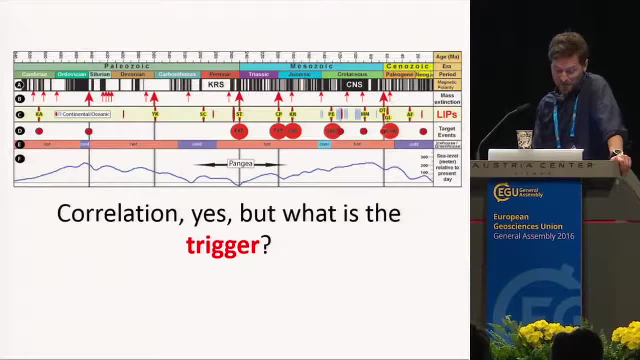 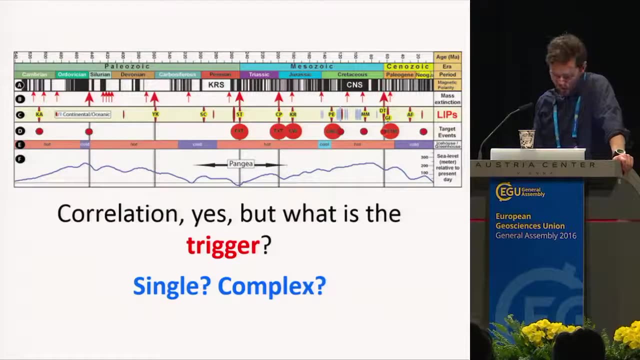 and all the other extinctions are related in time with large igneous provinces. But then again, what is the direct link between LIPS and environmental crisis? And that's a topic that I've been studying for 10, 15 years. It's not a simple question, of course. 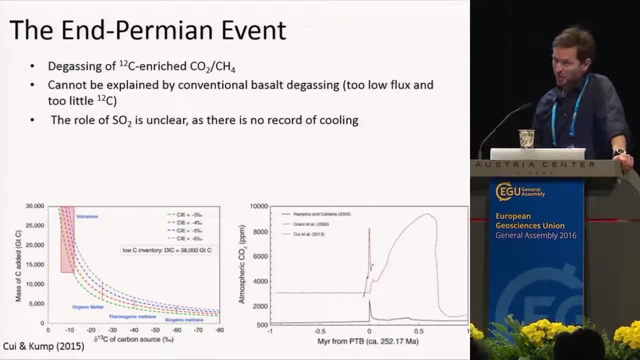 and the answers are kind of complicated, So I would like to continue now with zooming in on the end Permian event. So what do we know about the end Permian event? It's the biggest mass extinction, related to 95% demise of species. 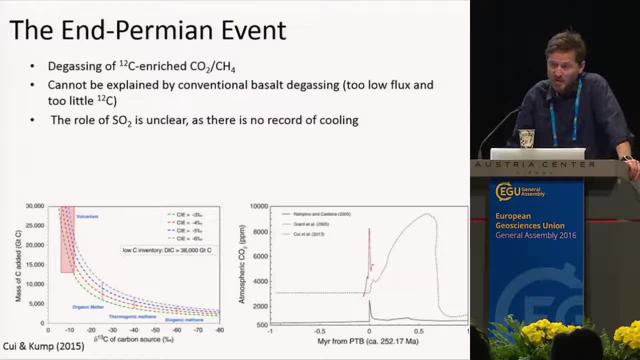 And what we know is that it was associated with a degassing of carbon-12 enriched gases, CO2 and or methane. And the interesting thing is that this degassing cannot be explained easily by conventional basalt degassing, And that's because the flux of basalt degassing is too low. 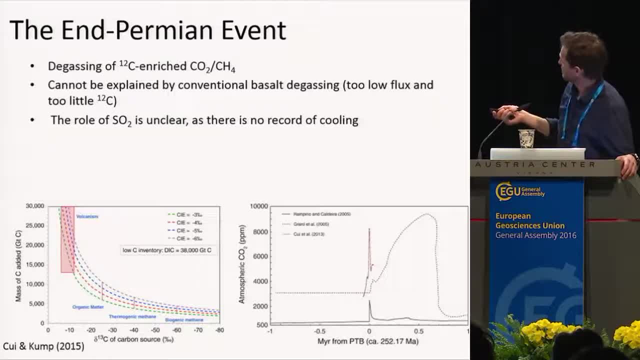 and that it contains too heavy carbon, which can be seen in this diagram down here By from last year that the mass of carbon ejected into the atmosphere and when you look at the carbon isotope anomalies in proxy data, volcanic CO2 is too heavy. 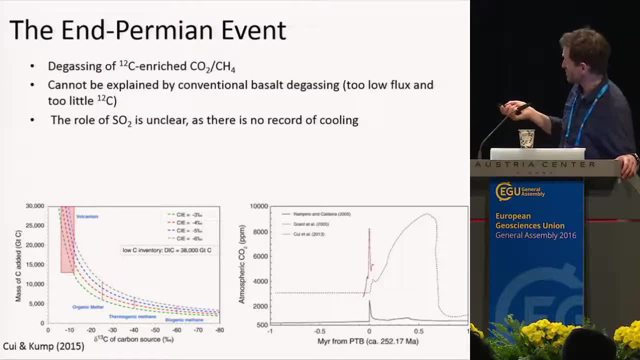 isotopically heavy to explain carbon isotope excursions, because it has a value of about minus eight And you need really really large amounts of carbon to explain carbon isotope excursions with volcanic CO2.. It's much easier with carbon coming from organic matter. 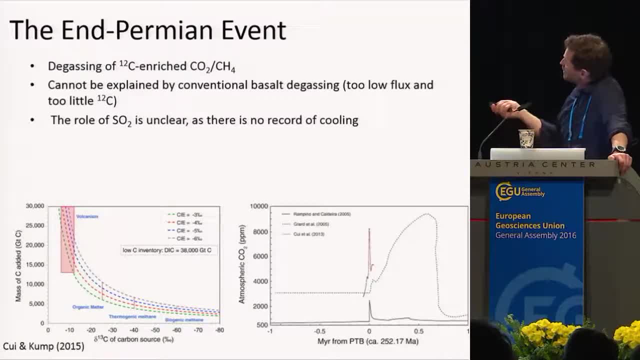 thermogenic methane and also biogenic methane. You need lesser volumes to explain the same type of carbon isotope excursions in the geological record And of course, also at the PTE boundary. the atmospheric CO2 concentrations rose really high, depending on which models you take. 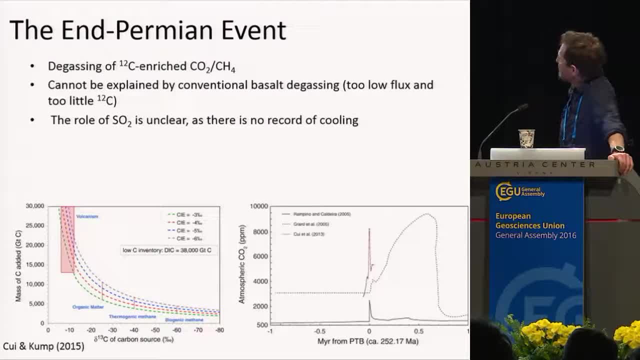 But still we're talking about a rise of maybe several thousand ppm CO2 in the atmosphere. The role of SO2 in the solid earth, degassing and, in the end, permanent, is unclear. If there was substantial volcanism, we could expect that SO2 was emitted to the atmosphere. 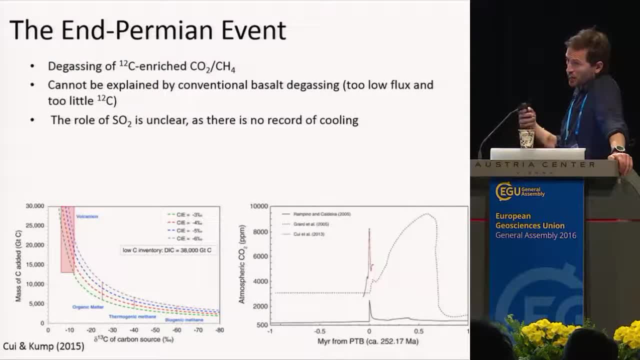 and that there should have been an associated global cooling related to SO2 being ejected into the stratosphere. The thing is, there is no record of cooling at that time period. A major challenge is that when you look at proxy data, the resolution is typically in the thousand years range or more. 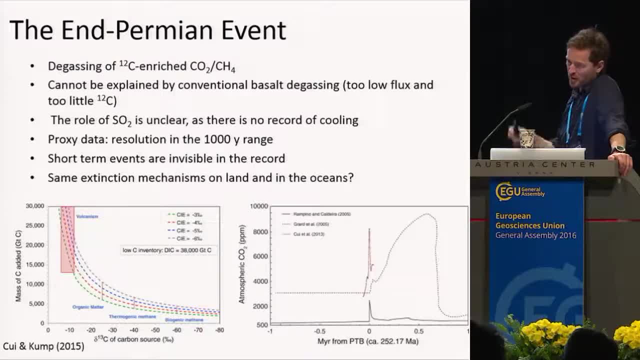 meaning that you might only have one data point or a few data points across a 10,000 year time period. And, of course, if you have degassing from volcanic eruptions, those perturbations and anomalies will disappear after a period of. 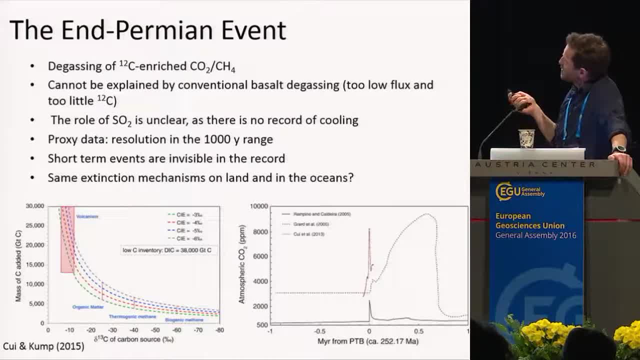 let's say, 10 years maximum. So the big thing here is: if there was any cooling related to SO2, would you even see it in the proxy data records? Probably not. Short-term events are kind of invisible in the records. 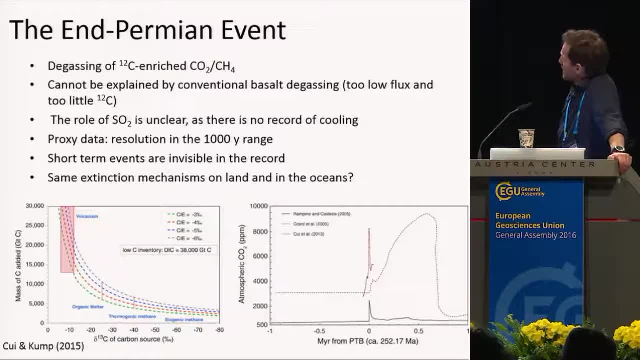 You get like an average signal when you look at proxy data records. Another big thing with n-permin is the relationship with extinction on land and in the marine realm in the oceans. Did the same extinction mechanism operate on land and in the oceans? 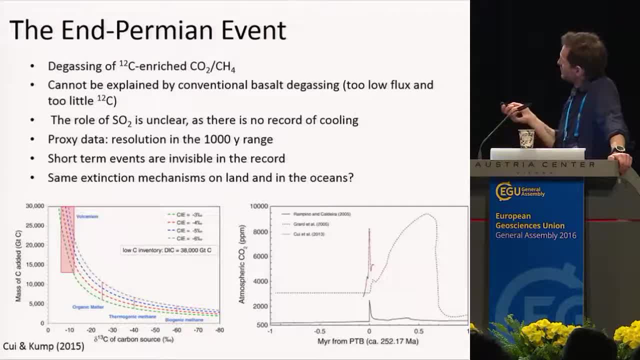 or was it totally unrelated issues? For instance, on land we have the global warming forcing and also atmospheric effects related to ozone levels, And in the oceans, the extinction is related to oceanic anoxia, which is in a way, connected to CO2,. 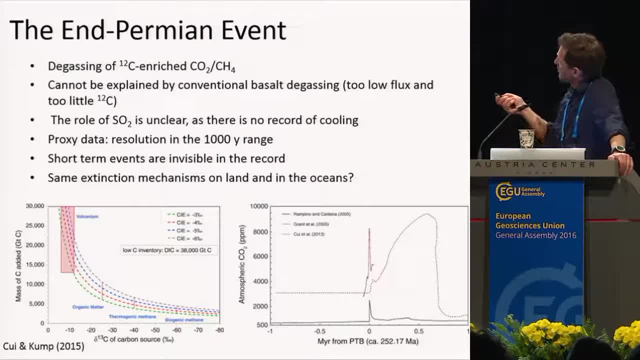 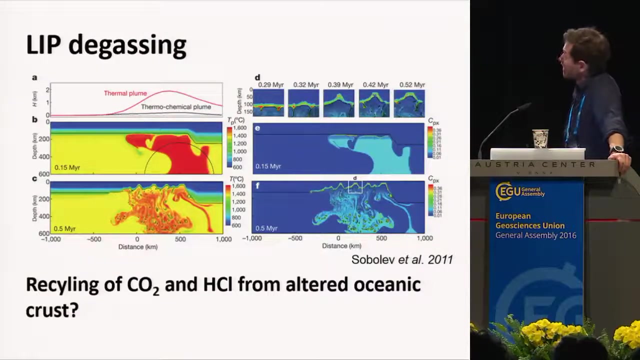 but also to ocean currents and ocean currents at that time. So the pattern is fairly complicated when you compare the different reservoirs and the effects in those. So I said that the volcanic CO2 degassing cannot really explain proxy data, but I would like to stress that there's a couple of models available. 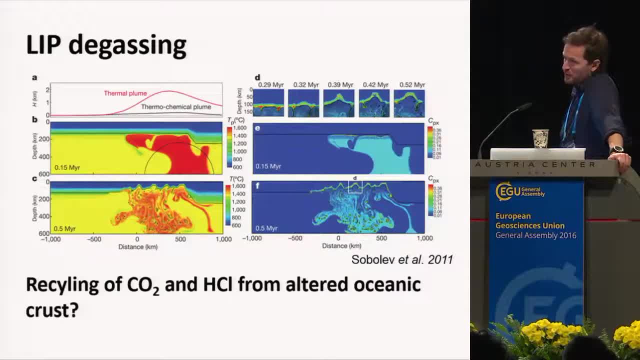 that might provide answers to why volcanic eruptions, let's say basalt degassing, also could have resulted in higher CO2 outputs and also other gases like HCl. So this is a model by Sobolov et al from 2011.. 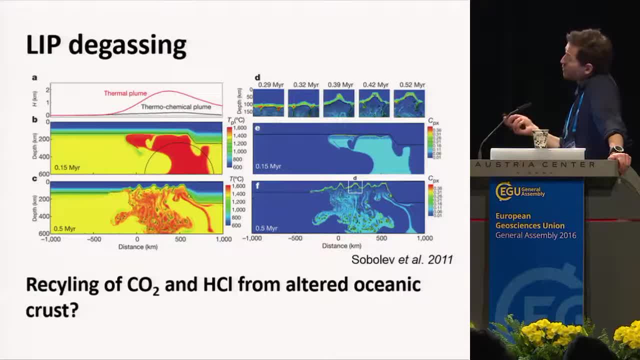 And what they really suggest is that, based on the n-permin case and the sub-Aran traps in this province, they claim that recycling of CO2 and HCl from altered oceanic crust in a mountain then contribute to the degassing and that can explain the extinction. 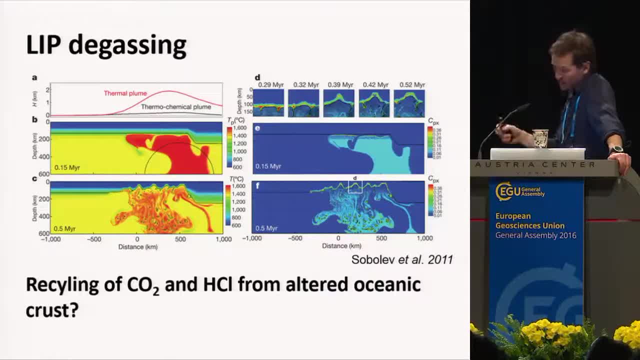 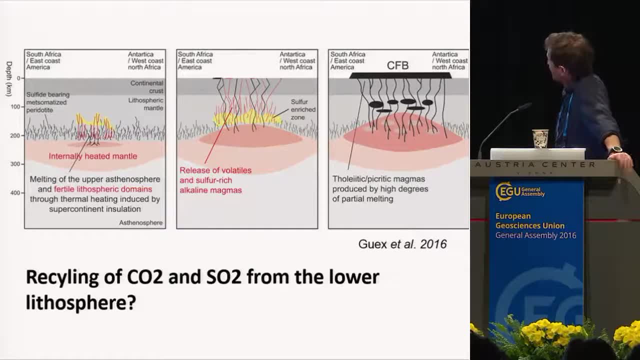 then purely by looking at the volcanic system, the basalts and the basalt degassing alone- And this has recently been followed up by a publication this year by GUE et al, And they suggest that recycling of CO2 and SO2 from what they call a thermal erosion. 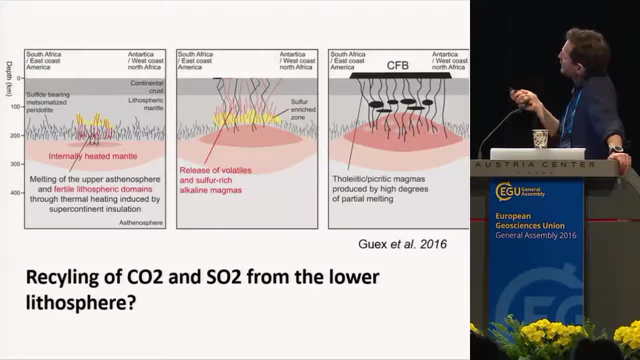 of the lower lithosphere, mainly in a way a fairly similar process to the Sobolov et al suggestion, but that recycling of crustal material can explain higher CO2 degassing and SO2 degassing compared to a normal basalt type of degassing alone. 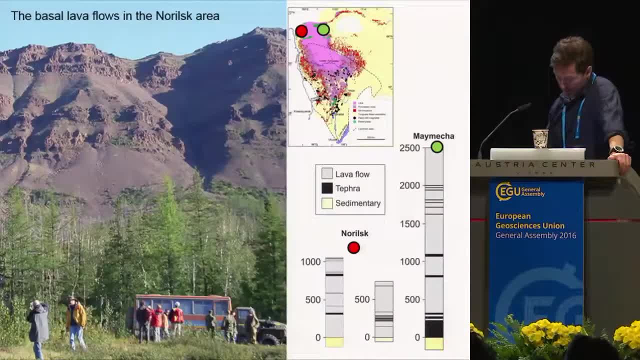 So these ideas are interesting If you look at the basalts in the province itself. this is a map of East Siberia. You see the province, the volcanic province, in red. it's sills part of the sub-volcanic plumbing system. 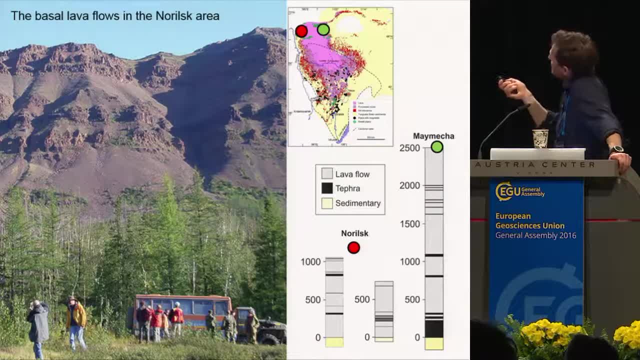 and in purple colours it's pyroclastic deposits and these lava flows and the flood basalts. So the idea is that with these recent publications that degassing from the basalts alone maybe could have triggered the extinction, We do find fairly substantial thicknesses. 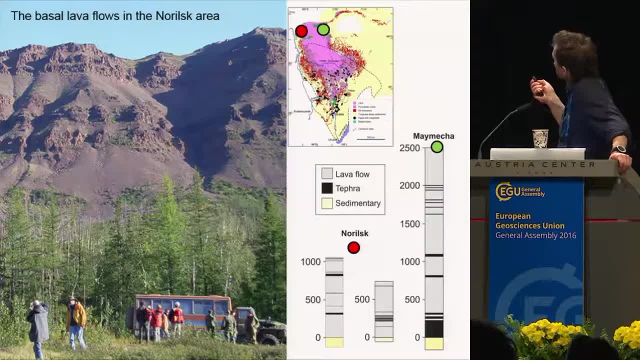 of basalts in the province Thickest in the Myrmecha area up here. so it's about two and a half kilometres preserved of lavas. In the Norilsk area, which is a little bit further west, we have about a kilometre of preserved lavas present. 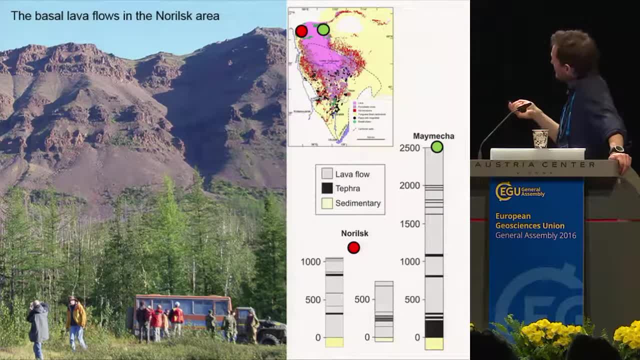 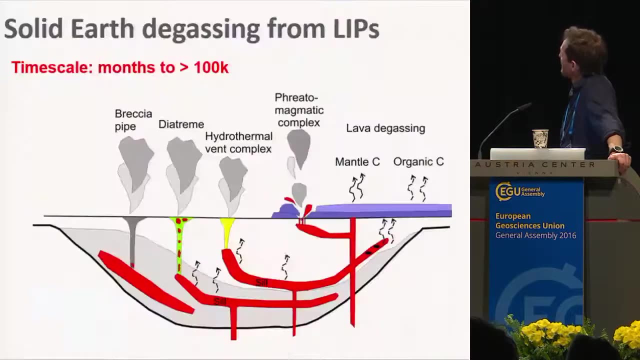 And then we have the paleolandscape that these lavas erupted upon. So to summarise that part, the research idea is out there that still the basalts can explain the extinction of the P-T boundary. So I want to move on to a topic. 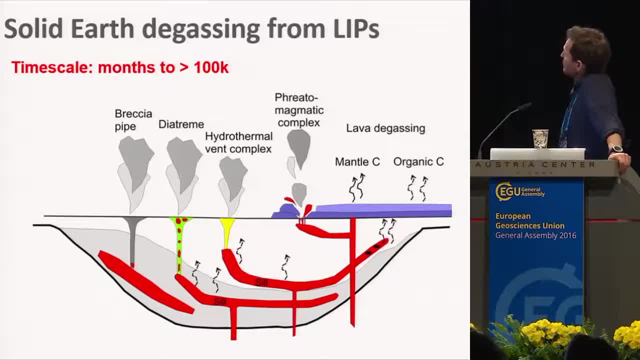 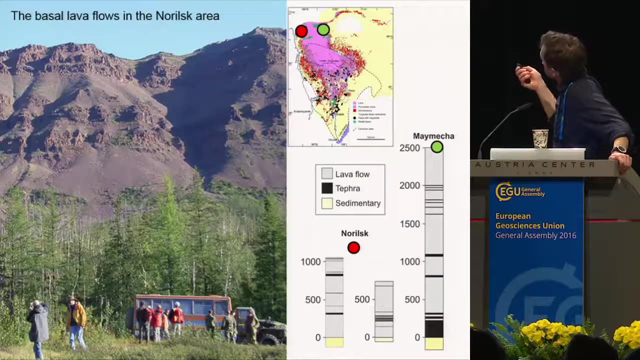 which has been my contribution into this story, and that's solid earth degassing from the sedimentary basins affected by the large-scale provinces. So if I go back one slide, I mentioned the sediments. we see all the sills in Siberia. 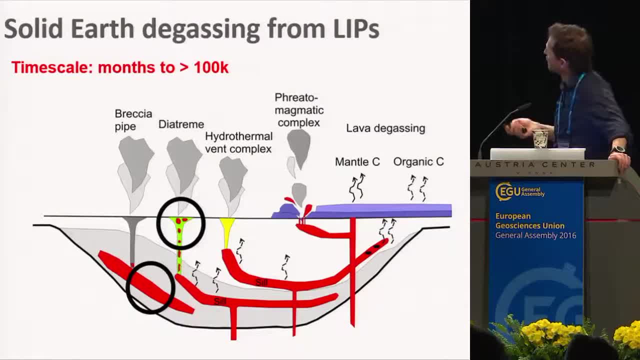 and sorry, this is kind of like a schematic cross-section across Siberia or any other type of volcanic basin, as we call them So volcanic basins. they contain a lot of sills emplaced into the normal sedimentary strata that we find in basins. 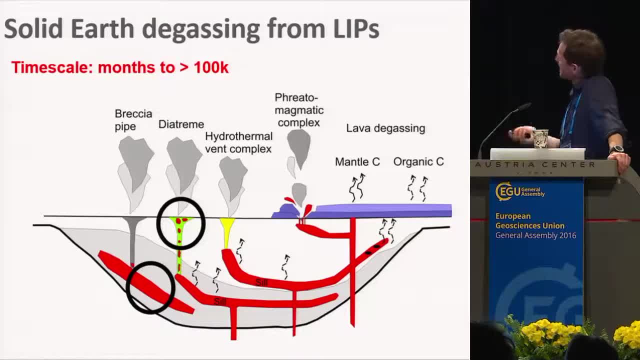 It can be shales, it can be evaporites, sandstones, etc. And the idea is that the portion of the large-scale provinces being emplaced in sedimentary basins generates a lot of heat. When they cool, they heat the sedimentary strata. 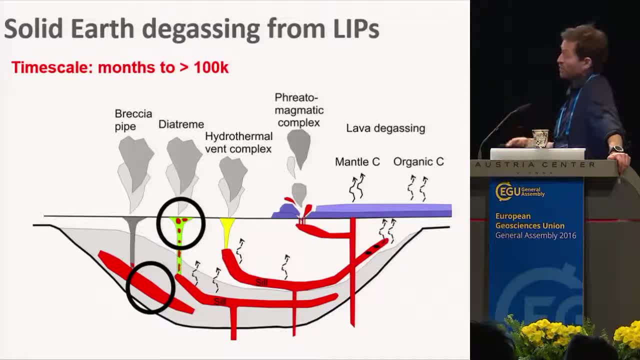 and metamorphic reactions, and degassing from the sills contribute to overpressure, and that overpressure generates gas venting to the pallet surface, forming craters, pipe structures, etc. And this is, of course, in addition to the normal basalt degassing. 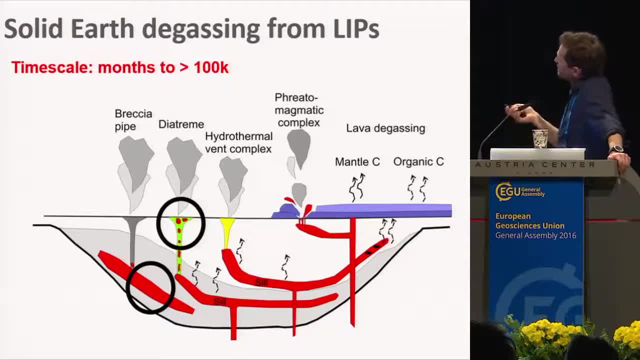 that happens at the surface. So we find pipe structures in sedimentary basins that are related to large-scale provinces' sills. We call them. you know it's pressure pipes, diatremes, hydrothermal vent complexes and also ranging into what we call. 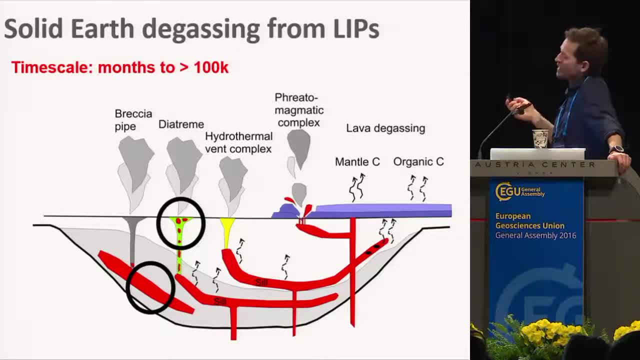 phreatomagmatic complexes where the magma is interacted with shallow groundwater. So this is kind of like a complex picture of what happens when a large-scale province enters the upper crust and sedimentary basins. So my role in this is to try to look at the bigger picture. 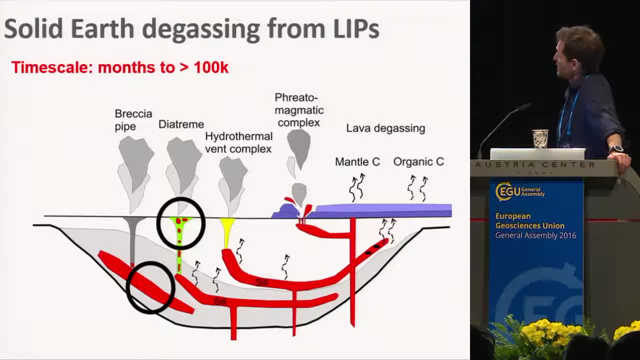 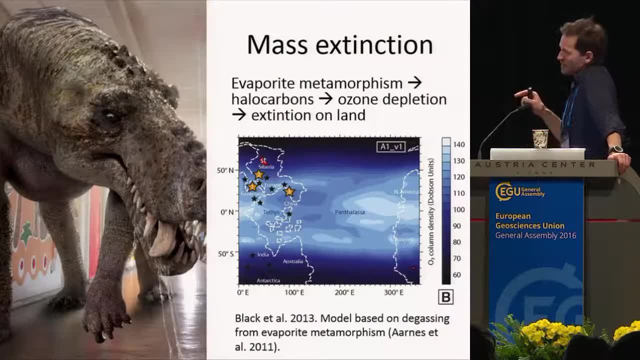 of the volcanic, the sub-volcanic aspects of large-scale province formation. Okay, so when it comes to this, the sub-volcanic part in the Siberian traps- it has been suggested that the sub-volcanic part 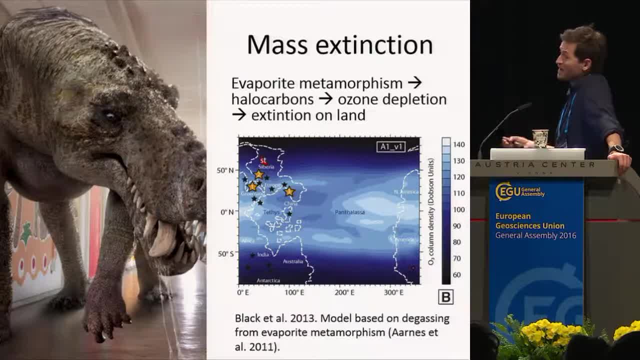 that is, the sills, is directly responsible for the mass extinction at the P-T boundary when it comes to the continental part, the land part of extinction, And the suggested mechanism is that the metamorphism of evaporites, which, of course, are vast reservoirs. 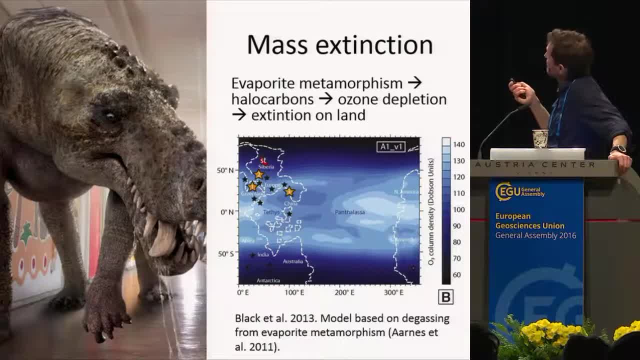 of halogens and sulphur led to the formation of halocarbons, and the ejection of halocarbons into the atmosphere led to ocean depletion and then extinction on land, And this is supported by findings of mutated pollen, of spores, by many researchers. 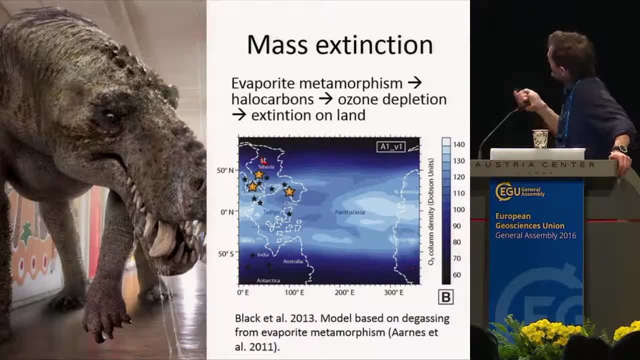 including people here in the audience, And this is summarised on this figure by Black et al from 2013.. Which the modelled output of halocarbons into the atmosphere and looked at the atmospheric chemistry effects of ozone. So what is plotted here is: 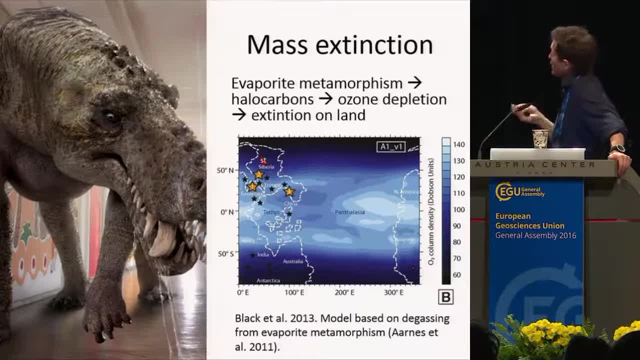 ozone depletion. so the darker colours, the lesser ozone in the atmosphere. And this is then coupled with what is known from the proxy data record, with mutated pollen plotted here as dots, So it's a fairly good agreement with degassing from evaporites, the ozone destruction. 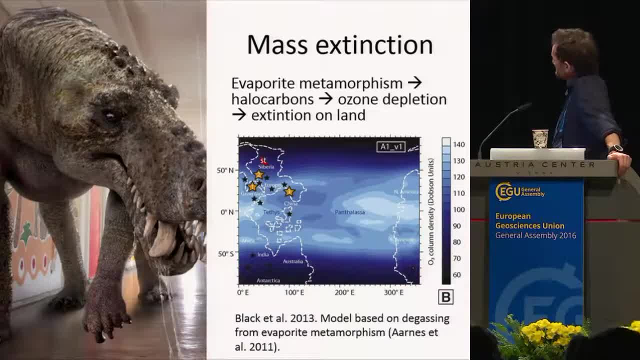 and then mutation of pollen, at the end, permanent. The thing is, when you look at the details of what this model is based upon, that is, the degassing from the basins in Siberia, there's not that much data available and this idea is basically from a paper I wrote. 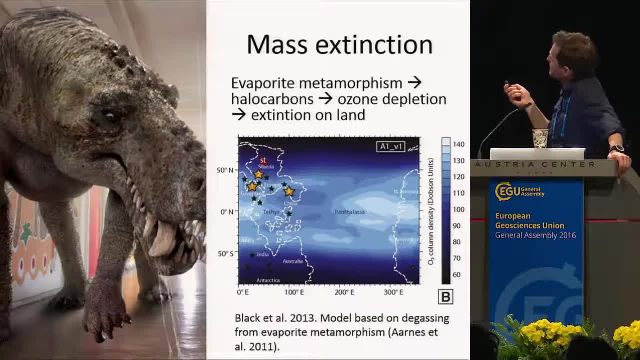 in 2009, where I did experiments with salts from Siberia in the laboratory, heated them up in a GC and then looked at the gases being generated, And it was actually a lot of halocarbons being generated in these experiments, supporting that this, this is a feasible. 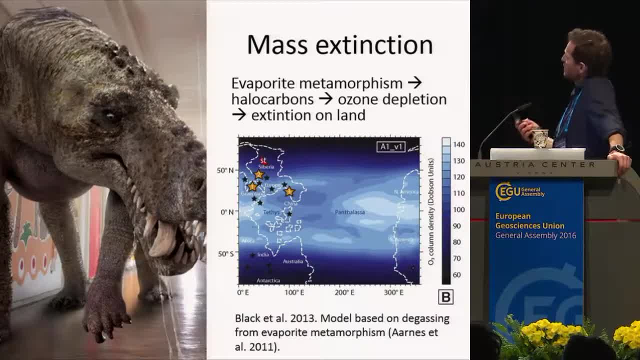 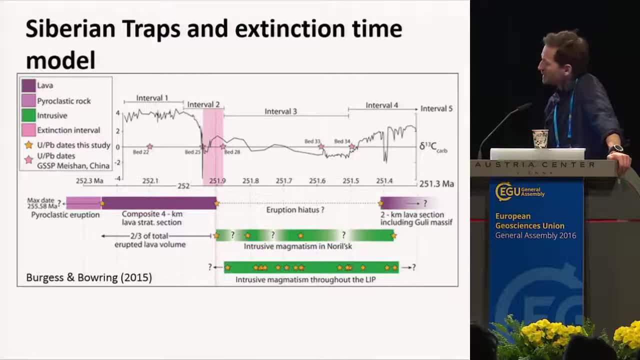 mechanism to explain the continental extinction. But if you look at the data behind that, it's poorly constrained and we need more, let's say, a better understanding of the cells in the basin to be able to really constrain the model. And that's what also part of this presentation will. 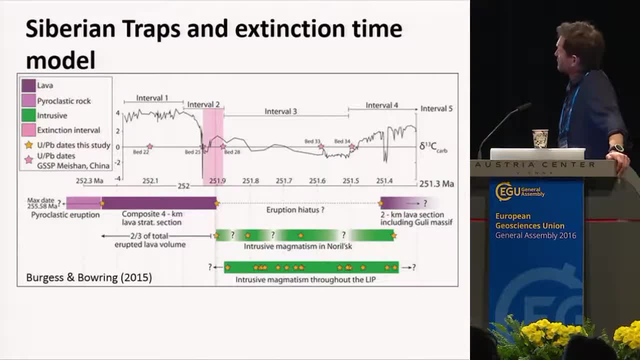 go into. We can zoom in a little bit on the Siberian traps and the formation of the Siberian traps and how it links to the extinction models suggested. So this is a time model of the Siberian traps and how it developed together with the carbonized stoves. 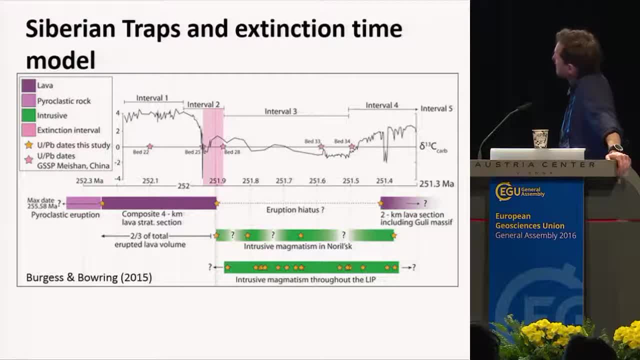 from the same time and the time model is from Burgess and Bowring last year. So what we see is that in Siberia, the explosive organism from the basalt started about 252.3 million years ago and then, shortly after, shallow sills in place in the sedimentary. 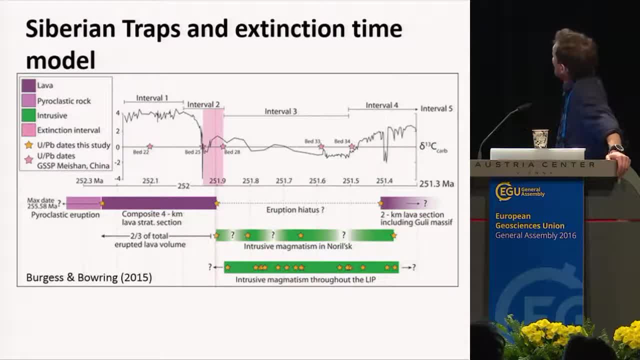 strata lasted until 251.4 roughly ma, And this corresponds fairly well to both the extinction intervals. This is the main extinction interval and then the carbonized top anomalies And as we see here, it's a near perfect agreement between the carbonized top. 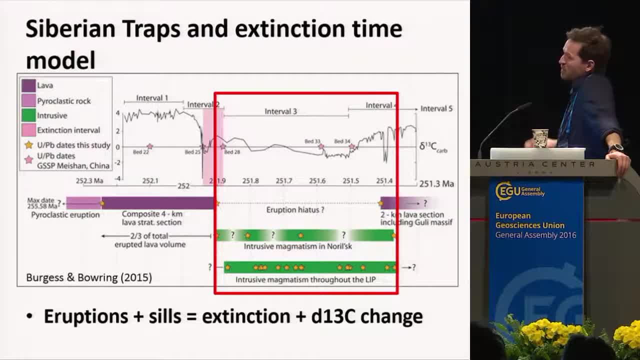 excursion at the PD boundary and then the intrusive magnetism with the sills etc in the basins in East Siberia. So this supports the idea that the eruptions, the early eruptions and the sills contributed to the extinction and also the carbonized top anomalies. 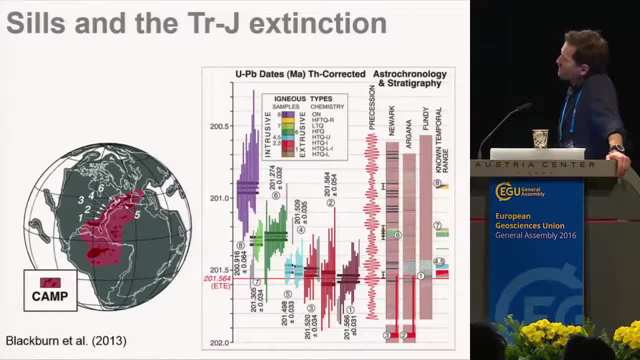 seen in the proxy data record. The same pattern is also probably present for the Triassic-Jurassic extinction. So this is data from Blackburn et al just a few years ago. So what we see in this diagram is a reconstruction of the Central Atlantic Mammatic. 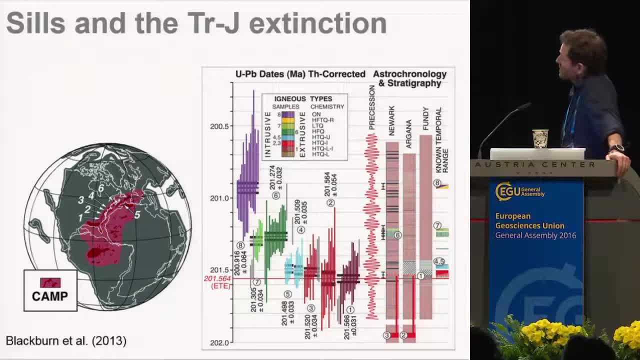 Province. It formed 201.5 million years ago And it's the main explanation for the Triassic-Jurassic extinction that we heard also one of the previous speakers talk about. So the message from this study is that certain ages from sills from various 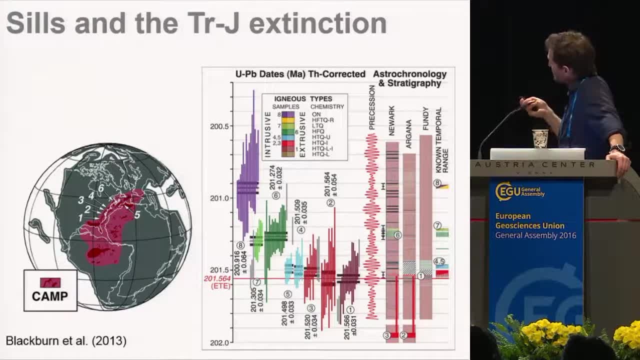 places in this province correspond nearly perfectly with the extinction interval at the Triassic-Jurassic boundary, Also stressing the importance of this sub-volcanic part of the large English province. So the sills, the metamorphism and the pipe degassing. 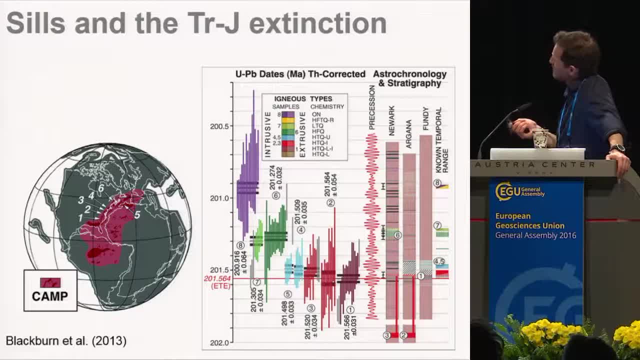 But still, these aspects of the Camp Vulcanism and the Triassic-Jurassic are not really fully explored. But we have some new results, also from studies, for instance in Brazil. so I encourage you to come to the session that we have after lunch, where some of these 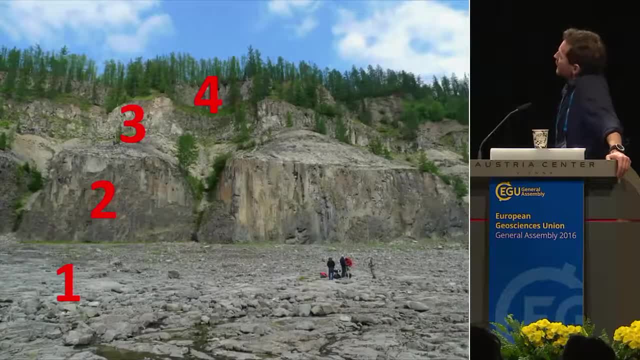 details will be presented. So I've been talking about sills, the sub-volcanic plumbing system of large English provinces. So what do these rocks actually look like? So this is an example along one of the major rivers in East Siberia. 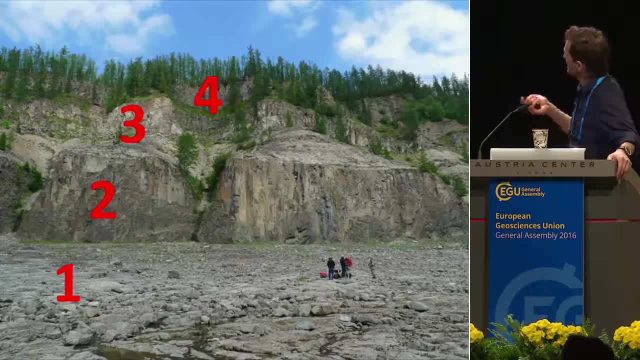 We went there last time in 2010 and what we see here is a stack of sills. It's a thick one here, A sill here, a third up here and a fourth on top And in between the sedimentary rocks and the black. 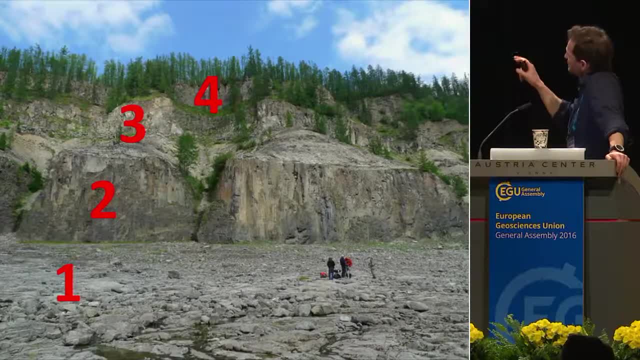 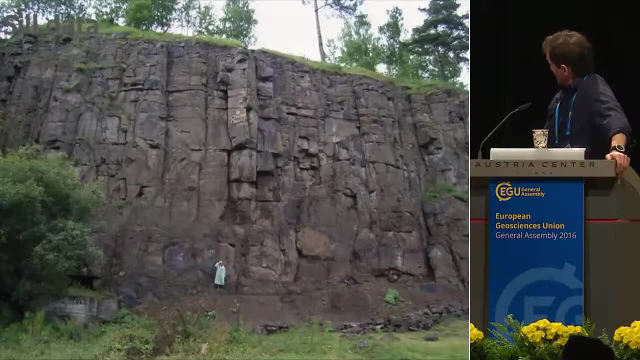 layers are coal and metamorphic coals, So this is a fairly typical scenario. It's a huge stack of sills. We find them everywhere. This is a different location. This is the so-called Brodsk Sill in the southern part of the province. 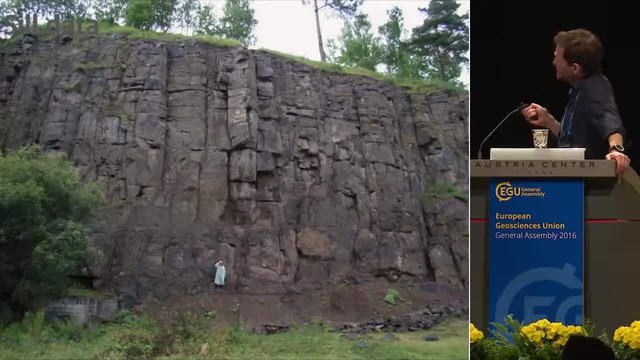 This is my colleague, Sverre Planke, for scale, And this sill is vast. It's really thick. It's about 200 meters thick And it's the age it has been dated and it's part of the Burgess and Bowring paper. 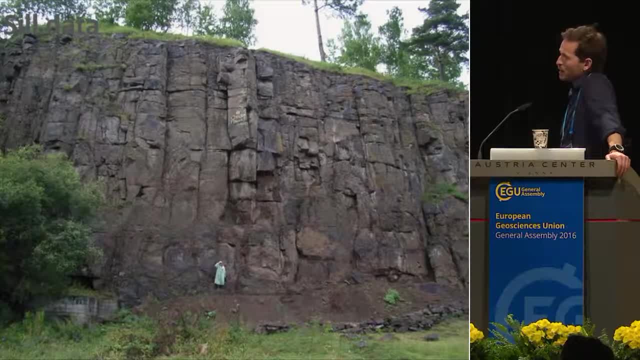 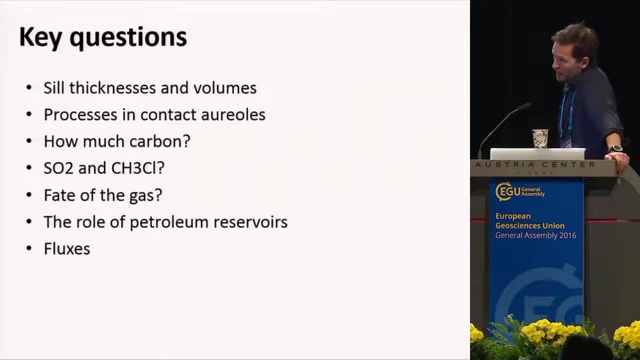 As I mentioned earlier, it was in place and formed at the same time as the carbonized excursion at the P-T boundary. So this is what the sills typically look like in the field. Some of the key questions which I think are remaining in order to 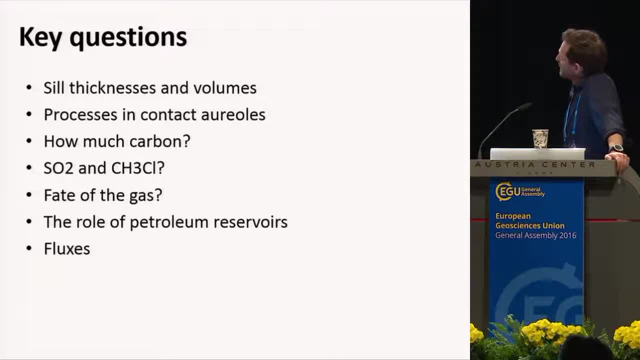 understand the link between the Siberian traps and permanent extinction is the actual sill thicknesses and volumes that we find in the basins, Because if you look at the literature available, there's actually not that much data around The Russians they have drilled. 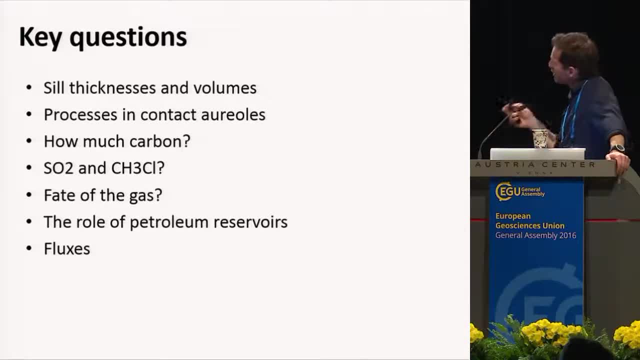 everything. They have seismic data etc. They have a course, but it's so difficult to get material from them, So we don't really know that much about sill thicknesses and volumes, And this is really crucial if we want to understand the metamorphic effects on the basins. 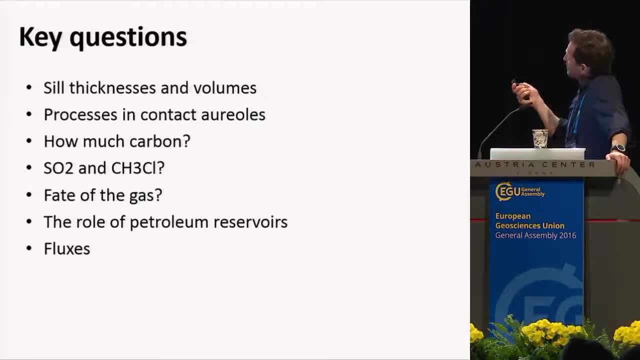 We also need to understand better the processes in the contact orals, especially when it comes to the carbon budget and how much carbon was formed and how much carbon was degassed. We need to understand how much SO2 and halo carbons also were emitted, and this 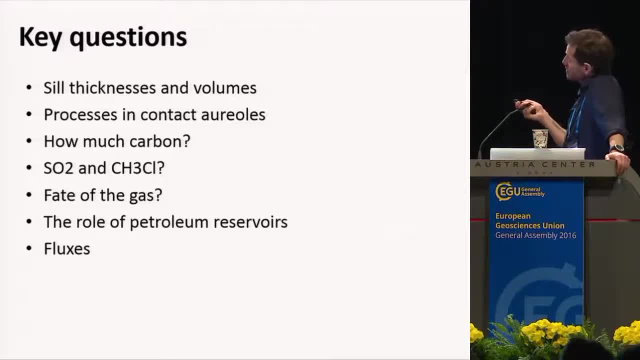 is a major uncertainty Because, also, as I mentioned earlier, in particular with the SO2, there's not really anything in the proxy data that can tell us anything about the SO2.. The fate of the generated metamorphic gas is, of course, a major issue, Did it? 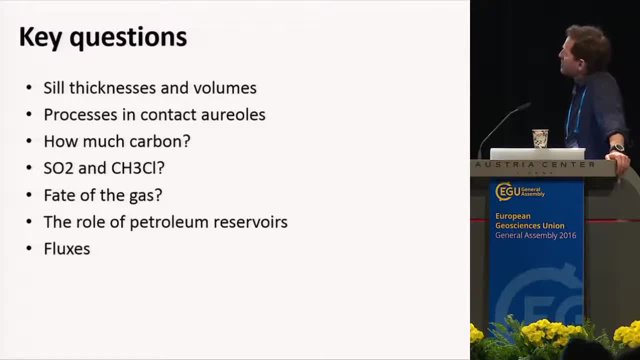 get stuck in the subsurface, or did everything get vented to the paleoatmosphere? I'm also really concerned about the role of the petroleum reservoirs, because in East Siberia we know that the petroleum system was active during the Permian and that the sills 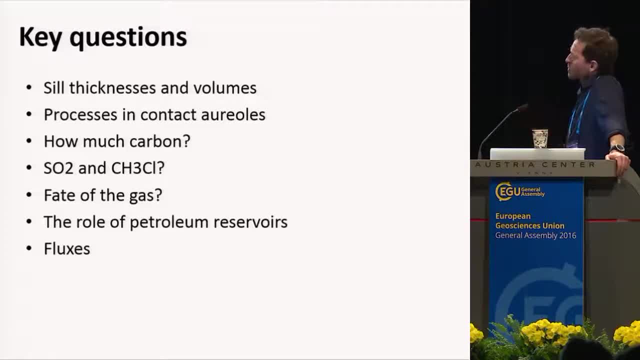 also affected petroleum reservoirs, And this part is really hard to quantify because the petroleum is, of course, localised in particular areas and it's hard to understand the big picture when it comes to how the sills affected petroleum reservoirs. And, of course, finally, if you want to understand, 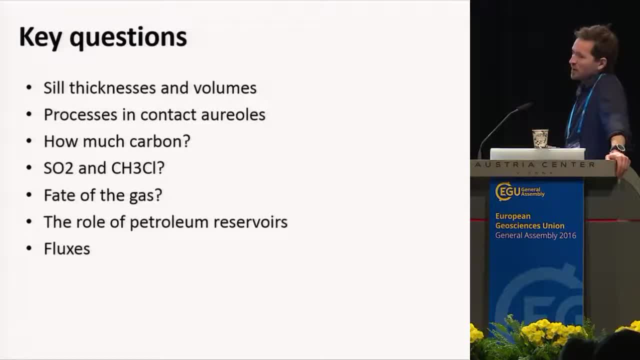 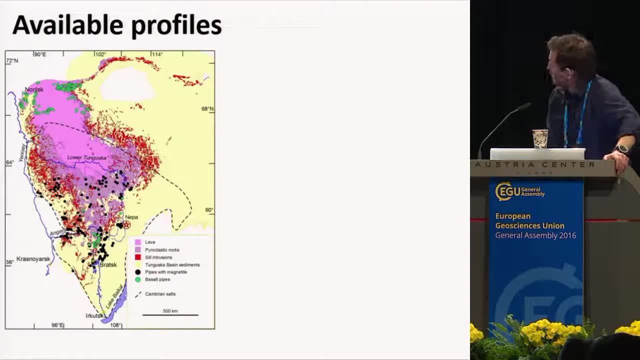 the paleoclimate and the extinction. we need to have fluxes that can also be used in Earth's system models. I want to show you a little bit about the geology of East Siberia. So again, we have the sills in red and we have 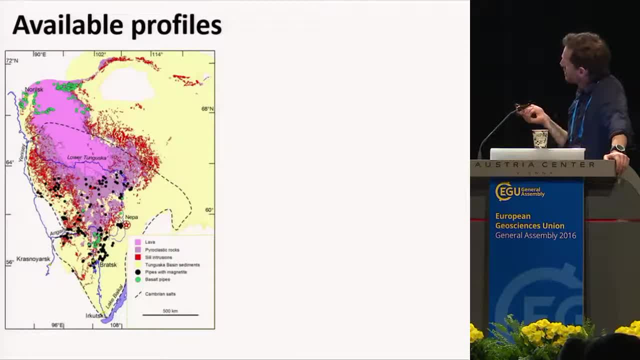 the lavas in purple colours and also the pyroclastic deposits. The black dots are pipe structures. They are degassing structures up to a kilometre in diameter and I think this is one of the links to understand the relationship between the Siberian traps and 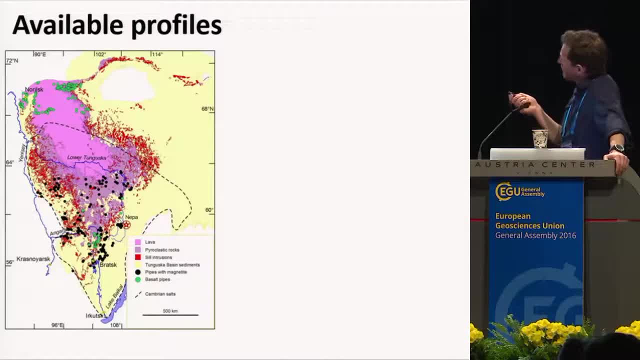 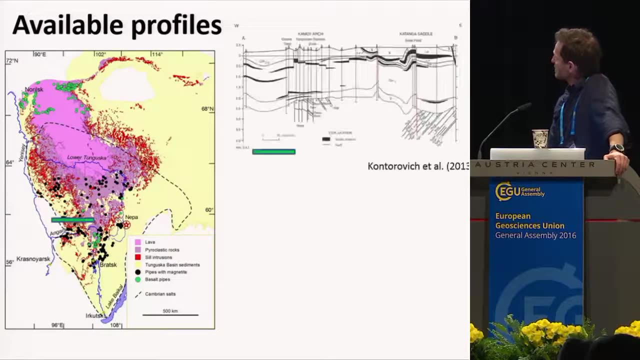 the Permian crisis, Because we have all the sills, we have the gases generated in the contact orioles and then we have the degassing pathways that we can actually study in the field and we can say something about them When it comes to the sills in the surface. 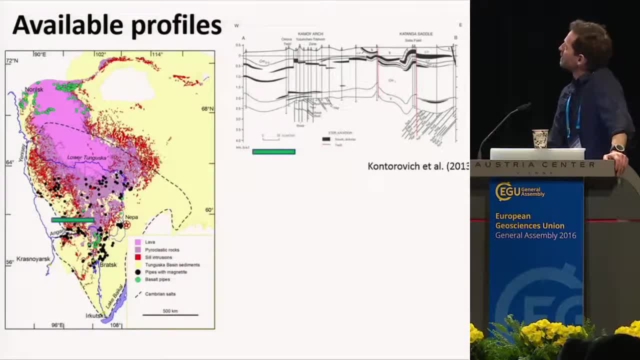 we have the outcrops, but the outcrops are not that great, mainly along the rivers. But we do have some seismic profiles and some borehole profiles, For instance this one from Kontorovich showing the sills in black. 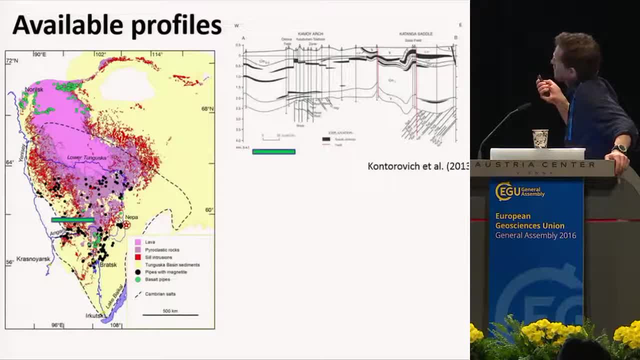 and the symbols. here the Cs represent evaporite deposits, So it's a vast reservoir of evaporites up to two kilometres in thickness, and the sills are then placed into these evaporites. We can move on to a different profile a little bit further south. 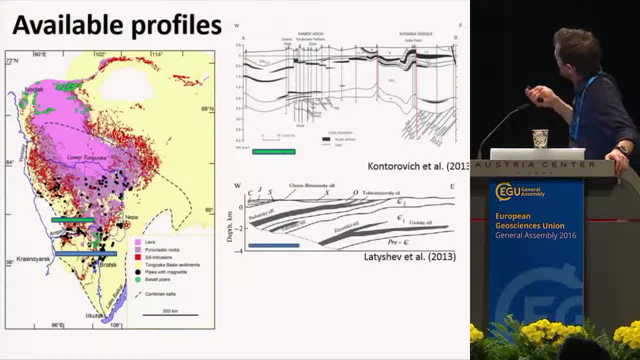 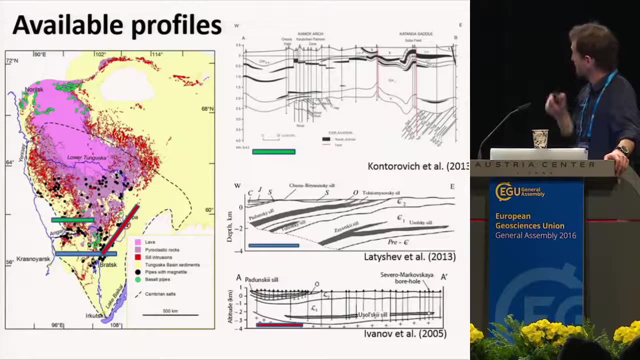 and we have the same story. We have the evaporites and we have the sills and a third profile in a slightly different direction. Again, we have sills and we have thick deposits of evaporites. So the question is: 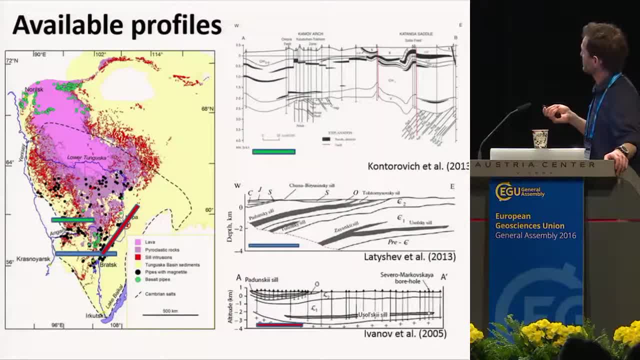 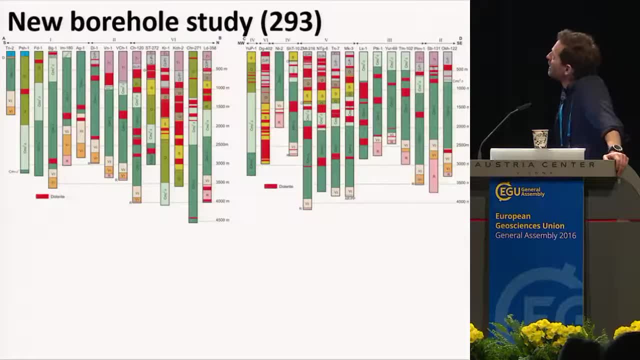 is it possible to get samples from some of these systems? Is it possible to get sill data and also to get the contact oriole data from boreholes, And this is a work in progress. I have some colleagues at the Moscow State University. 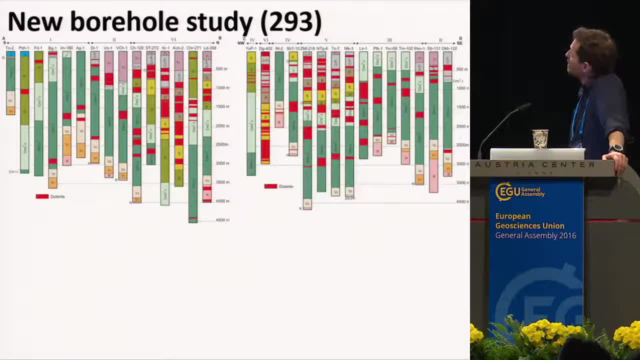 and they have access to a petroleum industry borehole and we have access to this database. At the moment we're looking at almost 300 boreholes to get better statistics of sills, their thicknesses and distribution within the sediments. 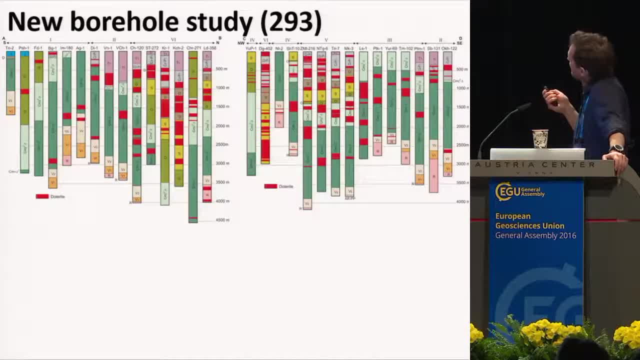 And this is simply a stack of some of the boreholes. So what you can see in green colours is the evaporites and in red is all the sills. So, basically, the sills are everywhere, Probably representing a volume greater than the lava volume in the Siberian Traps. 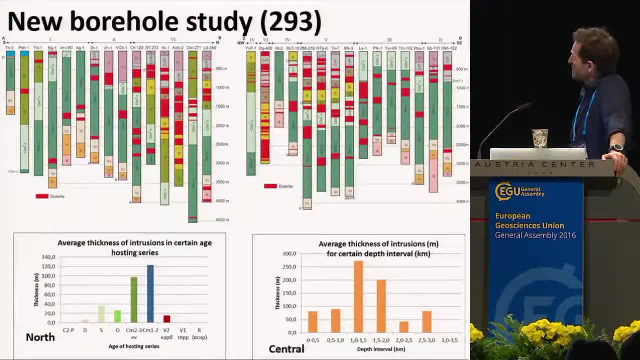 We also have done statistics on this and looked at where the sills are thickest and so on, and the message here is that when you look at thicknesses of individual sills versus the sediments where they are emplaced in, we have the seas. 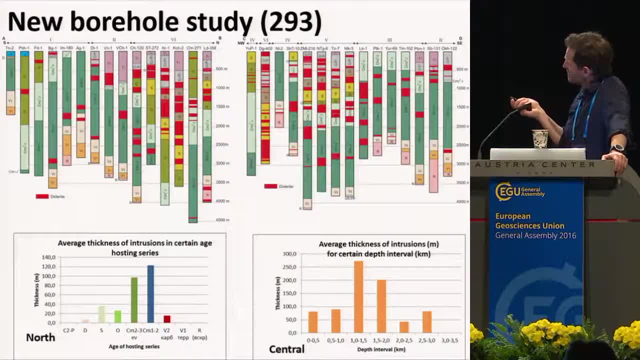 again, which is the evaporites, and this is also where we have the thickest sills. Thicknesses in some places in the north, up to 120 metres thick, and then other places more central in the basin, also in the same evaporite intervals. 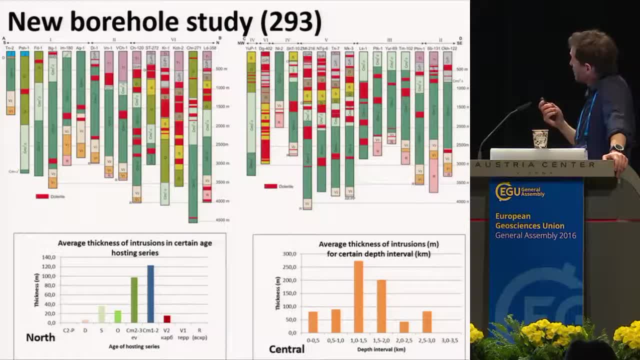 we have sills more than 250 metres thick, And what we also know from studies of contact metamorphism is that if we have a sill of 250 metres thickness, there is a contact aureole above and below of roughly the same thickness, So a sill of 250 metres. 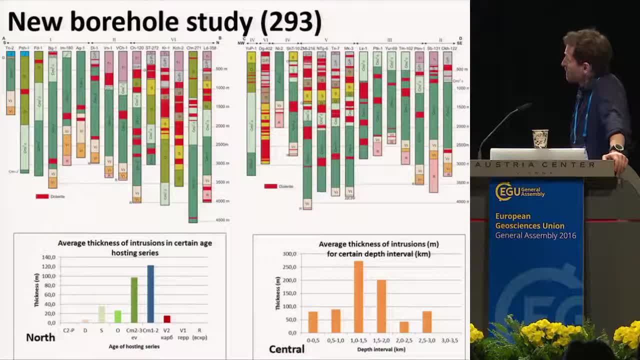 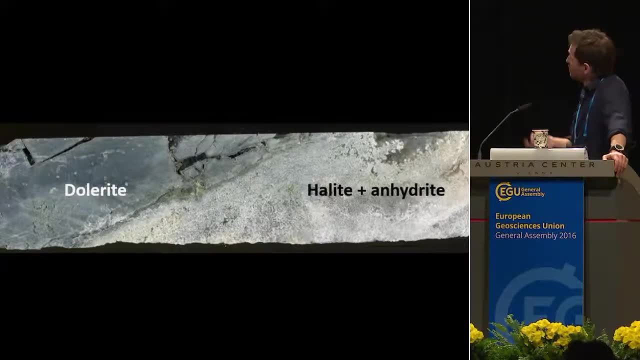 can be associated with 500 metres of metamorphic sediments. And we look at the scale of the basins in East Siberia, the volume of metamorphic rocks becomes really big. This is one of the cores that we have gotten from boreholes, and just to show you what. 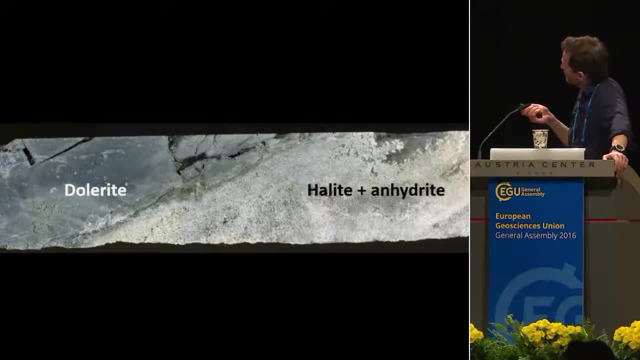 these sills look like- and the evaporites. what we see here is the direct contact between a sill- the thickness of this particular one is about 200 metres- and then we have halite here and anhydrite, which is all the white stuff. 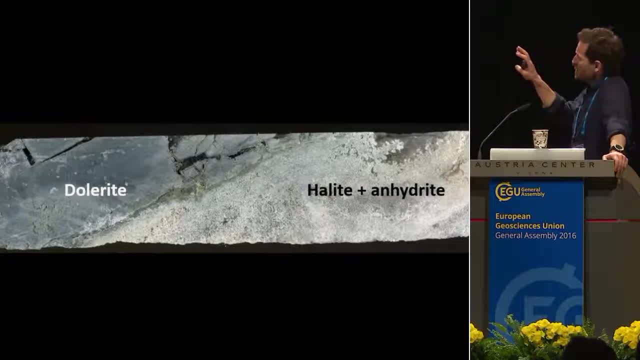 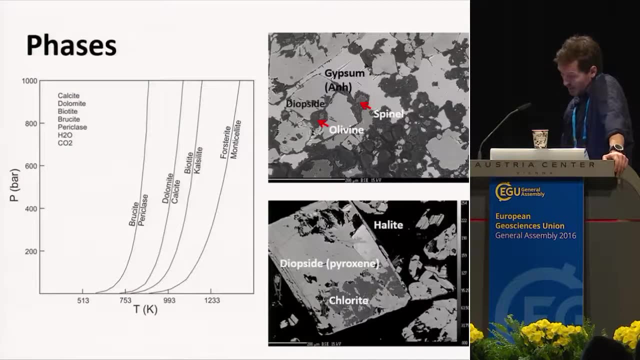 And then we have veins with halite going into the dolomite. So this is a fairly typical picture of what we see when we look at the rocks in Siberia. And then, of course, we can look at the minerals, the phases, we can look at phase diagrams. 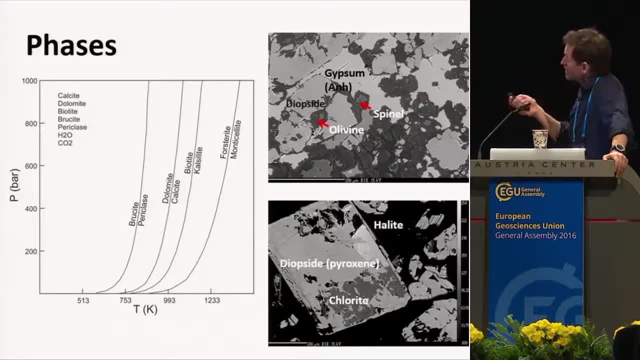 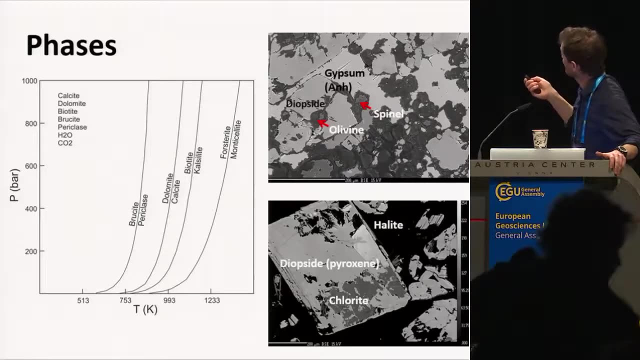 for instance, when you heat a dolostone or a sediment rich in carbonate and, let's say, evaporite minerals, we have prograde phase reactions, we have bruiser that breaks down to periclase, dolomite, calcite, etc. Then we can look at what we find in the field. 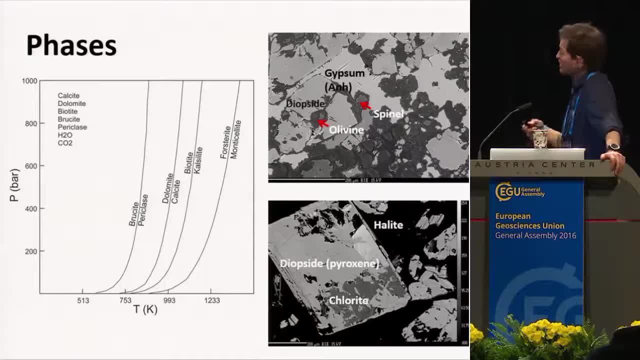 and then compare with phase diagrams to constrain the temperature history and also the devolosalisation history. These microprobe pictures are simply examples to show you. in the upper part, phase assemblages saturated with sulphate, with gypsum anhydrite. 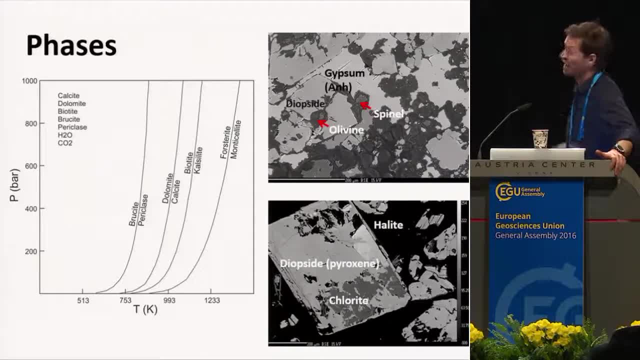 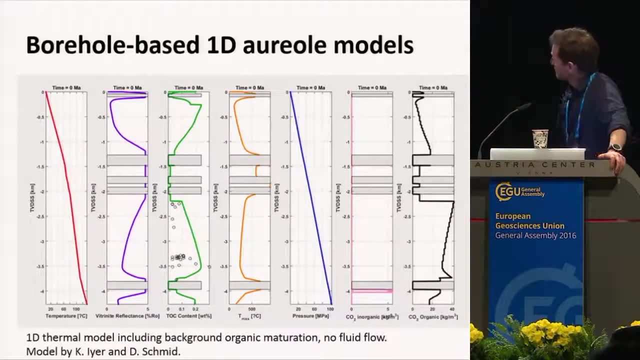 and, in the lower part phase, assemblages saturated with halite, So it's basically pyroxenes growing in halite. Okay, so what we're doing at the moment- and this is work in progress- is to use some of the data. 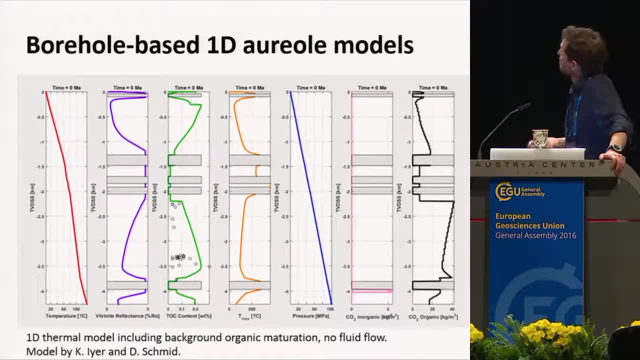 from the boreholes and to constrain the metamorphic evolution by 1D thermal oral models, And this is just one example that we have the lithologies in the borehole, We have all the cells in this particular borehole. it's one, two, three, four. 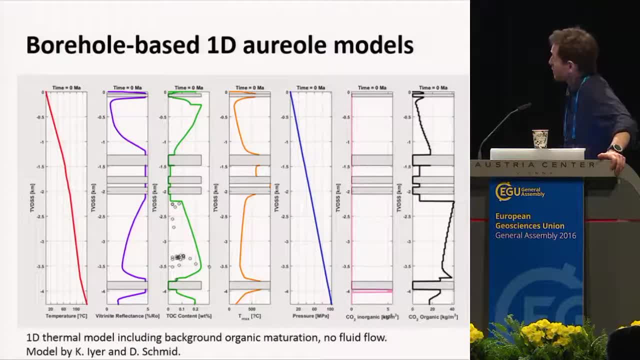 five thick cells going down to about four kilometres. So it's really really deep boreholes And what we're doing with this is to use the total organic carbon contents of the sediments and then we can also calculate in green here the theoretical. 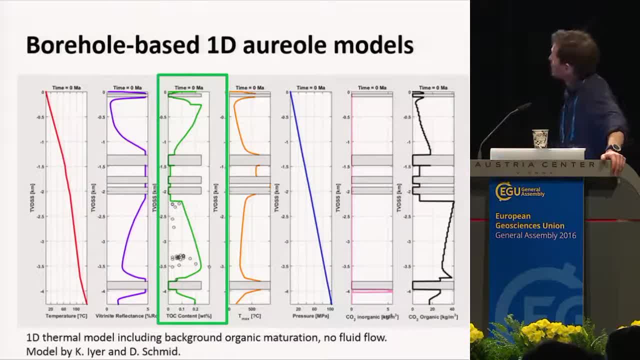 organic carbon content, And then we can quantify how much organic carbon was lost and transferred to gas by using the easy row model that we can put into this. On the right hand side, again, we get quantified the amount of CO2 produced from organic reactions, but also 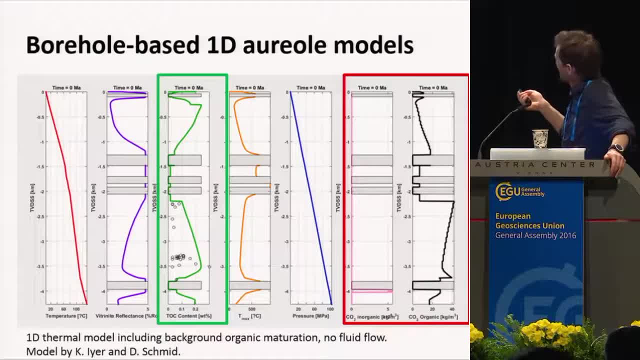 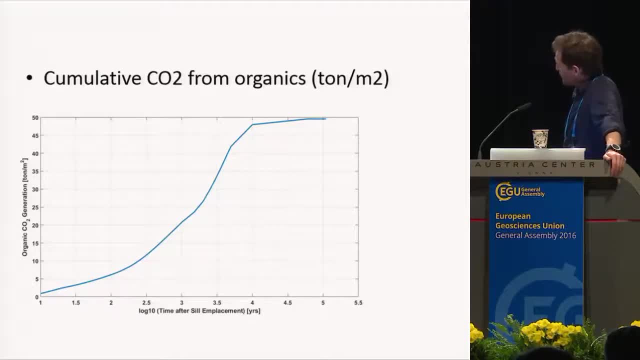 from carbonate breakdown, So we can both look at the inorganic and organic phases. This is just one example of output from the model. in this case it's organic CO2 production, cumulative versus time, And then this is work in progress, as I mentioned. 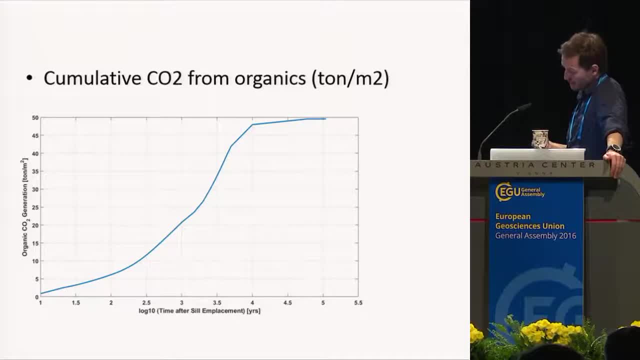 so the idea is to use this on a wider scale and then to quantify the gas production based on the specific case calibrations. One important thing is that, when it comes to the production of CO2, the organic phases are much more important compared to the carbonates. 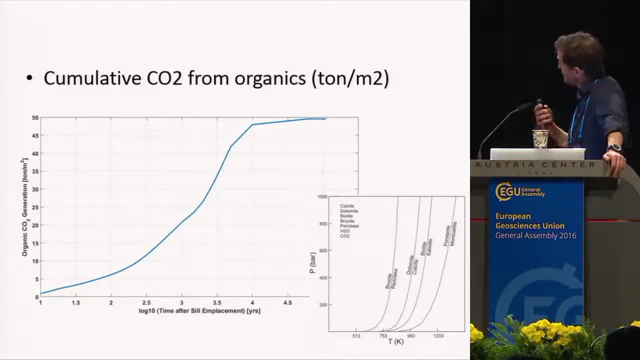 That's because if you want to de-volatilise carbonates, you need temperatures roughly above 400 degrees, and that only takes place in a narrow zone close to sills, whereas the organic content is much more sensitive to temperature, so you can generate. 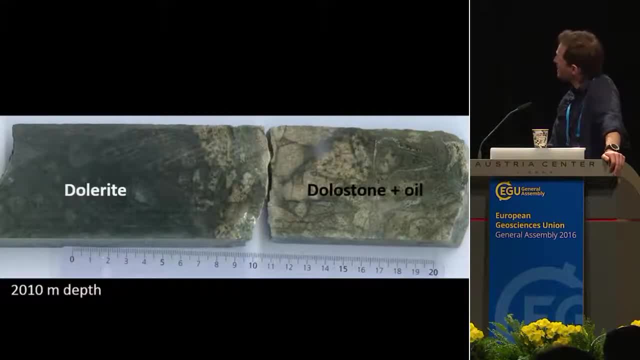 more CO2 from the organic stages. I mentioned earlier the role of petroleum reservoirs. This is one case where a thick sill has inclusions of dollar stones, which is sedimentary rock saturated with oil. So it's definite that we have examples where there is interaction. 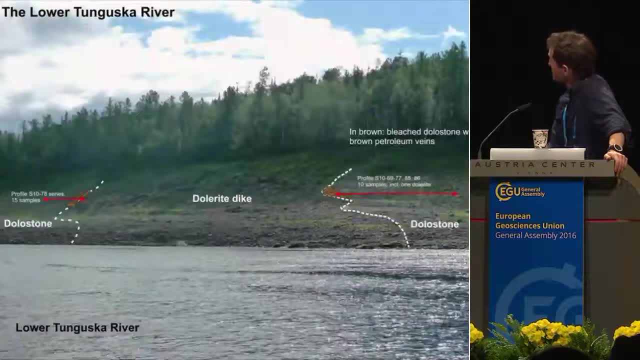 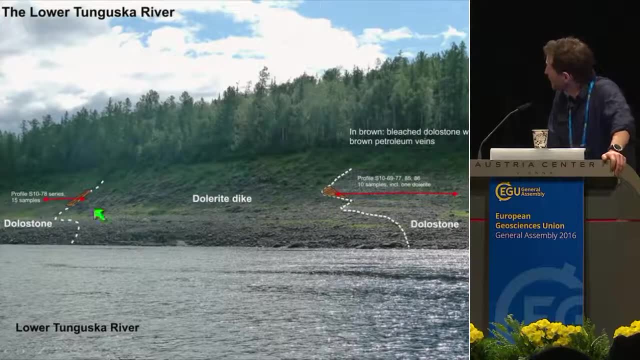 between dollarite or the sills and petroleum reservoirs. We also find this in the field. In this case it's a fairly wide dike that we find along one of the rivers. We have sediments next to the dike. it's dollar stone. 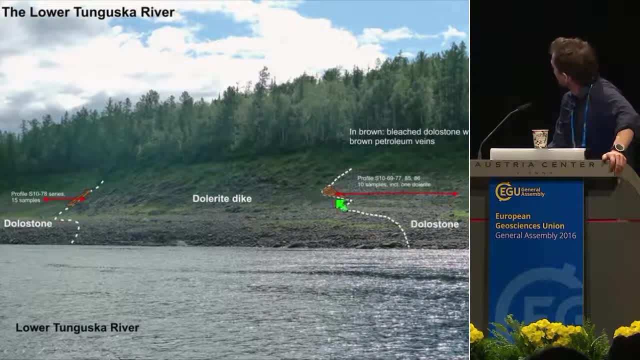 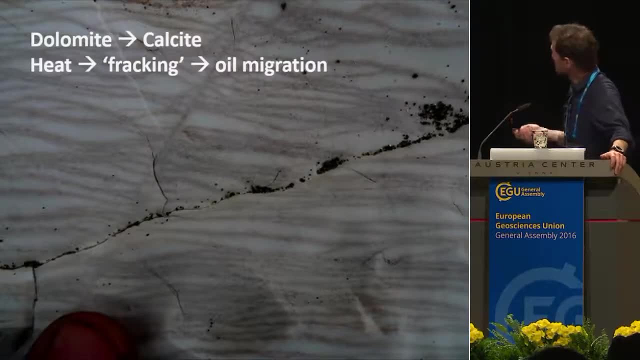 and then you can see the margin of the dike And you can zoom in on this particular brown spot along the overcrop, and what we see here is a metamorphic rock. It's now consisting of calcite, and then all the brown veins. 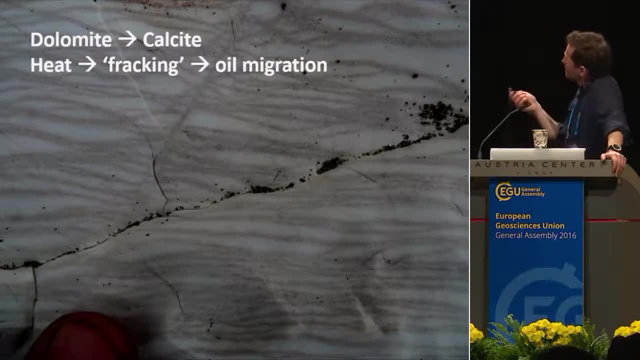 are oil veins. So it's a system where there's a lot of heat providing, heating the sediments and then kind of like a natural fracking system, and then oil is moving into these hot oils and also being devolatilized. 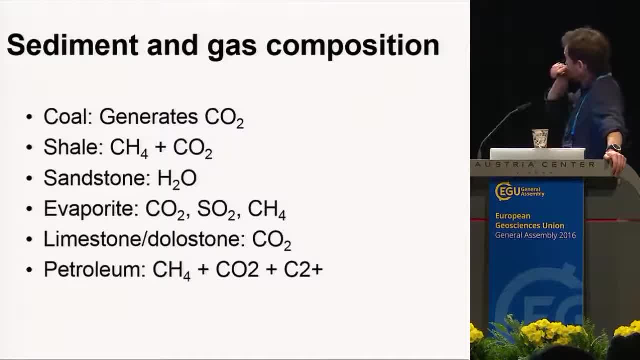 To summarize some of the effects on the sediments: if there's coal in the basin, which is the case in the sub-area also, we get CO2, we get methane CO2 from shale. if you have sandstones or plastic deposits with clays, 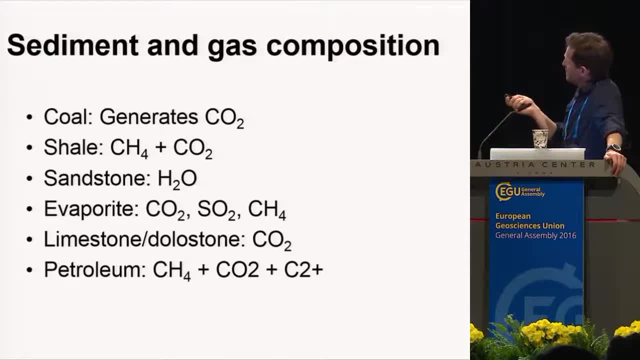 and so on. it's mainly water being released, Evaporates, there's a range of gases- CO2,, SO2, and methane- and then we have the limestones generating CO2, and, in case of petroleum system being heated, we have methane, CO2,. 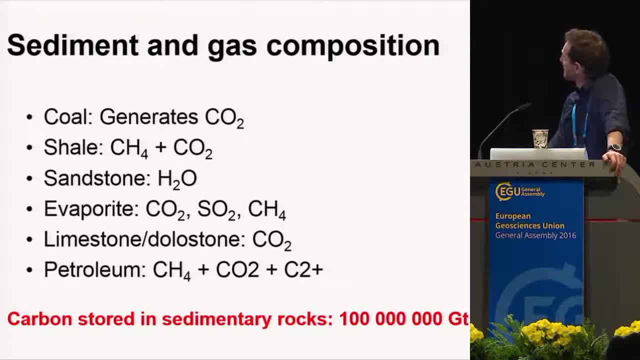 but also maybe higher hydrocarbons. I'd like to- I'm getting towards the end here, but I'd like to also stress that- why we think this is important on a global scale, and that's: if you look at the carbon budget on Earth, it's actually 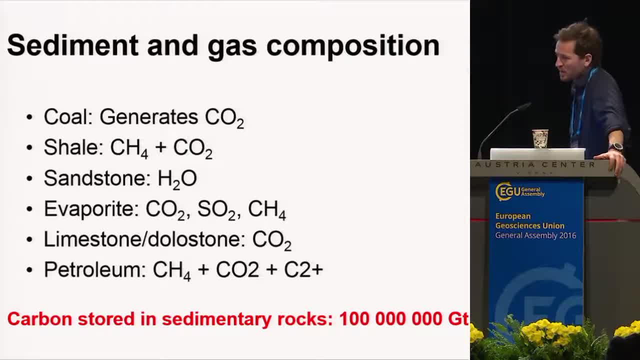 maybe as much as 100 million gigatons carbon stored in sedimentary rocks, and that's a vast reservoir. So what I'm suggesting here is that the sills and the pipes is a fairly rapid and efficient way of transferring some of the carbon stored in sediments. 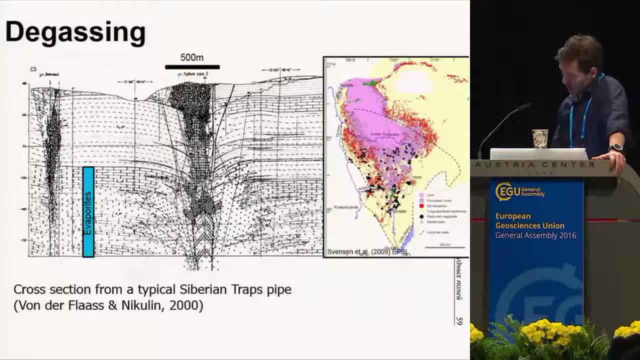 directly into the atmosphere. The degassing pathways are pipe structures. I mentioned earlier all the black symbols on the map which are pipe structures and they look like this. This is from a compilation some years back from Russian workers, where you see huge pipe structures. 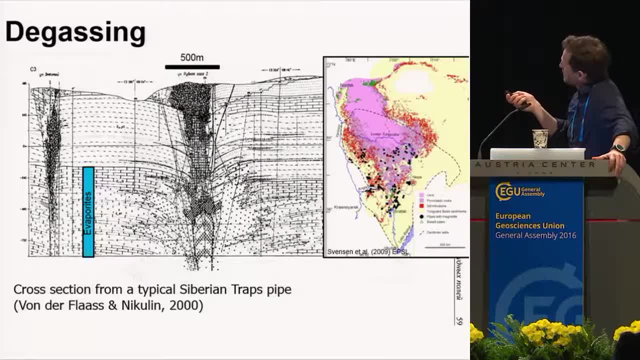 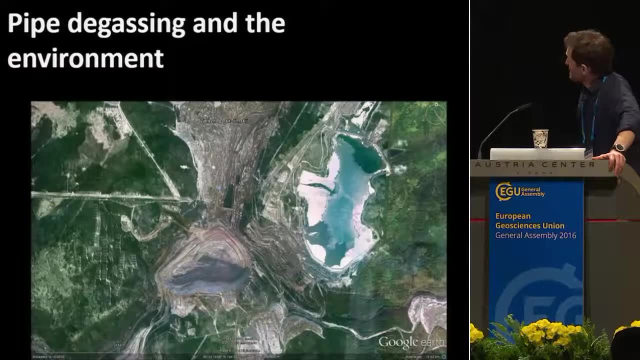 rooted in kind of like mini magma chambers within evaporites in the basins, So these probably acted as efficient degassing pathways and also probably really explosive, delivering the volatile loads into the stratosphere. Some of these structures are currently mined, like 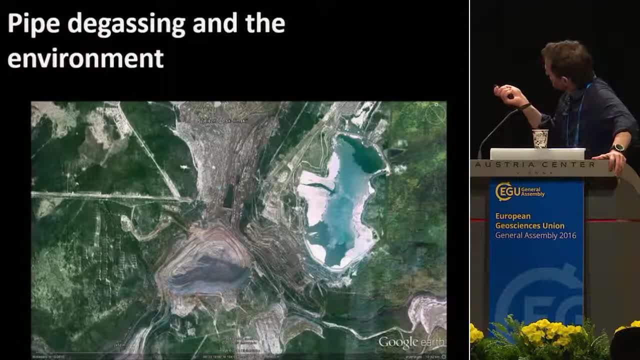 in this case, what is in the middle of this open pit is one of the circular structures, and they're mined for magnetite, which also stresses the link between a large-scale fluid flow in the basins, petroleum reservoirs and also the 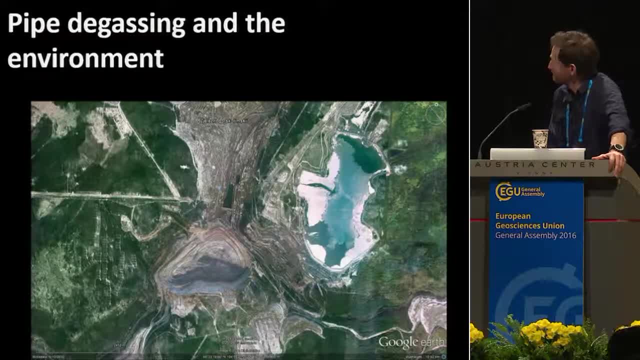 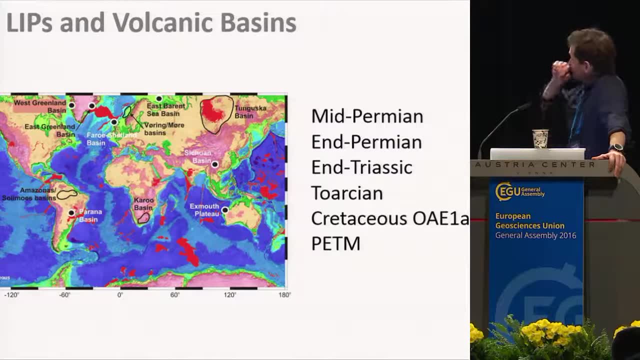 mobilisation of metals by the brines derived from the evaporites. This is one of the last slides. I've been talking about LIBS and volcanic basins and the Siberia case in the Teguska Basin. I would like to stress that. 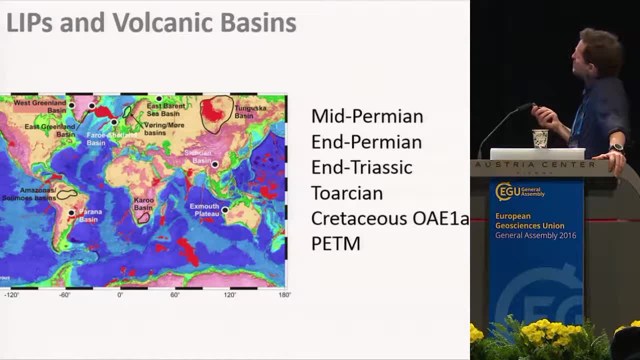 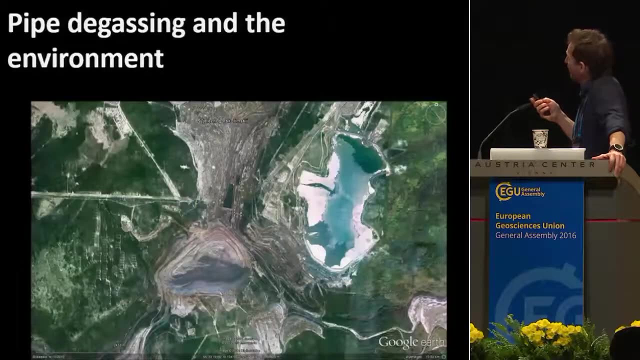 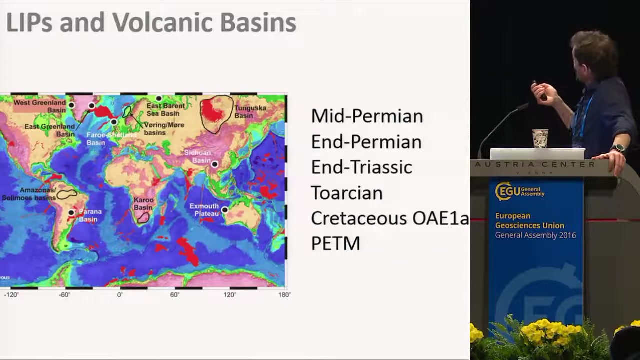 this is not the only case where this type of SILS degassing system works. It has been applied to understand the mid-Permian extinction by SILS in the Shishuan Basin by colleagues in Grenoble. Something happened Then. Permian yes. 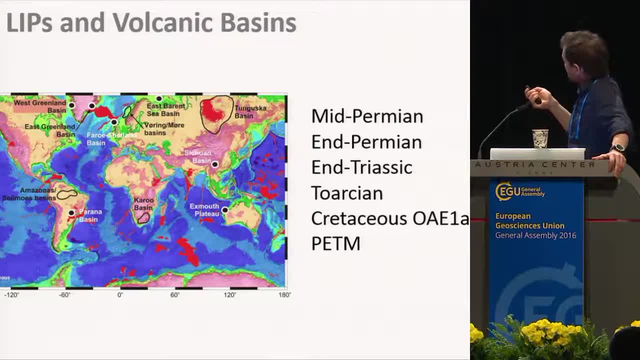 We mentioned the end of the Jurassic with the basins in Brazil. We have also used it to understand the Tuarsen event in the early Jurassic by the Karoo Basin and the SILS there. We are applying it to the Cretaceous Oceanic. 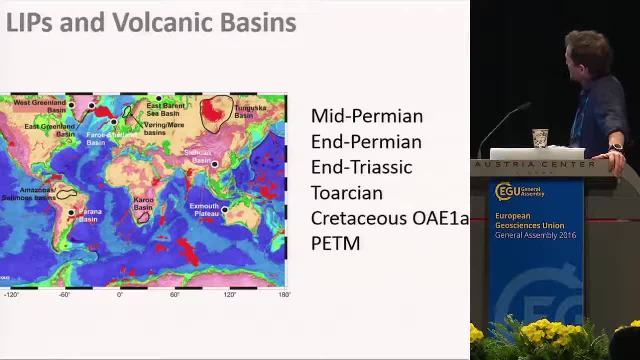 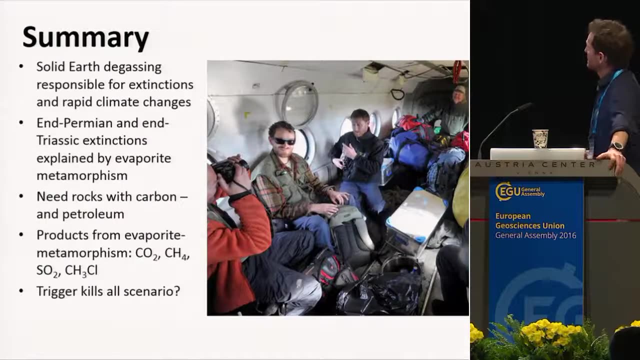 Anoxic event by the High Arctic Large Ignorance Province formed at the same time. and lastly, the Pallasian-Easian Thermal Maximum activity in the North-East Atlantic Volcanic Province. Okay, I summarize by saying that likely that solid earth degassing is responsible. 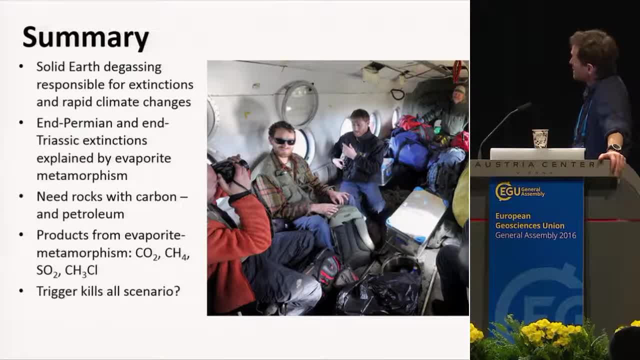 for both extinctions and also rapid climatic changes. I would like to stress that the end-Permian and the end-Triassic extinctions might be explained by evaporite metamorphism, because these are the two biggest extinctions and the only basins. 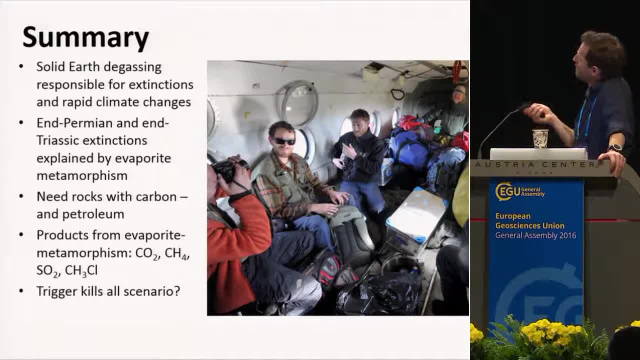 affected by SILS, which are rich in evaporites. We need rocks with really high carbon contents and maybe also petroleum contents, to explain the carbonized excursions that we see in the proxy data records. The products of evaporite metamorphism, including the 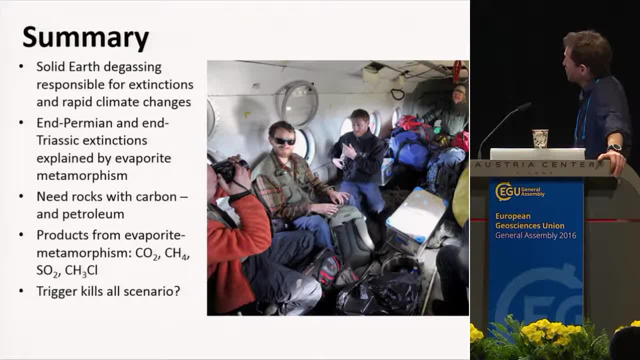 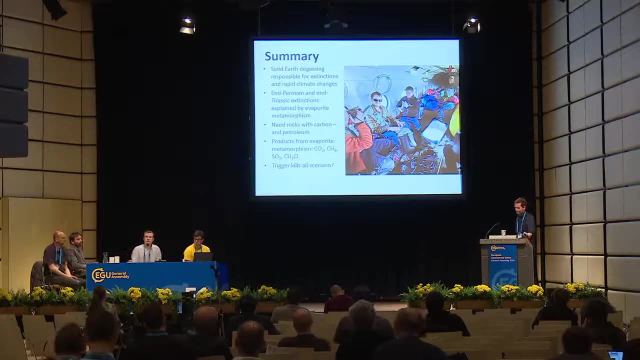 halocarbons might explain the proxy data records at the end-Permian with the breakdown of the ozone layer and then the mutated pollen. Thank you, Thanks very much. We're running late for the coffee break, so maybe just one quick question. 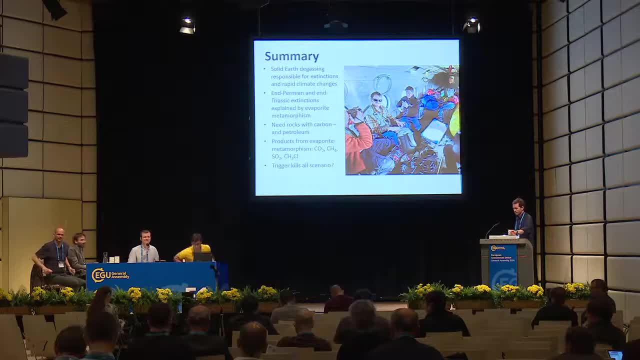 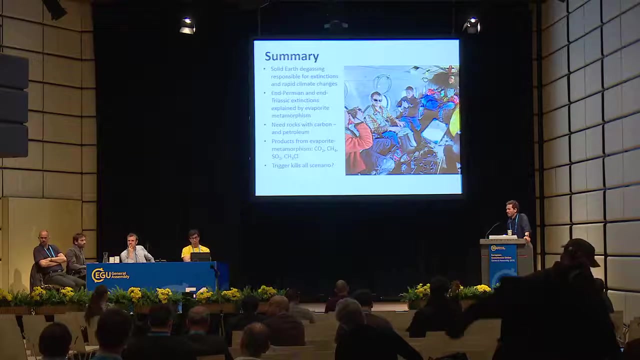 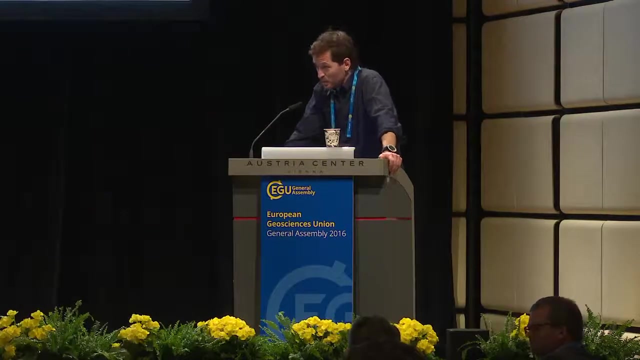 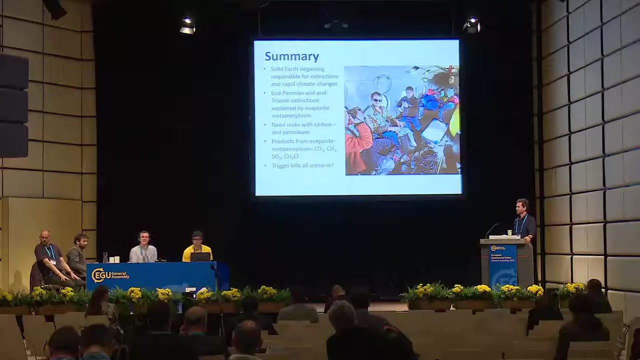 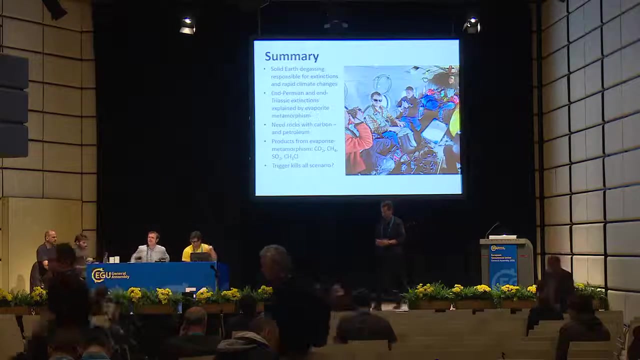 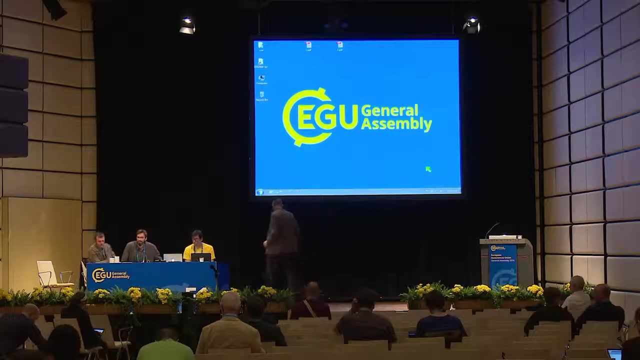 or coffee break Up to you. 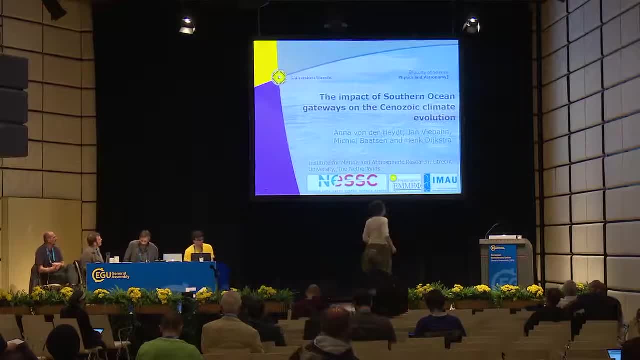 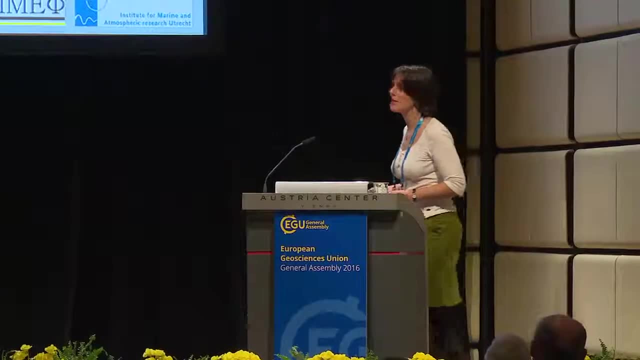 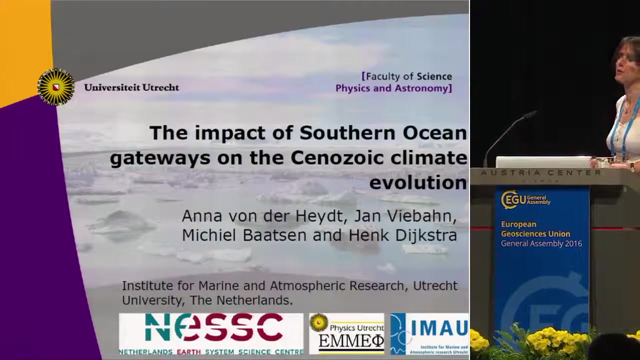 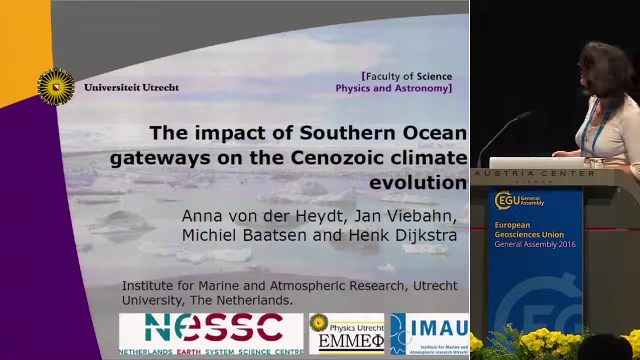 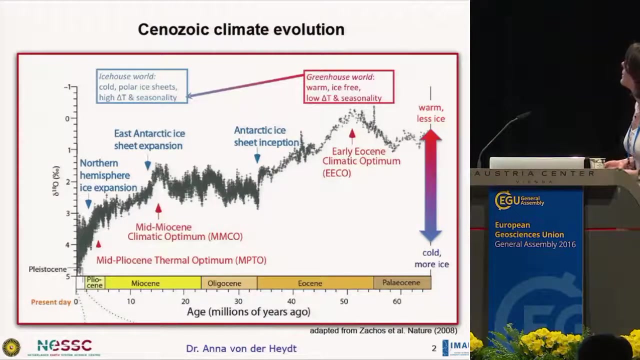 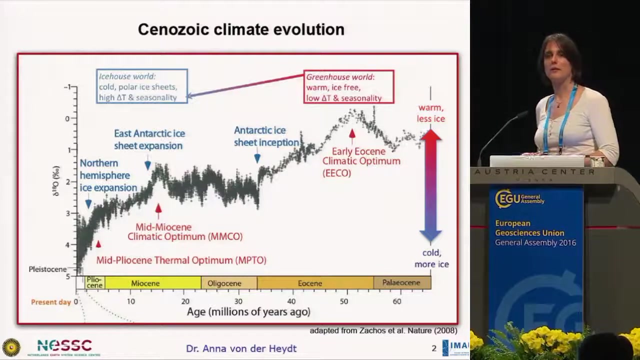 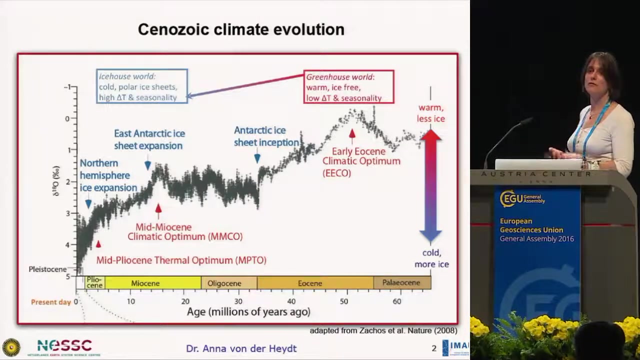 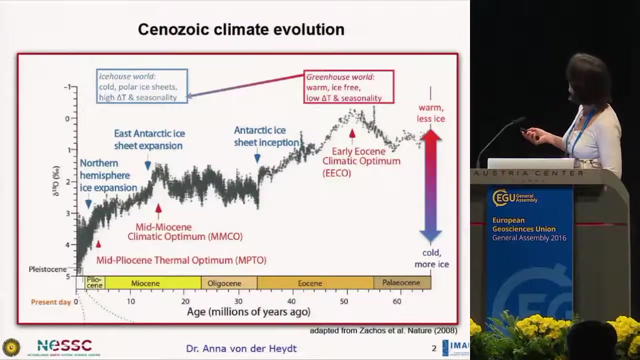 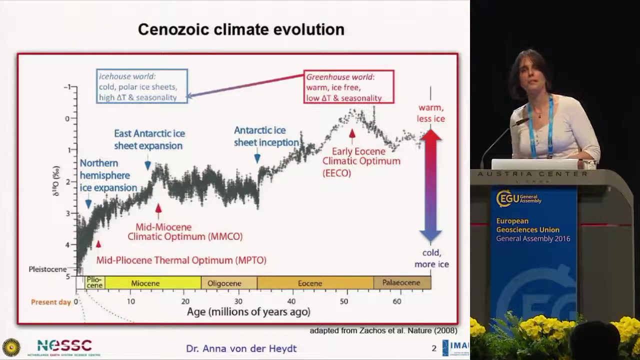 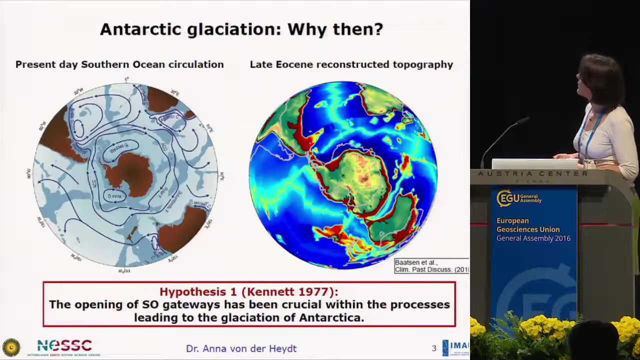 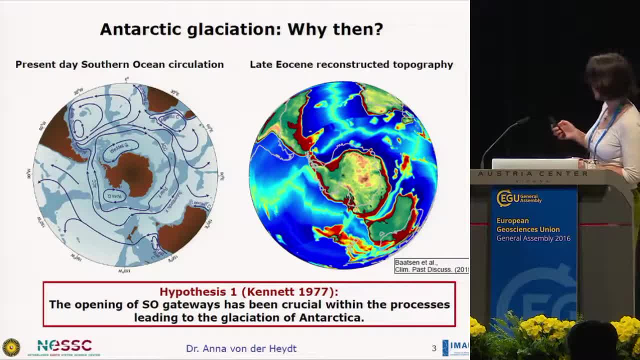 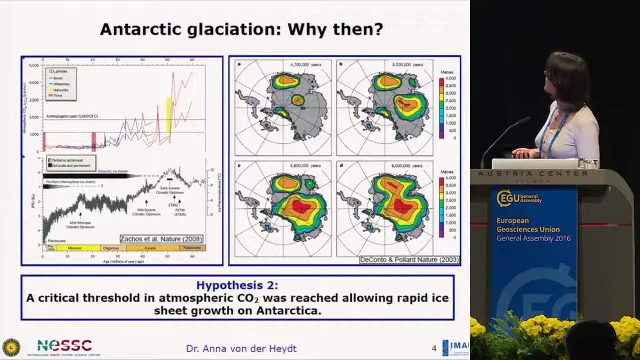 And when you look at the CO2 record here, well, it is going down over the xenozoic. 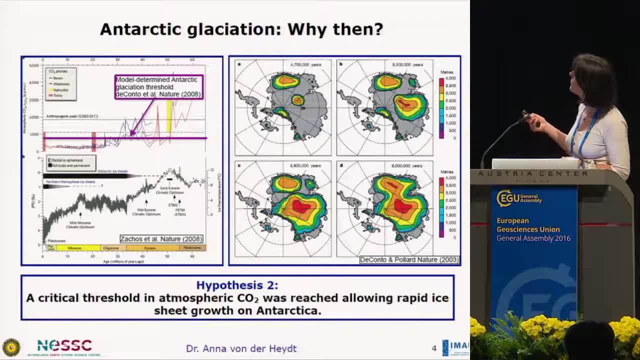 This is what you, at least, can see. This line here is the model-determined threshold for inductive glaciation, and it sort of fits into the range of CO2 values that have been measured for the Eocene-Oligosyne boundary, So it is possible that this plays a role as well. 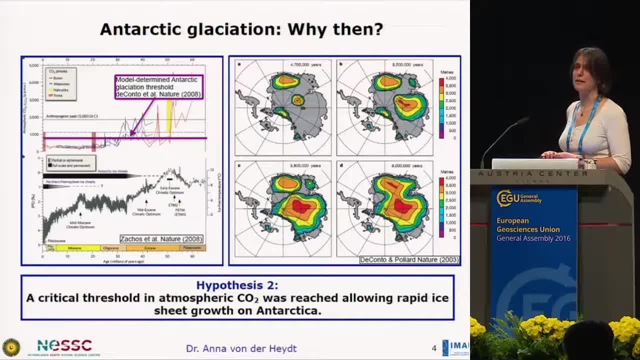 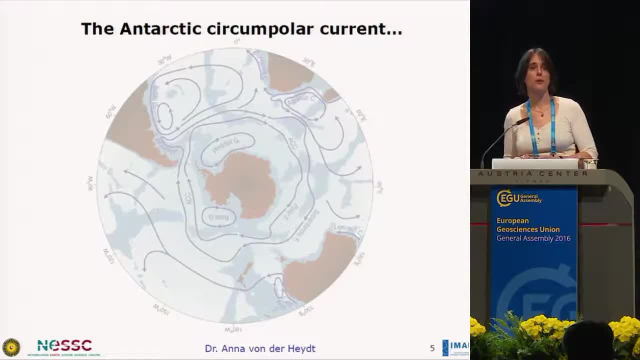 Now we all know that the world usually is much more complicated than one effect only, so probably there is a combination of many factors playing a role in this inception, And what I'm going to focus on here is that this Antarctic circumpolar current that exists today- 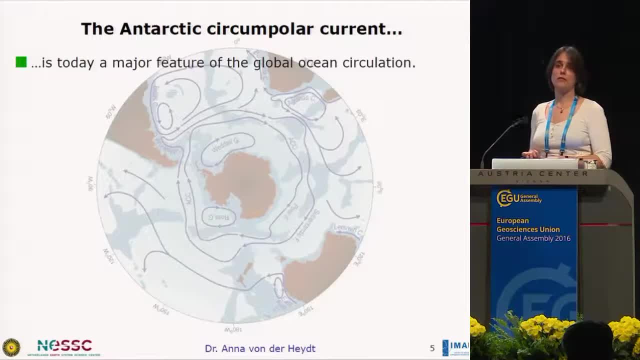 is, of course, it is a major feature of the ocean circulation today and it is really the biggest current on Earth, the strongest current on Earth, and it has wide consequences for all kinds of biological productivity And cooling and temperature distributions and even the North Atlantic meridional overturning circulation. 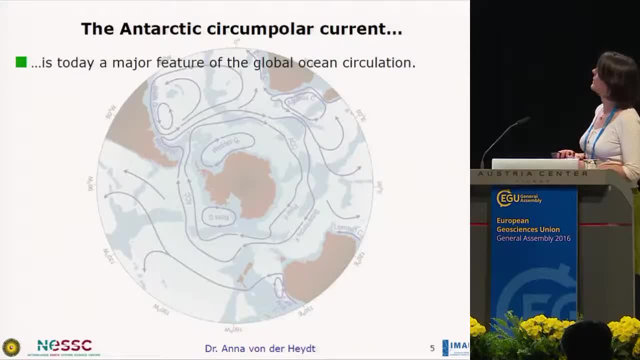 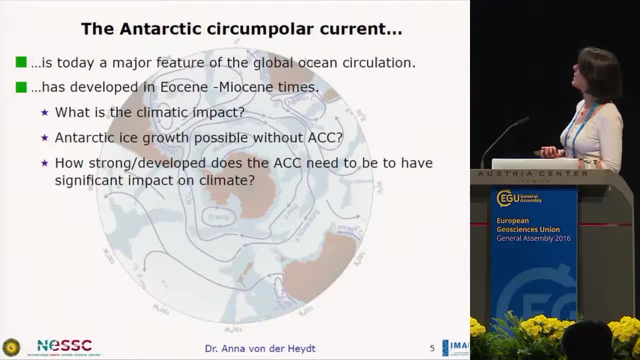 is sort of affected by that, And what is also clear is it has developed over time. So in the Eocene there was definitely no. There shouldn't be an ACC present, simply because of geometric constraints. So when these gateways are closed, you cannot develop an ACC. 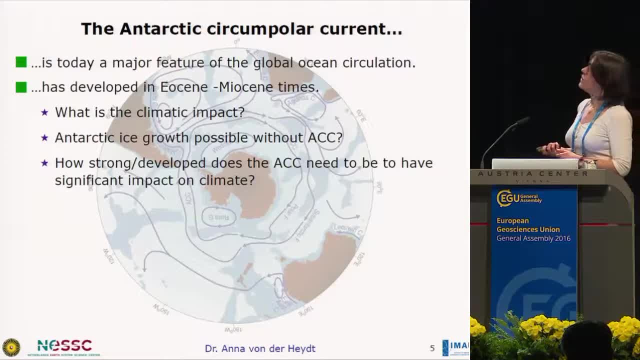 So it's still relevant To ask: what is the impact of a developing ACC? And again, as we see that the world is more complicated, it will not be the question of a present ACC or a non-ACC, but there are steps in between. 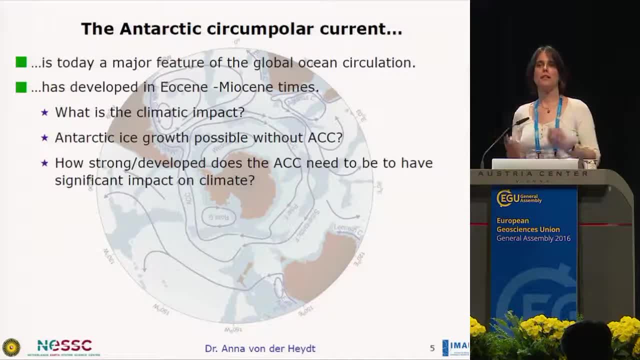 I mean, how strong does it need to be before you feel any climatic impact? Probably there were different steps, with maybe a weak one or only through flow to some gateways, but not a deep-reaching, Fully developed Antarctic second polar current, And another question that is interesting to ask also is: 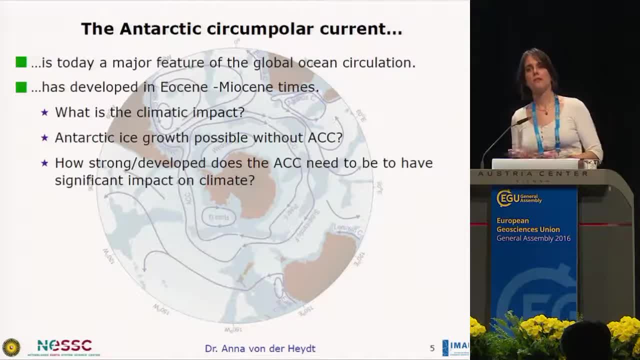 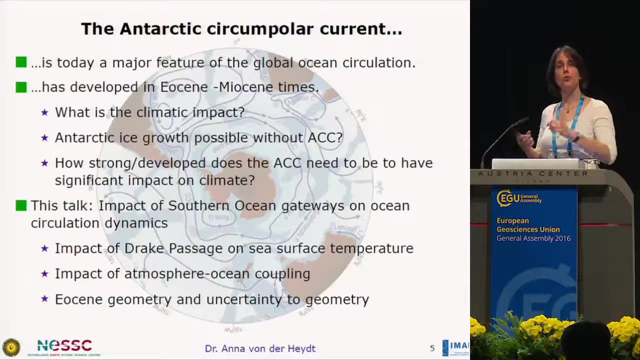 is Antarctic ice growth possible when there is no ACC? So maybe there is sort of a preconditioning necessary of the climate system before you may reach this CO2 threshold. Now what I'm going to focus on is the impact of these two Southern Ocean gateways. 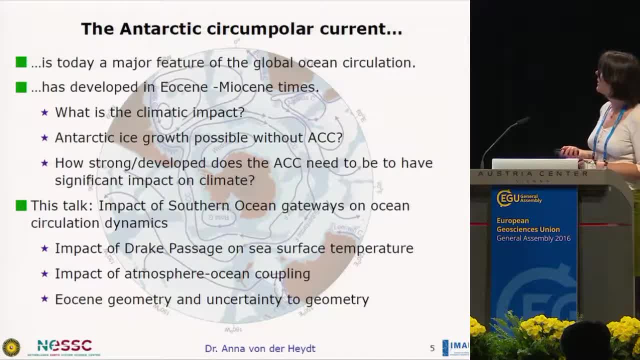 on the dynamics of the ocean circulation, And I'll I'll go through rather idealized model simulations for the present day also to simply isolate the effect of the Drake Passage on the sea surface temperature. I'll expand that then with different resolution and a fully coupled model. 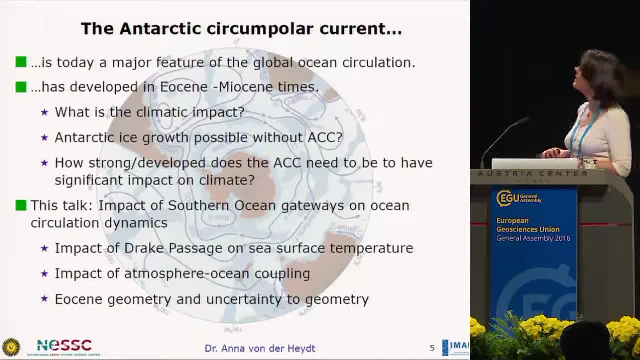 so we see what happens if you couple the ocean to an atmosphere, if you still see the same effect, And in the end I'll show you also first results of a realistic eocene contribution. I'll show you how we can assess the uncertainty in the continental geometry. 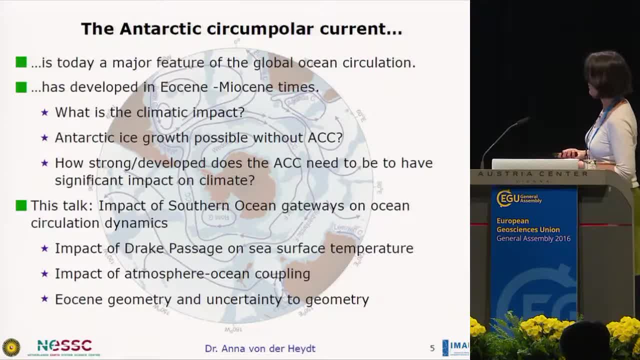 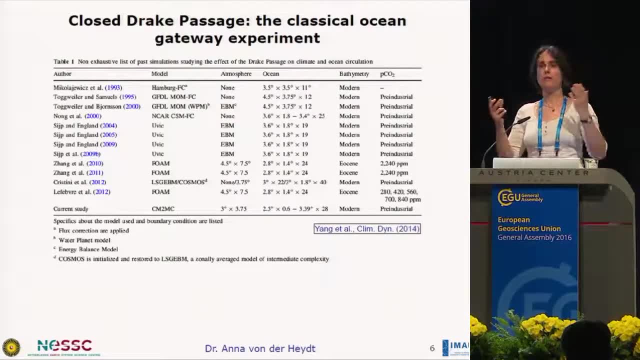 and how we can assess the uncertainty in there and what effect this has on the ocean circulation. So really, the classic ocean gateway experiment is using the present day continental geometry and closing Drake Passage, And there are many, many studies that did this already And they all see well more or less similar effects. 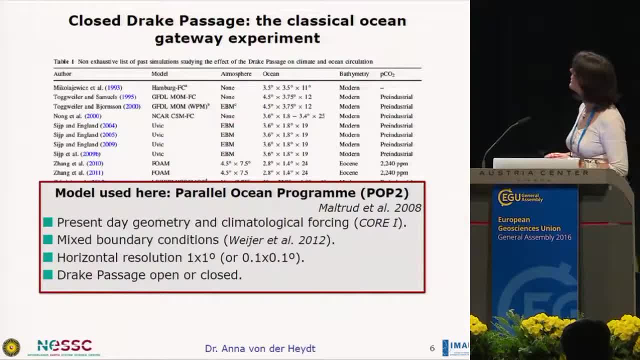 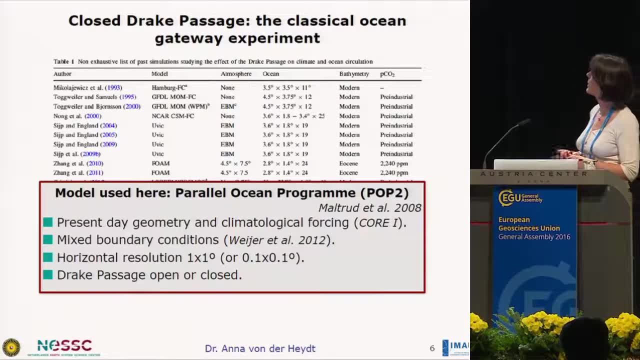 They see some warming in there. I'm going to present another one here now, using the parable ocean program, the POP model. And well, this is forced by present day climatological forcing. Very simple: It uses mixed boundary conditions. 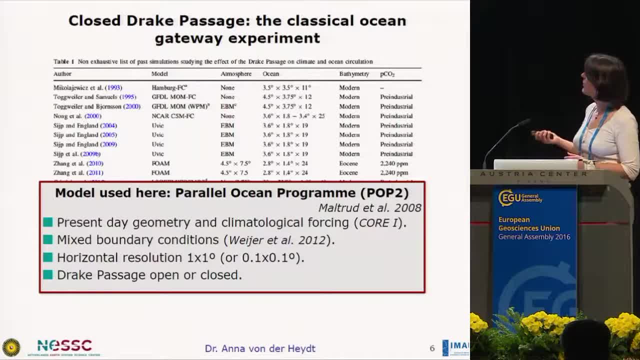 as many ocean-only models do, And initially it has a horizontal resolution of one by one degree. I have to mention here that most of these earlier studies and all paleo studies usually use relatively low horizontal resolution, I mean sometimes even lower than this one. 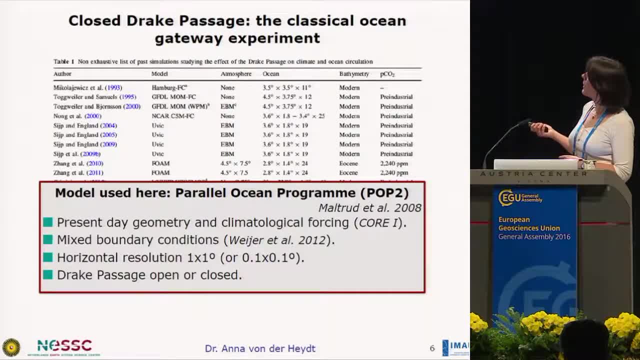 like three degrees or these kind of things. And the new thing here now is that nowadays we know that I mean vortices and high spatial resolution can be very important for the ocean circulation. So we can run this model also at one-tenth of a degree resolution. 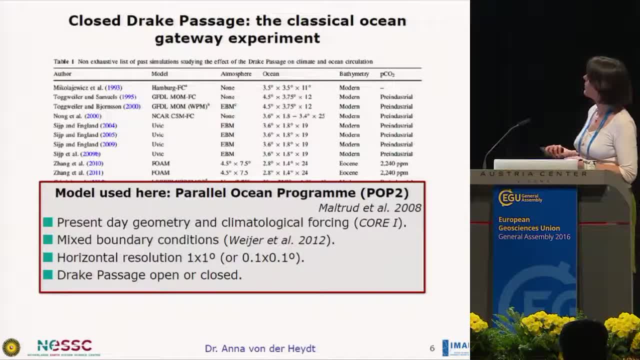 And I'll do that, I'll show that later, And we do again the classic experiment. We have one simulation as a present-day control with an open Drake Passage and another one with a closed Drake Passage. And we have one simulation as a present-day control with an open Drake Passage and another one with a closed Drake Passage. 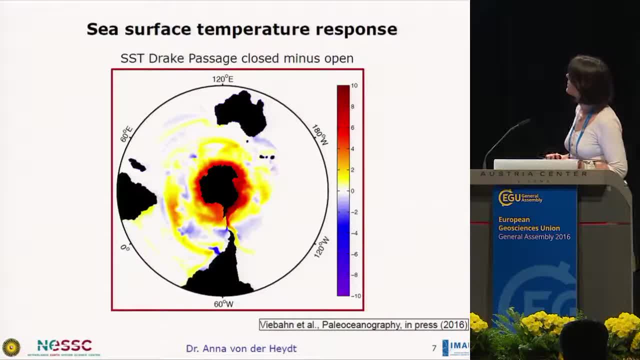 Now, this is of the one-degree resolution simulation, the result of sea surface temperature response. So what you see is that this is the difference of the case where Drake Passage is closed minus the one where it is open, And you clearly see that when Drake Passage is closed, 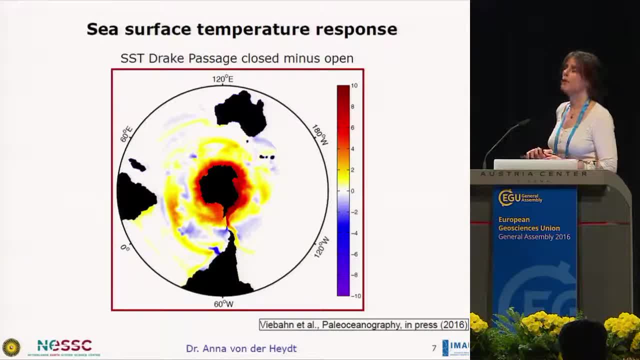 it is warmer around Antarctica, And quite considerably warmer In a few degrees. It is very localized here around the Antarctic coast, But you see a clear warming in there And we can also understand why that is. if we look at the flow Now, what you see here now is something that is 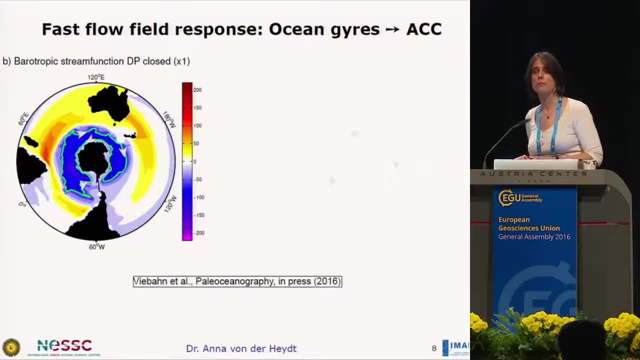 maybe only familiar to oceanographers. This is the so-called barotropic stream function And that represents the flow of the oceans, So the vertically averaged flow, basically, And if you draw these lines, for example, then you can draw some arrows on there. 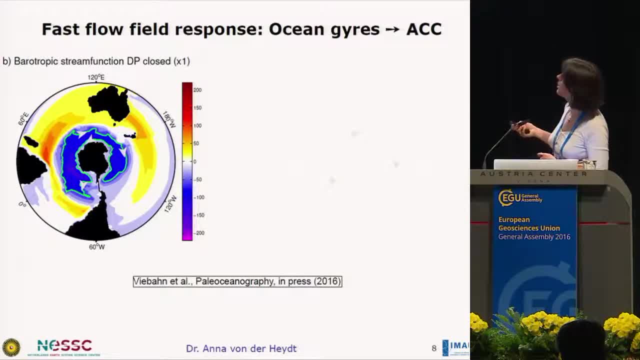 that indicate the flow direction actually, And what you see when Drake Passage is closed is something that develops in all oceans in the polar regions. when you have a boundary. This is the so-called subpolar gyre. It goes around here, So you have wind driving the flow there. 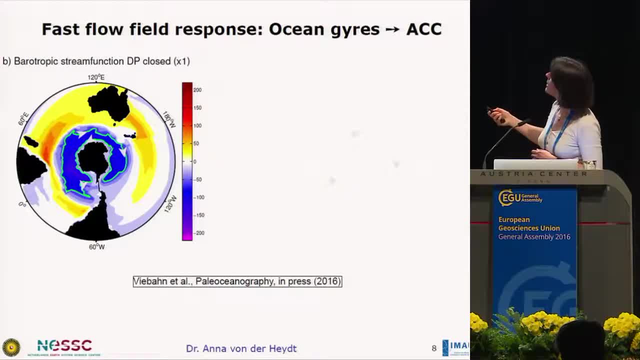 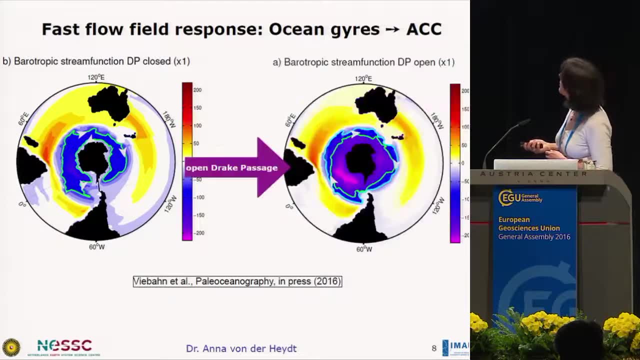 And at some point it needs to go back simply- And you have the subtropical gyre here as well that flows the other way around, Basically like that. Now, when you open Drake Passage, it turns out that most of these streamlines 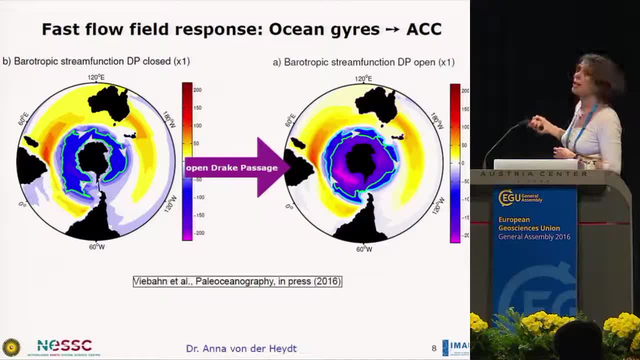 in the subpolar gyre they turn into the Antarctic second polar current, So they no longer can transport warmth from these latitudes to the Antarctic coast. So it's very clear why this warming occurs when you close Drake Passage Now. I mentioned that already. 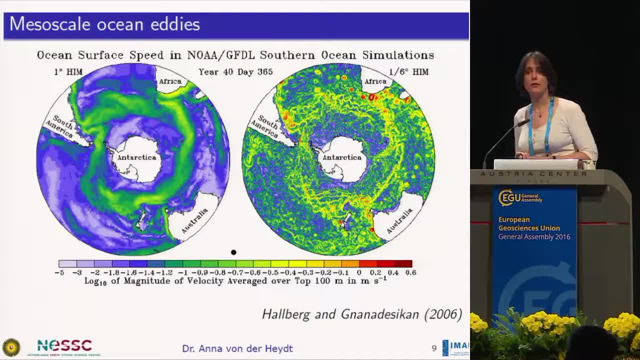 In the meantime, it is well known that the ocean is not a slow and laminar flow, but it's very turbulent And in particular in the Southern Ocean, for the Antarctic second polar current, it is important to represent these eddies and vortices. 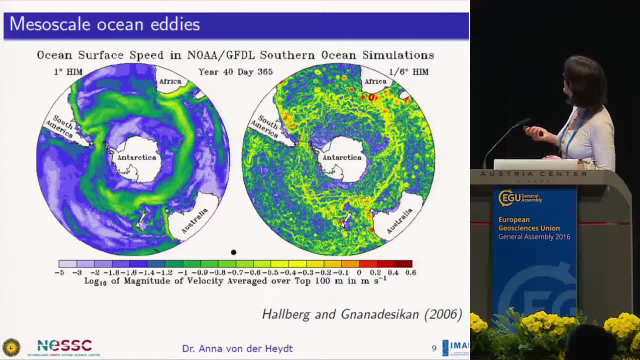 in the correct way. So therefore, this has been shown for the present day also, that when you use a high resolution, that you get many of these eddies and vortices, a lot of structures in there that of course also affect transport of properties. 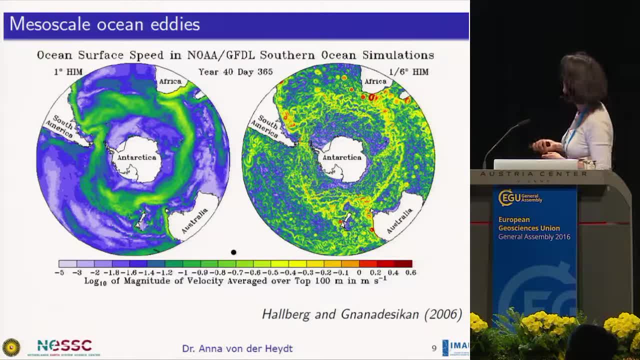 of heat and salt and nutrients and upwelling. Upwelling is different in these eddies, And so all kinds of dynamics is represented in this higher resolution. So we thought, well, let's do the same experiment at a higher spatial resolution. 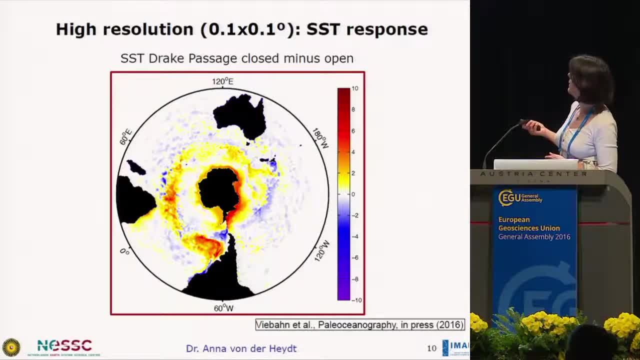 And this is the result: We have again a Drake Passage open and a Drake Passage closed experiment, forced with present day conditions at 1 tenth of a degree horizontal resolution. And again here, this is the difference in sea surface temperature between Drake Passage closed minus Drake Passage open. 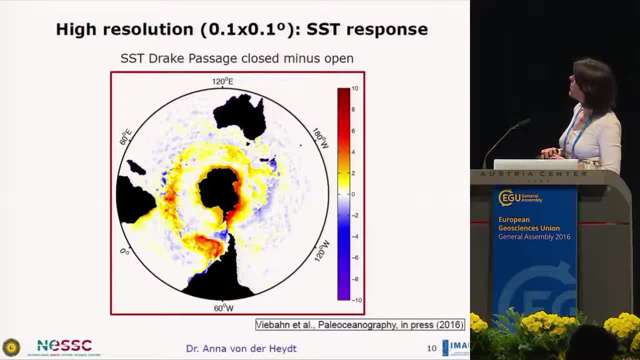 And you see again this warming, although there are also some differences. I mean, you see of course much more local, small-scale structure, but you also see that there is some peculiar warming here at the somewhat higher latitudes. There is no warming in between here. 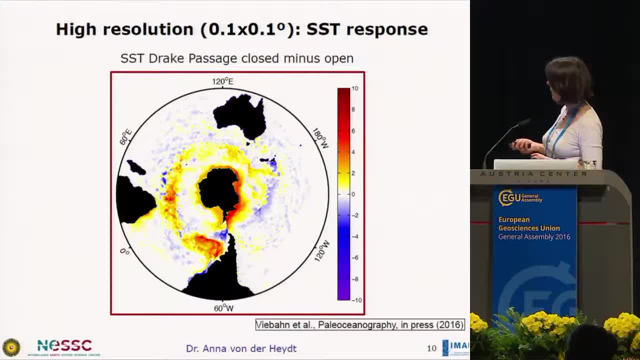 So it's much differently distributed. Now, if you average around Antarctica, so you do a zonal average still, the response is relatively similar, but you do see quite some differences. Oh yeah, and I think I have to say here that this, of course, is becoming important. 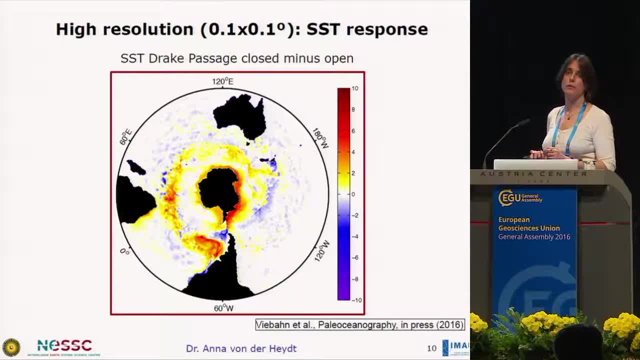 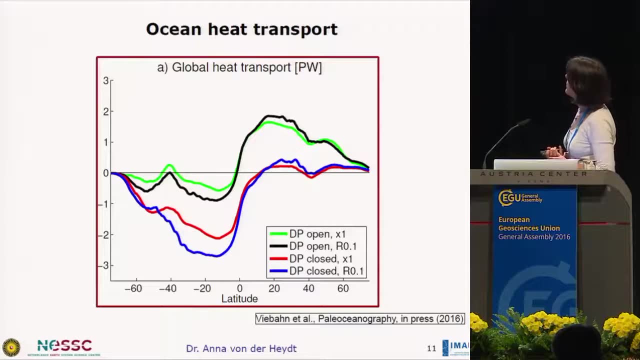 when you start comparing simulation models with really data, because, of course, paleo data, they come from single cores and it depends whether you resolve these localized bonds or you don't. Now, what does this? warming is basically the ocean heat transport. 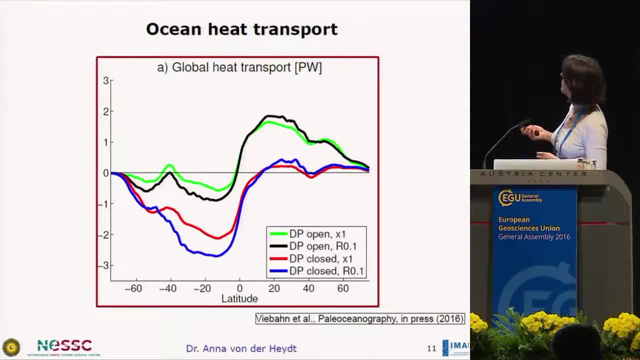 and now this is somewhat complicated. Many curves on here of the meridional heat transport, so it's only integrated. Here is latitude And the black and the green lines. these are sort of the present-day Drake Passage open simulations at the two resolutions. 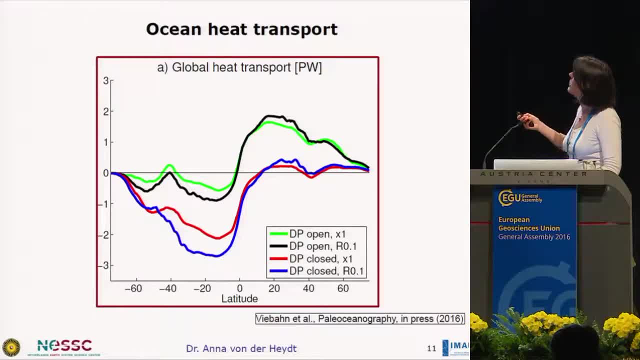 so the black one is the high-resolution case. They look fairly similar, although there are some differences in there in the eddy resolving and the one And well. we have usually somewhat less heat transport in the southern hemisphere to the south than in the northern hemisphere. 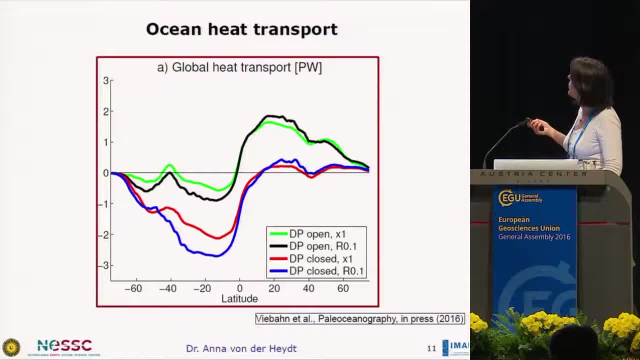 Now the Drake Passage, close experiments, the blue and the red one. they are very different, so they have much more heat transport in the southern hemisphere and much less in the northern hemisphere. Now, actually, what matters for the warming is these differences here in the subpolar gyre? 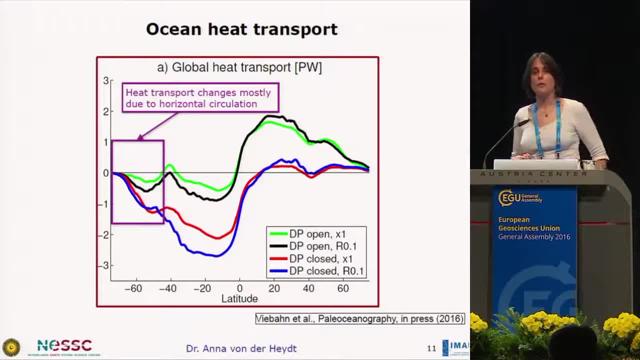 and you see some differences in heat transport. They are not large but obviously there are enough to do this warming in the end. These other changes here, they are actually due to some other effect that happens due to the Drake Passage closing or opening. 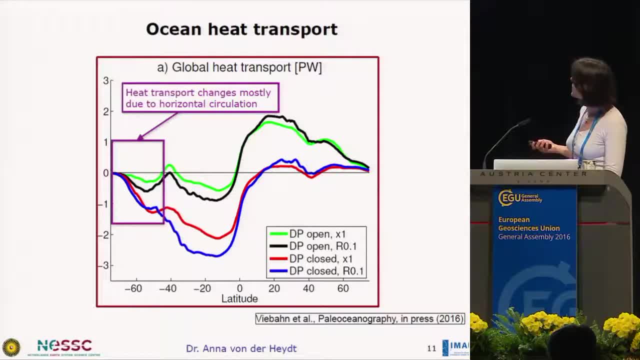 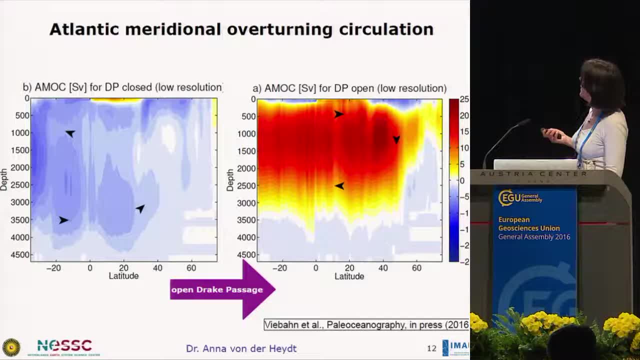 depends which way you go, which I didn't show yet- and this is the meridional overturning circuit. So what happens when you close Drake Passage? in a simulation of the present day where you have simply the normal Atlantic meridional overturning circulation? 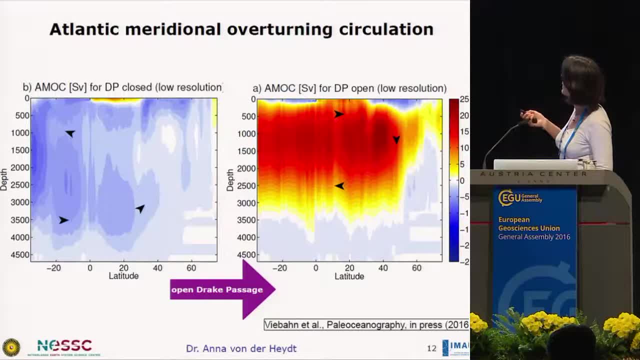 here again as a stream function. so this is latitude and this is depth through the Atlantic. These arrows indicate sort of the mean flow direction. So when you close Drake Passage, immediately this circulation collapses, It shuts down and even well, sort of reverses. 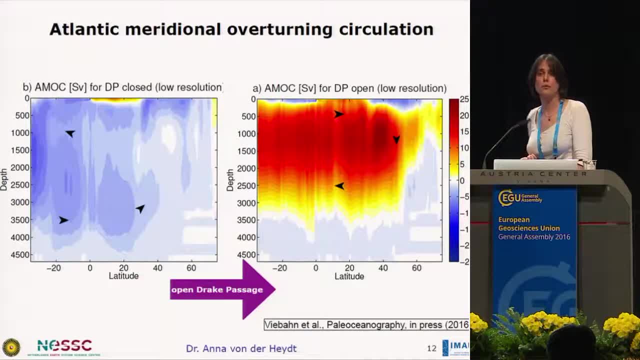 in the end, And that of course affects a lot more the heat transport and simply the direct effect of the Drake Passage closing, which is on the horizontal flow in the subpolar gyre. So this warming that we see around Antarctica is actually, say, the basis of this hypothesis of Kennet. 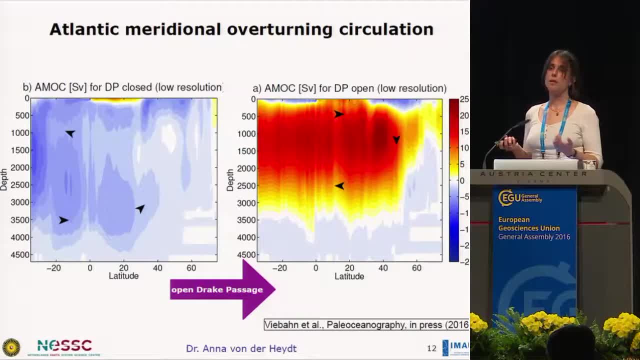 and this is a very robust feature. I mean, it is clear that this would happen always when you have a normal wind distribution. When you close the Drake Passage, you will get a subpolar gyre, So we expect that, indeed, this warming. 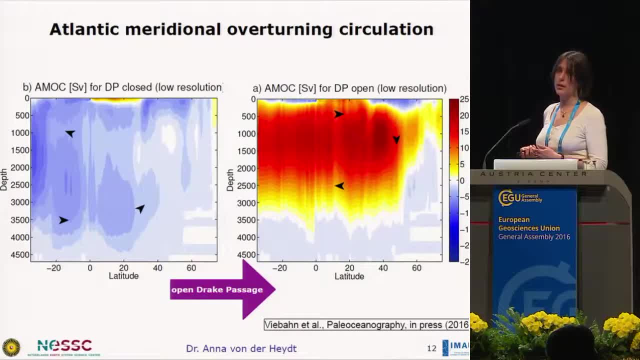 due to closed gateways in the Southern Ocean. this will always occur. What is less sure or less certain is how much warming you will get, Because this, of course, can depend on certain details. We've seen already between the high and the low resolution simulation. 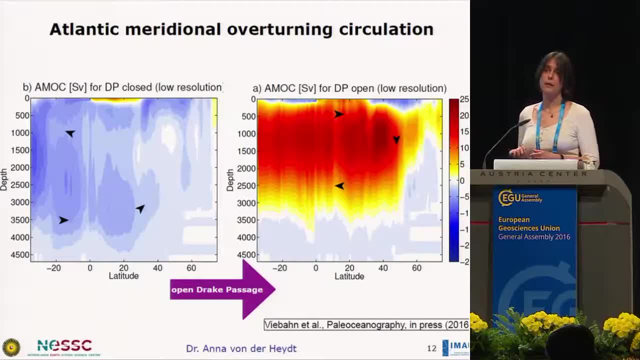 there are quite some differences in the magnitude of the warming And we've seen the heat transport. Of course it depends whether or not this Atlantic meridional overturning circulation will collapse or not, And it can also depend on how much the heat transport. 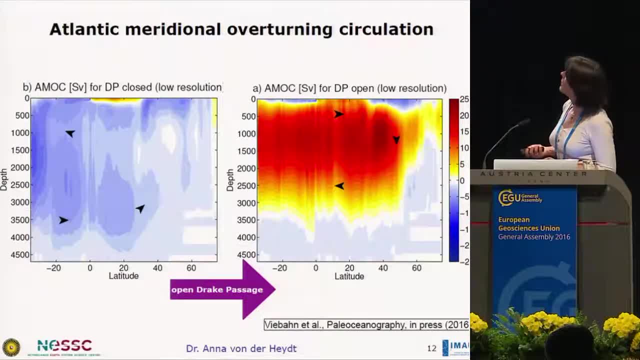 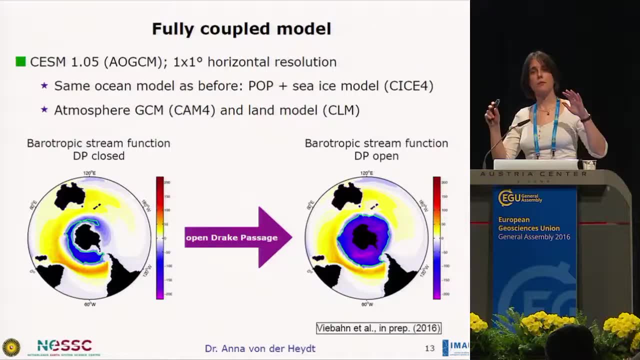 really affects the sea surface temperature And this is why we started a different set of simulations where we actually coupled an atmosphere. I mean, in the previous one there was a prescribed surface forcing for the ocean, But when we couple the atmosphere we can see different effects. 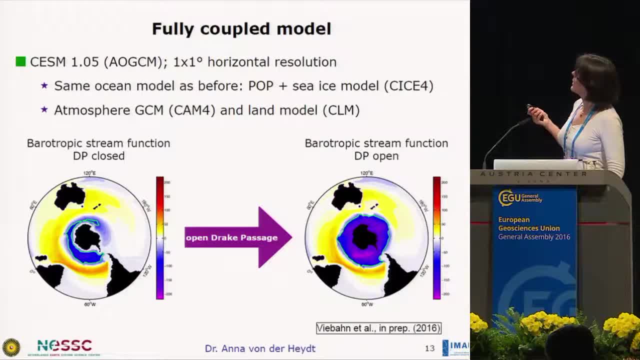 So we used the same ocean model And actually the model we are using now is the CESM. It contains the POP model as the ocean part and it has, in addition, a sea ice module on there. It has an atmosphere, a three-dimensional atmosphere model. 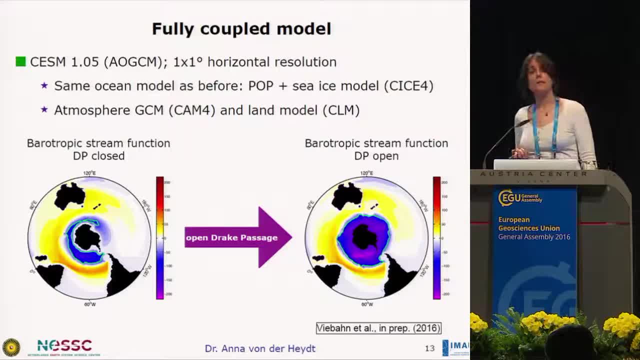 and a land model on there And we do again the same classical experiments And what we see is basically the same effect as to the horizontal circulation. This is again the barotropic stream function in the Southern Ocean. You see, with a close drag passage. 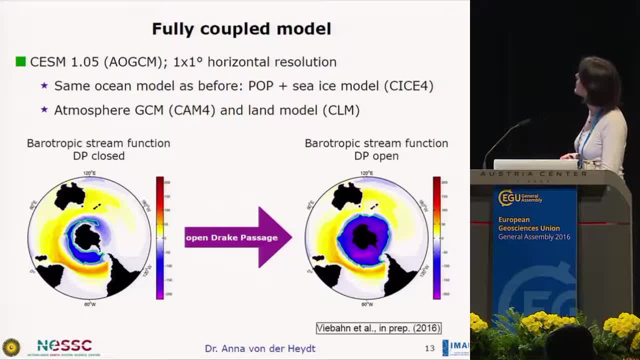 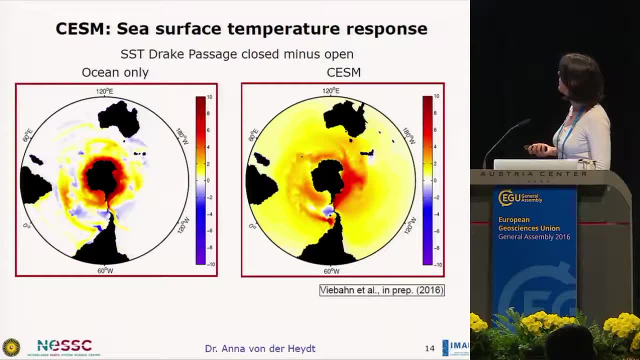 this subpolar gyre and most of these streamlines turn into the Antarctic circumpolar current when you open the drag passage And you see also quite some warming. Now this is the CESM, the coupled model, warming in there. And as a comparison, 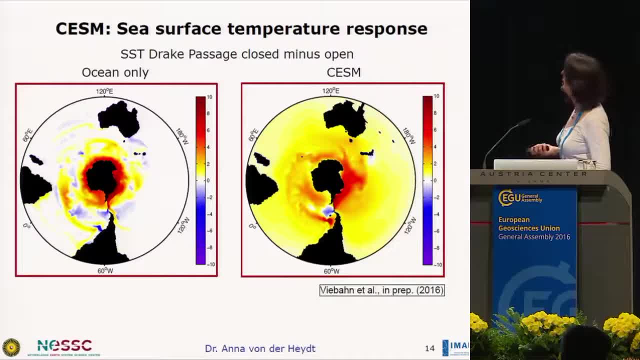 this is what we had in the ocean-only simulation. Now there is warming indeed, but there are quite some differences. I mean it's much less localised around the coast. Still, there is a localised warming here at this side of drag passage, say. 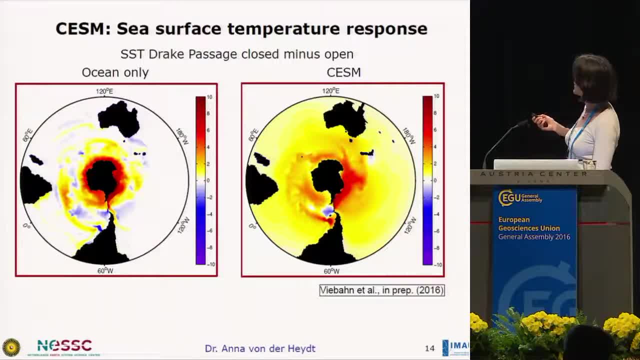 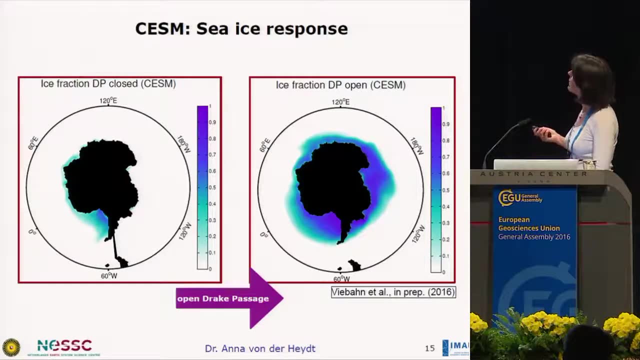 But you also see that it's more spread out and you have a lot of warming here at lower latitudes in the end. Now, there are different reasons for that. One is certainly that now we have sea ice to dynamically evolve And in the warmer case, 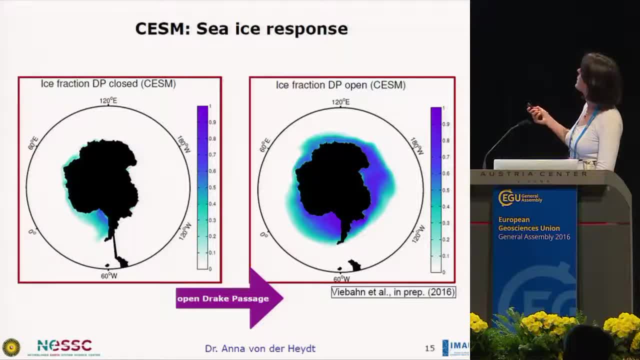 when drag passage is closed there is a little sea ice, But here, with the open case, we have much more sea ice to develop, And that of course influences the surface heat fluxes also, so you distribute the warming much more. 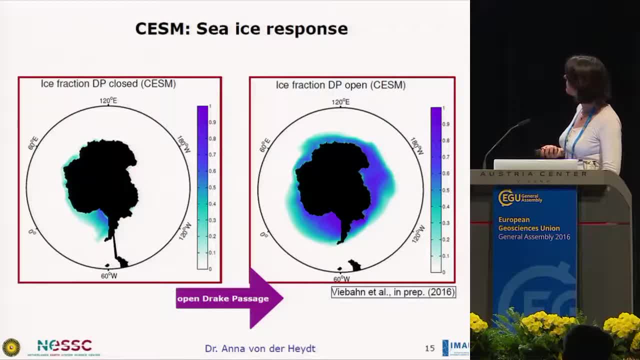 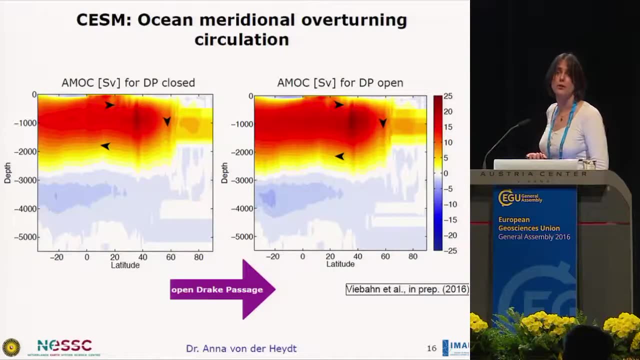 also to outside the sea ice region in there- And another factor might be particularly for this low-latitude warming that we've seen- is that in this case the ocean circulation in the Atlantic does not collapse when we close drag passage. It stays more or less the same. 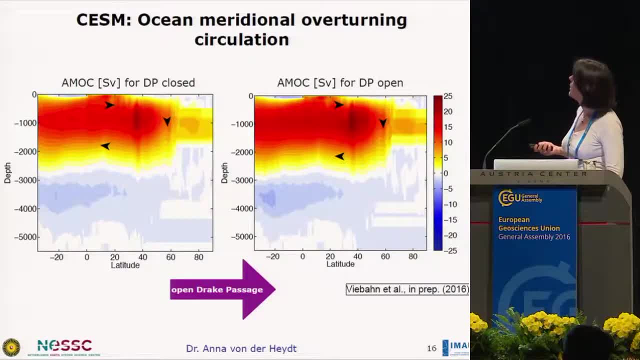 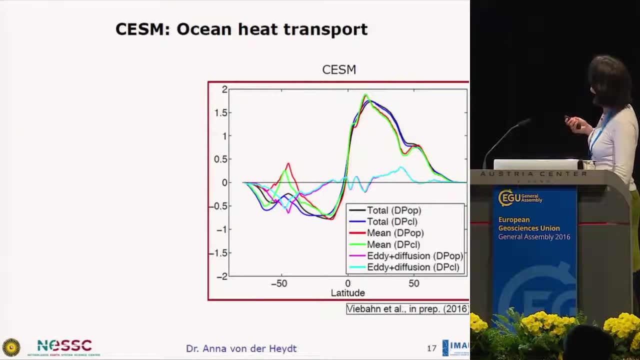 so also in both cases, And that means that also the heat transport becomes a bit more easy to understand, a bit more difficult. Now in this plot here I would like you to focus on the blue and the black line. The blue one is the total. 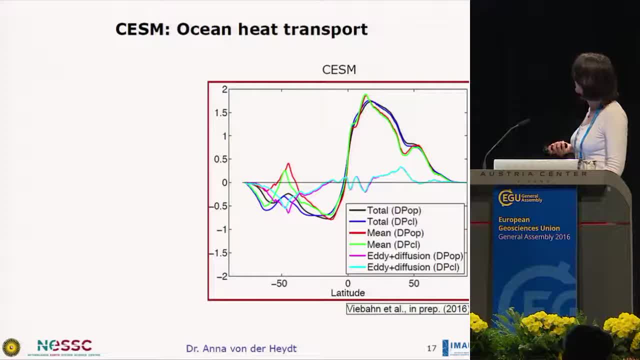 marginal heat transport in the ocean with a closed drag passage And the black one is the present-day one with the open drag passage And you see, particularly in the Northern Hemisphere they are very similar. So there is no change in the meridional overturning circulation. 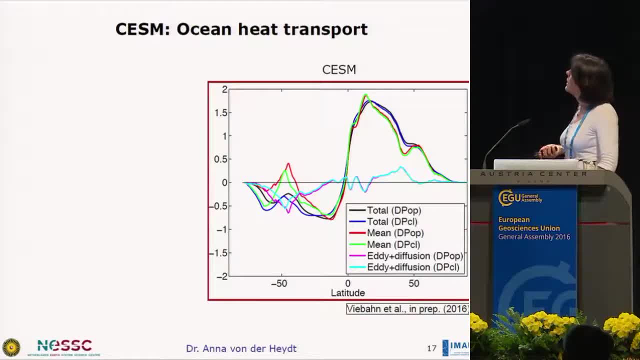 And in the Southern Hemisphere you do have differences. I mean they look small, although you have to realize that these are zonally averaged heat transports in the ocean, so it's still quite some magnitude that affects that here And it of course has some impact. 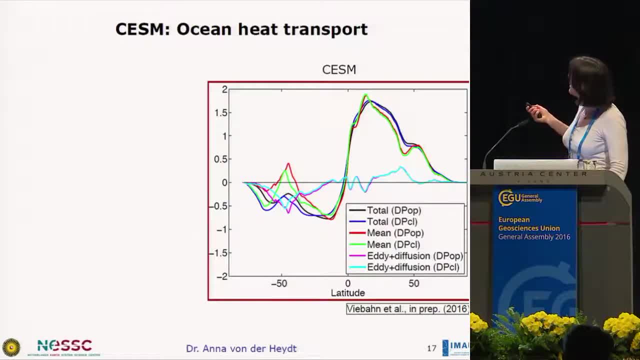 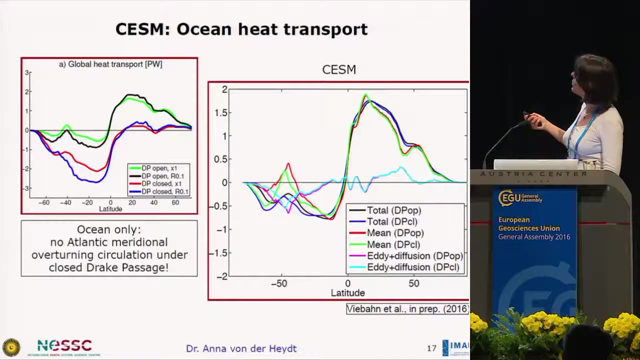 on the sea surface temperature distribution. You also see differences in heat transport at somewhat lower latitudes, which may already there affect the sea surface temperatures, As compared to the ocean-only simulations. this is what I've shown before. when we compare the green-black 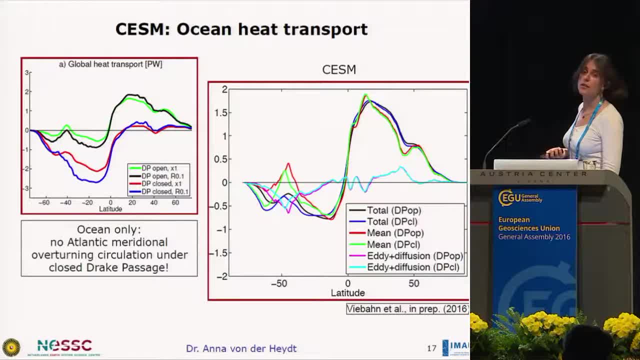 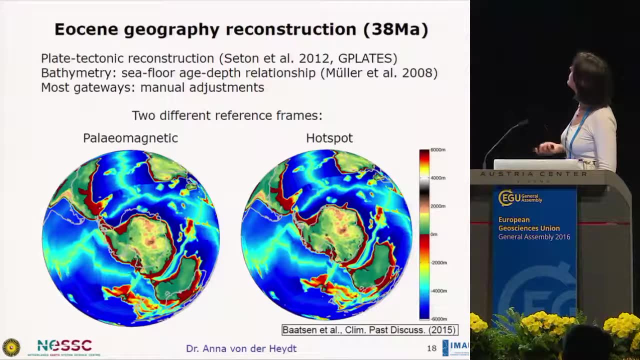 versus the red-blue. There are, of course, much larger differences, which are mostly due to this overturning circulation collapse. So this was all for really a present-day geometry. Now we can ask, of course, what really happens in the Eocene. 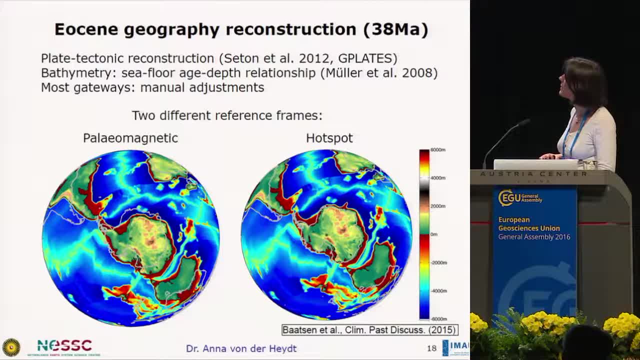 when, potentially at the end of the Eocene, or at some time at least, these gateways opened And therefore what we have done is generated a new geography reconstruction for the late Eocene. It is relatively general, so it should be easy to generate. 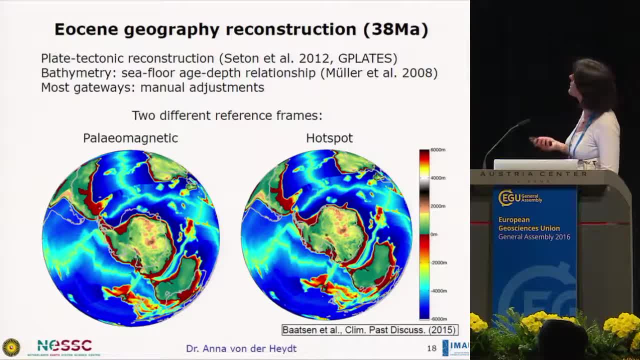 different time slices as well with the same method. It starts with a plate tectonic reconstruction where you can go back in time basically wherever you would like to go, And we used well different data sets, for example for the bathymetry. 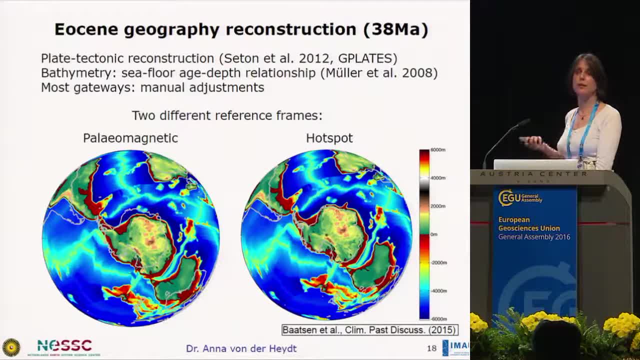 At the seafloor. these age-depth relationships tells us a lot about how deep the ocean was already, But there are many regions in the world that actually need manual adjustments to there, and these are particularly the gateway regions. So you need to add more information. 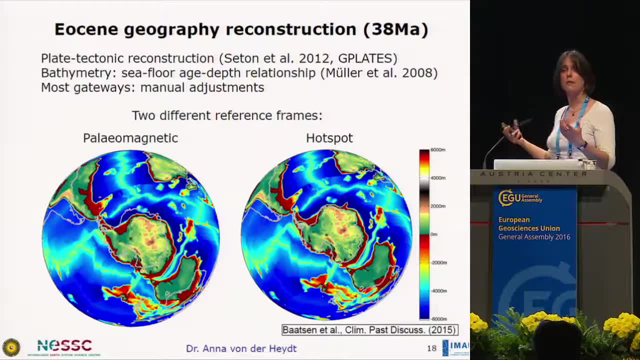 into this original reconstruction to get really a fully globally covering reconstruction that can be used in a climate or an ocean model. And the interesting thing is that when you go to these plate tectonic reconstructions you can use at least two different reference frames. 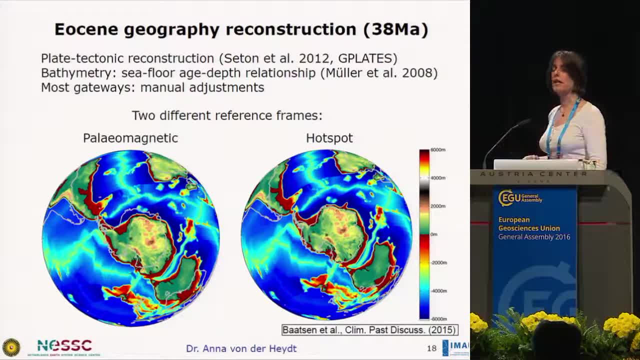 with respect to these rotation of the plates in time. One is the paleomagnetic reference frame, the other one is the hotspot reference frame And at first sight you may say, well, there are not such big differences in there, But it's good to look at these grey lines here. 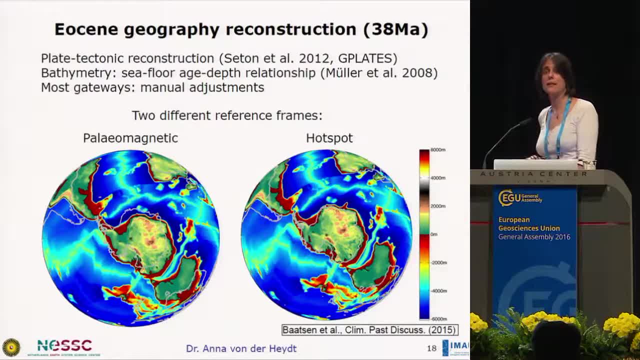 which reflect the present-day coastal climate. And that tells you that in the paleomagnetic reference frame, Antarctica has moved quite a bit from the South Pole. In particular, it covers now lower latitudes here with land, While in the hotspot reference frame, 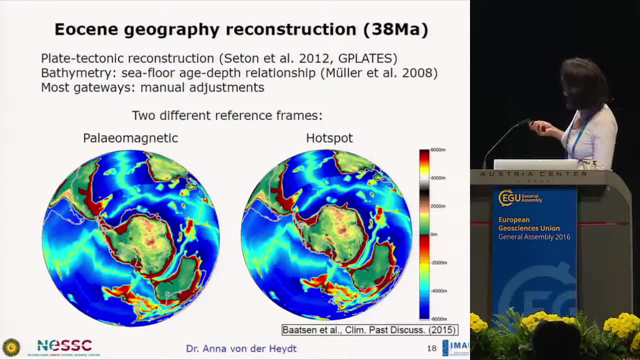 it is almost at the same location as today. Now, indeed, the shape of the continents is not different in these two reference frames. but the position can be quite different, and particularly for the Antarctic continent Now, as we are oceanographers and not plate tectonic experts. 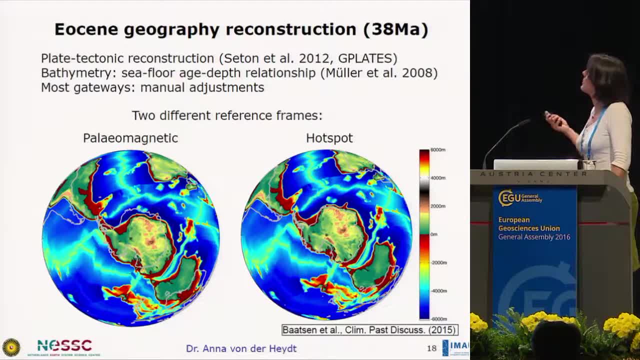 it is, of course, well, it may be debatable which of these reference frames is better or less good, But we can see it simply as an uncertainty. we have on the plate tectonic reconstruction on the continental geometry actually. So what we did is we used these two geometries. 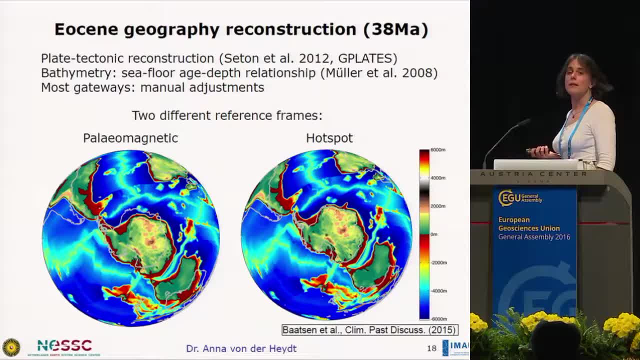 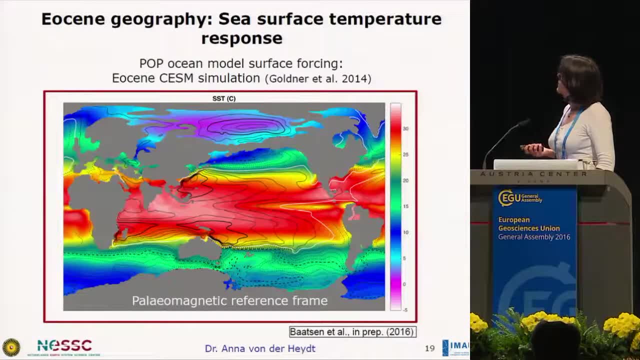 in the same ocean model as before and did long simulations. We did a long simulation with that And this is the result for the sea surface temperature. I'll tell you in a minute more. Now, when we do this simulation, we can no longer use the surface forcing of the present day. 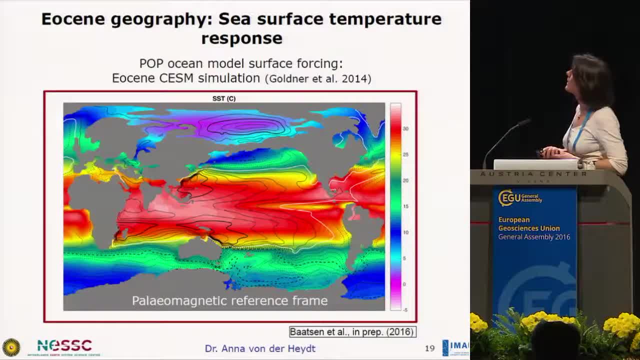 of course, because really the continents have shifted. What we did instead is we used an Eocene-coupled climate model simulation that existed already. It was at a lower resolution, at high CO2 concentration, And it used a slightly different continental geometry. 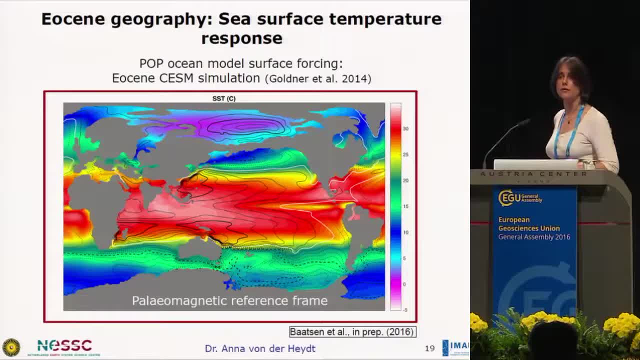 but it was still possible to sort of interpolate the surface forcing to the geometry we used here. Now this is The colours, is the sea surface temperature and the lines: is the barotropic or the sea surface height actually something that represents the barotropic stream function? 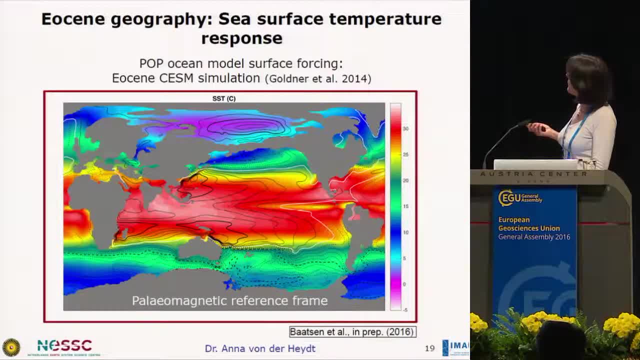 the flow. I would like to focus you mostly on the colours, the sea surface temperature, And this is the result for the paleomagnetic reference frame, And this one is the result for the hotspot reference frame. Now, if I go back, 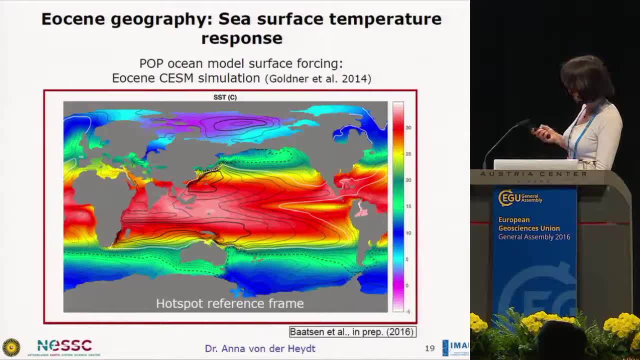 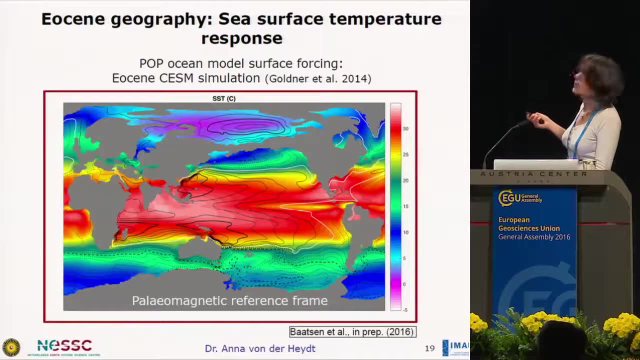 you can focus on this region and on this region And what you see is there are quite some differences in sea surface temperature. So here it is relatively cold there and warm here, while in the other it is cold here and warm there. 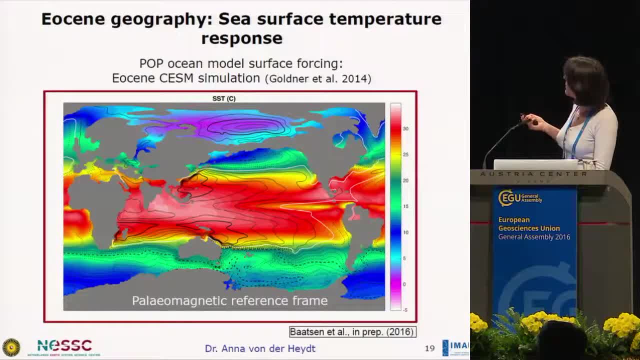 And obviously this has to do with a sort of a subpolar gyre in both hemispheres. in the Pacific that is there or not. Now, in both cases you have some transport through both of the gateways, although they are relatively small. 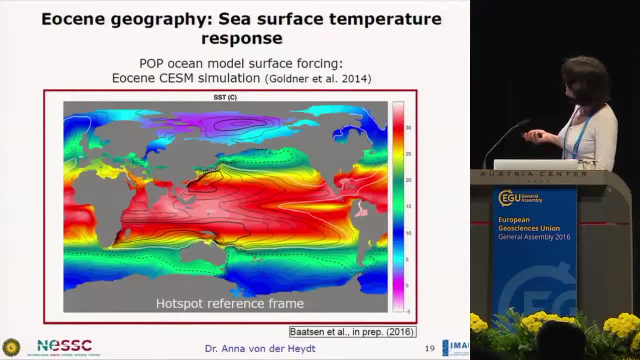 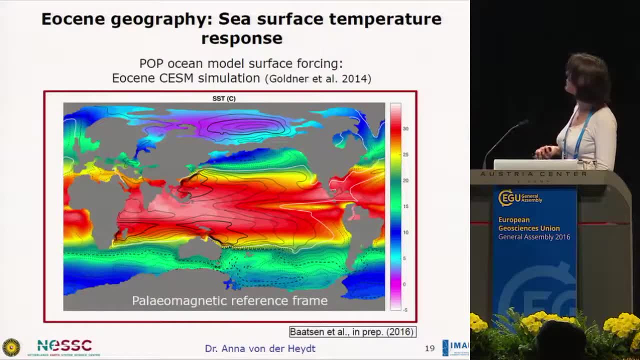 as compared to the present day. Interestingly, they are the same width and depth in both reference frames, But still you have in one of them, you have through the Tasman gateway, you have much more transport, Much more transport than in the other. 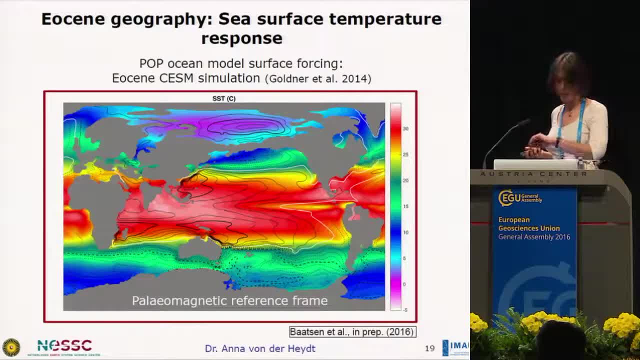 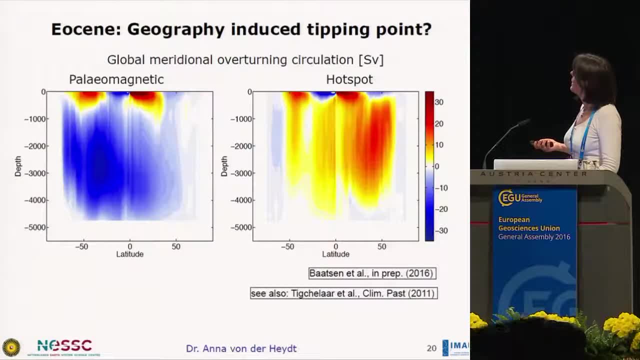 So there is some, and it is the same surface forcing. So there is some intrinsic variation in the circulation itself And the reason lies probably again in the overturning circulation. Now, as the Atlantic is very small, there is hardly any overturning. 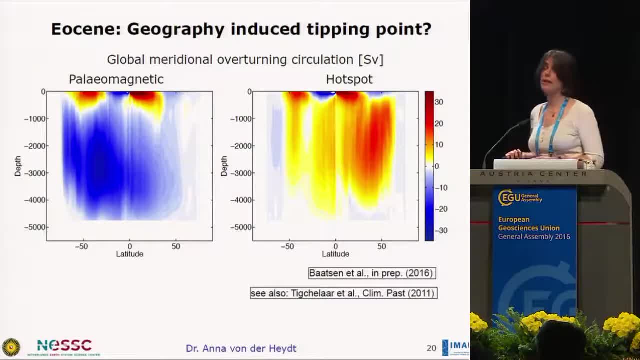 in the Atlantic, but most of it is actually in the Pacific happening now, And you clearly see that the overturning circulation in the paleomagnetic reference frame has deep water formation. So it goes that way: It has deep water formation in the South Pacific. 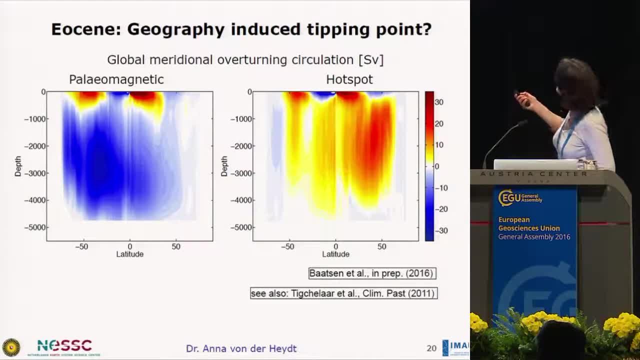 While in the hotspot reference frame it has deep water formation, The cell goes the other way around: It has deep water formation in the North Pacific. So these are really very different patterns And of course there are some heat transport differences associated with that. 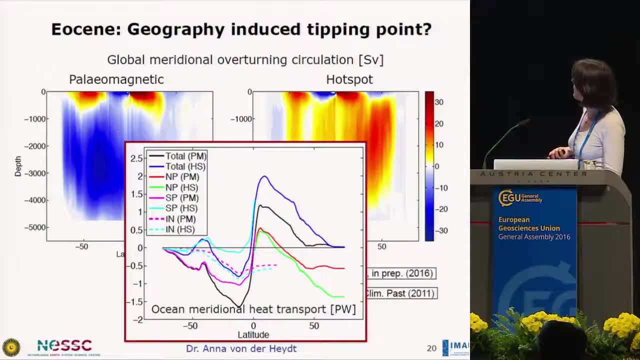 Now again the black and the blue line. this is the total ocean heat transport in this simulation. In one case you have much more heat transport in the Northern Hemisphere and less in the Southern Hemisphere, And in the other one it's exactly opposite. 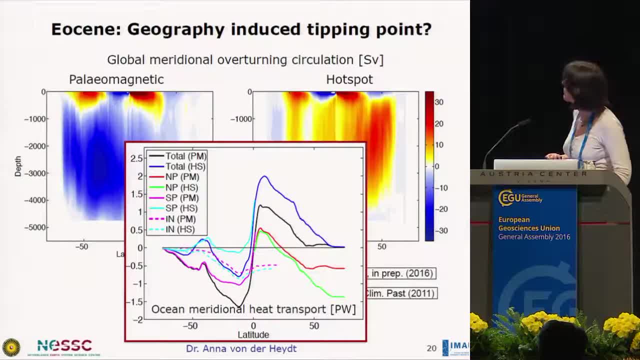 So this of course makes a big difference for the sea surface temperature distribution. So the black one refers to the paleomagnetic reference frame and the blue one to the hotspot reference frame, which we simply associated with. well, uncertainties in the reconstruction. 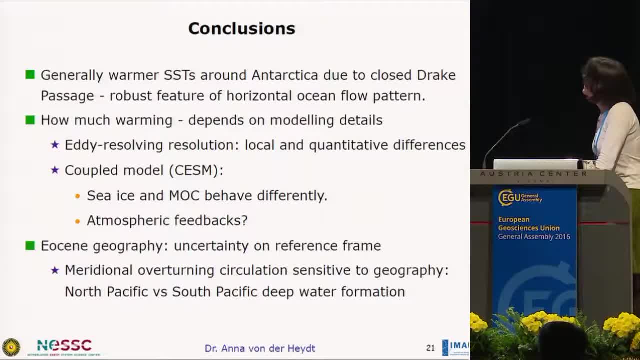 So, to conclude, the warming around Antarctica when you close Drake Passage? this is obviously a very robust feature. that must occur simply due to the horizontal ocean currents, And it's very unlikely that the wind structure would be completely different than it is today. So you would always 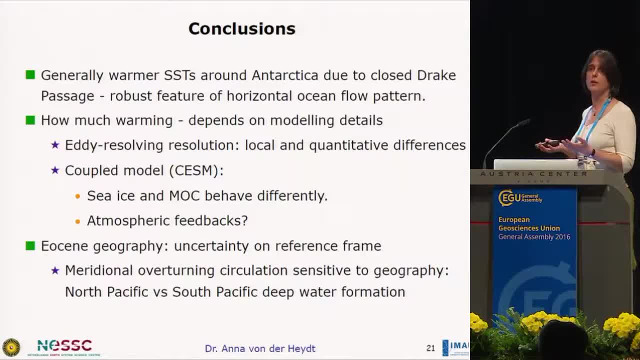 if there are some barriers, you would expect that there are subpolar gyres and subtropical gyres to be developed in there. Now, how much warming occurs? this is much more difficult to answer because this really depends on, well, the resolution of the model. 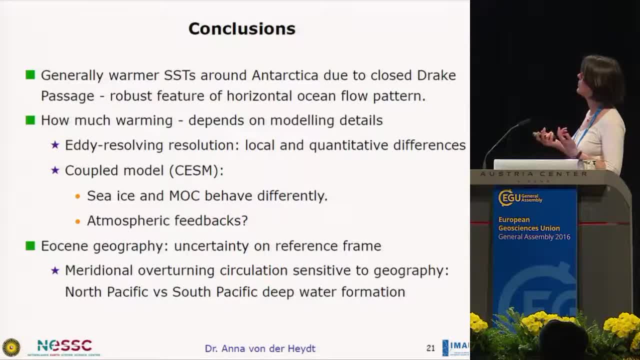 and whether it's coupled or not, and whether well the realistic geometry is used. This certainly depends on other factors as well. Now, when we go to any resolving spatial resolutions, there are particularly local differences, but there are also some quantitative differences. 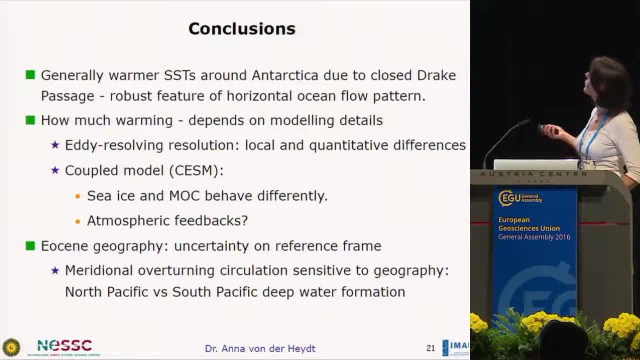 So in general you have less warming in the higher resolution. When you couple an atmosphere and a sea ice model, then you clearly see that the sea ice plays a role in the distribution of the temperature, the sea surface temperature change and also the overturning circulation. 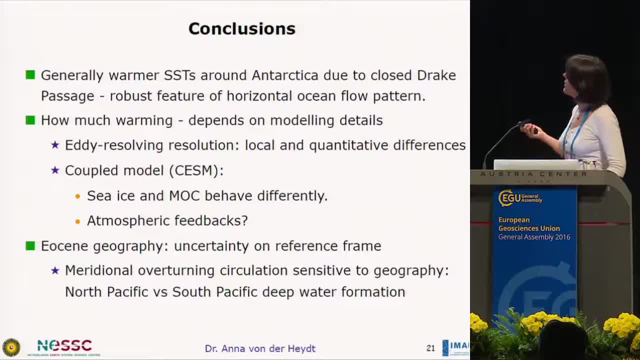 behaves differently in this simulation. There may be some atmospheric feedbacks, which we didn't look at yet, that enhance or weaken this warming. so there is a lot more to learn from these coupled simulations Now when we go to a realistic reconstruction of the Eocene geography. 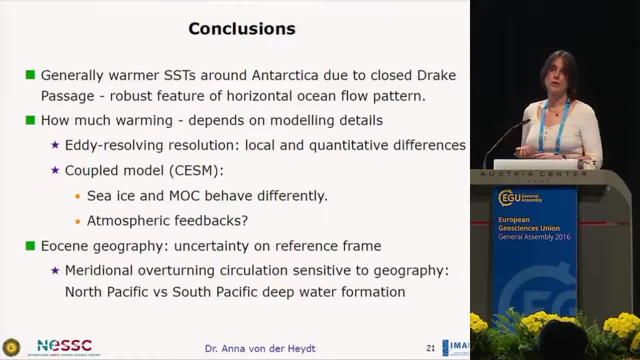 we see that there is quite. we can see it as an uncertainty in the reconstruction and the interesting thing is that actually, to rather small differences in the continental geometry and the ocean circulation is rather sensitive as to which type of overturning circulation it generates. 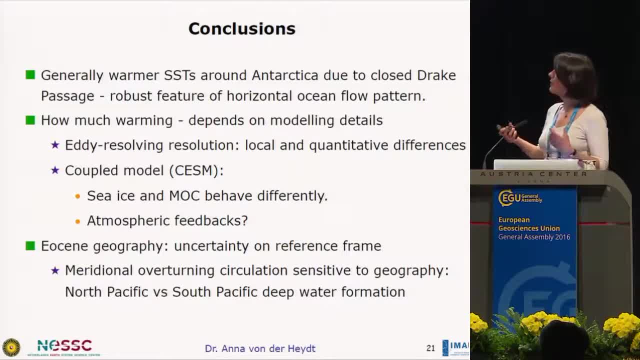 So it might very well be that some small change happened at some time that switched the overturning circulation to some other mode, and by that you would already get less heat transport to the southern hemisphere, such that you could more easily grow the ice than before in the other circulation pattern. 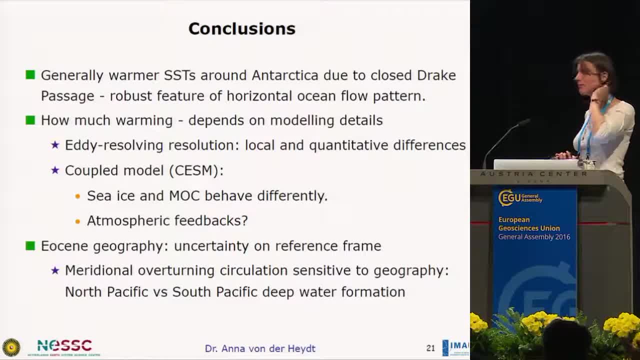 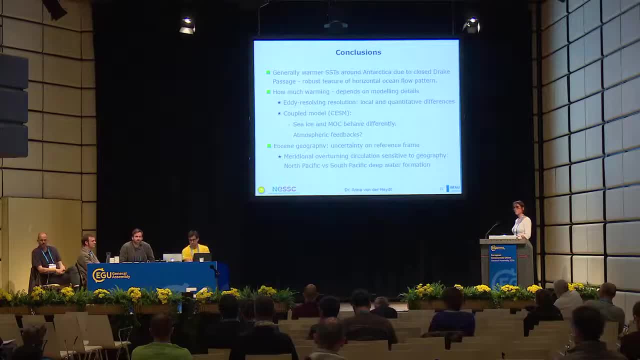 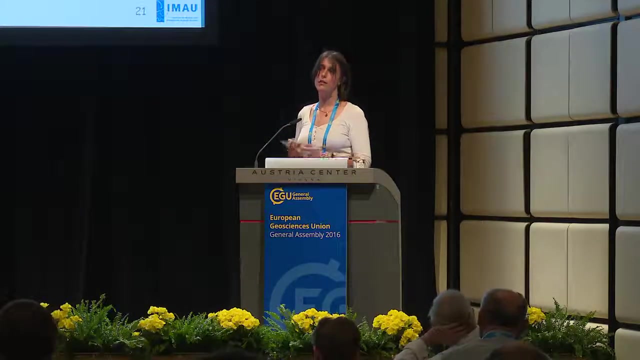 Thank you very much. Thank you very much for this great talk. We have plenty of time for questions, so please go ahead. 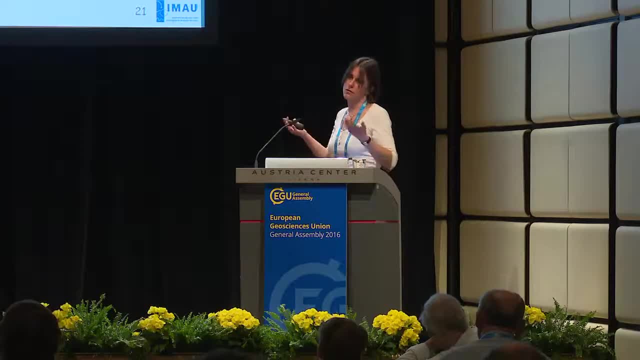 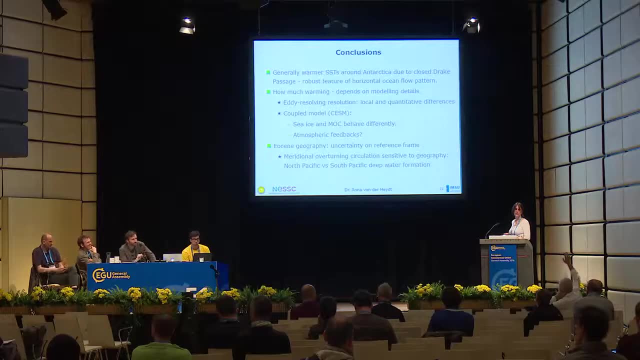 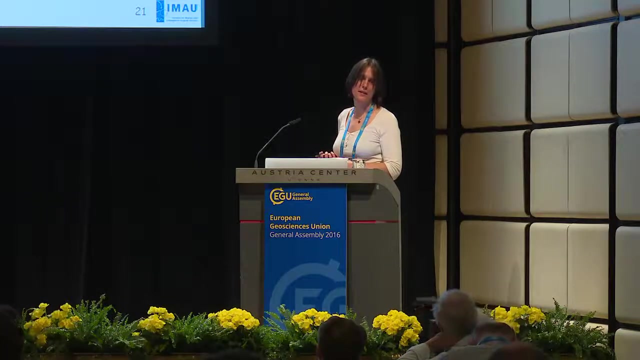 This is indeed the next step. Yes, Yes, Yes. Well, this is true, and, but this is particularly. I mean, we know this for 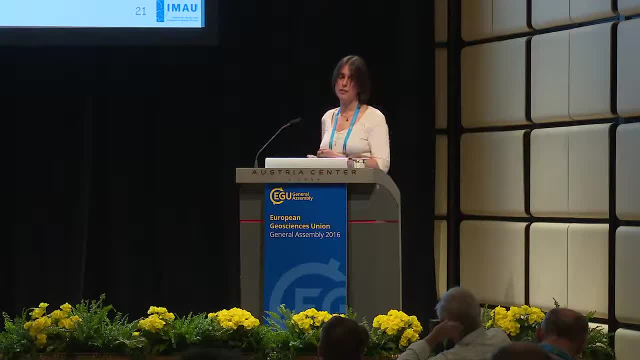 the present climate, where the overturning takes place mostly in the Atlantic. Now here we really get a very different pattern, and it's not a priori. it could be, but it's not clear that this really also this compensation also happens. so it could be that it's indeed. 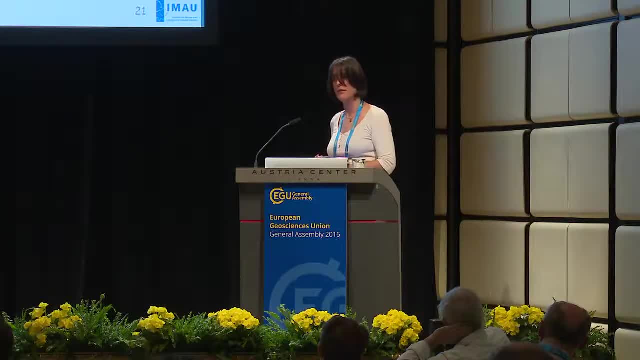 more sensitive when you have a completely different ocean circulation. Yes, Well, here I think you're using more SOD story. Yes, Yes, Yes, Yes. Well, yeah for temperature. yes, Yes, Yes. 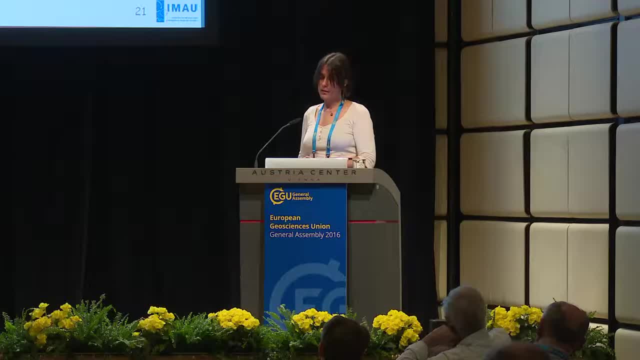 That's true, That is right, Although, again, in this case the special resolution may play a role as well. I mean, when you go to a higher resolution, it might be easier, even in the coupled context, to break down the overturning circulation. 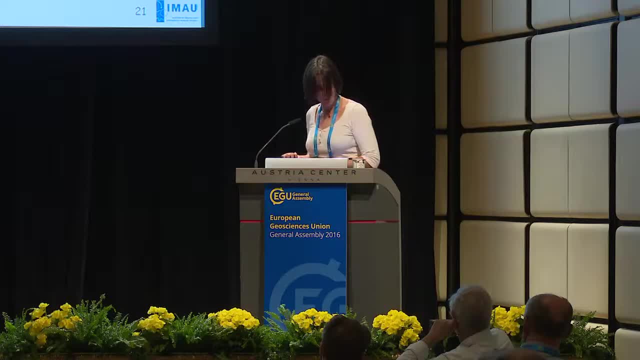 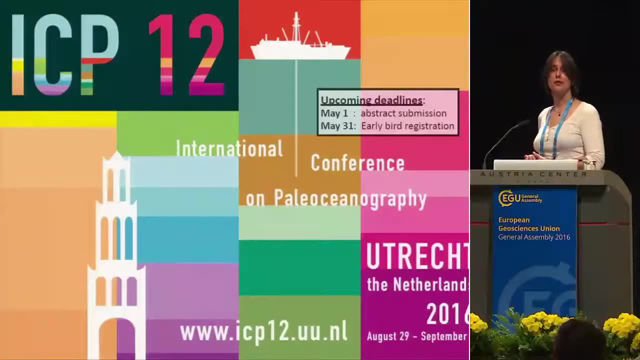 Yes, That's right, That's something we're looking at. That's something we're very interested in as well. Yes, aff impacted very important and an opportunity to mention one more thing: The International Conference on Palaeoceanography will be in Utrecht this year. so for those, 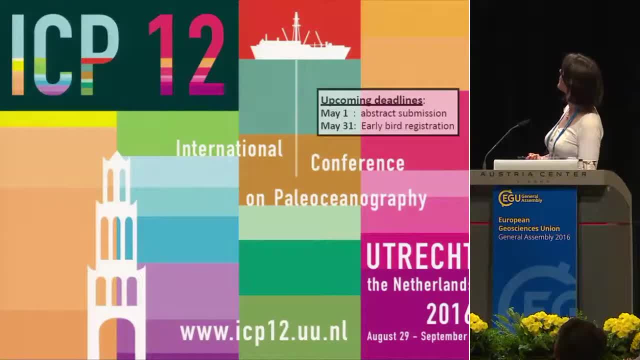 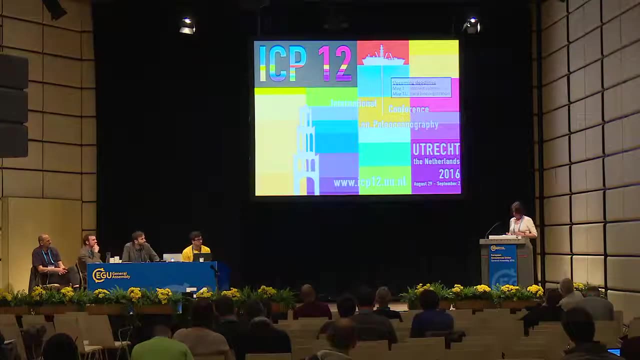 who have not seen that yet, and for those who already know it, this is a reminder. the abstract submission deadline is very close, so we would like to see you all in Utrecht this year. Oh, Oh. 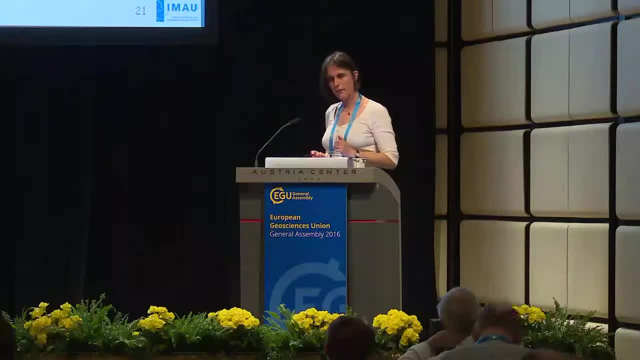 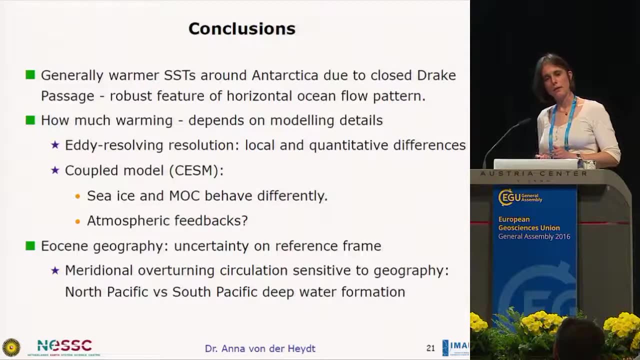 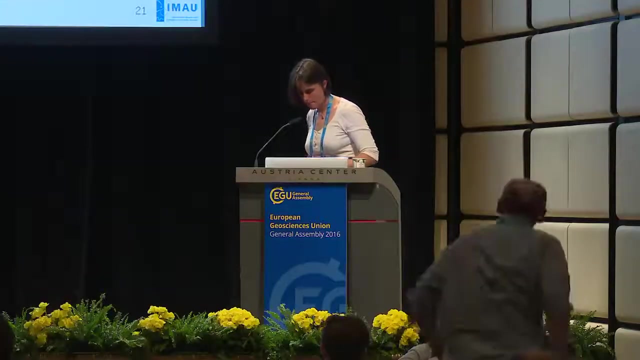 The ocean model simulations were 2,000 years long and the coupled simulations were somewhat shorter, I think around 1,000 years already. yeah, Thank you very much. So next talk is Jean Braun. We'll talk about interactions between the dynamics of solid Earth. 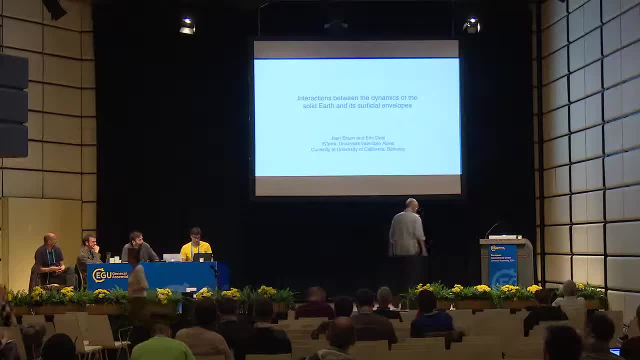 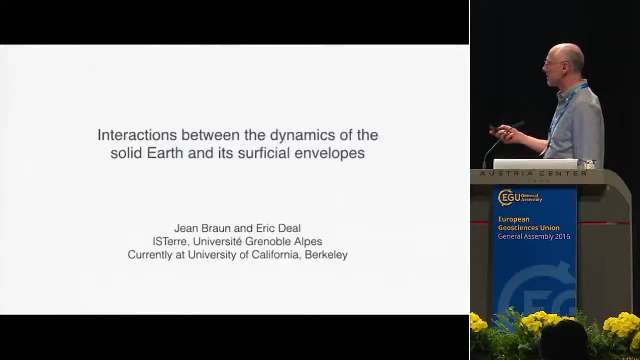 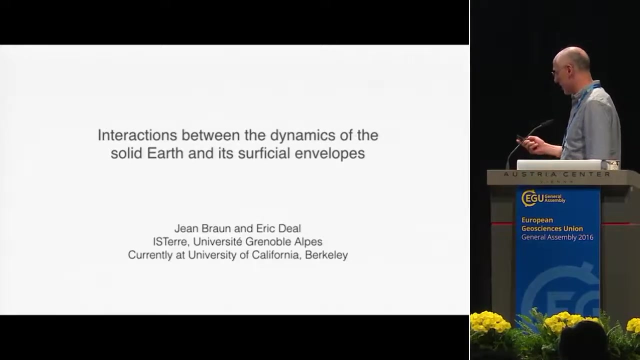 and its superficial envelopes. Good morning and thank you for the invitation. What I want to talk to you today about is Is how the Earth's surface, the solid Earth's surface, may actually be. Its erosion can actually be controlled by the climate of the Earth. 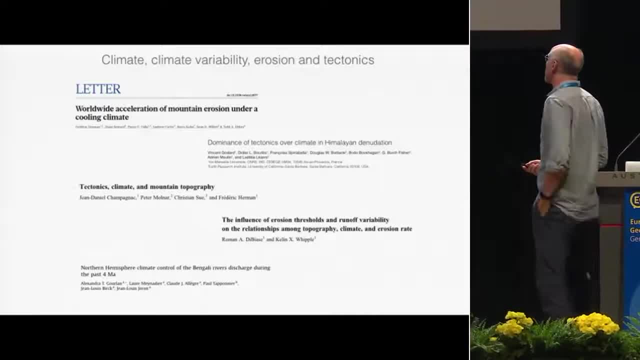 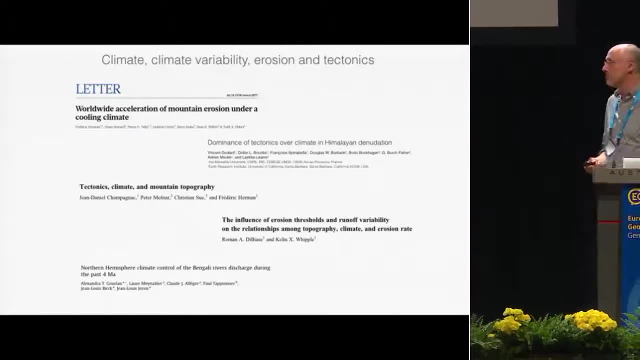 In surface processes. in science, there's been a debate that's been going on for a long time now, where the climate and, in particular, precipitation, play an important role in controlling the rate of erosion at the Earth's surface, And this is obviously important for the Earth's system. 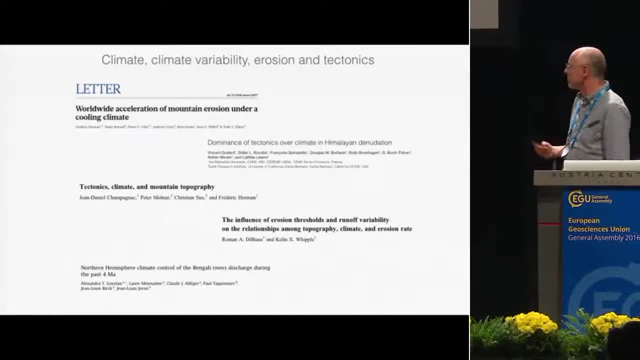 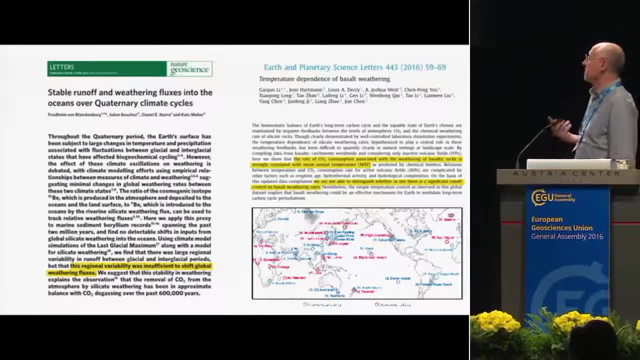 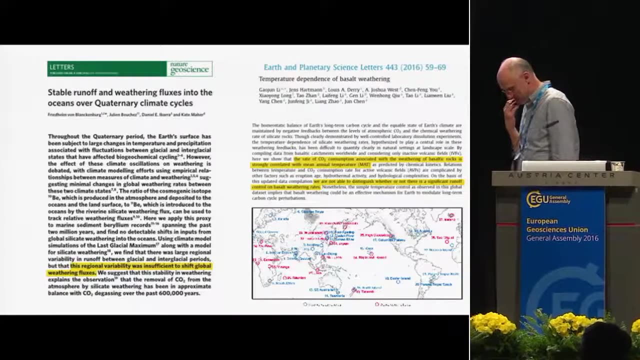 because erosion of the surface will lead, for example, through CO2, the rollback from the atmosphere will potentially lead to a change in climate. So there are very potentially efficient coupling between the solid Earth and the atmosphere that have been investigated a lot. 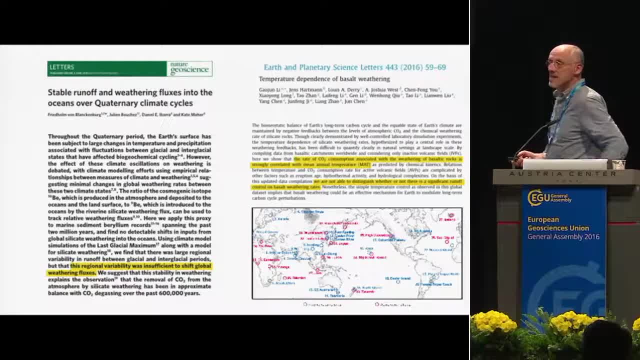 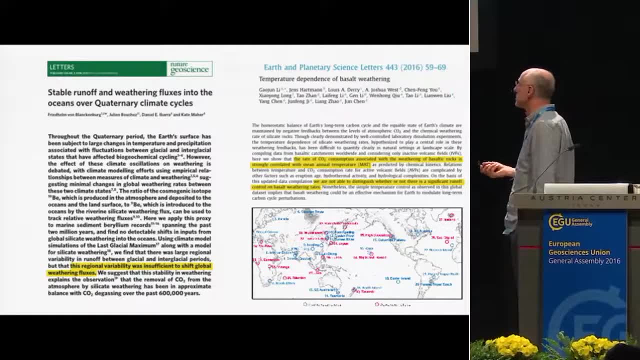 Now the picture is not clear whether these links exist. This is a recent paper by a group at Potsdam and others that showed from observations- and I won't go into the detail of that- that during the last glacial-interglacial change in climate. 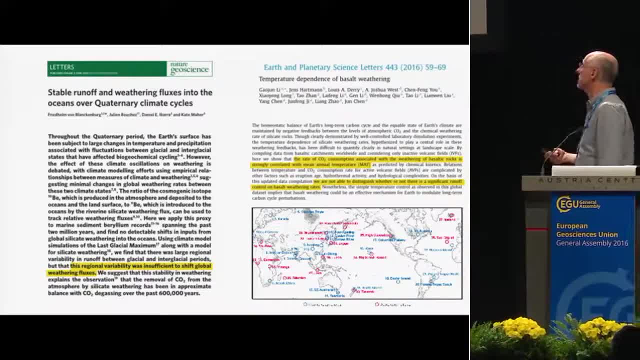 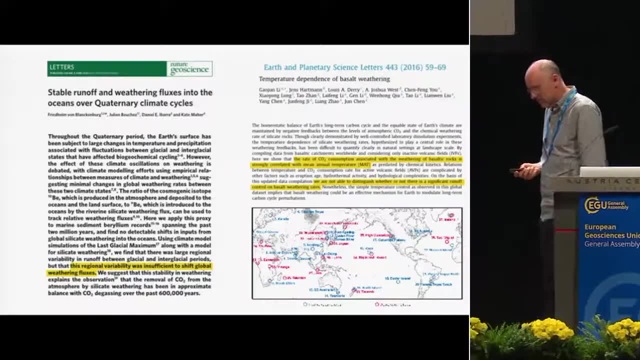 there appears to have been no change in the global weathering and the global erosion of the surface. This is another paper. This is a paper that. This is a paper that. This is a paper that came out very recently that shows that there might be a very strong control of temperature. 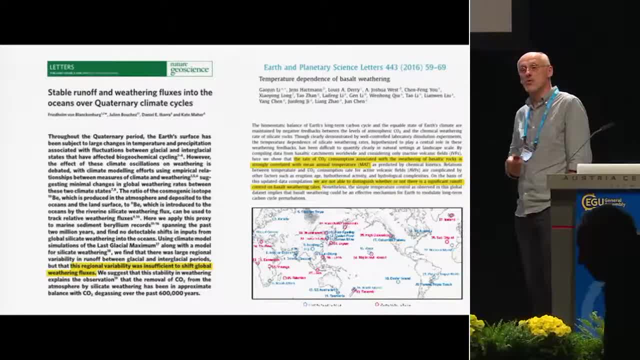 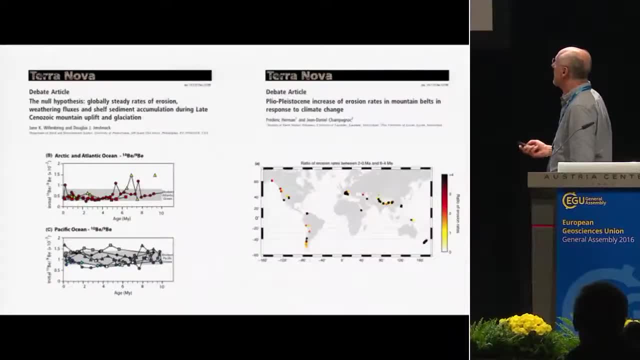 on the geographical variability of erosion or weathering, but there is apparently very little variability associated with precipitation. This is another paper, another set of papers that came out recently in Terra Nova that describe a debate between the two ideas that during the recent cooling of the Earth's climate, 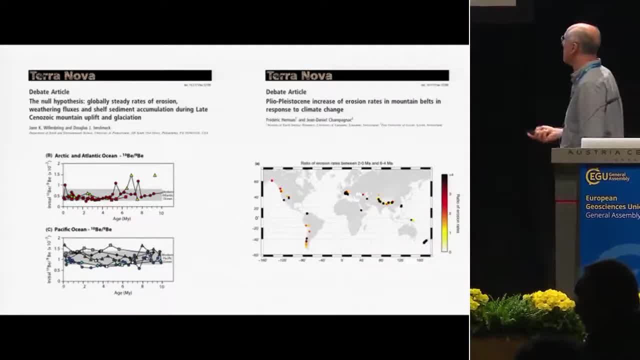 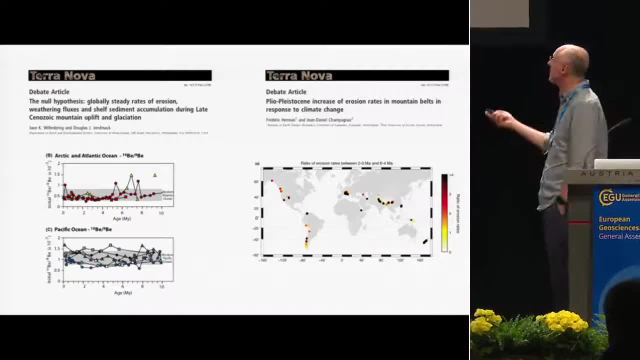 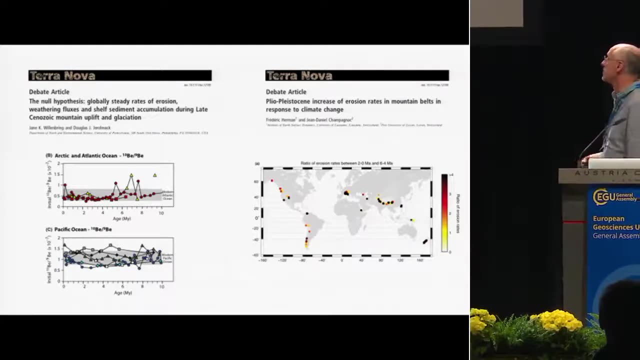 and potentially a change in precipitation and, obviously, temperature. there has been a strong erosional response, especially in mountainous areas that have been eroding much faster, whereas another paper here, another part of the debate, demonstrates from other arguments that there has been no change, no global change. 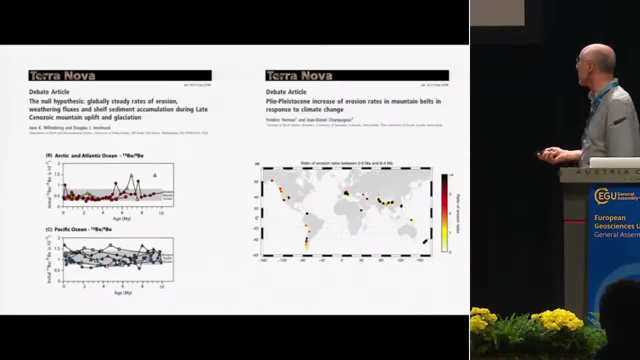 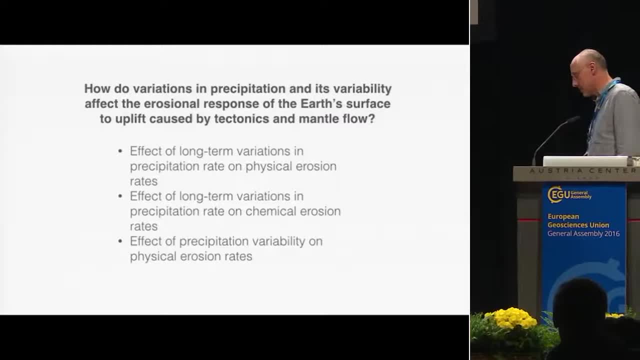 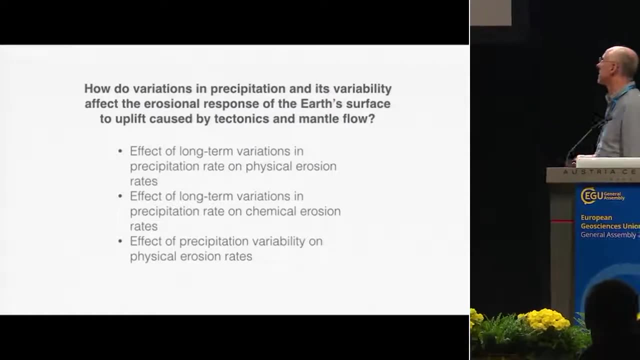 in this chemical or physical erosional flux. So what I want to do today is go through three points, that is, a bit of projects that I have developed with various colleagues in the recent years to look at what from a geomorphologic point of view. 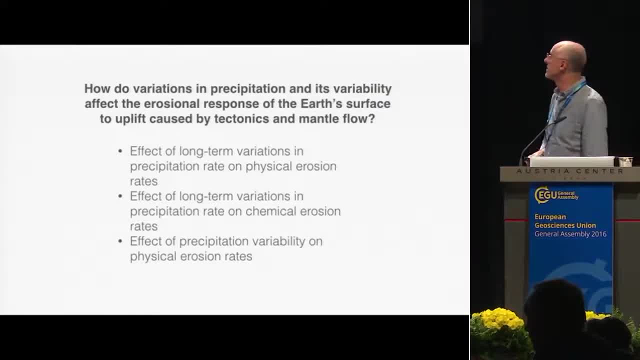 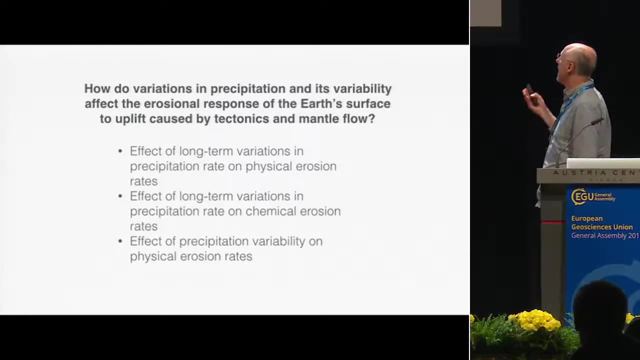 what are the consequences of long-term variations in precipitation rate? first, on physical erosion, that is, the erosion by rivers. second, on the chemical erosion rates, that is, the product or the weathering process. and I will also talk briefly- hopefully I have the time. 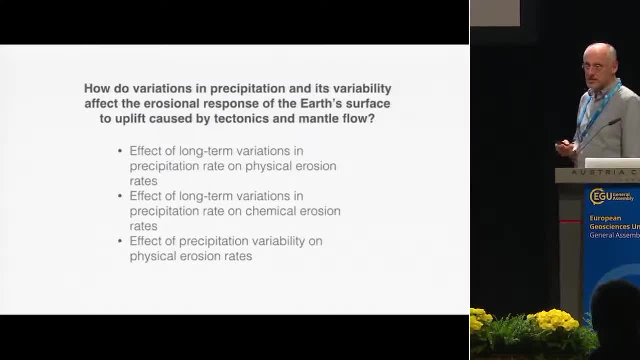 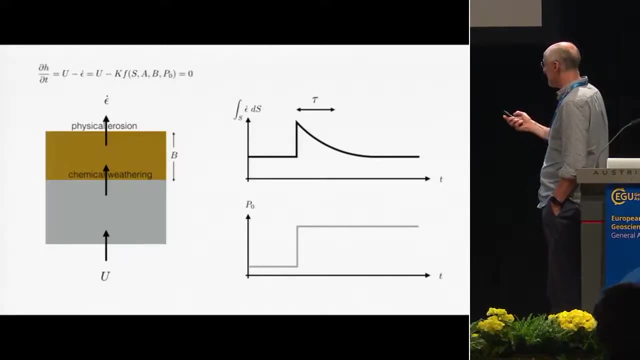 about the effect of variability in precipitation and how the changes in the variability in precipitation- not just the mean precipitation- may also affect long-term physical erosion rate. One point that I want to make before anything else is to note that at the Earth's surface, 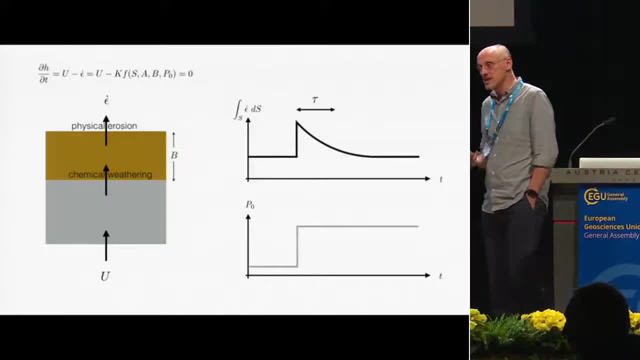 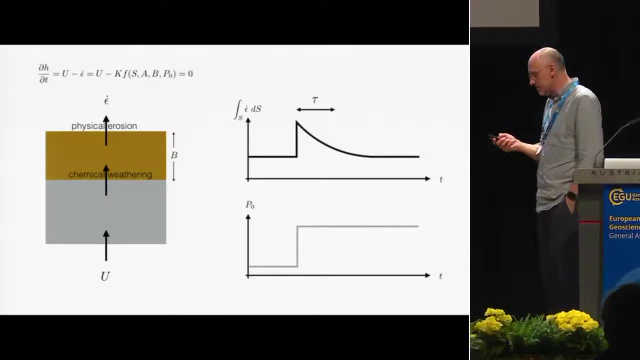 the erosion, whether it's physical or chemical, is mostly in response to uplift by tectonic processes or mantle flow. And that has a very important consequence. that, if you consider, for example, the erosion rate, that if you consider the erosion rate, 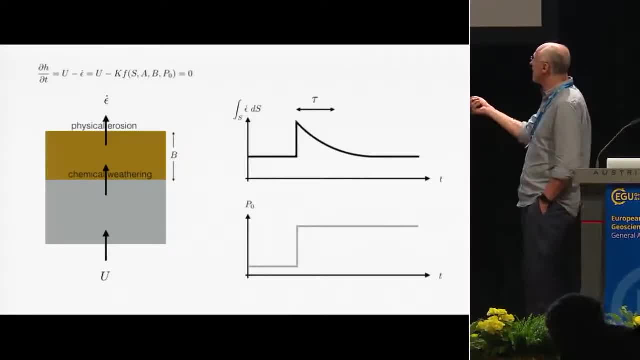 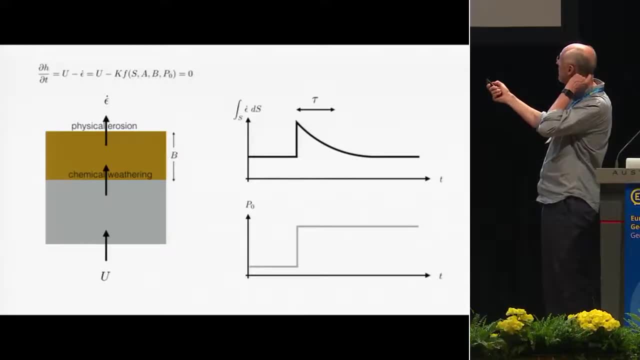 that, if you consider the erosion rate, if you consider a piece of crust here or a piece of Earth that's being uplifted by the tectonics or by the mantle and being physically or chemically eroded at the top, this is a response to that. 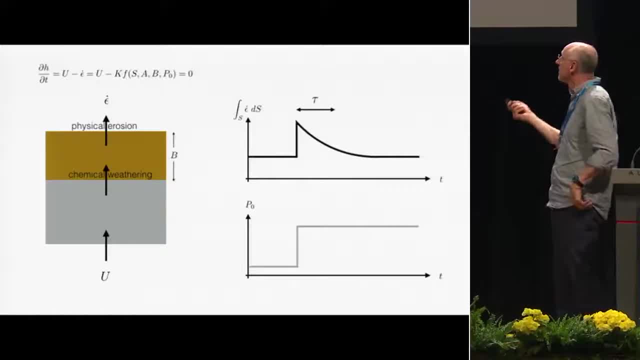 And so almost many places on Earth, or, if you wait long enough, you will get into a steady-state situation, whereas the erosion rate of a mountain or a catchment or even the surface of the Earth had reached some kind of steady-state. that is basically the uplift rate. 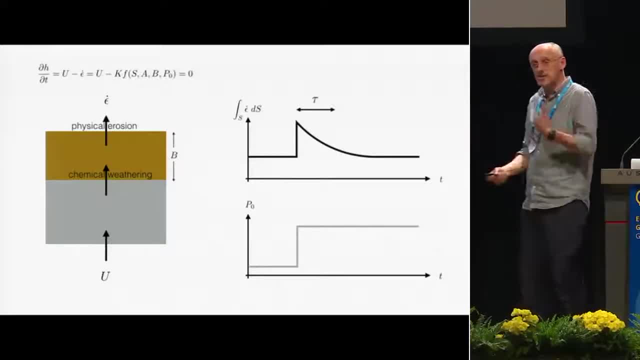 If you change the precipitation rate or any factor that may influence the erosion rate, you will get a response from the system. Maybe if you increase precipitation you will increase erosion rate, But if you wait long enough, even at that very high precipitation rate, 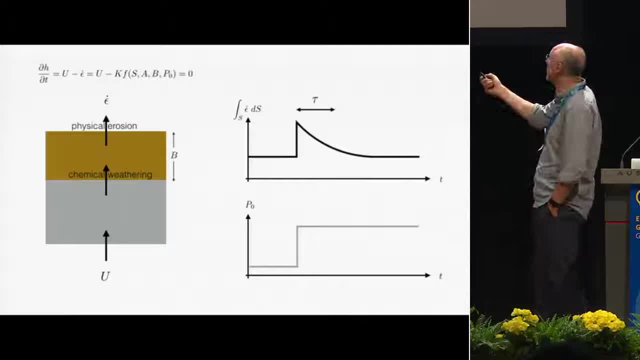 the system will have to go back to its steady-state value, such that again the erosion rate will equal to the uplift rate. You, apart from some very, potentially very special places, you will not change the uplift rate by changing the erosion rate. 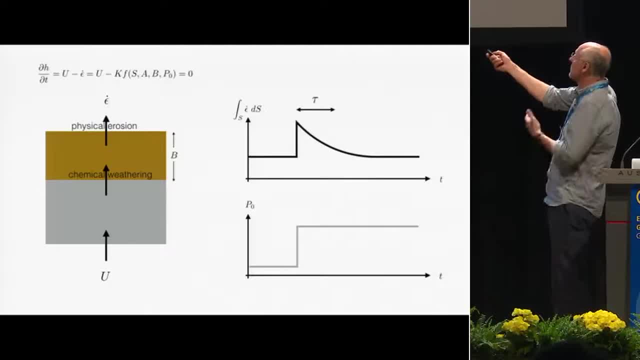 And so the system will adapt it slowly, it will adapt its slope, it will adapt its regular thickness or something like that, but at the end it will go back to its original steady-state. And so what really we should be focusing on is the length in time of that response of the system. 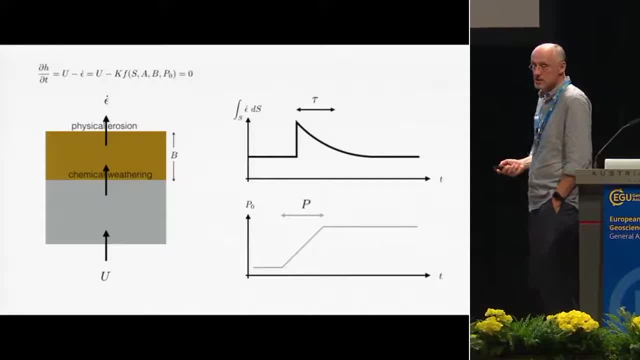 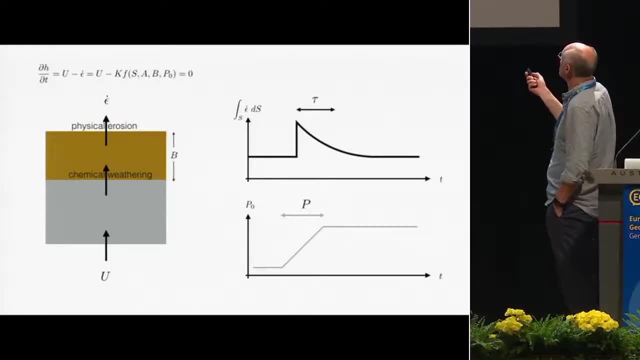 to a perturbation, And you also have to consider that the perturbation might not be of finite length, but has a length or a period, And we see right away that the relationship between the period and the response time is going to be very important. 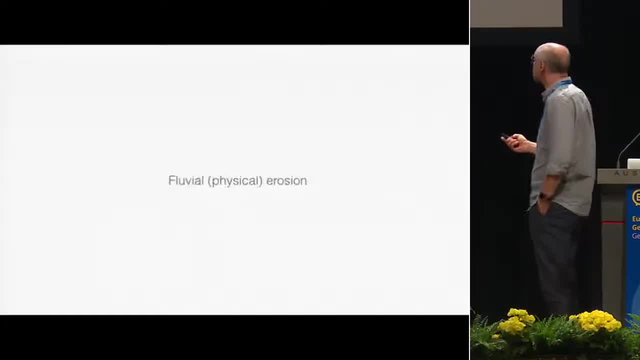 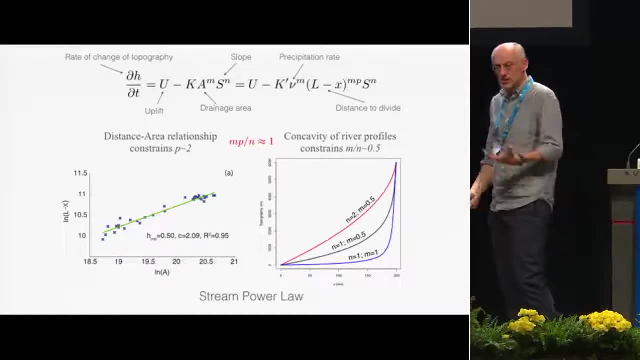 to decide whether or not we have a response and how important it is. Let's move to the fluvial erosion. So this is the classical equation that we use to represent in geomorphology, the erosion by rivers. It says that the rate of change of the surface is the uplift. 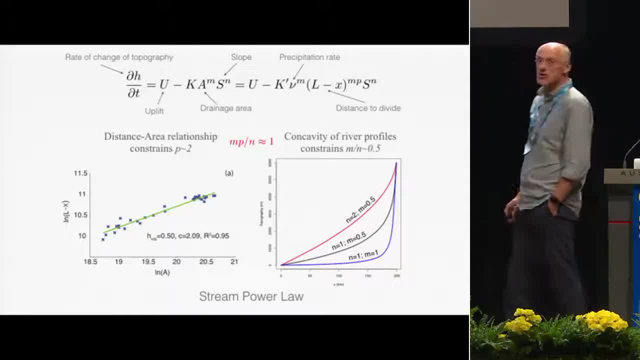 you don't want to forget the uplift rate minus the erosion by the rivers, And that term here is the product of the drainage area, which is a proxy for the discharge of the river, so you can actually express it as some kind of a length. 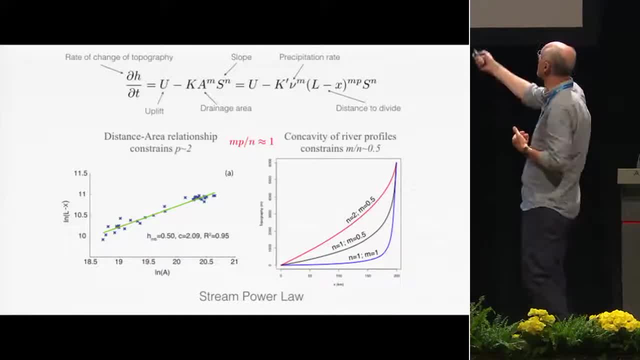 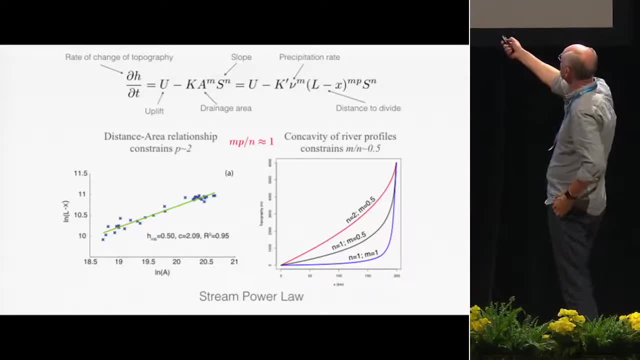 times the mean precipitation rate in the catchment, and then a second term, which is the slope. We don't know the value of k, the coefficient between these geometrical factors and the erosion rate, but we know quite well the ratio of m over m. 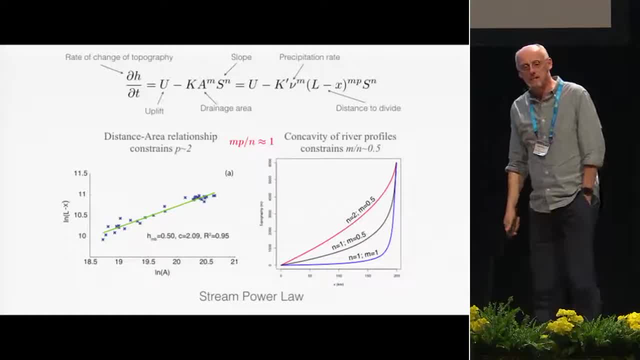 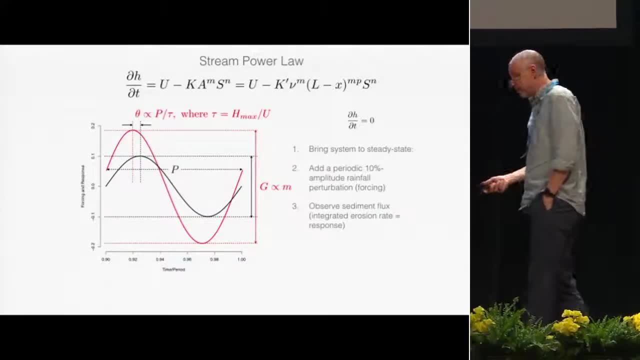 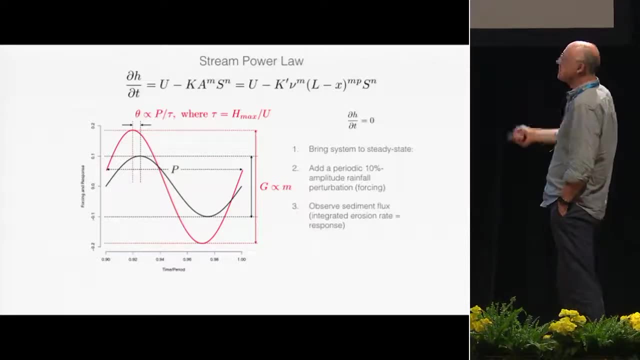 and we know quite well also this other little exponent here, p. The point is that what we can do with this is perturb the solution of that equation, if you want, by imposing a periodic, periodic variation in precipitation rate, And we can compute from this equation. 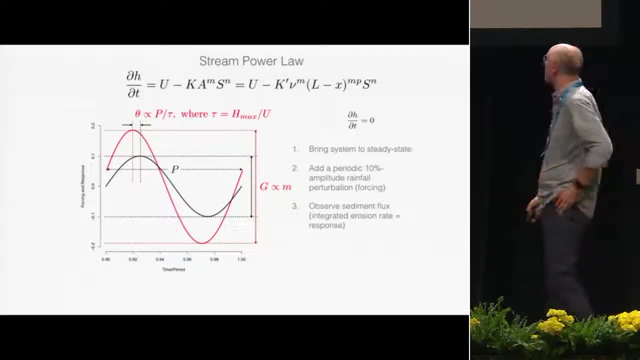 the response of the system to that perturbation in precipitation rate. And what I'm going to focus today is on showing you what the gain is. The gain is defined here as the amplitude of the response divided by the amplitude of the perturbation. So here, if I have a 20% variation in precipitation, 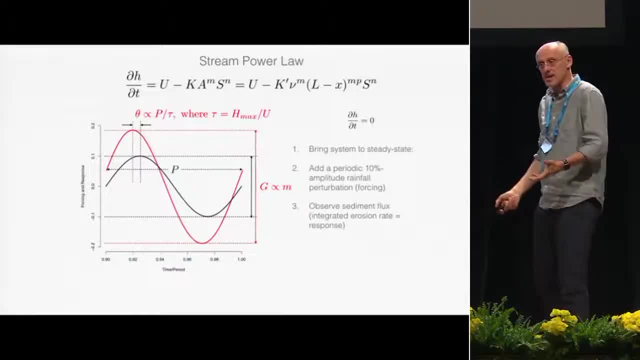 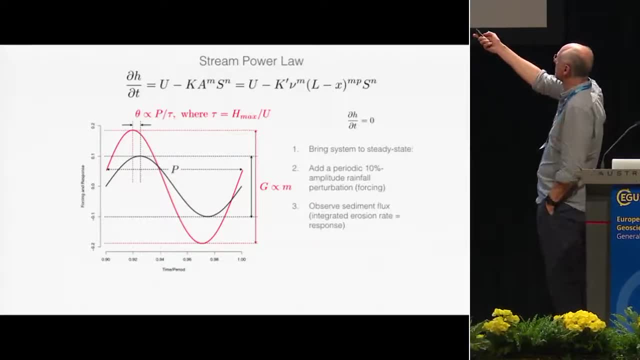 or in precipitation rate, and I get a 20% variation in erosion rate, then I get a gain of one. I can also talk, but I want today to talk about the potential of the creation of a time lag between the forcing and the response. 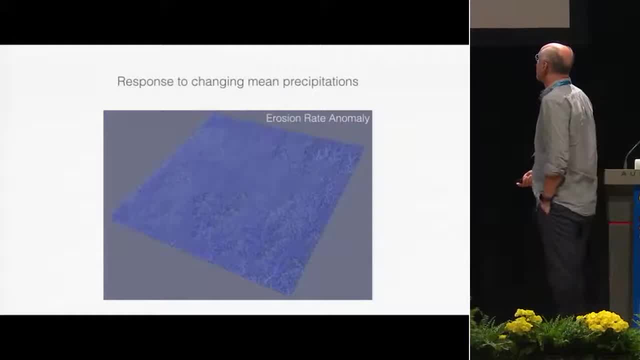 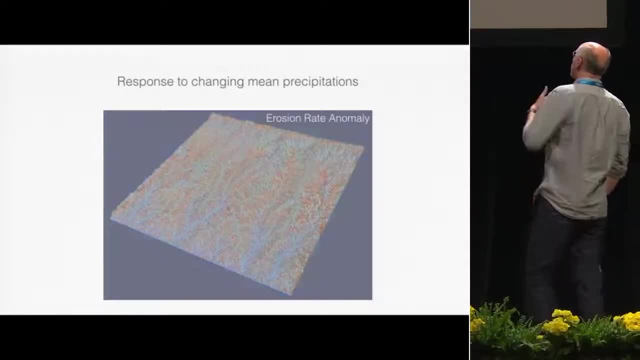 but I don't have the time to talk to you about this today. This is a simulation where we solve this equation in platform on the side of a mountain, And what you see here is what happens in terms of erosion rate in a mountain when you impose a periodic variation. 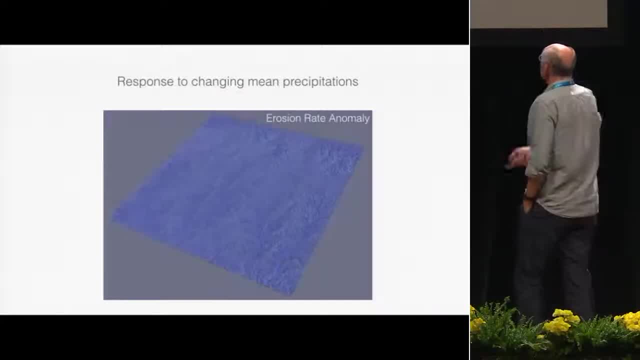 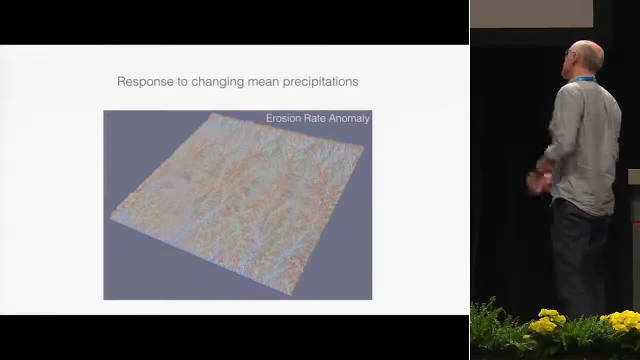 in precipitation rate, And you see here these waves of erosion that go from base level, from the base of the mountain, up the mountain, and it seems a very complex system to analyze. One thing I want you to notice is that all the rivers, regardless of the length, 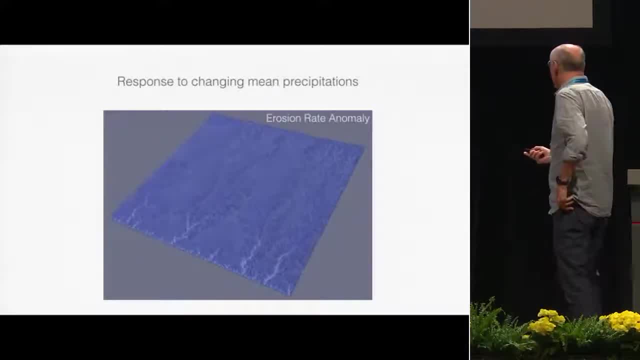 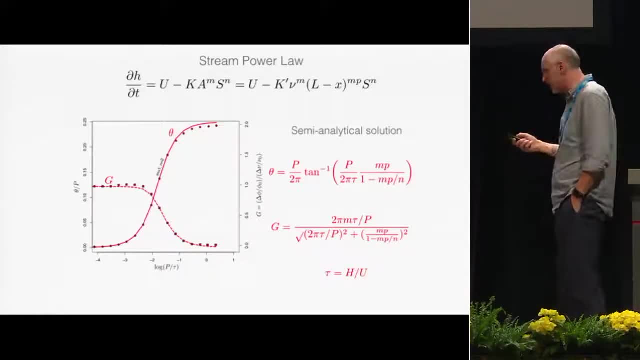 are responding simultaneously, We can actually massage the equation, as I like to say, to show that there is actually an analytical solution, which is shown here, for the gain, between the gain of the forcing versus the response of the system And what is really important. 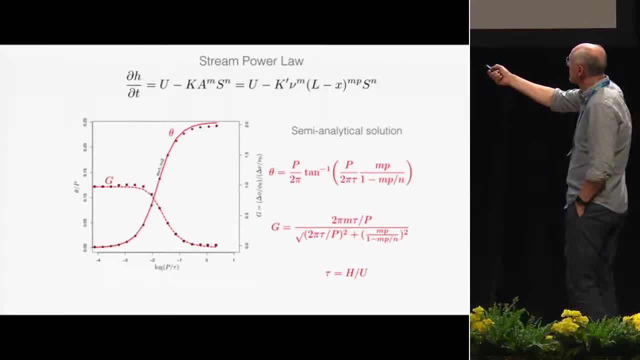 I want you to focus on the shape of this curve here. What I'm putting here is the gain as a function of the period of excitation divided by the response time of the system And, for fluvial erosion, the response time of the system. 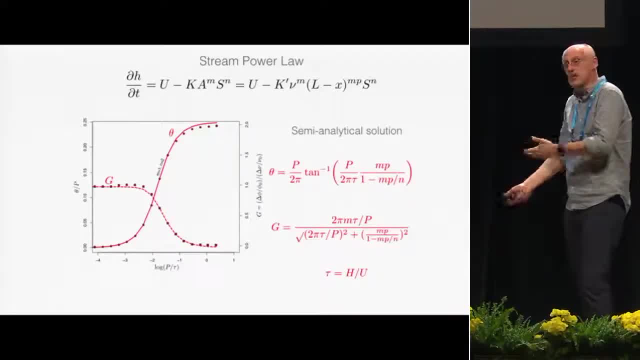 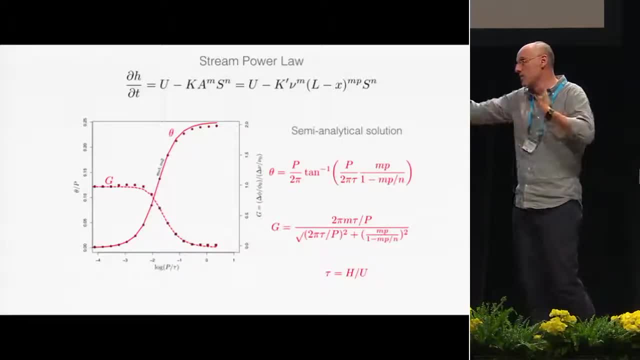 is the height of the mountain divided by the uplift rate or the mean erosion rate, And you see that the response time does not depend on the size or the length of a river or the width of a mountain, only depends on its height and the erosion rate. 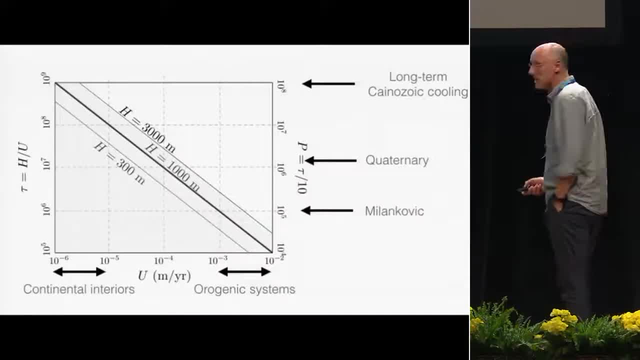 And so what this means, if I translate this in real numbers, that if I look at this characteristic timescale and how it relates to the period of excitation, I can tell from this very simple computation that rivers that are in very fast eroding waves 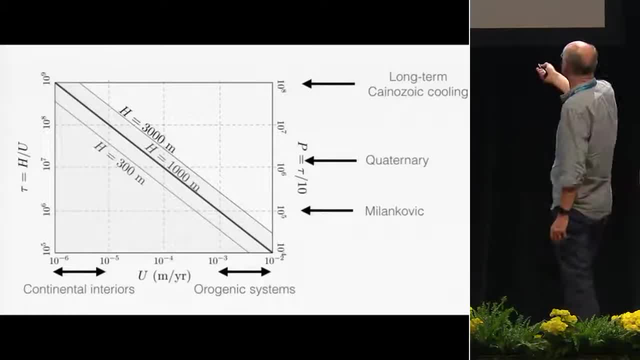 and not lifting areas can only respond to perturbation at a very short period. If you go slower than that, the river will be able all the time to respond to the perturbation and develop a new geometry, so that at the base of the mountain, 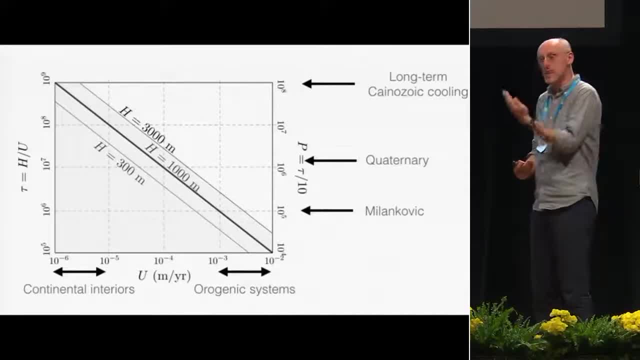 you will not see any change in erosion rate. The system is capable to match the change in shape so that for a given precipitation, the erosion rate doesn't change. If you look at large continental intents in the interior or regions characterized by small uplift rate, 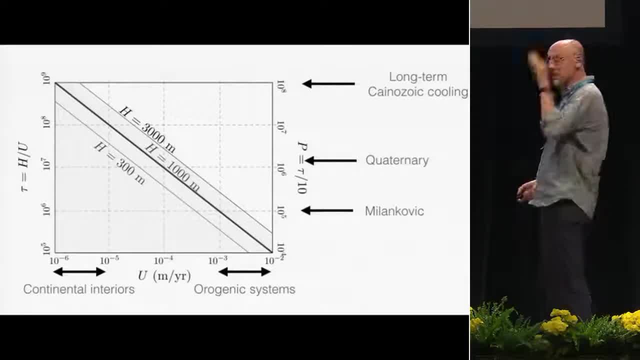 and small erosion rates. they can respond to variation in precipitation. so you will see a change in the sedimentary flux, in the physical erosion rate, at a large range of periods, all the way from the Milankovitch period, let's say. 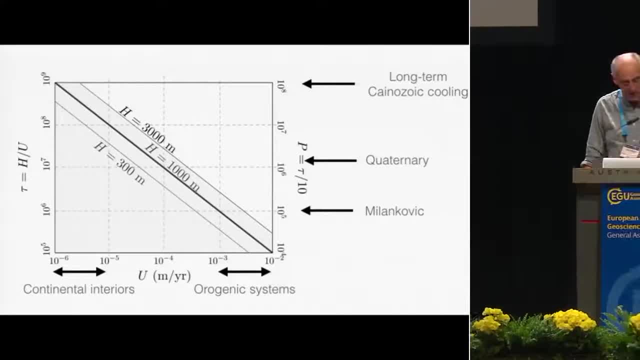 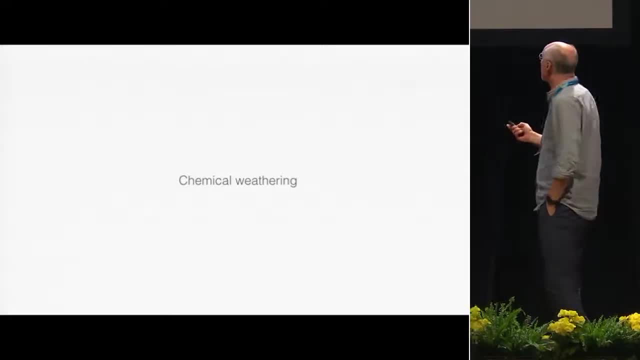 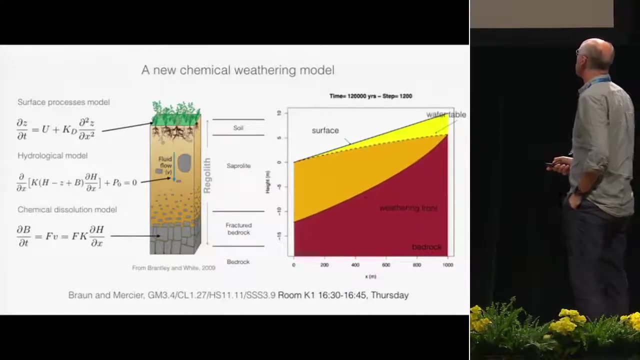 all the way to the very long-term sinusoidal cooling of the climate. Now, in recent months, I've been working on a chemical weathering model which I recently submitted for publication, and it's a very simple but, I think, very interesting model. I will describe if you want to come to another talk. 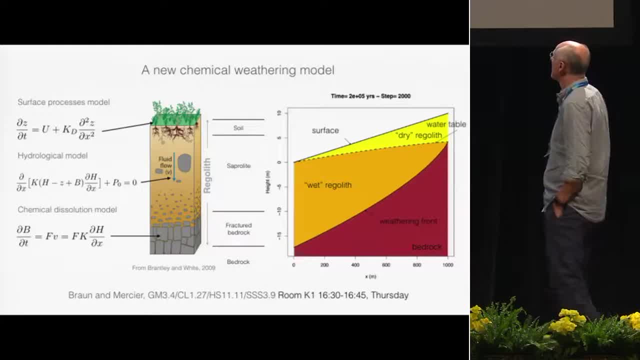 I have tomorrow in room K1. in the late afternoon I'll be able to give you more detail, But the idea is that we have a bedrock, an intact bedrock, that's being pushed by uplift, and through chemical weathering you transform that bedrock into a regolith. 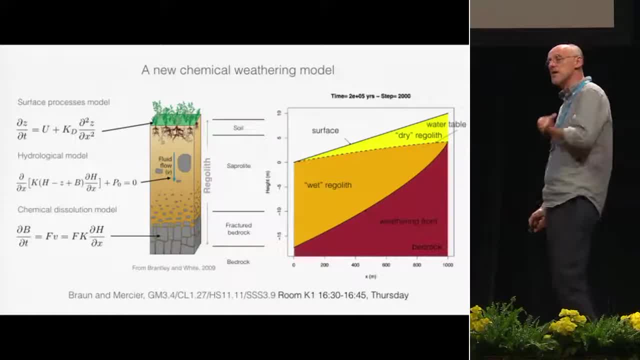 In my model. I assume that the regolith becomes an aquifer so water can flow through it, whereas the bedrock is much more impermeable. I actually say it is totally impermeable. So the regolith has a finite permeability. the bedrock has no permeability. 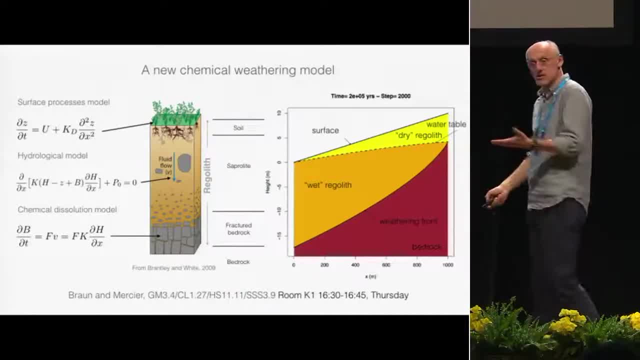 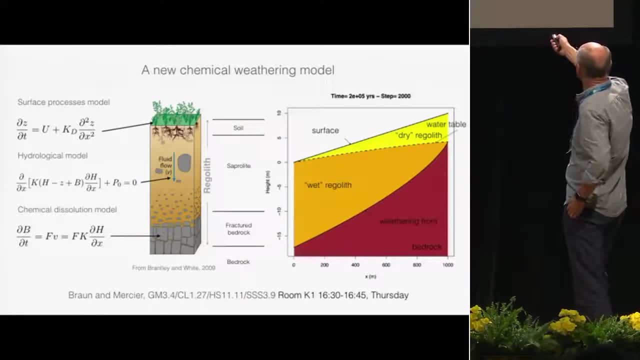 Doing that, I can actually compute. by solving a simple Richard's equation for unsaturated steady state flow in the regolith, I can calculate the geometry of the water table like shown here, And from the geometry of the water table I can calculate the velocity of the fluid. 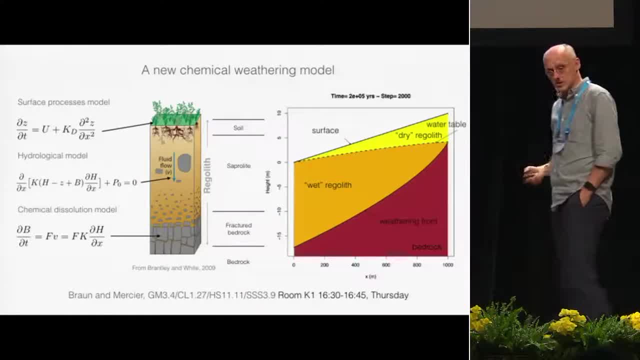 in the regolith. Now there's been a lot of work and I'll show you in a slide in a minute that says that the rate of chemical weathering is controlled by the ability of the system to transport the product of the weathering, the solute. 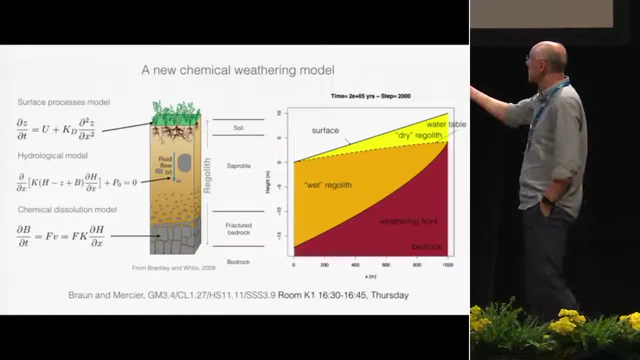 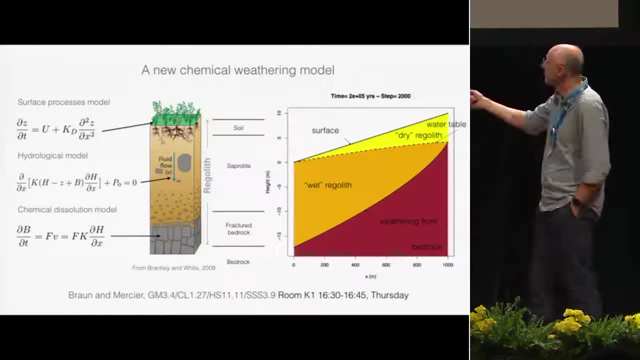 away from the weathering front. And so if you do that assumption, you can show very nicely that the rate of weathering from that vent, the rate of motion of that weathering front, becomes simply a function, a linear function of the velocity of the fluid. 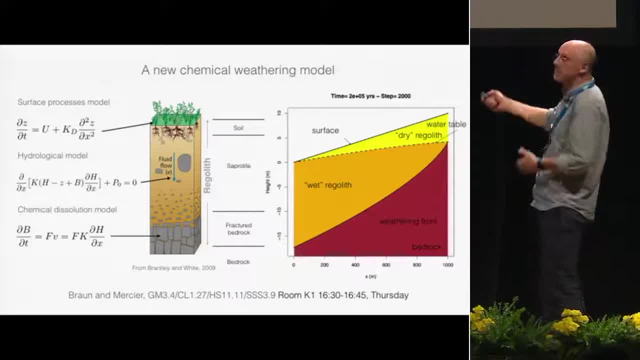 And so you see, this model, although it might be a bit complex, is actually three very simple Richard's equations: One that tells us how the surface is moving through time, a simple erosion, physical erosion model. Here we have a hydrological model that has in here the driving precipitation term. 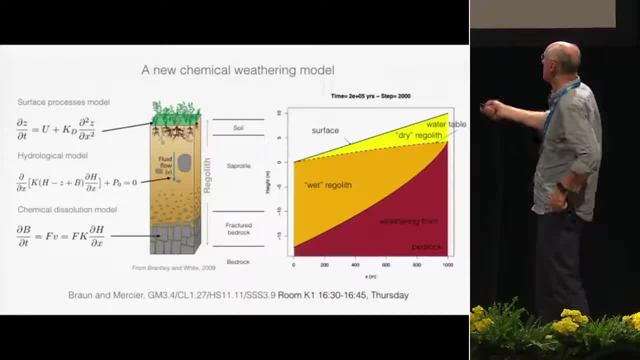 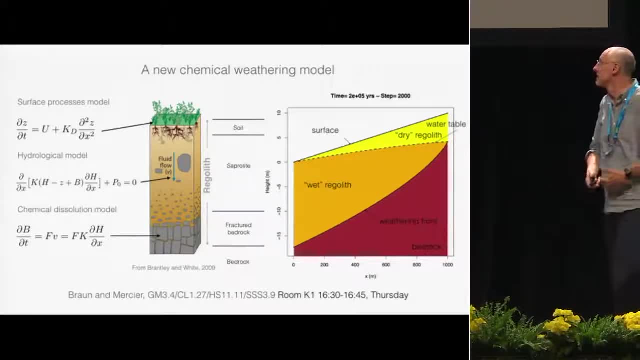 precipitation on the right term, but I'm going to vary, as you expect me to do, from what I told you earlier. And then here we have this chemical solution model, which is a very simple model, and I'll show you on what it is based very briefly. 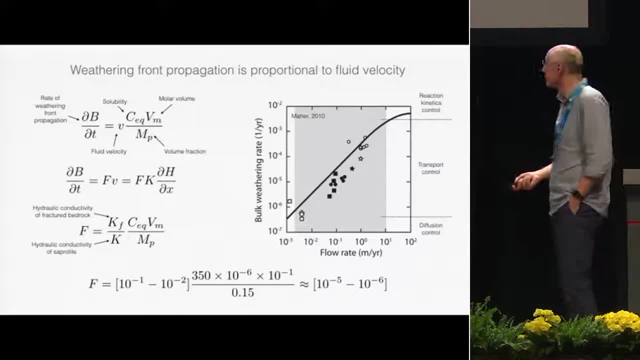 This is based on mostly the work of Kate Mayer, but many others have shown this that show that if you look at the flow rate coming out of a hill that's being weathered, you see that the bulk weathering hand rate of the hill is almost linearly related to the flow rate. 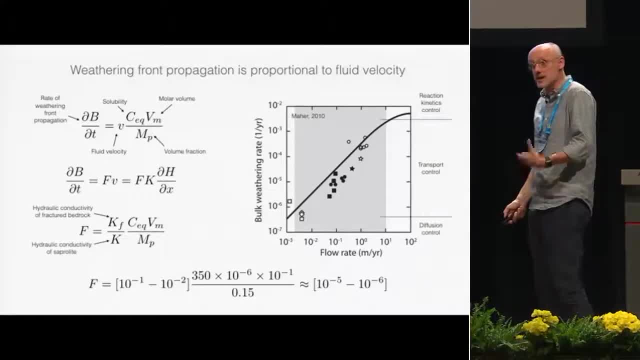 If you've got a very fast flow rate, then maybe the kinetics of reactions might play a role. or if you've got a very, very slow rate, then you have to consider the effect of diffusion of the solute in the fluid. But for a very large range of flow rates, 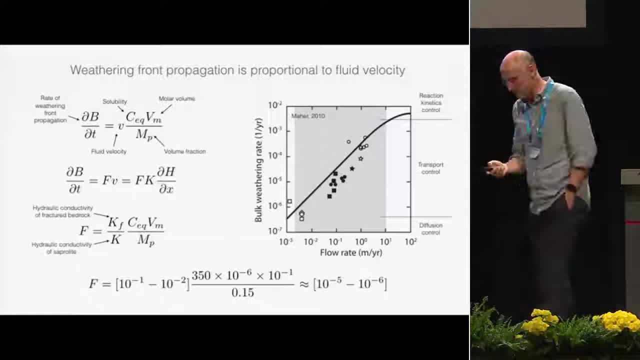 it's really the rate that is controlling the bulk weathering rate and therefore, in the simple formulation, the rate of propagation of the weathering front is the velocity of the fluid times, some constant that you can actually easily measure, one of them being the solubility. 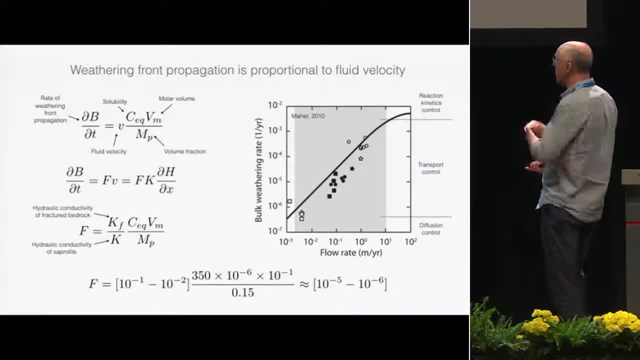 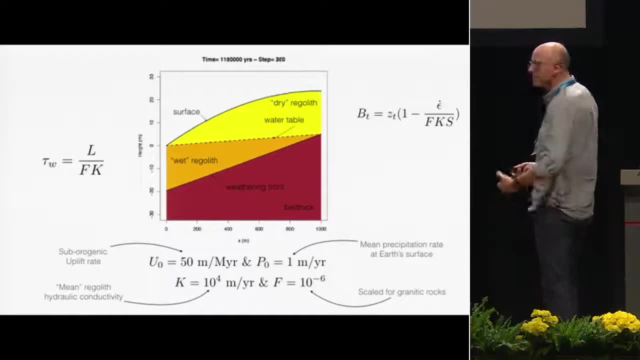 or the steady state concentration of the muon that you're solving through this reaction. So I've developed this model and I've actually played with it. I actually have even a plan form of it. However, I realized that this model is actually very rich in its behavior. 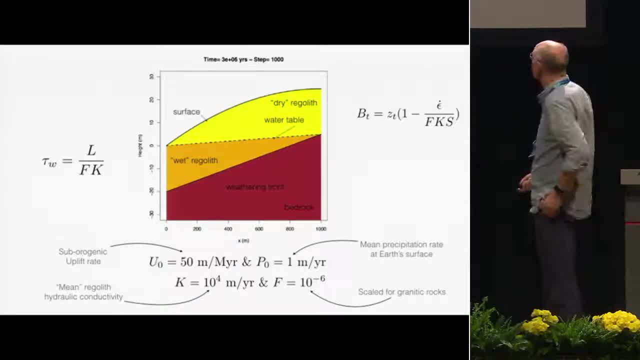 and I've simplified it by looking at 1D profiles to see what happens. And you see- if I think I can play this again- that very rapidly the system developed a thick, or a regular thickness or a regular layer of a few tens of meters and then it reaches steady state. 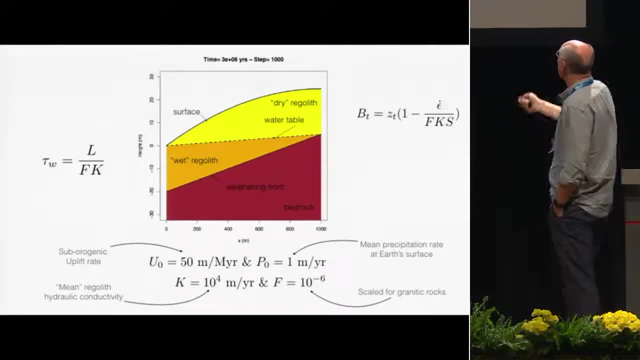 You see, the time is still going on here and the solution goes to steady state. What you also notice is that here, for the set of parameters that I've taken here, it's the uplift rate, the precipitation rate, the hydraulic conductivity and my F factor scale for granitic rocks. 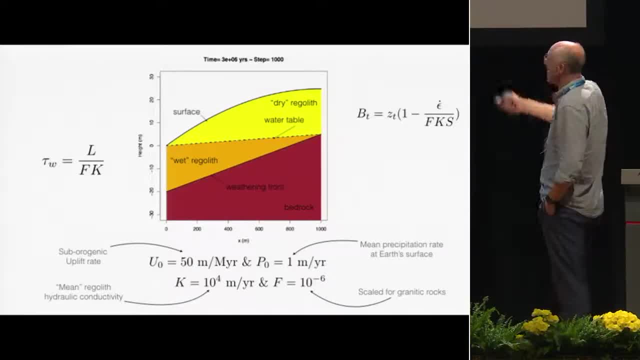 and you see that in that case I predict a regular thickness that's relatively uniform. You see also how the water table at steady state is relatively flat, as well as the base of the weathering front. What's interesting is that you can actually derive an analytical solution. 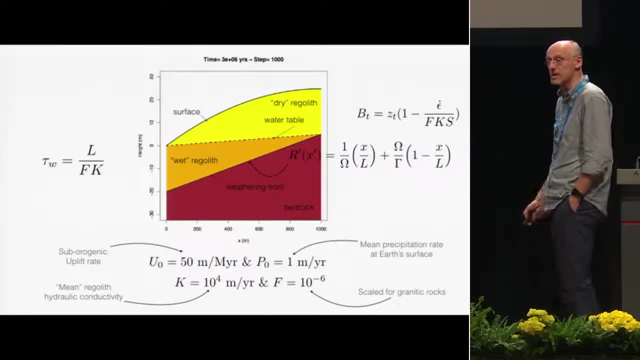 for the shape of the weathering front and the shape of the water table at steady state, And you can show very nicely that it is the product of two functions, one that grows like this and one that grows like that. that one and that one, And it's just the sum of two of these functions. 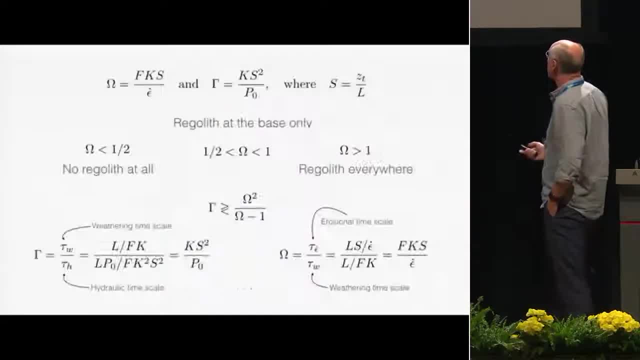 through that are multiplied by some dimensionless numbers. And these two dimensionless numbers are very important and you'll see in a minute why. There is one, we call omega, which has the product of my F factor scale, the hydraulic conductivity, the surface slope and the erosion rate. 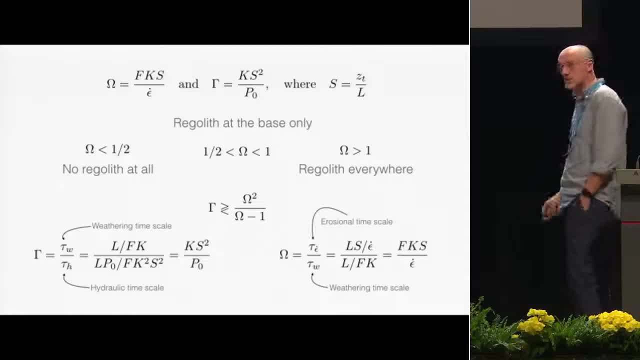 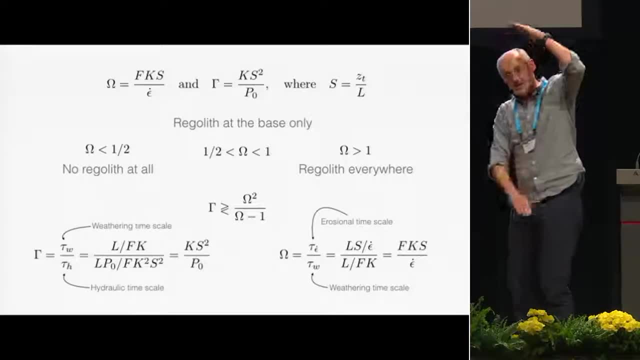 But you can also show that omega is in fact the ratio of two time scales. It's the ratio of the erosional time scale by the weathering time scale, And omega really controls the thickness of the regolith If you erode too fast. 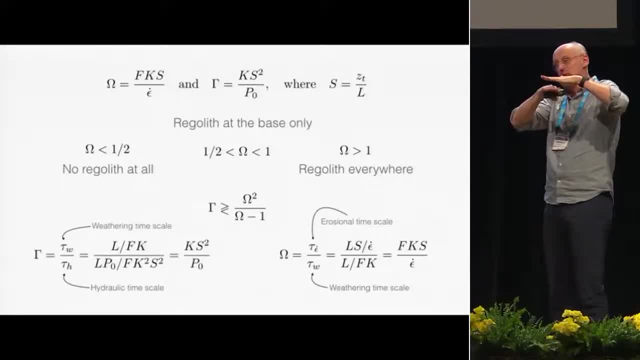 and you cannot weather fast enough, you get a very thin regolith thickness. Even if you erode very fast, you might have no regolith thickness. This happens when omega is smaller than one. there is little or no regolith thickness For omega larger than one. 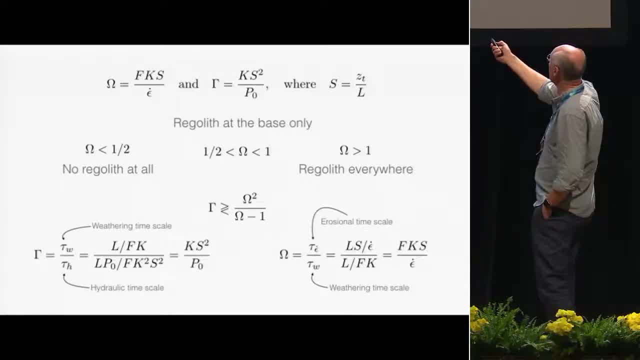 you have regolith everywhere from top of the landscape. The other dimensionless number is gamma. factor is the product of k. hydraulic conductivity times the square of the slope and you see slope becomes very important here- divided by the precipitation rate And you can show again. 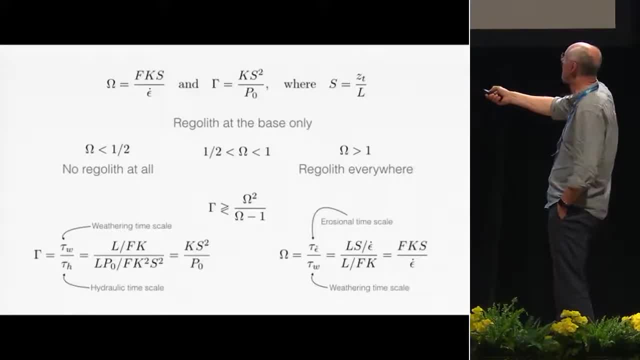 that gamma is the ratio of two time scales: the weathering time scale and then what I call the hydraulic time scale, the time it takes for the water table to adjust to any change in its geometry, or the geometry of the regolith, And you can show. 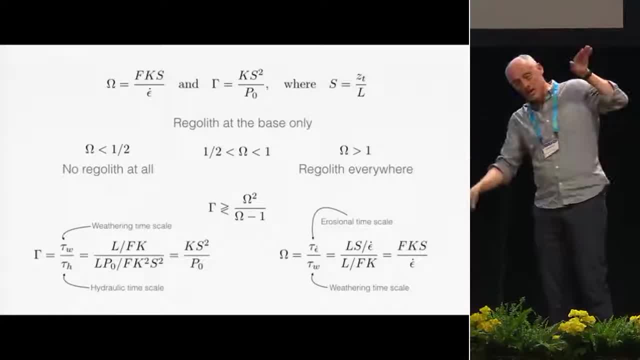 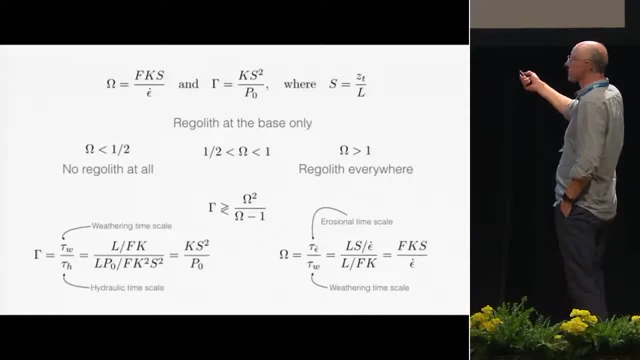 that gamma controls the geometry, whether it is thicker at the base of the hill or thicker at the top of the hill, And the condition is that gamma larger than omega square over omega minus one gives you thicker regolith at the top of the hill and dives lower. 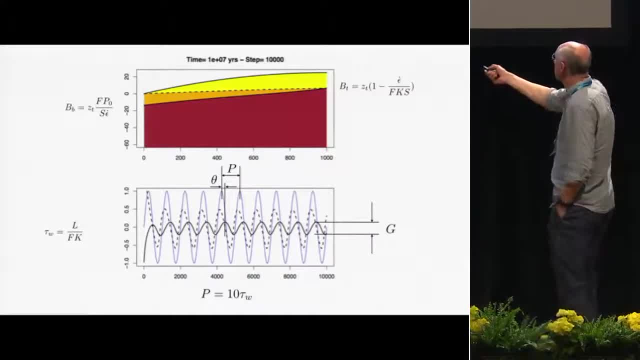 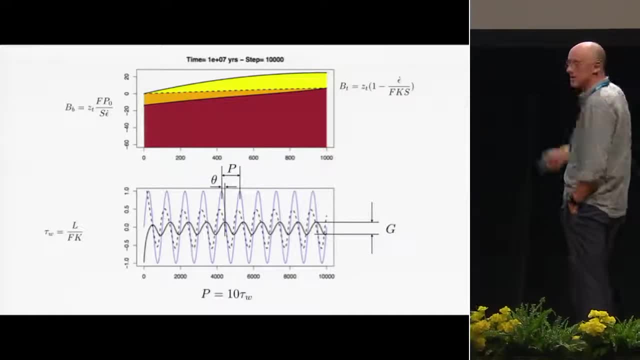 So what you can do is take such a model and perturb it by varying the precipitation rate at a given period and see again here: this is the thickness of the regolith and this is the mean thickness of the regolith layer, and this is the mean weathering rate. 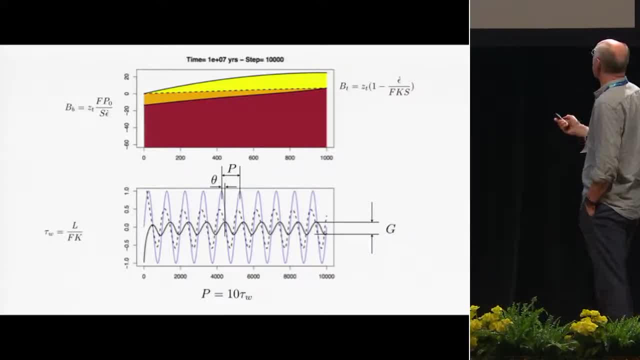 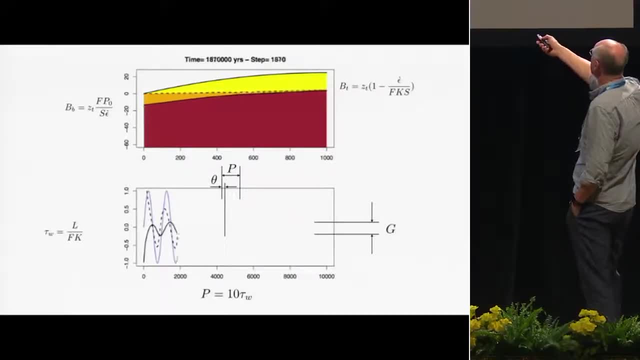 to achieve the regolith layer. So I want to show you- there is a little animation here which shows you how the solution evolves through time, and you see that it is not really simple, because there are two things happening. you have the base of the weathering layer. 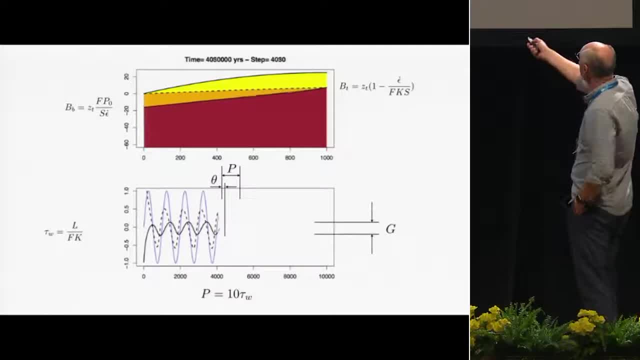 that is actually trying to adjust to the change in precipitation, but the water table is also changing to variation in precipitation and the two have to combine because the velocity of the fluid, which depends on the water table geometry, controls the rate of propagation of the weathering. 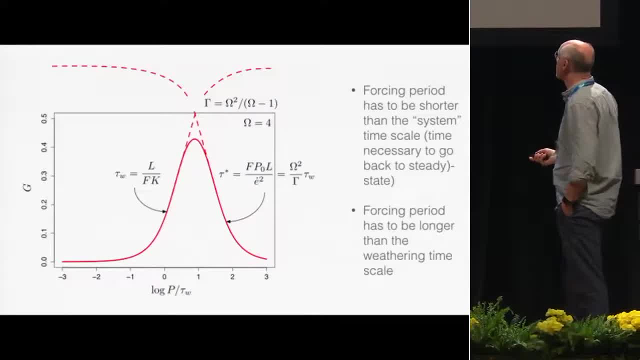 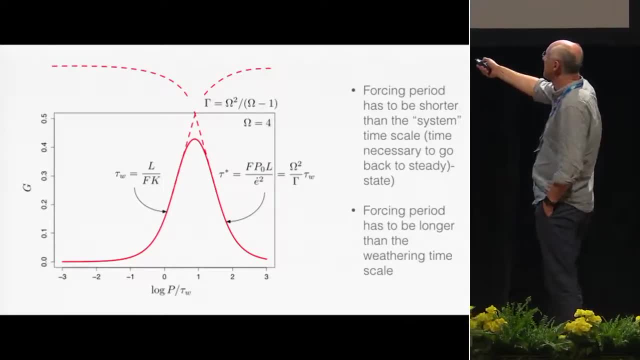 It is interesting that you can actually find again an analytical solution for the gain as a function of the forcing period, and what you see is that it is really the weathering timescale that controls the response of this system. So if you are close to ten times, 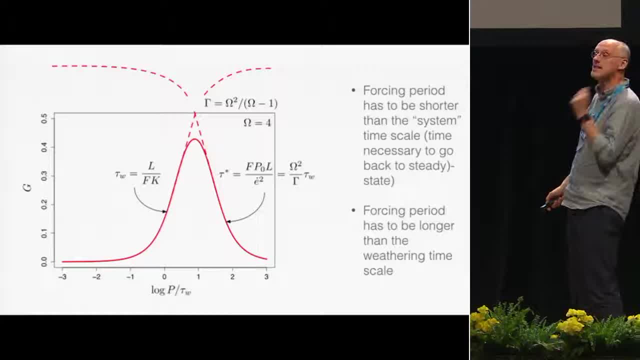 the weathering timescale. if you force the system at ten times the weathering timescale, you have got a really big gain. And I remind you, the weathering timescale is L over FK. L is the size of the hill or the object that is being weathered. 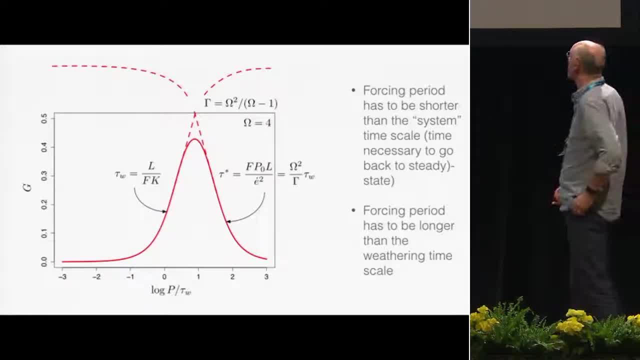 F is the chemical factor and K is the hydraulic conductivity. But what is interesting here, which is different from the fluvial erosion, is that we not only get one curve like this, but we get two curves, which means that there is a very narrow range or period of excitation. 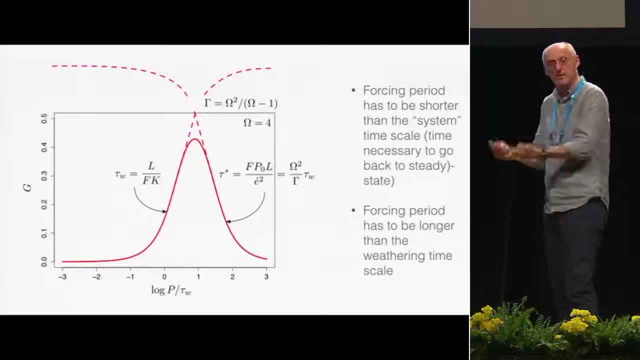 over which you will not actually see a response from the chemical factor. If you go a shorter period than that, the weathering doesn't kick in, it doesn't have the time to respond to short changes in precipitation. if you go too slowly, if you change it very slowly, 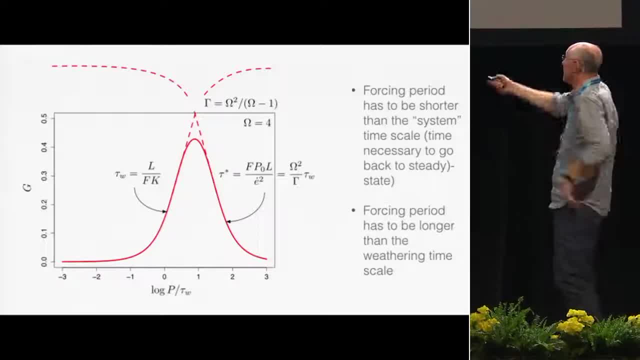 the system will always adjust and will always be at steady state and there will be no signal coming out of the system. Note that TW is mostly a function of length. this other timescale that controls that branch here is the same timescale multiplied by a combination. 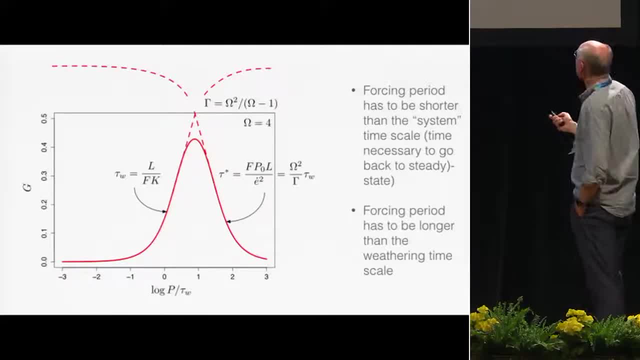 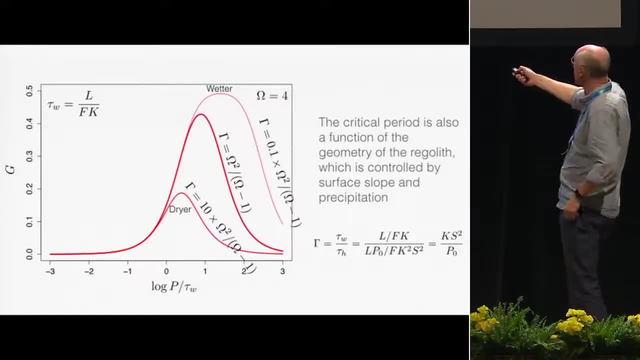 of my dimension and this number and you can show that if, for example, you change the gamma factor, which is similar to making it wetter or drier, you don't change that branch, you only change that branch. so you make it narrower or larger the range over which 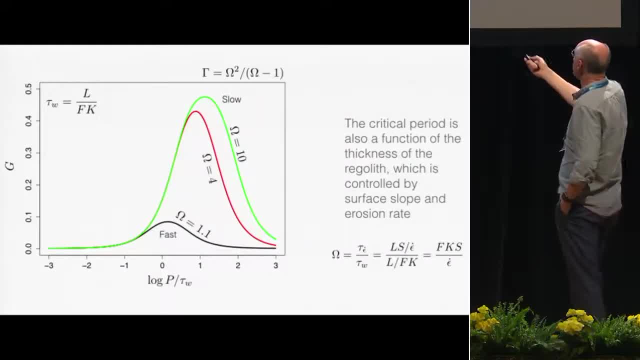 but it remains the range. If you change omega now by making it smaller and larger, you can actually be to a case here. when you get to omega equals one, there is no regular thickness and then obviously there is no response. but again, you see that the position 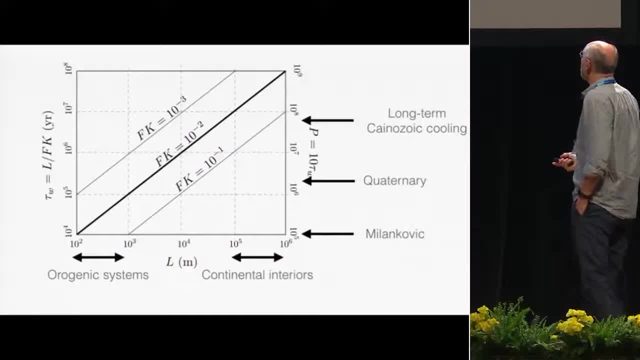 is mostly controlled by that weathering timescale, and so again we can go back to the diagram, and here it's a range, it's not a half space, which means that if the model I show you is correct- and this is a big assumption, but, as you see, 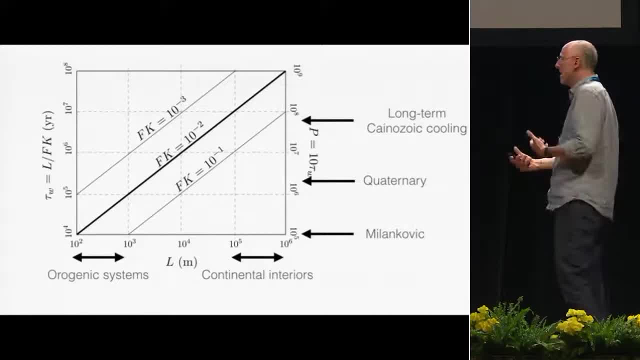 the model is based on very simple physical principles that we kind of all agree on. it's just that I put them together and if we look at that, we see that at Milankovitch cycles- so your 10 to 100,000 years- it's mostly origin existence scale. 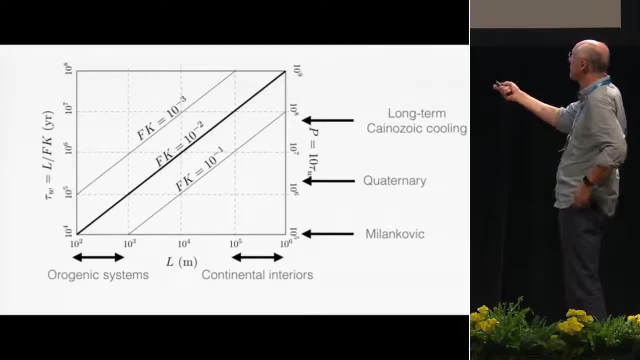 so the small catchment in the top of mountains that are going to be responsive. if you go all the way up to the tens, to hundreds of millions of years, it's only the continental interiors, thousands of kilometers aquifers, which will be able to respond to that. 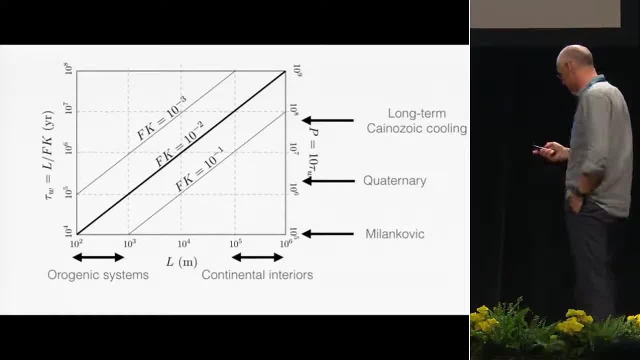 and in the middle you have all the other possibilities. so I think, more than anything, I think it's really important to realize that the period in which you're going to change the precipitation and, I think, in general, the forcing into your natural system, is very important to actually determine. 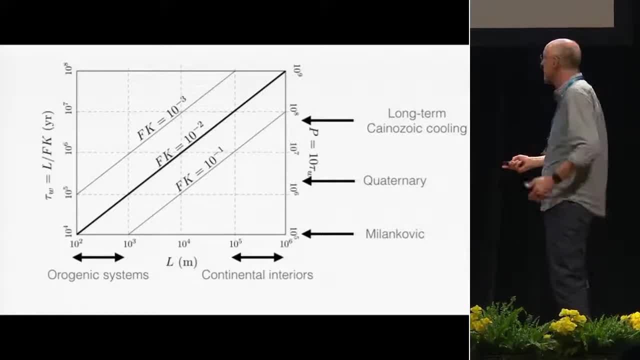 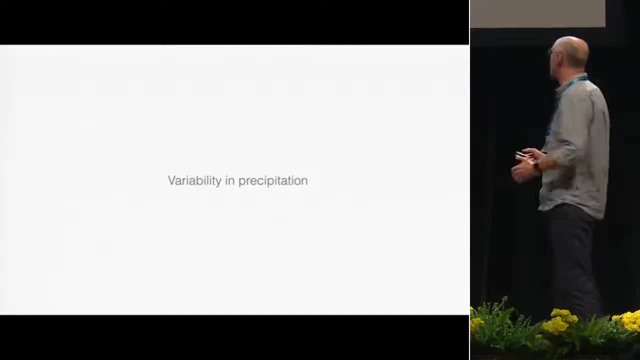 whether there will be a response or not, or the amplitude of that response. so I'll finish by moving to something slightly different, which might make things even more complicated, but this is a work of one of my PhD students, Eric Diehl, and I think this is also very important. 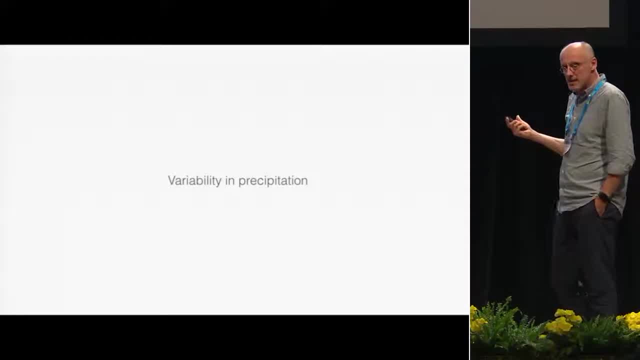 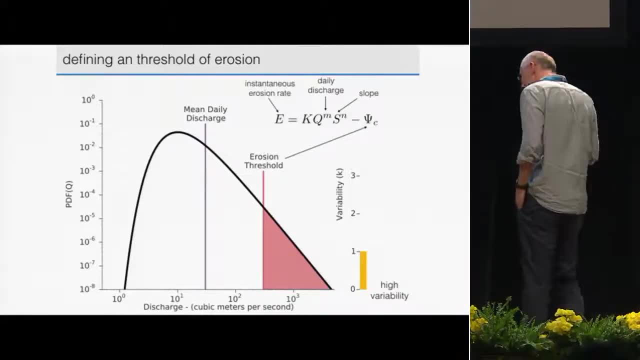 and we are not the first to say it, but all I've been telling you so far is that what happens when we change the mean precipitation, and we know in geomorphology that the variability in discharge of a river makes a big difference on how much it can erode. 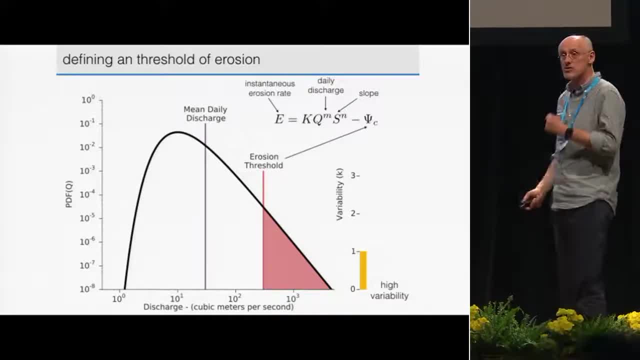 and this is because we believe that there are erosional pressures in the river, for example, and that means that only the large discharge events. this is a PDF: a probability density function of discharge, which is a proportion of a given discharge or the likelihood of a given discharge. 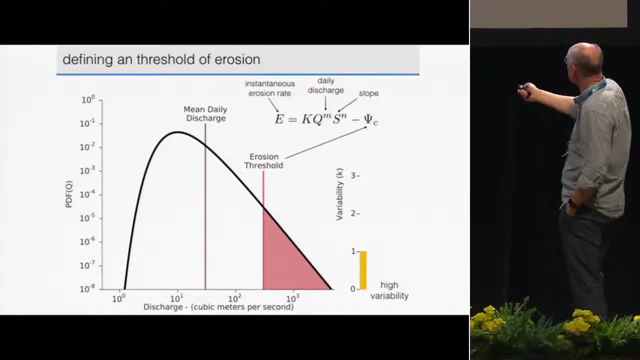 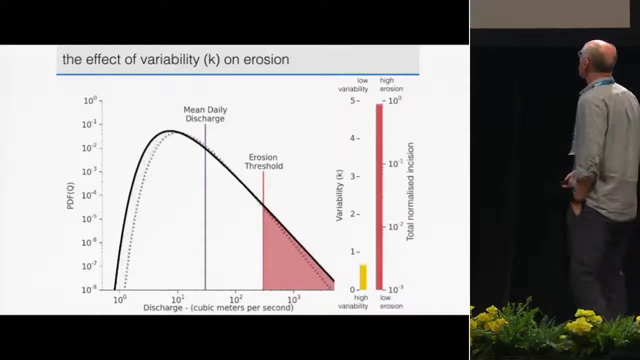 happening in a given river and if there is this threshold, it means that only the big discharge events will actually produce erosion. so the mean erosion of your river, which has this characteristic distribution of discharge, is the pink area here, and what I'm showing you here is a series of these distributions. 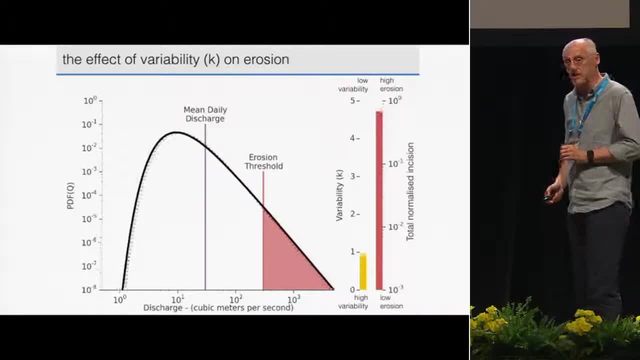 that all have the same mean precipitation or the same mean discharge in this case. but the variability changes and especially the slope of that tail here, and what you can see is that the area here which is this bar here can get really, really large when you have a big tail. 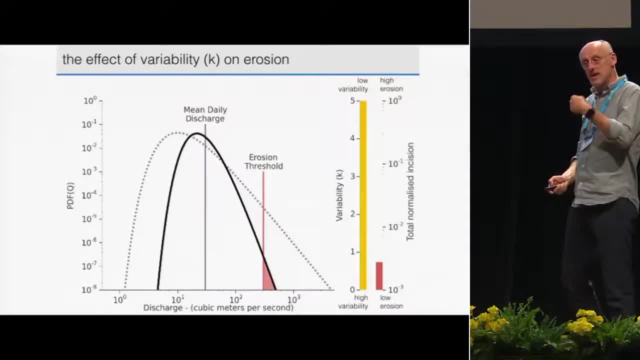 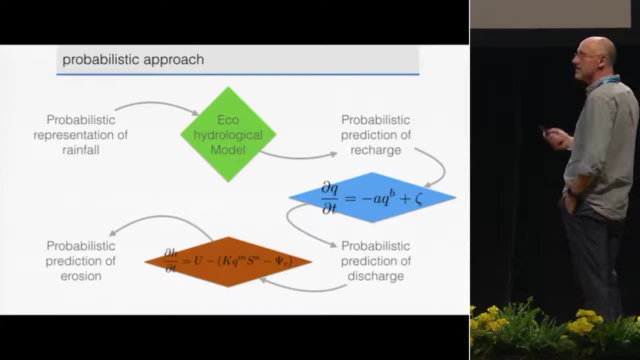 and very, very small when you have a small tail. so the high discharge events are very important. so with Eric, we've been again combining ideas and models from others, but we've actually done this in a purely probabilistic approach. so what we do is we take a probability, probability. 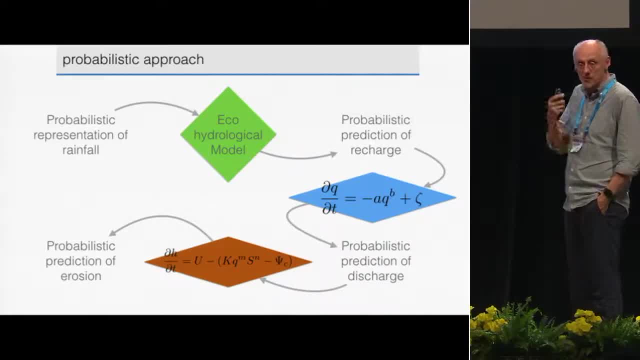 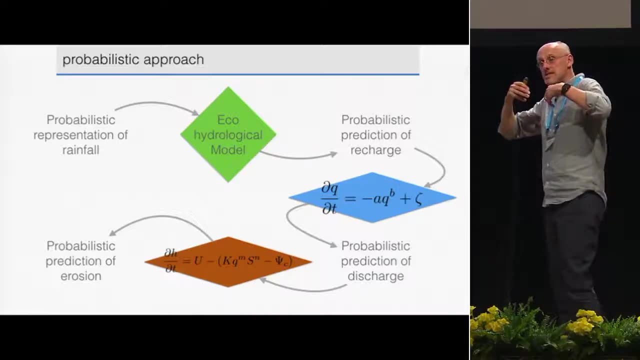 representation of rainfall, a density distribution function of rainfall events, and we feed it into what we call an eco-hydrological model that has been developed by us and by someone else that gives us, from that probability density representation of rainfall, a probabilistic representation of the recharge. 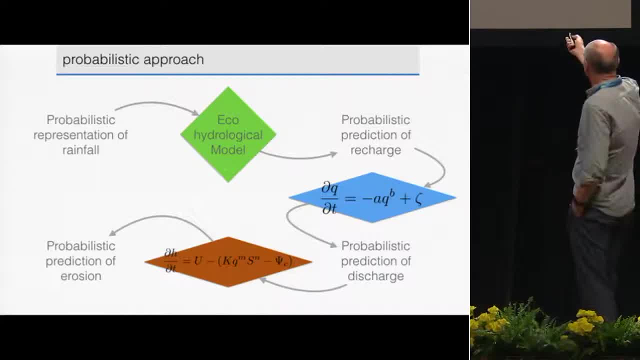 of the water that gets into the river, knowing that we can use a simple differential equation that tells you how the discharge of a river varies through time for a given discharge, and we can produce a probabilistic prediction or probabilistic distribution of discharge, which we can then feed. 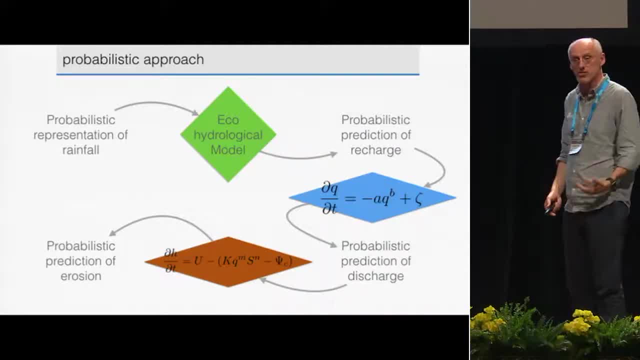 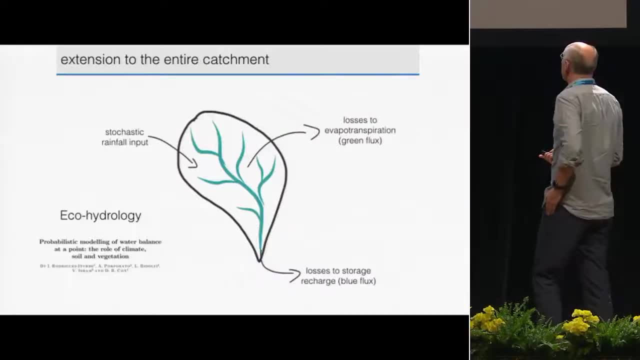 into an erosional model to get a probabilistic prediction of erosion rates. so you got from a PDF of rainfall all the way to a PDF of erosion and again. this is the simplified view of this eco-hydrological model, through which I'm not going to say much. 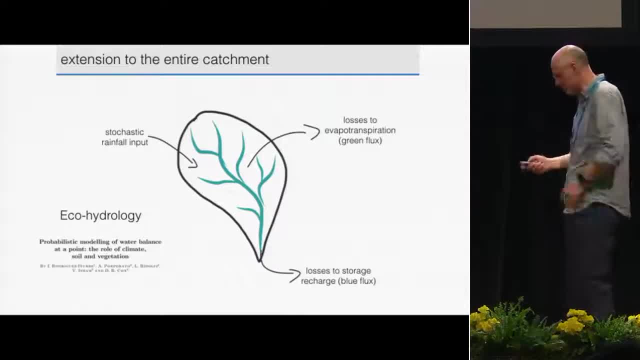 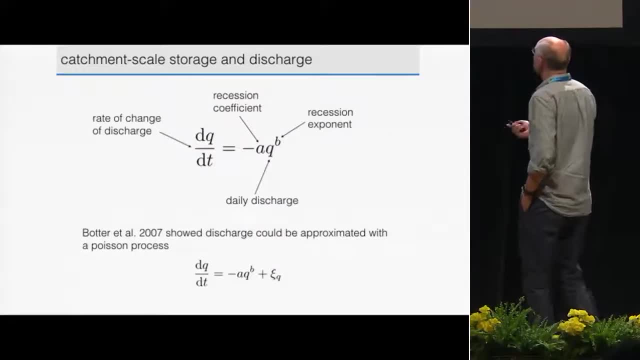 except that it has a typical soil thickness, it has a vegetation built into it. so a few parameters which you can kind of summarize with the response time of this system. this is the famous recession equation and we can constrain that very easily for a given river. if you sit at the bottom of a river, 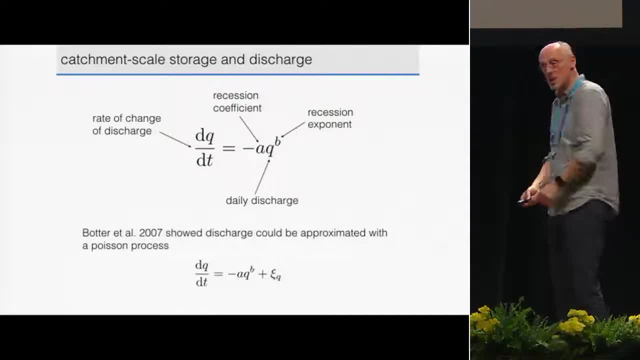 all you have to measure is how the discharge changes when a big storm hits the river, and that gives you the value of A and B. you do it for many big storms and you get the statistics on A and B, and so what we do- and it's not been the first time- 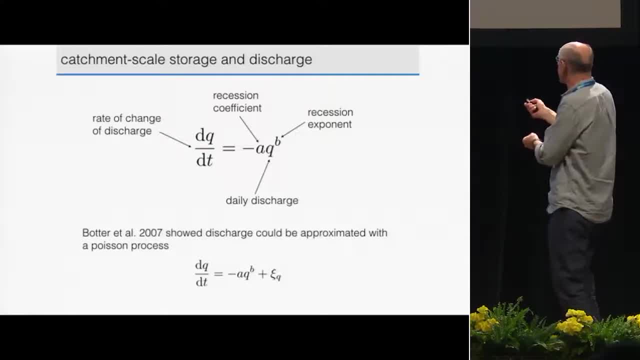 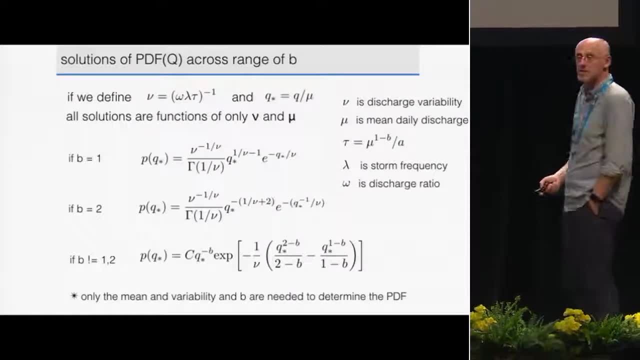 others have done it before- where you feed to this a stochastic or probabilistic distribution of events and you see how the system responds and you get a probabilistic distribution of discharge. and what Eric has done- which is really neat- is that he's actually produced analytical solutions for that. 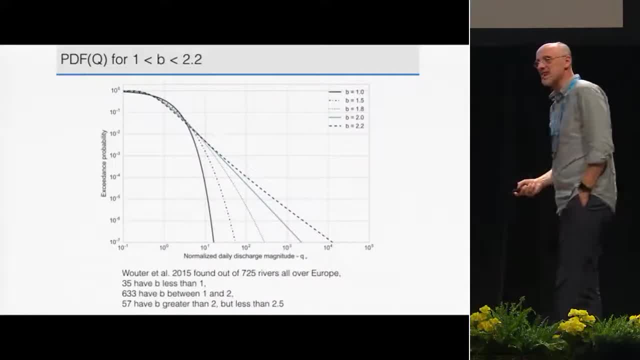 and I'm not going to get through that, don't worry. the point is that there is a very important factor: is that B exponent? and that B exponent really controls in the recession equation? it controls the shape of this day, and we know that it's very important for us. 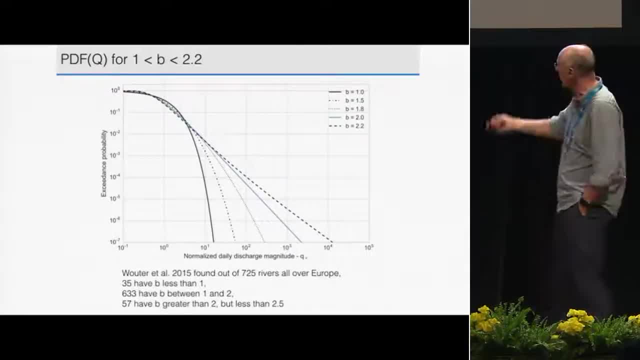 and what's really interesting, if you go to many rivers all around the world, or in this case, in Europe, you see that B is very variable, from less than one to larger than two in natural systems. so we see here: this is the distribution of now discharge, what we're given rainfall. 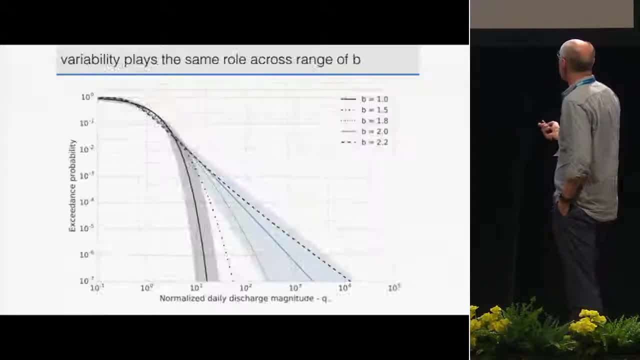 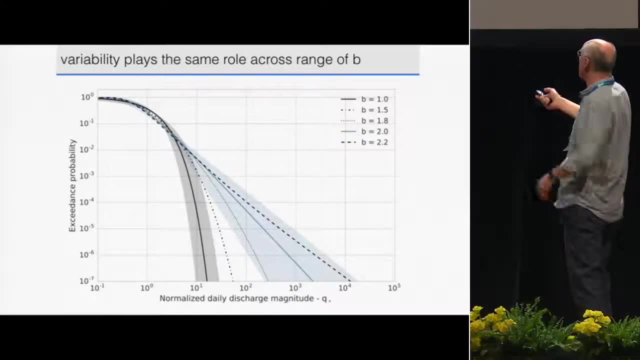 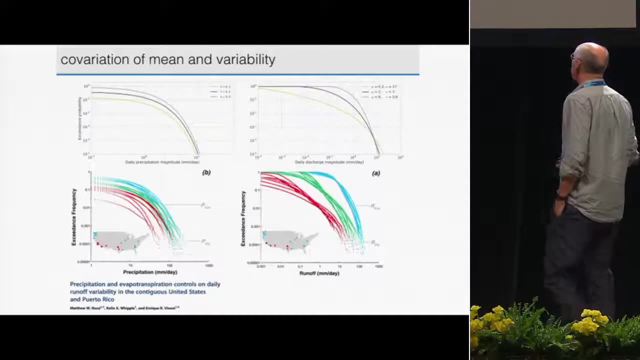 that you can derive from this model depending on the value of B and you can add to that variability and you see how the variability increases the distribution or decreases the distribution based on each of the B values. we can compare this to data. it works beautifully well if you take, for example, 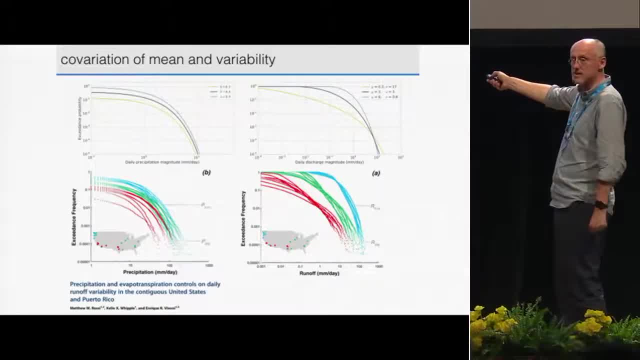 rainfall distributions from all over the US and compare them to the discharge, you see that the response it's not obvious. all the precipitation distribution have almost the same tail, but the discharge can be characterized by very different details and in our model we can do this very easily. 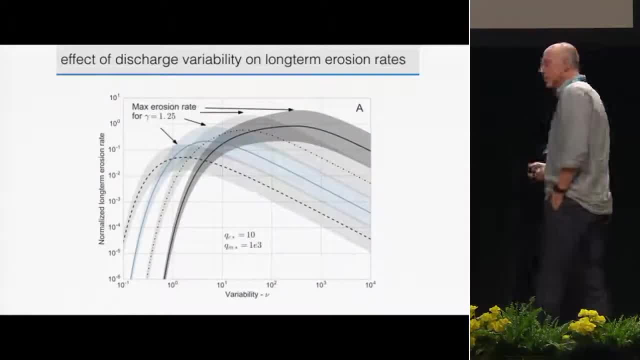 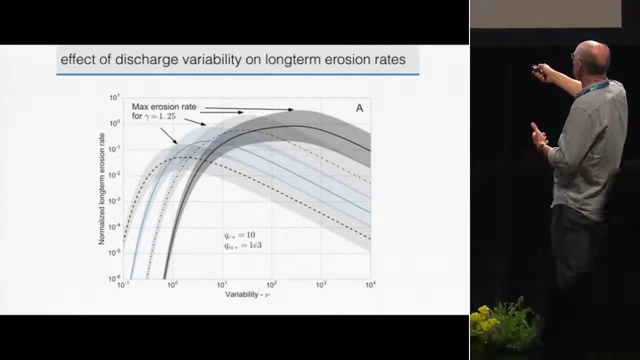 by changing the B value. the conclusion for this is: if we now plot erosion rate as a function of variability, it depends on B. of course we expect that, but what's also very important, we also predict that for each value of B, for each different value of B, 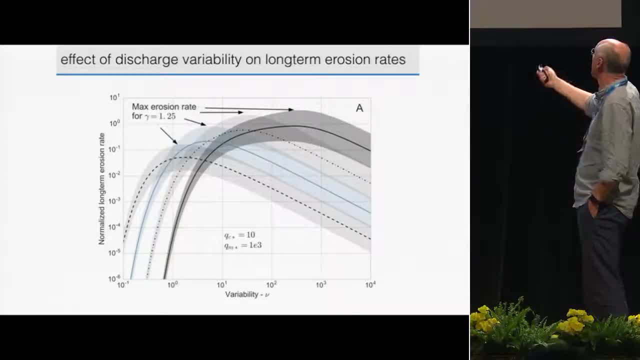 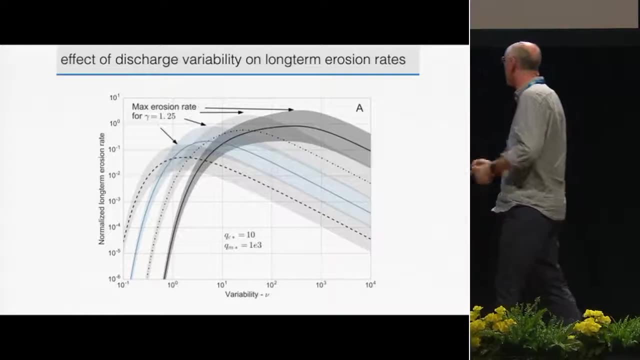 there is actually an optimum variability at which we get a maximum erosion rate, and so in rivers can be very efficient at high variability. let's take this blue curve here and this variability. but they will become less efficient even for a fixed threshold at high variability. and the reason for that. 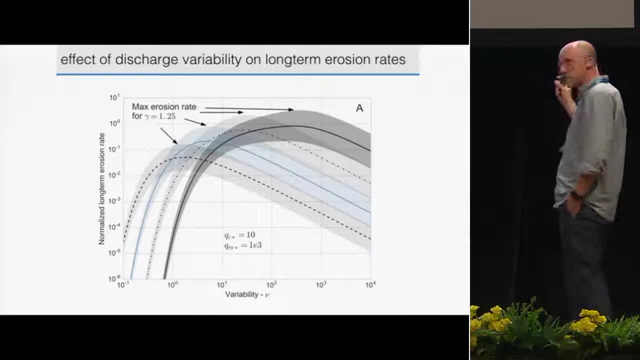 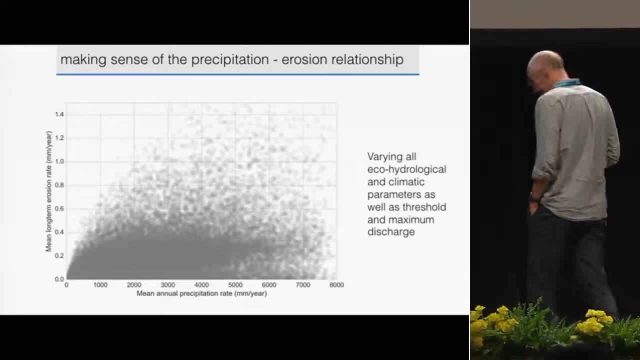 is because, also, as I mentioned, there is a: you have to include in these models the maximum possible discharge. the value of the maximum possible discharge doesn't matter, but you have to have one. now I'm finishing with these two plots which are very distressing. remember, geomorphologists are in this quest. 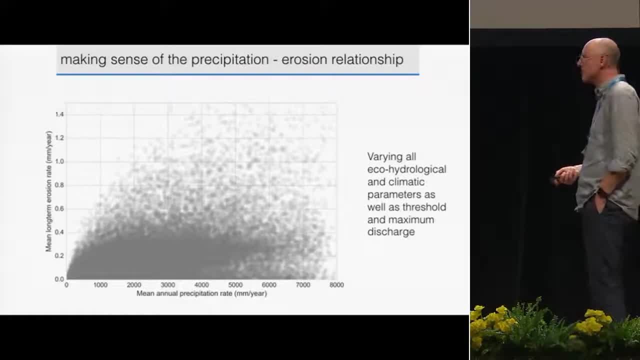 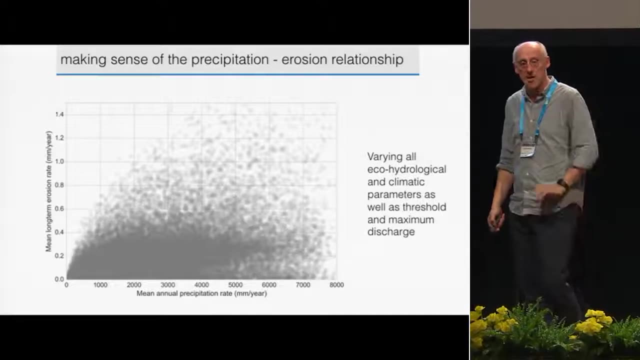 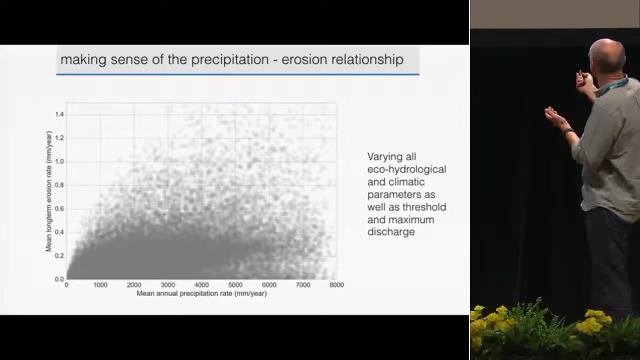 of determining whether there is a relationship between mean precipitation rate and mean erosion rate. is there a climatic control of erosion rate in mountains, let's say, due to precipitation on these? and what these plots show is that we've taken five parameters in this model, some that characterize 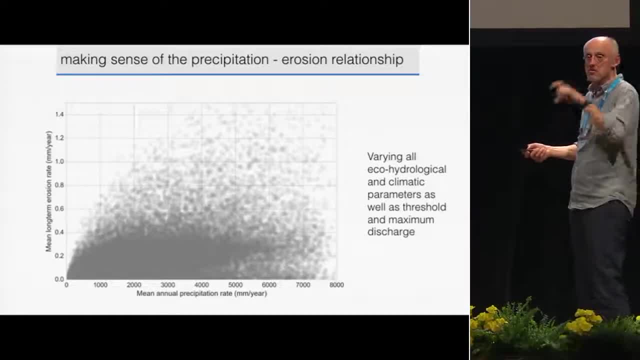 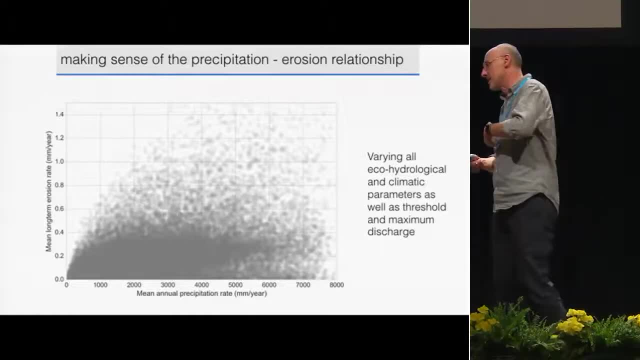 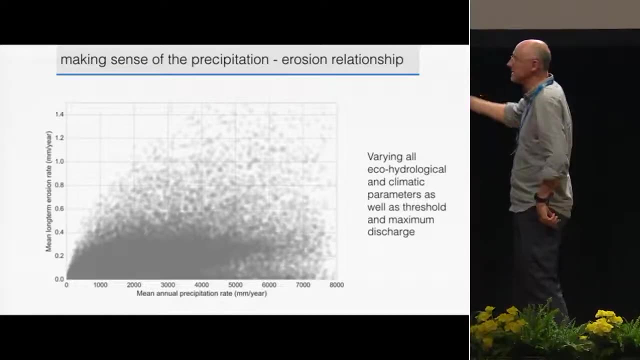 the equal hydraulic rate in the geologic model, mean soil thickness, vegetation and things like that. we've changed the climatic parameters, the b, the mean, the variability and the threshold, and then we have this analytical solution. we can plot this in five seconds and it shows you. 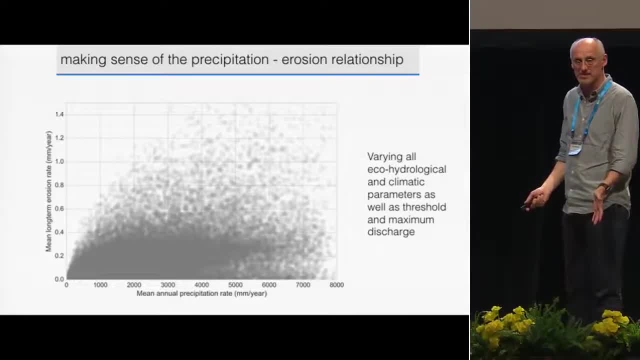 basically, there is no relationship. what this means is that if you try to figure out, for example, at the global, at the planetary scale, if there is such a relationship, it's very, very likely that you will never find it, and this has been a frustration for us, and I think it's easy to explain it like that. 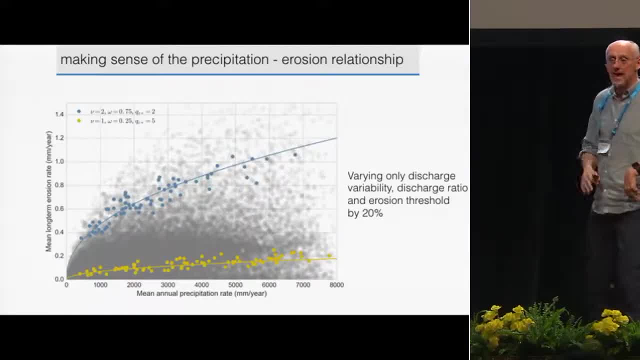 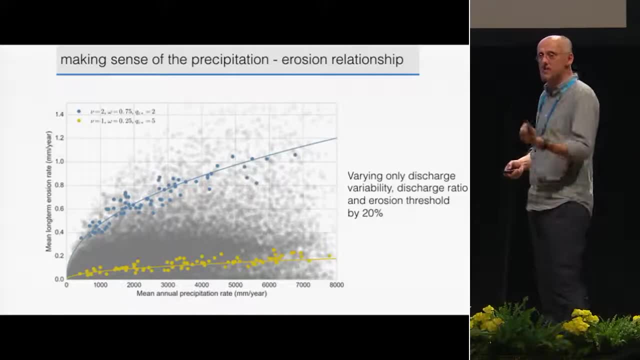 however, if you go to a place where kind of everything is constant and you say, okay, I'm going to go in this caption, and I believe it has a slightly different threshold from that caption, but everything is the same- then we can say that there is a clear relationship. 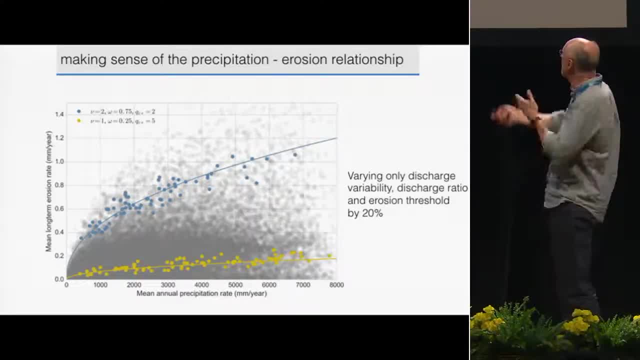 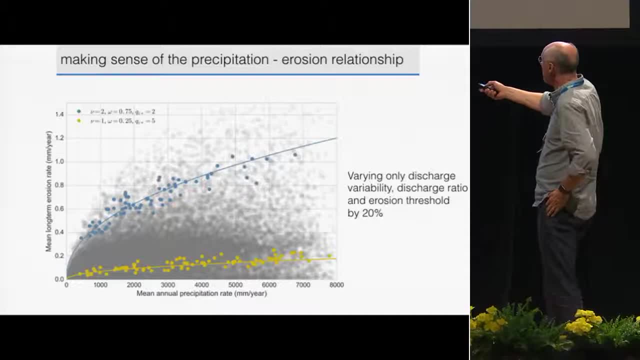 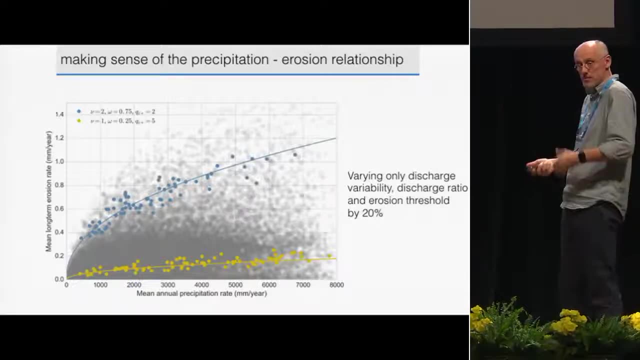 between mean precipitation rate and mean erosion rate, and the variability here is by changing the variability of the mean a little bit in these calculations, or the mean before. so in other words, if you are studying very carefully selected sites, you may be able to actually extract this from observation. 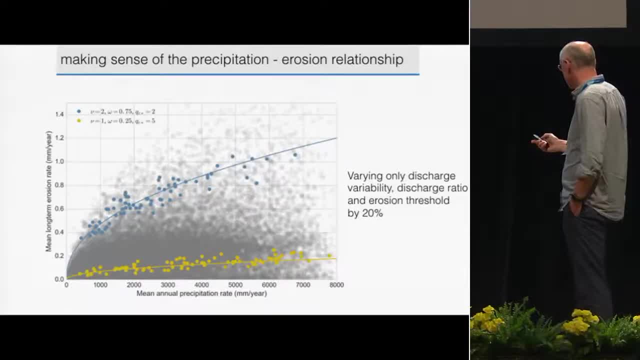 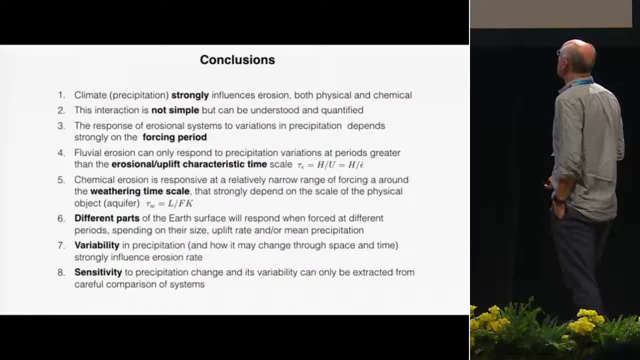 but at the global scale, it is no hope of doing it, and so this adds a new level of complexity in interaction and long term evolution of erosion rate at the surface of the earth, which you are only starting to explore. so my conclusions are: yes, I think the climate 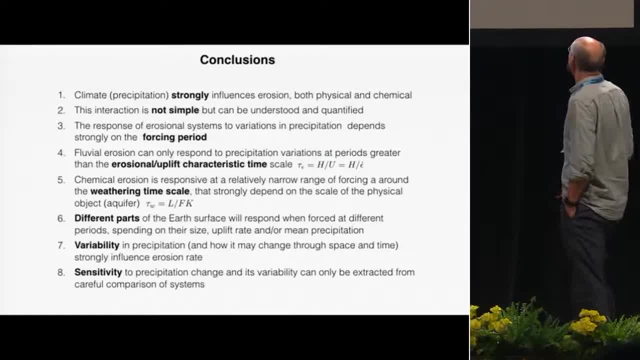 definitely strongly influences erosion, both physical and chemical, although here I only look obviously at precipitation variation, not temperature, which especially for the chemical weather it might be very important. the key here also to that interaction is not simple. one thing we must be very careful for us is to consider: 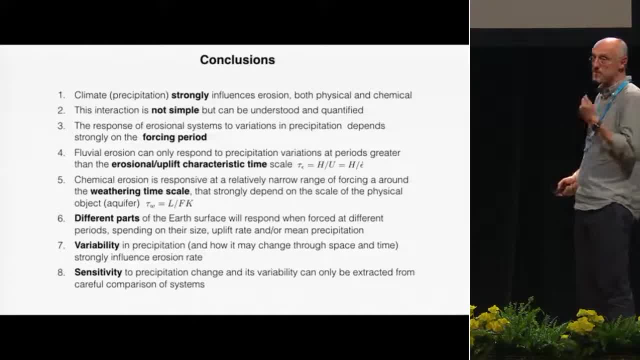 the period at which we are changing the precipitation, because for the fluvial erosion the response will be a strong function of that period of precipitation versus the characteristic period for erosion here, which is controlled by the output rate in the weathering system. it is the weathering timescale. 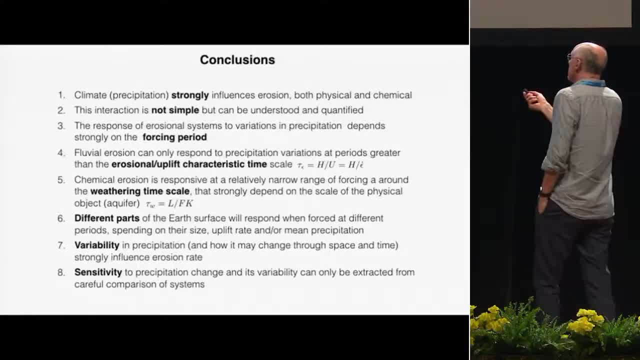 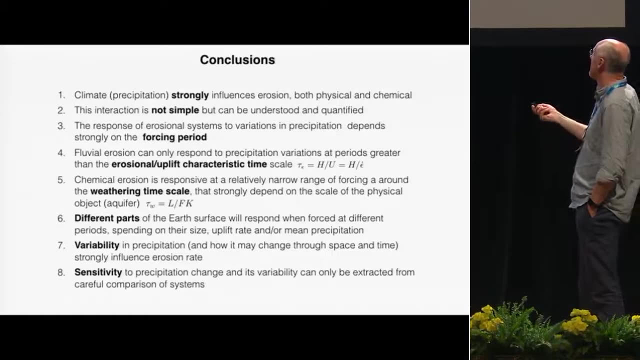 that matters, and that one is mostly controlled by the size of the system. so what we must conclude is that different parts of the earth system will respond differently at different periods. finally, the last two points that I make is that variability in precipitation unfortunately is not the main. 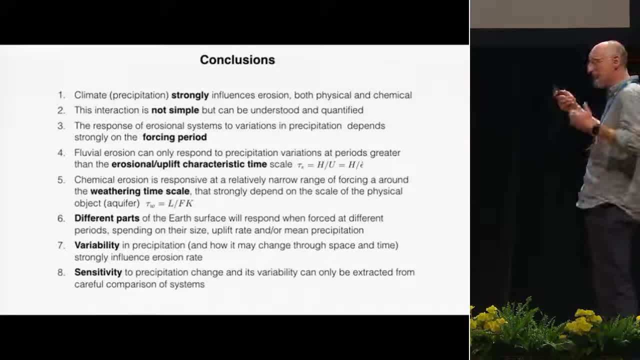 factor, but it is by the way it is. if we have a threshold in any of these processes, then the variability becomes very important and we have to be very careful when we go in the field or if we look for observations on characterizing the effect of that variability. 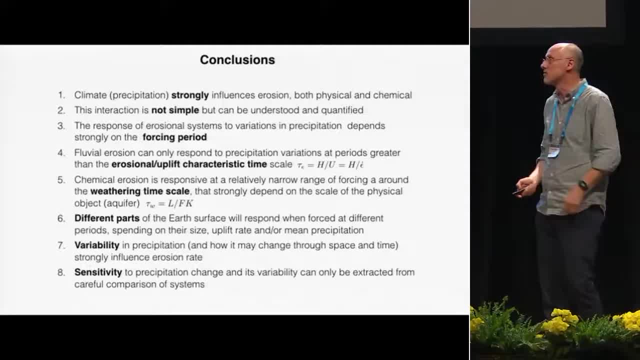 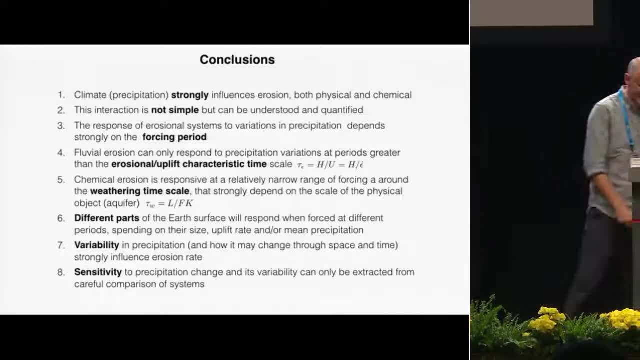 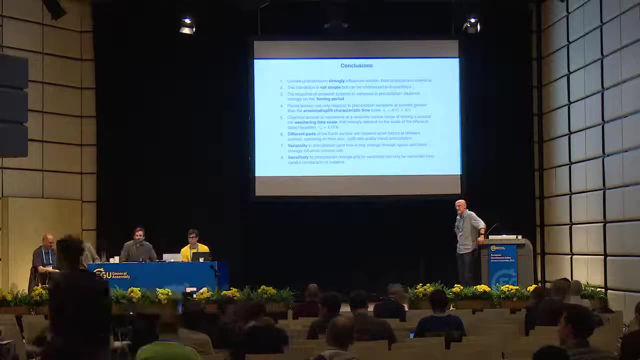 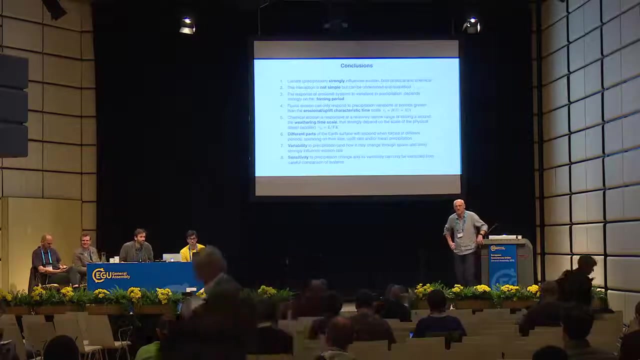 by being very selective on the, the object that we are going to see. I'll take questions. I have another slide that I'll take. Thank you very much, Sean, for this talk. yeah, Thank you very much. Questions. 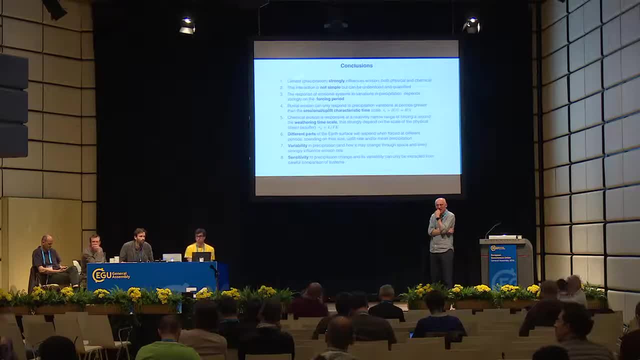 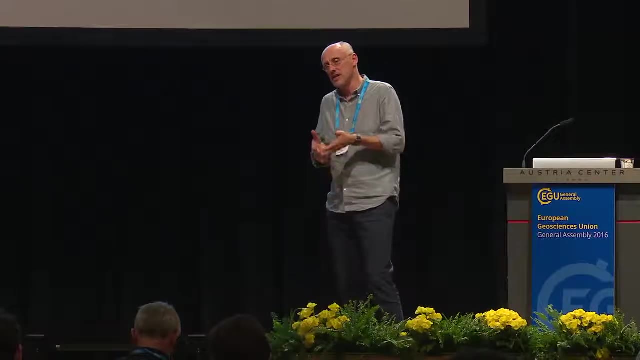 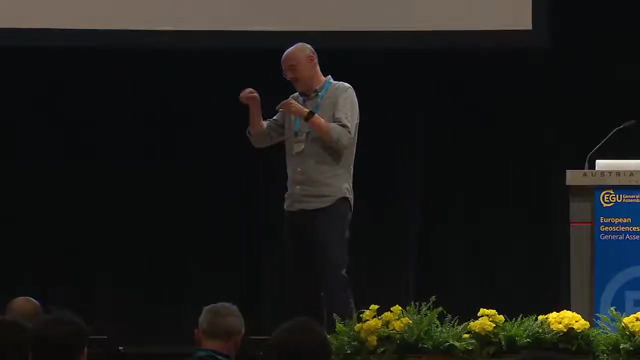 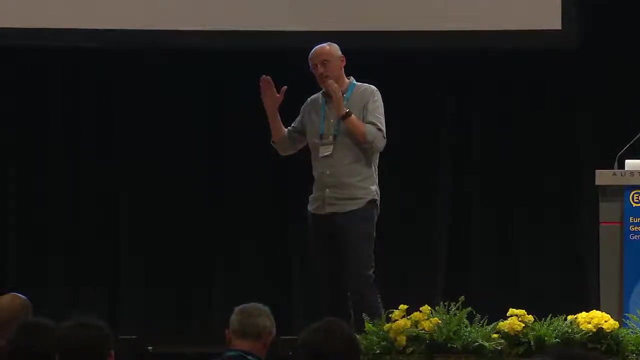 because clearly the length is essential and it's trivial, but it's obvious. but in the weathering process one of the key aspects is the length of the system and that is determined by the size of the aquifer. 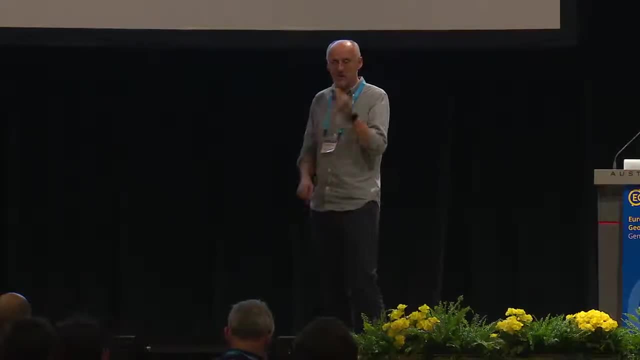 in other words, where you connect your hill to your base level, the water- and so that is the river, and so the position of that is strongly dependent on the physical environment. also, the erosion in the river is dependent on the water that you get in the river. 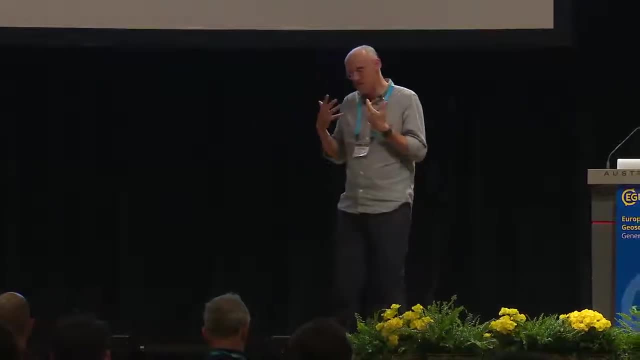 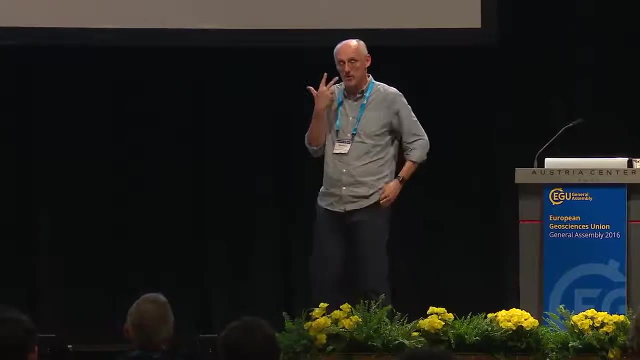 which is coming from the hill. so there is an easy, but we haven't done it. we haven't done the conclusion, an obvious coupling between the two. and clearly then we have three timescales to deal with: the weathering timescale. the response of the hydraulic systems to perturbation. 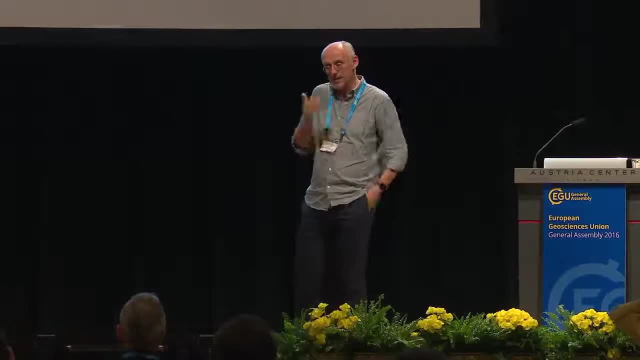 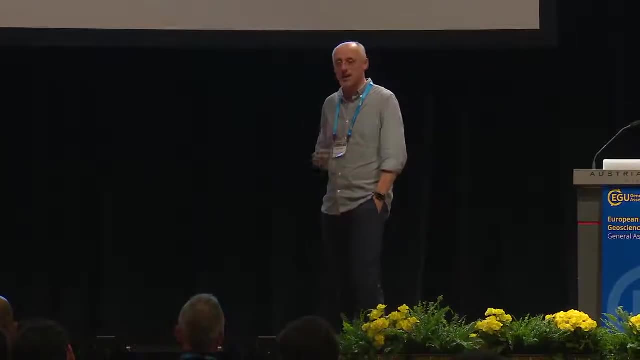 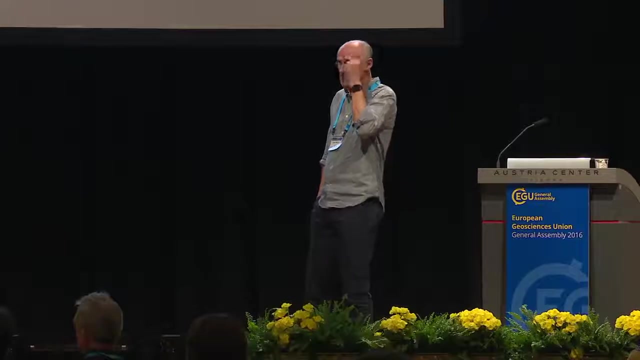 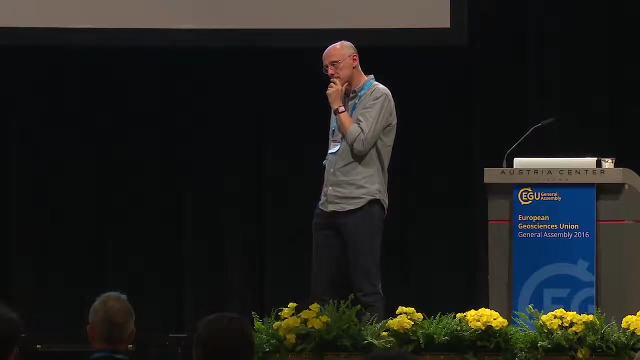 and the erosion, the physical erosion timescale. I suspect you know we should be able to get another one of these simple game formulas, but I haven't done it yet. Yes, Have you tried to plot precipitation stochasticity in terms of mean intensity and frequency? 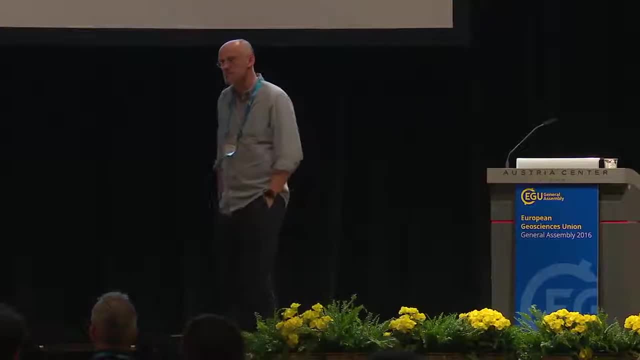 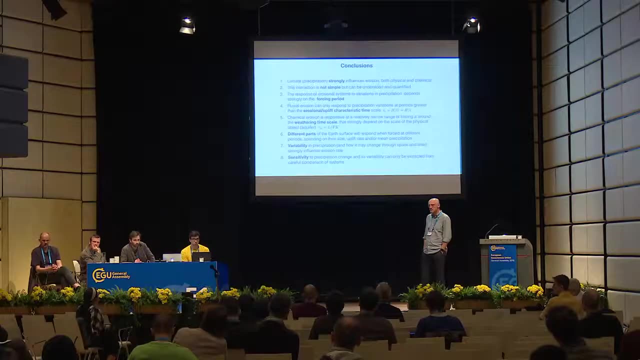 against mean erosion rate, because actually your model is driven by precipitation and fluctuation. right, The developer happened to be my canopy advisor and all of the summary from this result would usually be expressed in terms of intensity and frequency. so I wonder, is that because to choose to present it in terms of total precipitation? 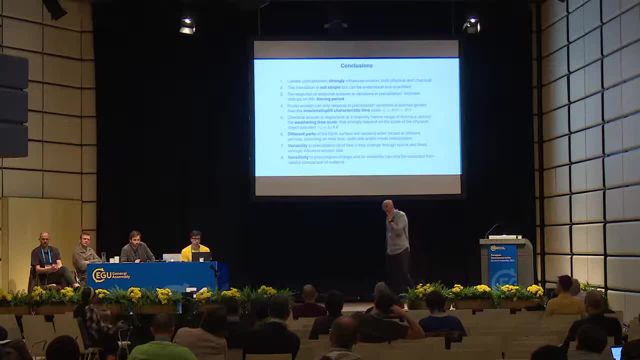 as a mean precipitation, instead of presenting it as a two-dimension of the frequency and intensity it might reveal more. So you're talking about the weathering right? Yes, The last slide. Oh, this one, Sorry. The physical erosion model or the weathering model? 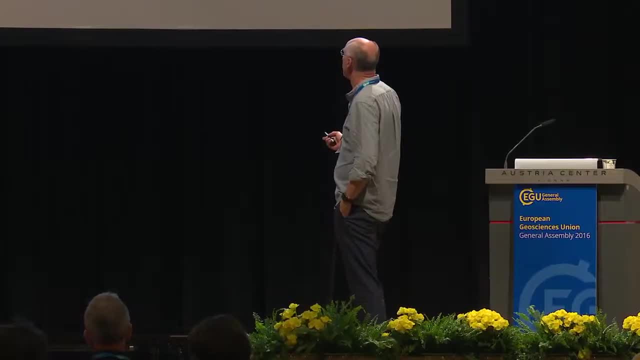 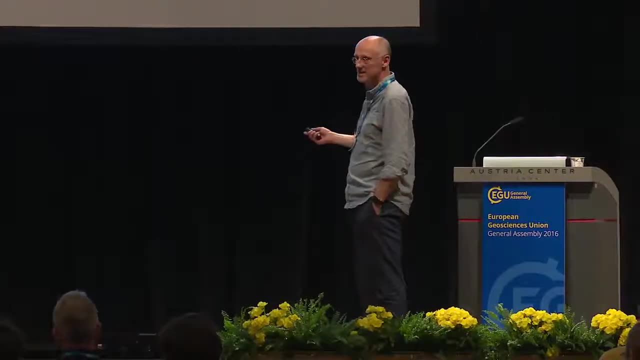 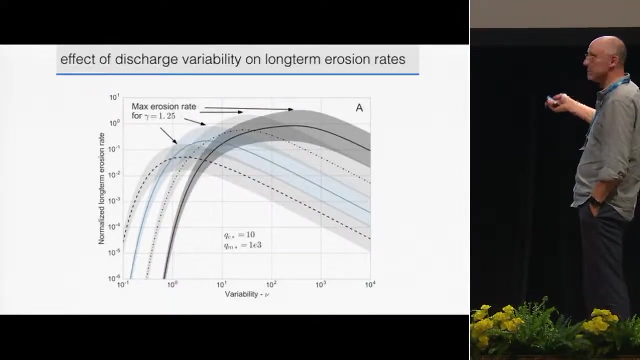 I mean the previous slide, This one. So, for example, in terms of like time productivity, if you counted: Okay, this is it okay. This is normalizing erosion rate as a function of variability in precipitation or, to be here, in discharge. 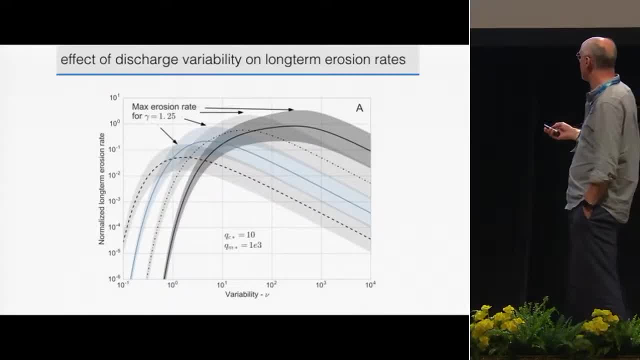 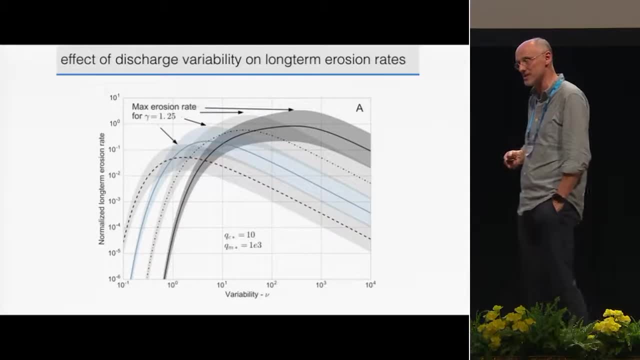 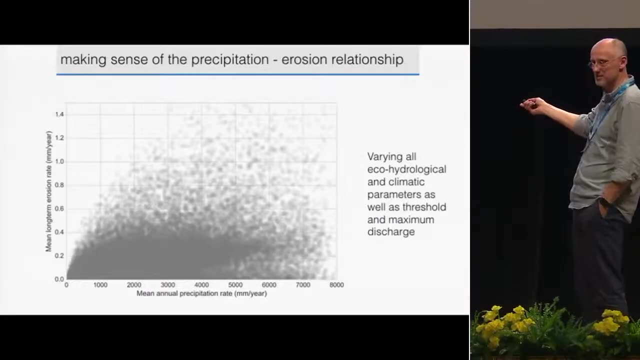 In total precipitation. Well, in discharge, which is what matters here, there's obviously a relationship between variability in discharge and variability in precipitation, but it's very similar, And this is the mean precipitation versus the mean precipitation. Yeah, we can plot it. It would show a similar thing. 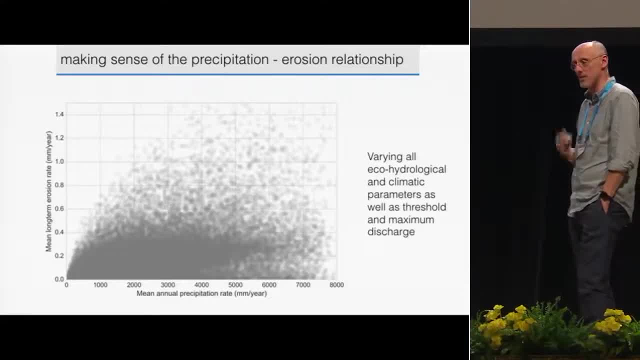 There's actually an optimum variability to produce an optimum, the largest possibility of erosion rate In my advice. I just wonder if you, instead of one dimension of precipitation, which is the mean amount, If it's, If you combine this with this, If you combine this with this, 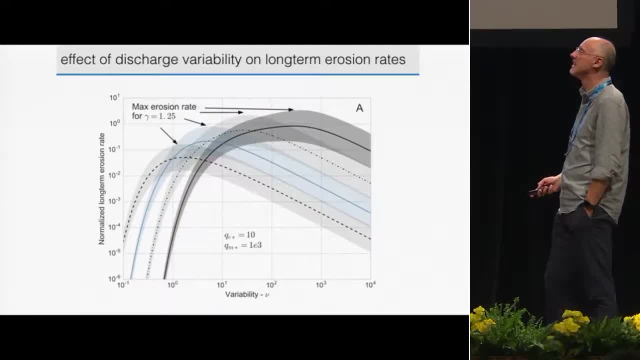 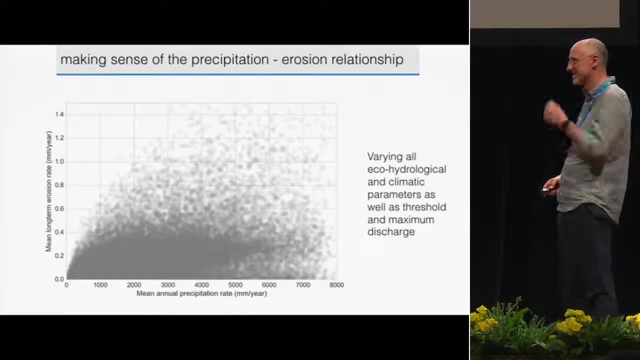 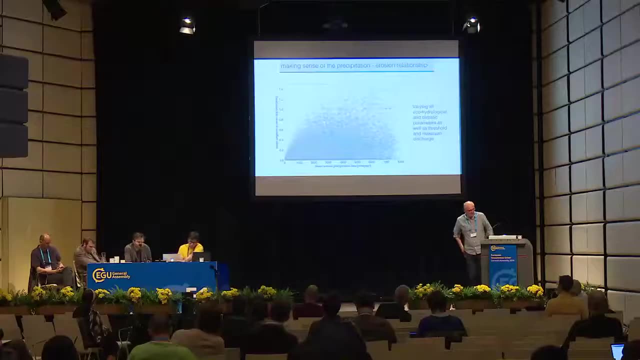 The dimension of the frequency and intensities of gravity. it removes more of the change. Yeah, you'd have to combine something like this with something like that. Thank you very much, Jean, And we skip to switch to the last talk of the session, which will be given by Yves Goderys. 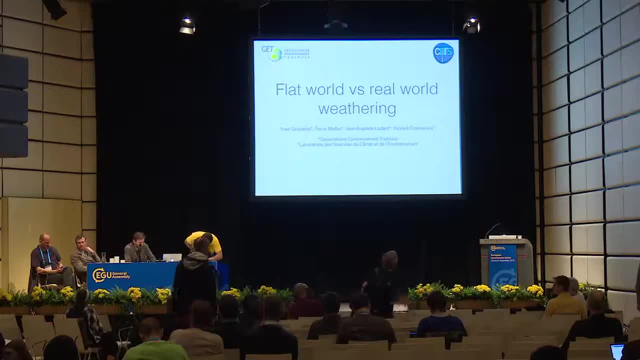 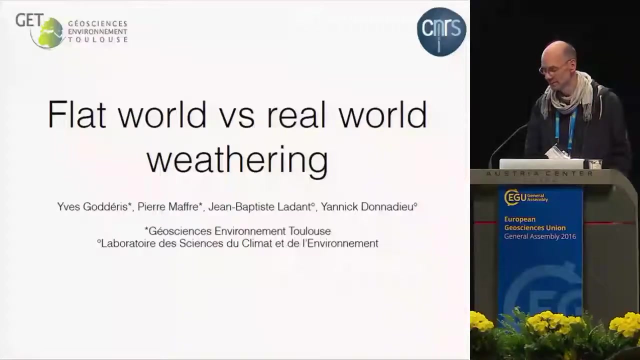 And Yves will talk about flat world versus real world and where is weathering The most important. So thank you, Thank you for inviting me to give a talk also. So I will discuss the weathering in flat world and real world in simple terms, And I will start with this diagram. 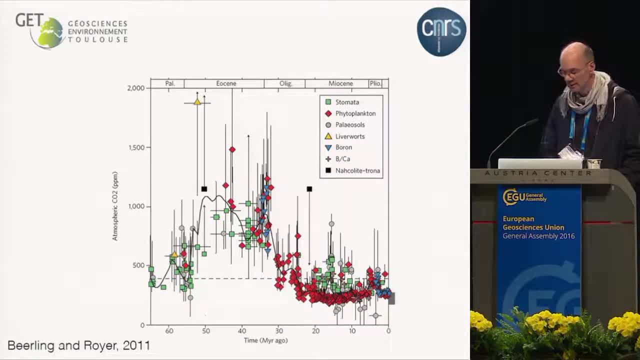 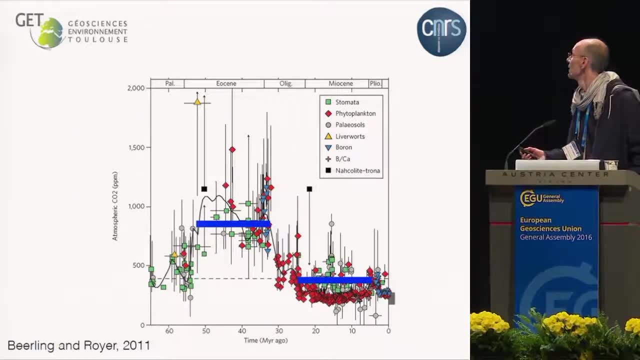 which is the CO2 level over the Cenozoic, And you can see that it can be defined more or less by a two-stage evolution: First high level at the beginning of the Cenozoic And then a decline of the CO2 lasting something like 10 millions of years. 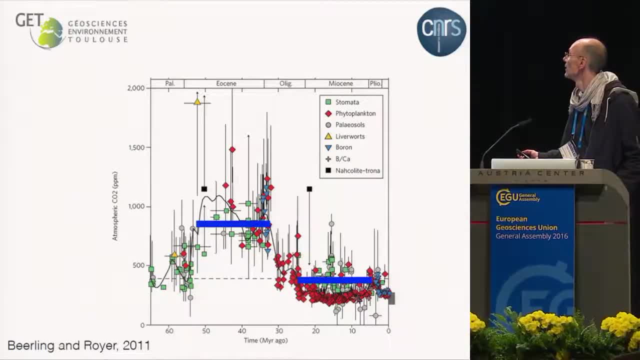 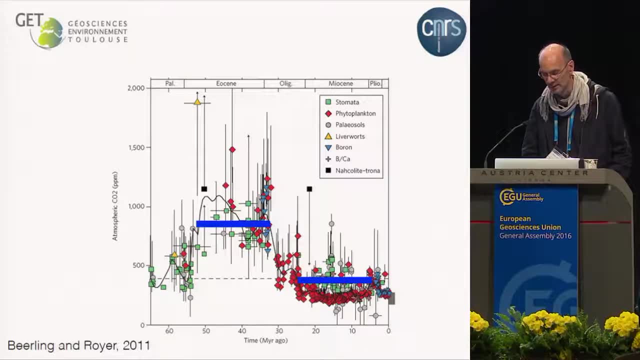 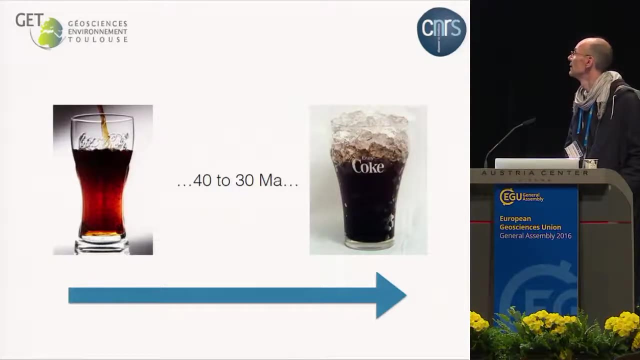 It's not instantaneous, apparently- And then a low level at the end of the Cenozoic. So my question is: how can we understand what is happening in terms of CO2?? And this is the way we are understanding today, more or less the Cenozoic climatic history. 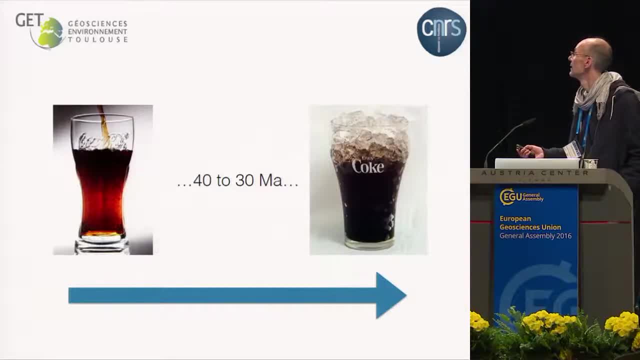 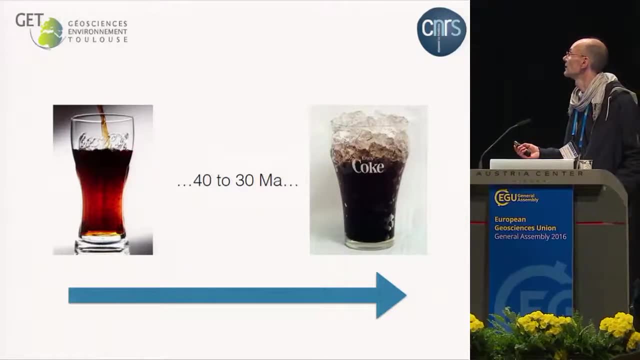 With the beginning of the Cenozoic you have no ice And then you are moving towards a fully icy world- Not fully, but largely icy world- With a transition period lasting something like 10 millions of years. So from the warm world towards the cold world. 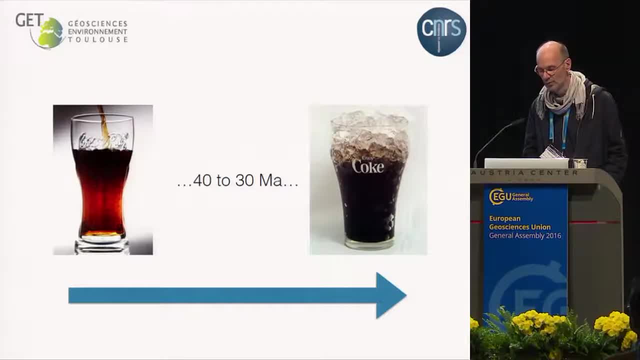 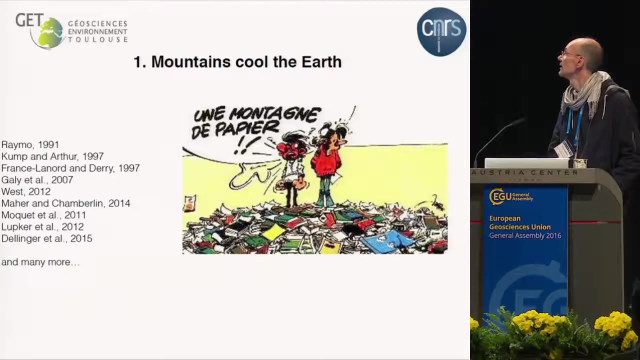 And the question is: what is the most important process explaining the change in the climate over the Cenozoic? Oops, sorry, Mountains. Mountains have generated a mountain of papers, And I just list some of them here. Sorry, I'm a fan of Belgian comics. 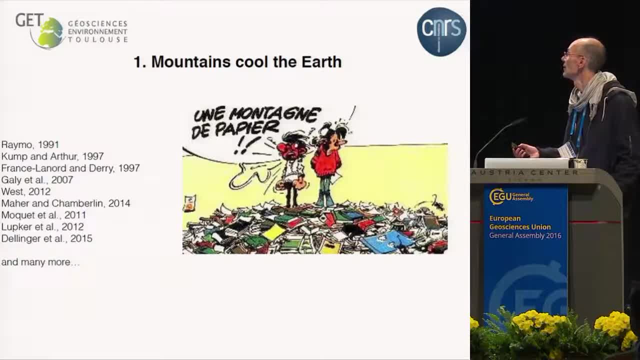 I'm just listing a few papers here, from Rainbow in 1991 down to De Linge in 2015. There are many more other papers, But I will just discuss a little bit what all those papers are teaching us In terms of the role of the mountain range. 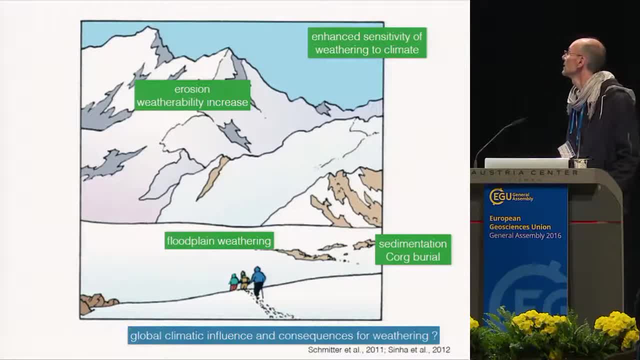 So this is a mountain. Among these papers it was evident that the erosion is increasing in mountains, Increasing the weather ability. Then product transfer to the food plane- This is not a food plane, but imagine it's green- To the food plane, where weathering is much more effective because temperature and runoff is much higher. 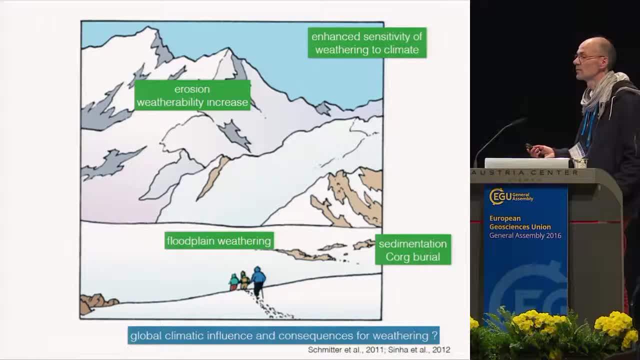 Then it has been proposed also and demonstrated, that the organic carbon burial is increased in the Bengal fan, Particularly for the Himalayan uplift, Due to the high sedimentation rates. And finally, recent papers have shown also that there is an enhanced sensitivity of weathering to climate. 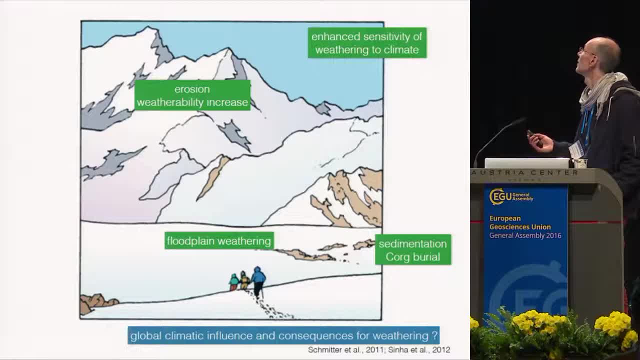 When you have mountains on Earth. This is a paper by Kate Maher and a paper by Joshua West. A question that is not so often addressed is the fact that What is the global climatic influence and consequences for weathering at the global scale of mountains? Because when people are looking at mountains, they are really looking at mountains. 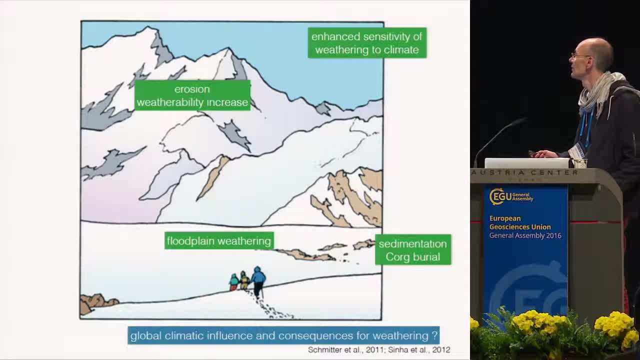 They are not looking at what is happening outside of mountain range. So this is a proposition we made, And I didn't find a lot of papers dealing with that, Only two papers: Schmitter in 2011, Discussing the global climatic influence, and Sina in 2012. 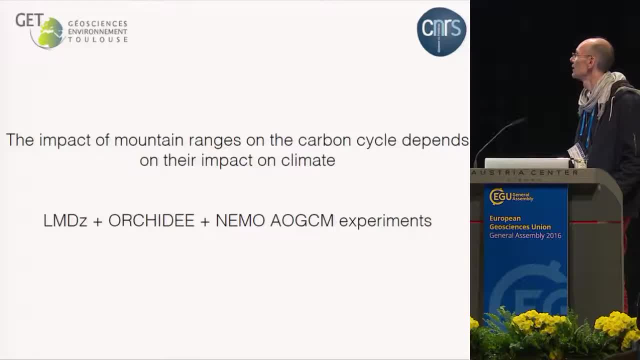 So we will explore this using an IPCC class model, Which is the couple between a climatic atmospheric model, A biospheric model and an ocean model, And we performed two experiments: The one with the real world and a lot of mountain ranges, And the other one with flat continents. 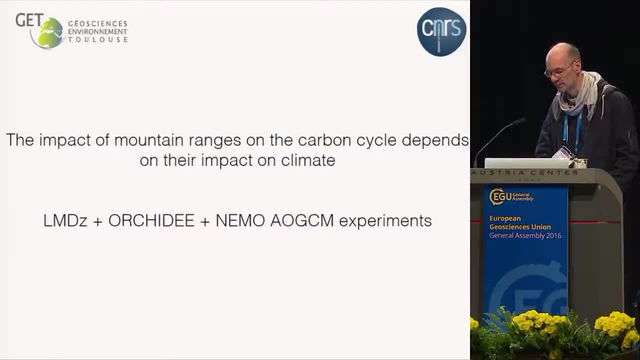 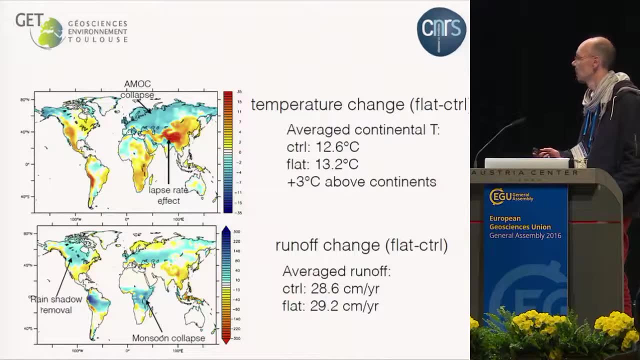 All the continents are flat at 200 meters altitude. So this is the change in temperature when you move from the control world, So the real world, towards the flat world, And you see here the temperature change. When it's brown and orange it means that you are raising the temperature. 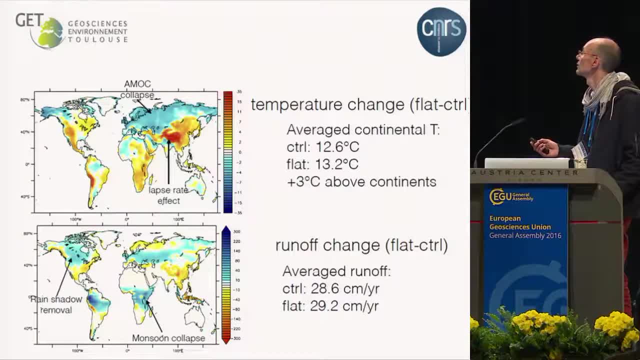 When it's blue, you are declining the temperature. So some important effect, The most important effect is the disappearance Of the lapse rate effect. When you are just decreasing the altitude, You are simply warming the surface And because of that you are globally increasing the temperature of the continents. By about 3 degrees Celsius. But there are also other, some specific things happening. For instance, a global cooling of Northern Asia and Europe Which is largely correlated to the Amok collapse, So the Atlantic meridional overturning circulation, Which collapses when mountains are removed from the system. 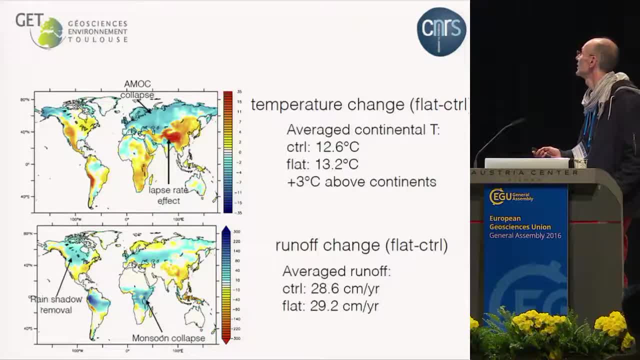 In terms of runoff change. Once again, this is the flat world minus the control world. You see that you have some place where the runoff is increasing rapidly, For instance here. This is because we are just removing the rocky mountains And because of that the rain shadow is not more effective. 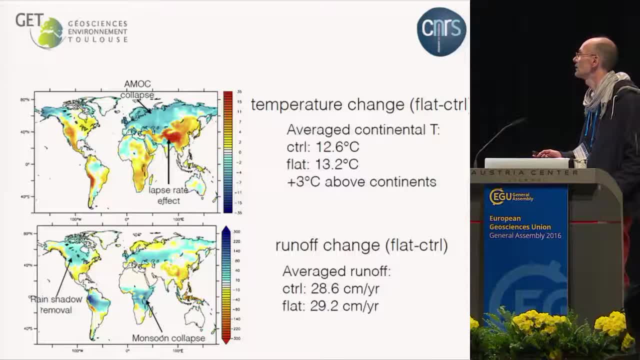 And the rain are reaching the interior of the continents, And here you have a big increase in runoff over Africa, And this is because of the monsoon collapse Linked to the fact that the Tibetan plateau has disappeared. There is also a big effect here. We don't know yet what is happening here. 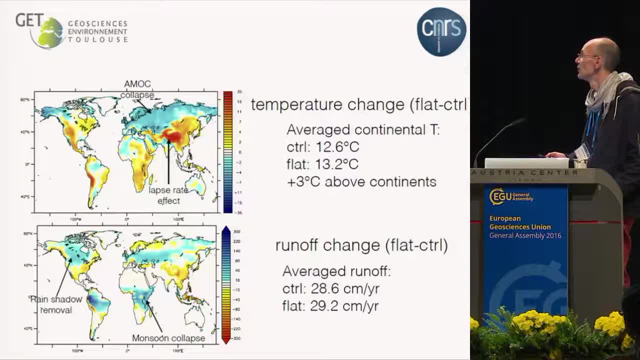 We don't know precisely for the moment, But we think that it is related to the collapse of the Amok. So this is under analysis. We have to dig a little bit deeper into this. This is the work of my PhD student, Pierre Maffre. I just have to say 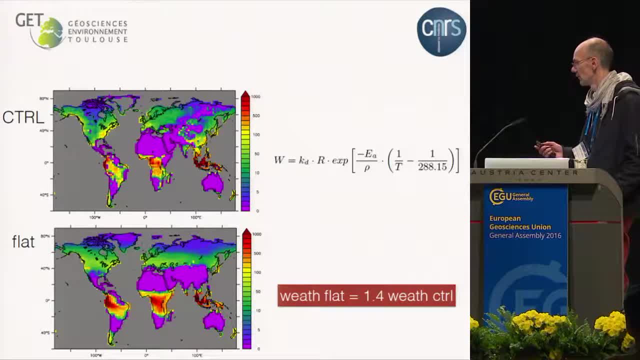 In terms of weathering, what happens? So if I use the classical law for weathering Which is generally used in global model, Saying that the weathering is proportional to the runoff And depends on temperature, through an Arrhenius law, Then you get, for the control run, this configuration for weathering. 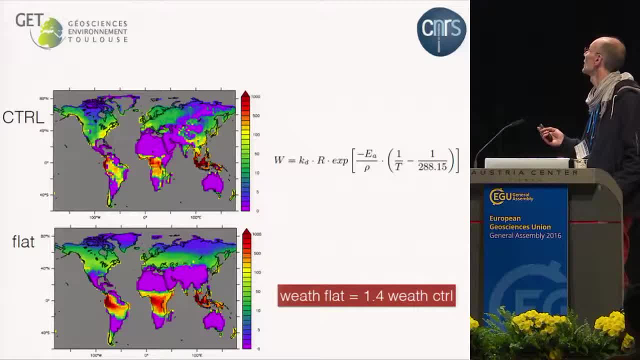 Which is high weathering in the tropical area, Where temperature and runoff are maximum. If you move toward the flat world, You will expect weathering to decrease Because you are just simply removing mountains, But in fact weathering is increasing. It increases by 40% using this law. 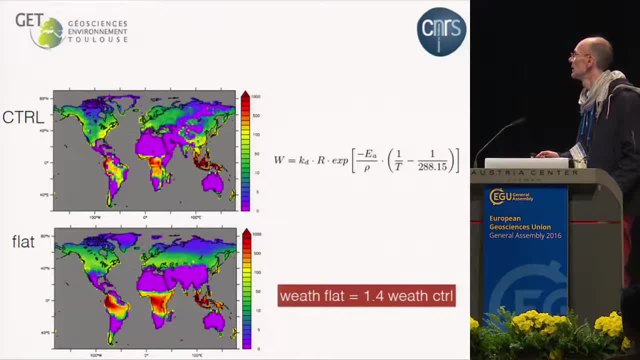 It increases by 40%, And this is particularly driven by the fact that in this area and here, Runoff is increasing in warm area, So promoting weathering And then consuming more CO2 from the atmosphere. Okay, that's the point. This is quite simple. This is quite obvious when you look at this law. 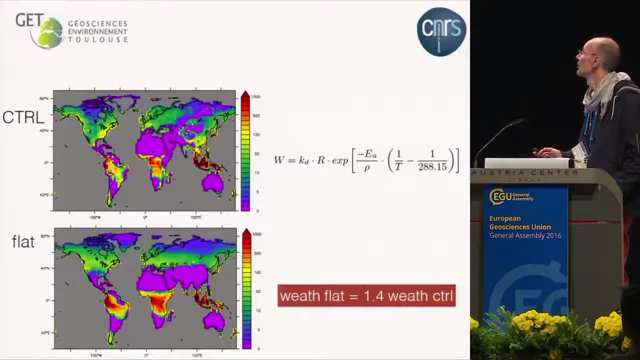 So this is why we think that this is not exactly how the weathering is working today. The most important weathering fluxes are not located in the tropics Because of a simple effect which is a soil shielding effect. So we modified slightly the model. We introduced physical erosion. 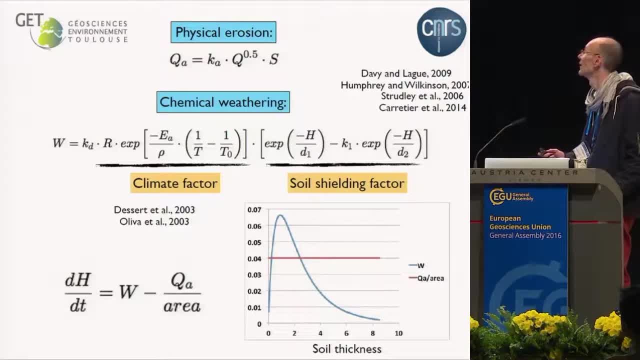 In a simple way compared to what Jean has shown you just before. We simply assume that erosion is proportional to the runoff, to the power 0.5 and to the slope. So this is what: at the top of the weathering pile, The physical erosion is removing materials. 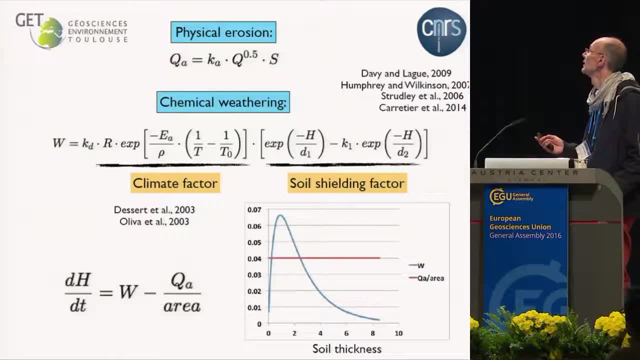 And at the bottom of the weathering profile. Chemical weathering is producing a lot of clay minerals and producing soils, And you see that we divide it into two factors: First, the climatic factors, as previously explained, Depending on runoff and temperature, And second, the soil shielding effect. 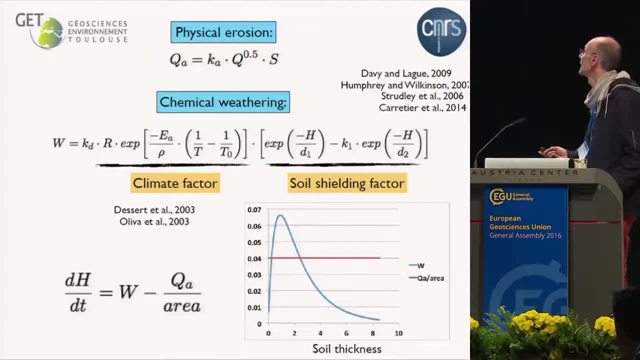 Which is depending on the thickness of the regolith, And it's looking like that if you look at the low. So it is increasing for low thickness, For low regolith thickness, And then decreasing rapidly when the regolith thickness is increasing. So this is a soil shielding effect. 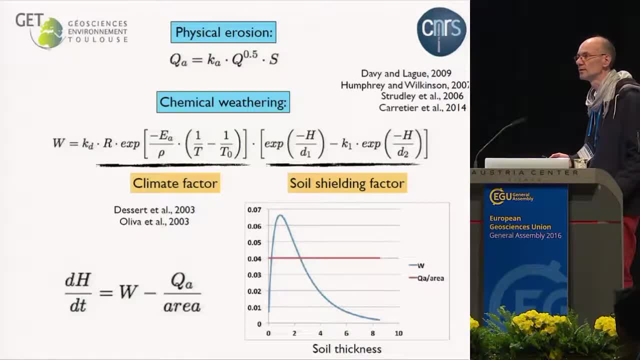 Because the water cannot reach anymore the bedrock, And so weathering is slowing down. We solved, for each point, For each pixel, this simple derivative equation. In fact, we solved it for steady state solutions. So we put it to 0 And we just simply calculate the weathering corresponding to the condition of equilibrium. 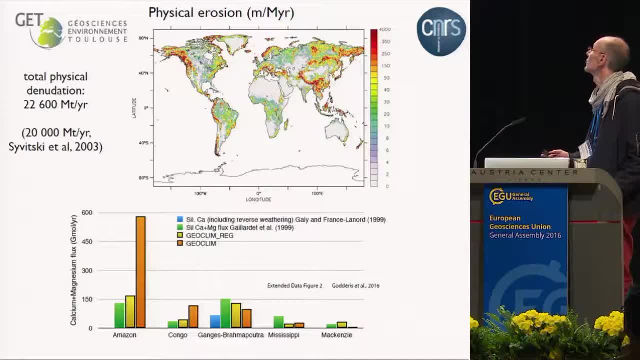 This is how it looks like for the physical erosion in the modern world, Which is not too bad. You have mountains contributing a lot to the erosion flexes, But also if you look at the weathering In green and blue, these are the data for the Amazon. This is roughly the CO2 consumption by the Amazon River. 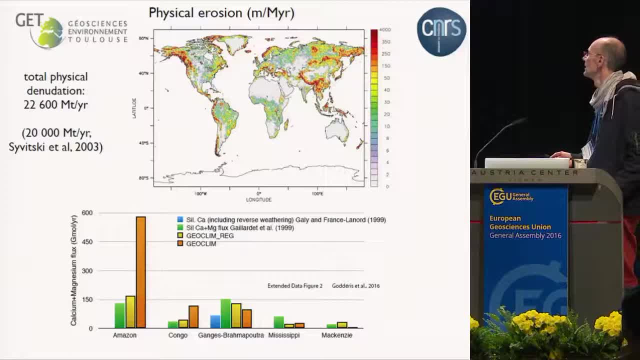 Congo, Ganges, Brahmaputra, TCCP and Mackenzie. And you see in orange what is calculated by the simple model using the previous low. I mean the low depending only on climate. You see that there is a large overestimation of the weathering in the tropics. 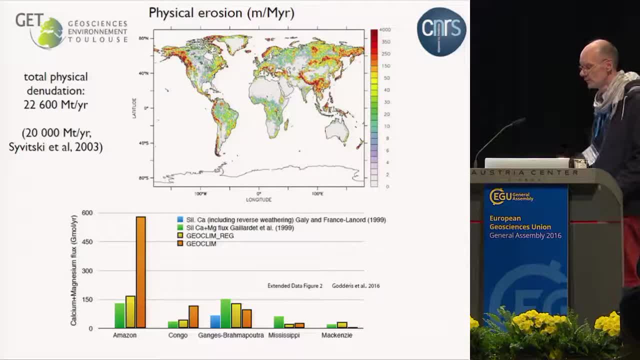 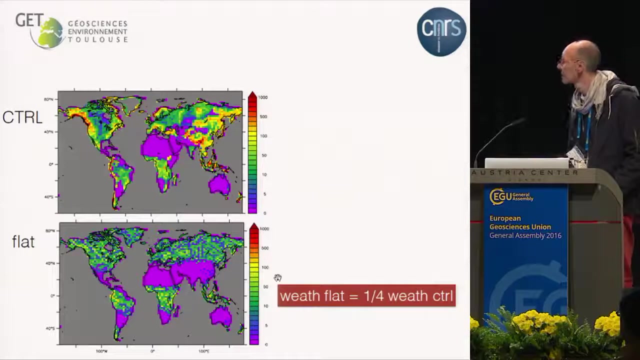 Because the runoff and the temperature is quite high. If we simply had this shielding factor, This one, Then we get the yellow boxes. So a large improvement of the model, Which is not yet perfect, But at least it's largely improved compared to the previous model. This is how it works for the control world now, with this new low. 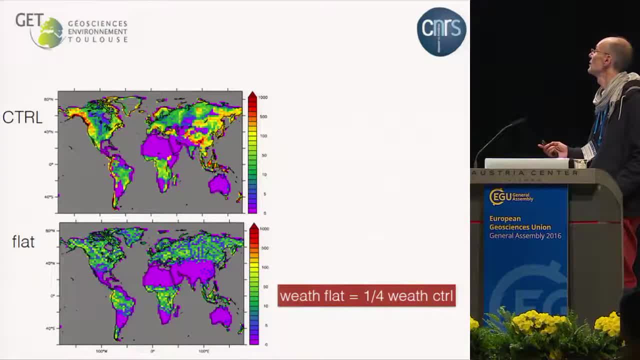 You see that in the tropics weathering has been decreased And it has increased in the tectonically active area. And if you move toward the flat world, you get this With a big decrease in continental weathering, Which is only 25% of the weathering of the control world. 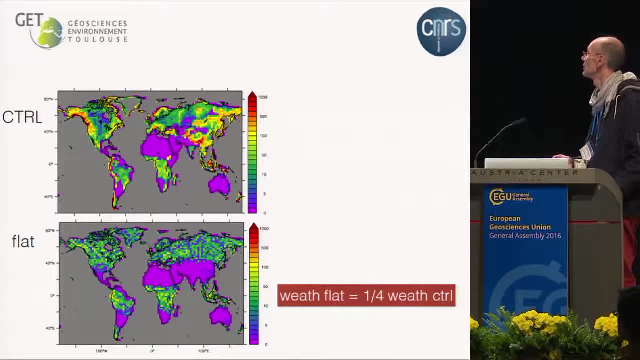 So there is a big effect by just removing the relief. There is a big effect on weathering And you are simply catastrophically decreasing the weathering in the flat world. This means, of course, that because the weathering is catastrophically decreasing, CO2 will rise very rapidly. 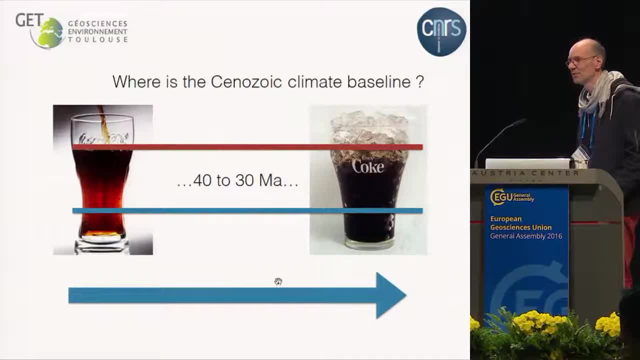 And then I'm going into the core of my talk. The question becomes the following: What is the climatic baseline of the Cenozoic? Is it a warm world, starting from the Cretaceous And then going into the Cenozoic? 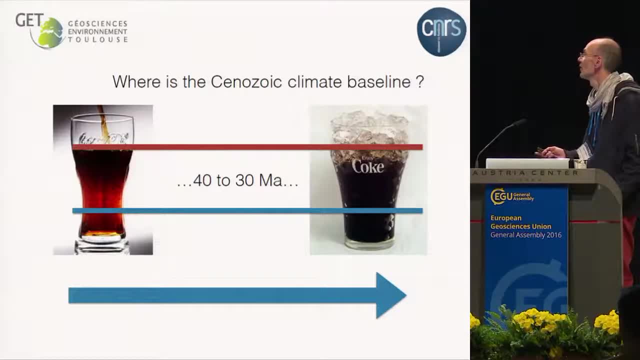 And then collapsing at the end because of the mountain ranges? Or is it a cold world And it is cold at the end and warm at the beginning, Because there is a big event here: the absence of mountains. So the absence of mountains would require a cold baseline climate for the Cenozoic. 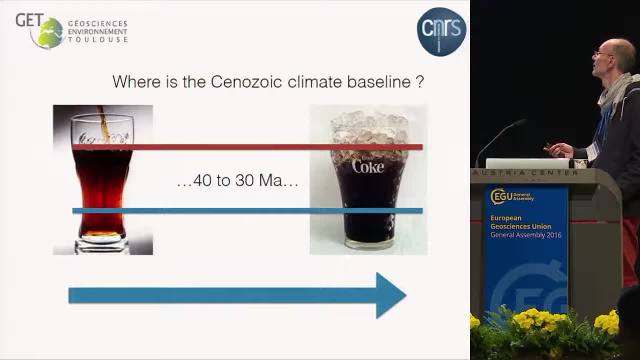 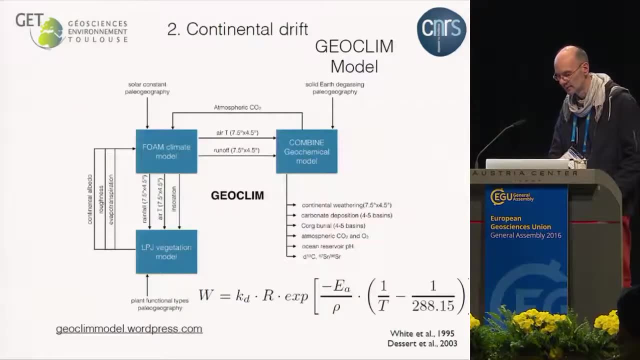 While the presence of mountains will require a warm baseline for the Cenozoic. So how does it work exactly? It's just the upside down, in fact. So we use a geoclim model. I will not go into details, But just let you know that it's a model coupling a 3D climate model. 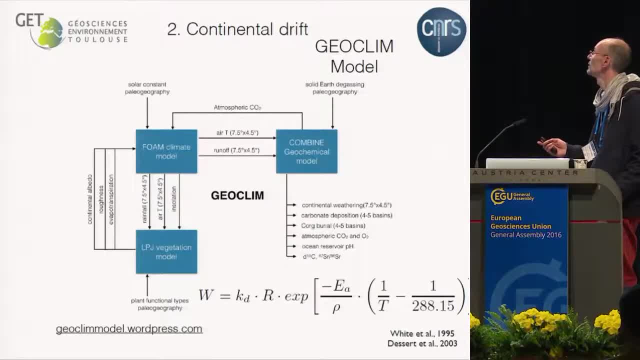 Used to calculate air temperature and runoff on the continents, Which are injected into a module calculating the chemical weathering of the continents. I'm not going into details. We can potentially discuss this even after the talk, And this is what Lefebvre et al have shown in 2013. 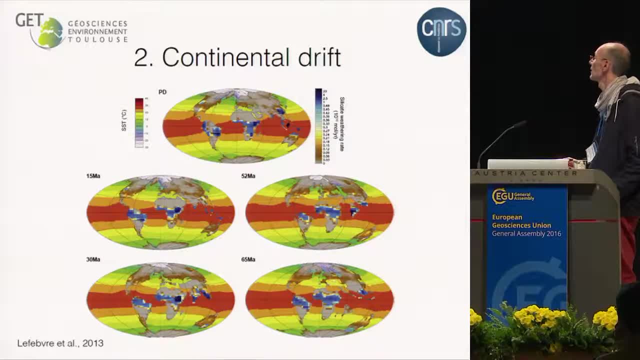 These are several simulations On the continents. you have the weathering rates With the old laws, So there is something still not clear about that, But we can discuss it, of course. This is the Cretaceous, the end of the Cretaceous. This is the Eocene, Paleocene, Miocene and present day. 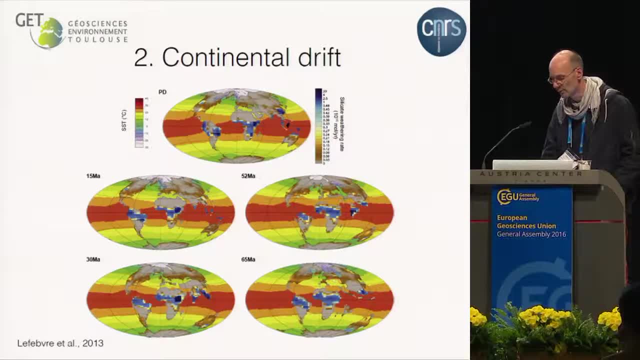 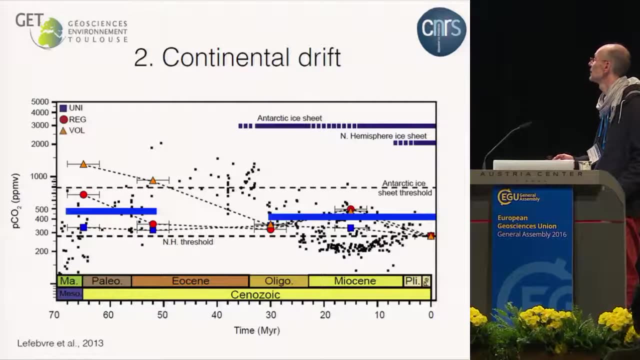 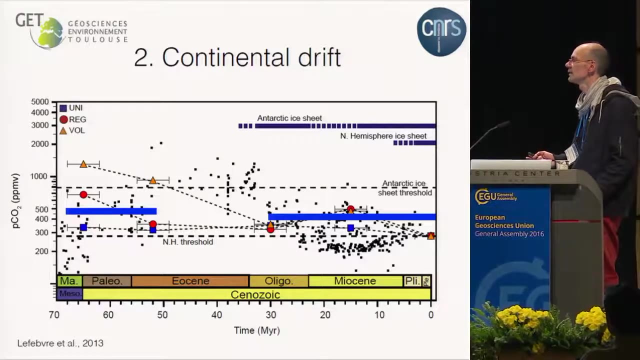 And you see that because of the dispersed configuration of the continents, There is a lot of rainfall on the continents And because of that they calculate an atmospheric CO2 level. These are the blue squares here. The black squares are the data. They calculate an atmospheric CO2 level which is below the glaciation threshold of Antarctica. 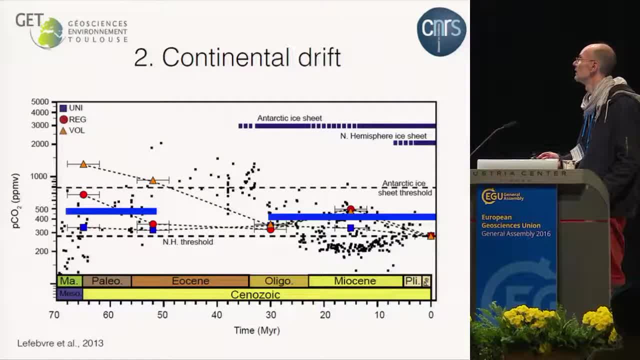 As early as in the Paleocene. So the complete Cenozoic is in fact completely cold, In fact characterized by a very low CO2 level, Because continental configuration is dispersed enough to bring a lot of water on the continents And to promote weathering. The solution they found to start the glaciation: not in the Paleocene. 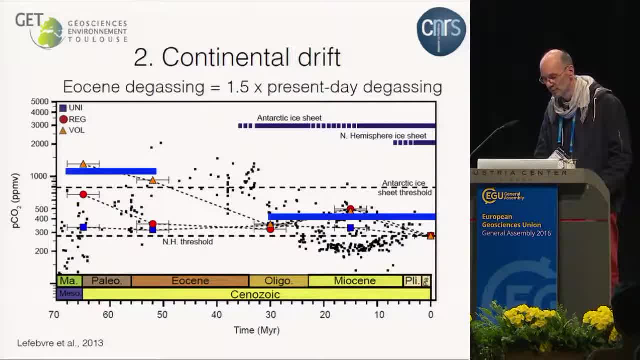 But to start it around the Oligocene, They simply increased by 50% the degassing rate of the Earth, Using some proxies that have been proven. This is one possible solution, But a bit disappointing because we have not so much constraint on the degassing rate of the Earth. 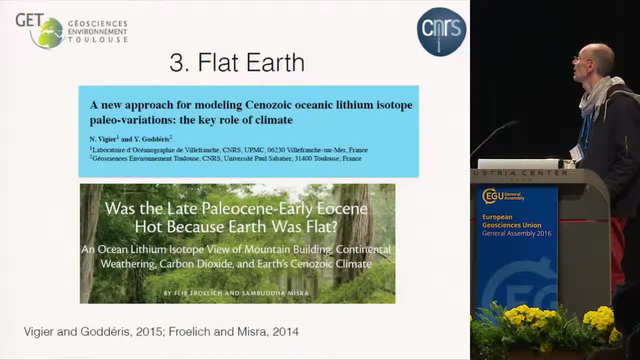 So the other possibility might be to warm the early Cenozoic By producing, by shielding the weathering rates with very thick regolith, And this has been published by Nathalie Vigier and myself last year in Climate of the Past, But also by Frélic. 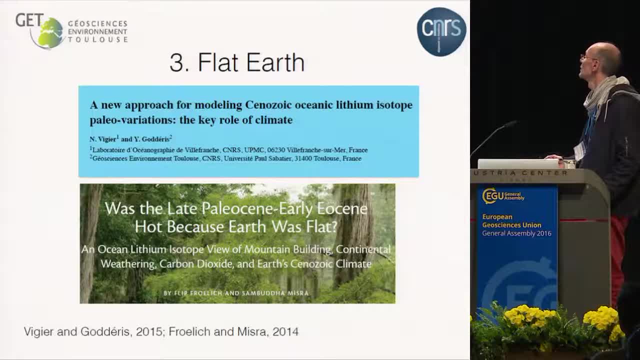 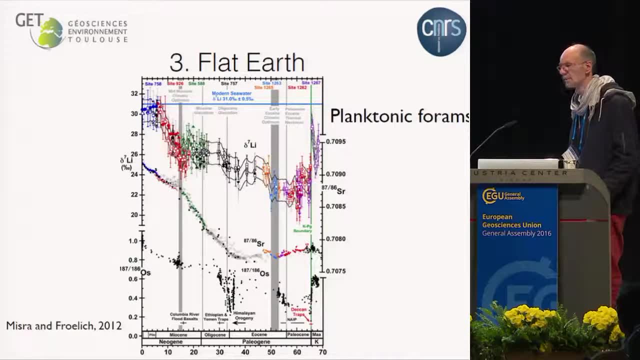 In a very interesting paper. Was the late Paleocene, early Eocene out Because the Earth was flat? The lithium is something important to understand the processes that are at play here. The lithium is rising over the Cenozoic. This is the lithium delta: 7 lithium measured. 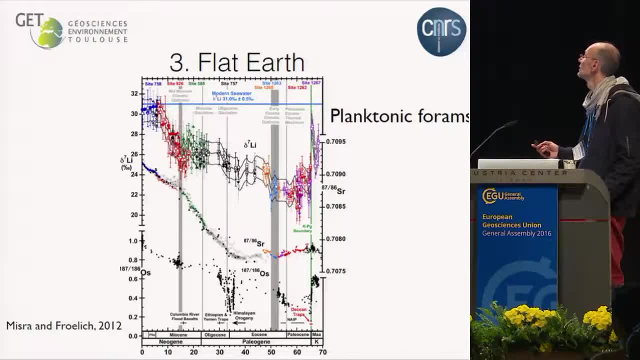 This is in fact the value of the sea water. So it is increasing through time from the Eocene towards the present day, Displaying very low level in the Paleocene and early Eocene. So it is not an easy signal to interpret And I will show you two different interpretations that came finally to the same conclusion. 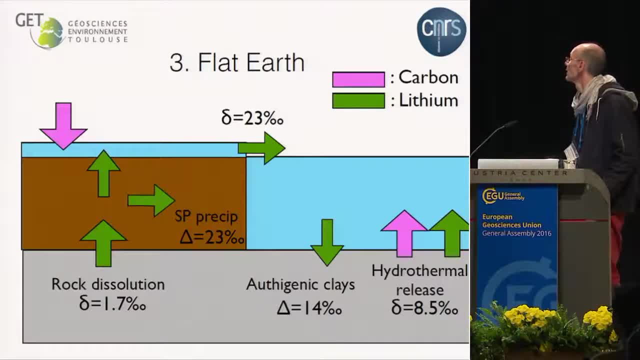 And that is interesting. So how it works? Lithium is produced by rock dissolution With a delta of 1.7 per mil. Then it is going to the ocean, But there is a precipitation of secondary phase Which are largely enriched in lithium. 7- No, Once again. 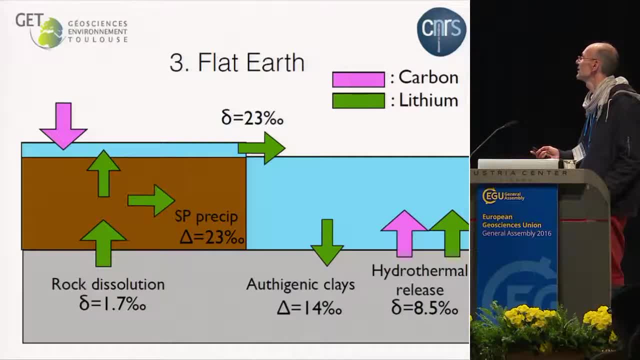 The rock dissolution is producing lithium. Lithium 6 is preferentially stored in secondary phase during precipitation of Kaolinite, Smectite and so on. And lithium 7 is going to the ocean With a delta 7 lithium of about 23 per mil for the river waters. 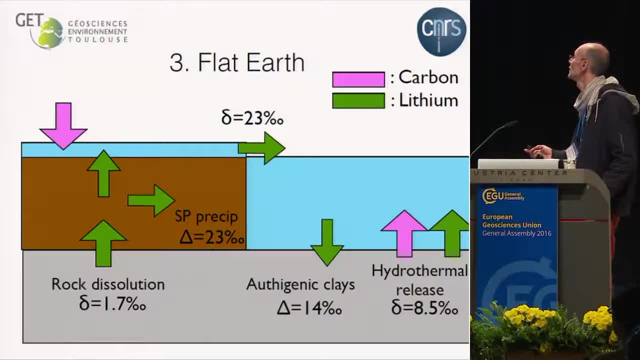 And a lot of processes are still happening inside the ocean, But I will concentrate on the continental part. So the idea is quite simple: If you are producing a lot of secondary phases, You will fractionate a lot And you will increase the delta- 7 lithium of rivers. 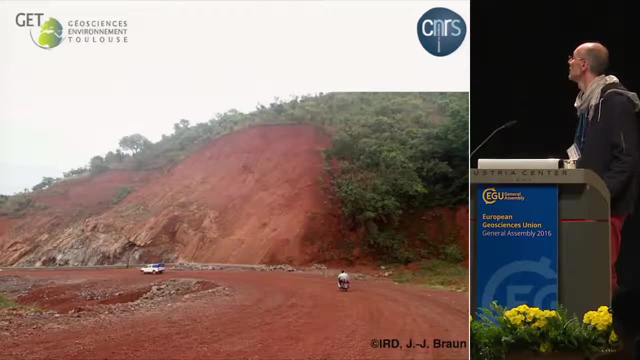 So I am talking about this one. I am talking about shielding of the rocks. This is in Cameroon And you see here a lateritic profile Which is quite thick And the bedrock is just at the bottom And you see that all this can store lithium And can reduce the drainage of the water down to the bedrock. 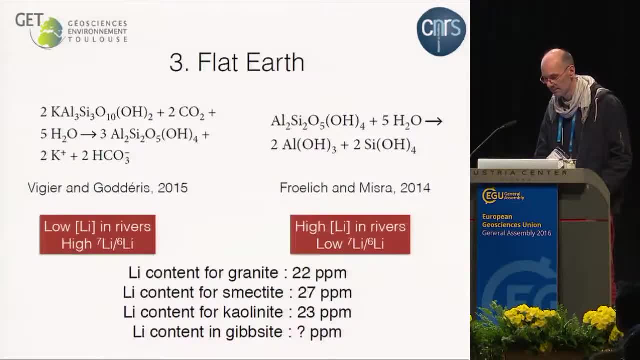 And then reduce the CO2 consumption. The idea is quite simple. We propose that when you are weathering during the Eocene, You are weathering a granite- Let's say this is a Kefelspar granite Attacked by a carbonic acid Precipitating Kaolinite. 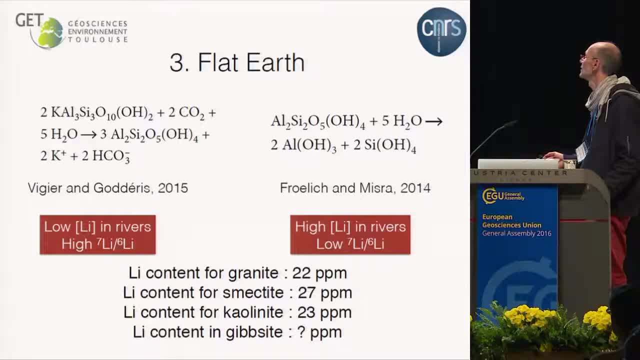 And you see that for granite and for Kaolinite You have almost the same content in lithium. So if you are precipitating a lot of this, You will have a low lithium in the rivers But a very high delta 7 lithium. Ok, But the other solution. 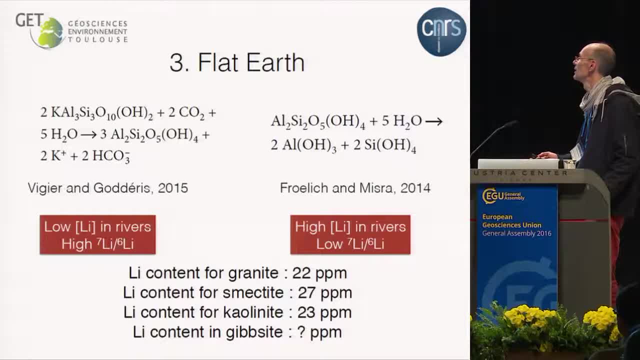 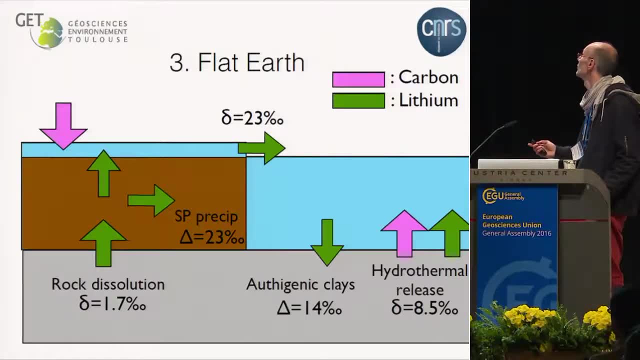 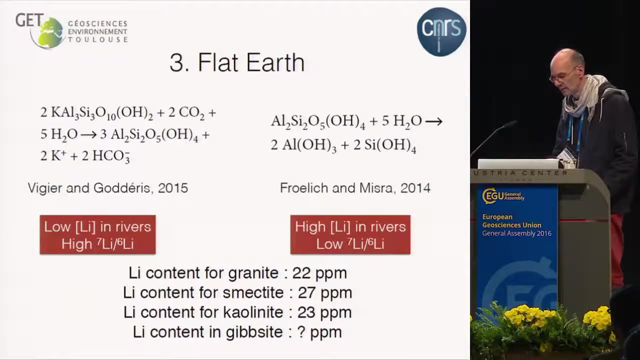 This would produce. I will show you on the next diagram. If you put a little lithium in the rivers, You will reduce this input into the ocean And then you will drive the lithium of the ocean To lower values. The other solution is to go a little bit further. 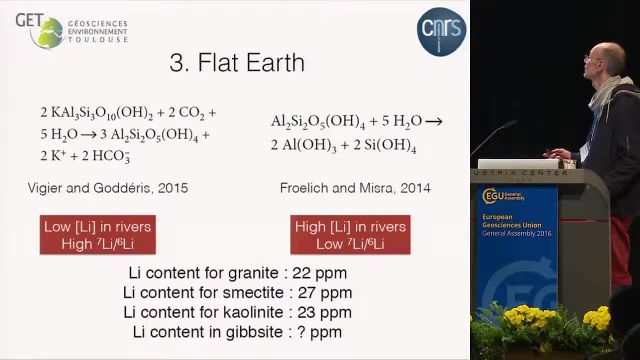 And this was proposed by Froelich and Misra. They are saying that in the tropical climate Even the Kaolinite here Is still reacting, dissolving and producing gibbsite, And they are arguing that gibbsite is not containing any lithium, Which is not yet clearly demonstrated. 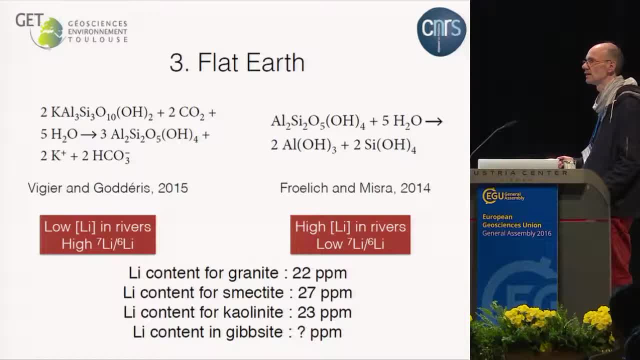 There is a paper just published in January Showing that there is lithium in gibbsite, So it's something not completely clear, But the idea is that if you are just releasing All the lithium stored in the Kaolinite During the dissolution, You will not have any impact. 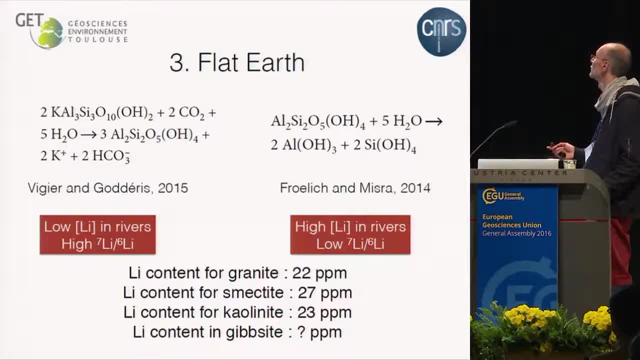 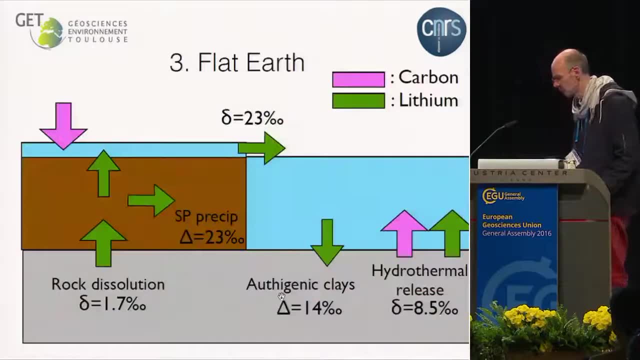 You will get a high lithium in rivers. All the lithium released by dissolution of the rocks Will come back to the rivers, But with a very low lithium 7 and lithium 6 ratio. I'm not sure I'm clear. I'm wondering. So the idea is that all the lithium released here 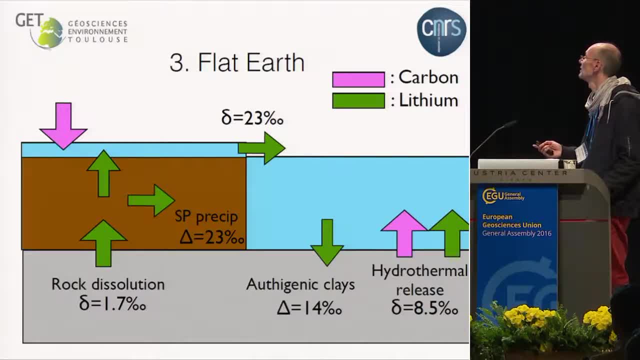 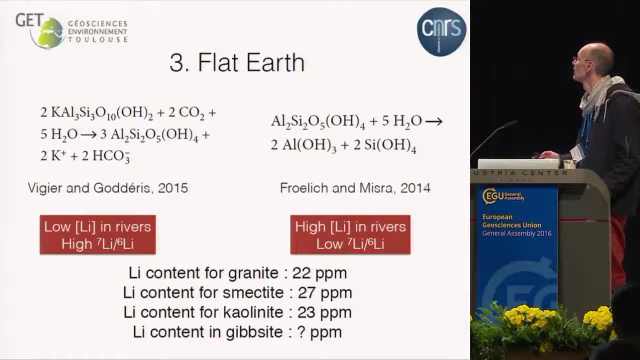 At a very low value Is just ending in the rivers Because it is released from the secondary phase dissolution. So two solutions: Low lithium in rivers And high isotopic ratio In the early Cenozoic, Or high lithium in rivers And low lithium isotopic ratio in the rivers. 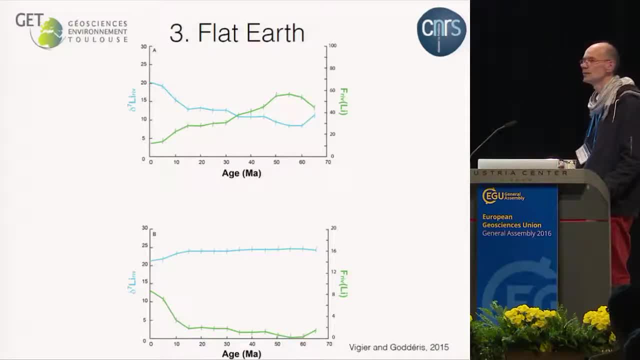 And this is how it looks like. Both models are just reproducing Exactly the lithium isotopic composition Of the seawater, So they are both valid. The first one, Which is mainly the Misra and Froelich hypothesis, Is saying that you have A lithium isotopic ratio of the rivers. 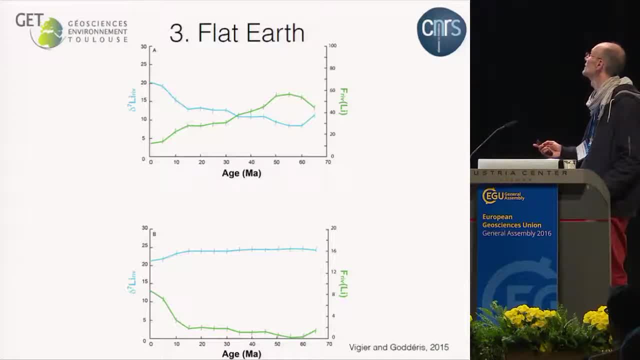 Which is increasing through the Cenozoic And the flux that is decreasing. But the other solution is to keep The lithium isotopic ratio of the rivers More or less constant And saying that it is stored in secondary phase At the beginning of the Cenozoic. 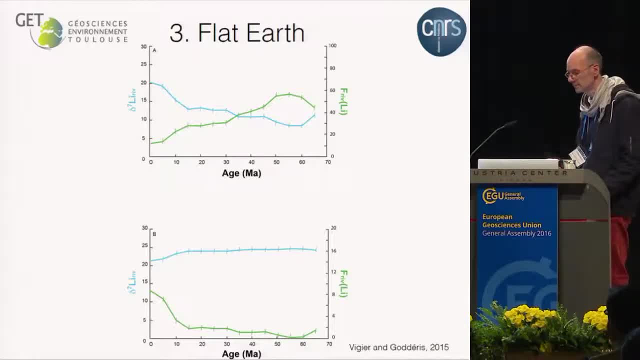 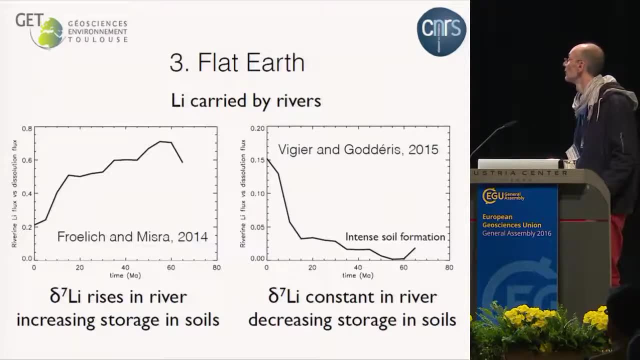 And then it is slowly released into the system. I have plenty of time, So once again Going back to the results of this simple model, This is the riverine lithium flux Versus the dissolution flux. So that means that here In the model of Froelich and Misra, 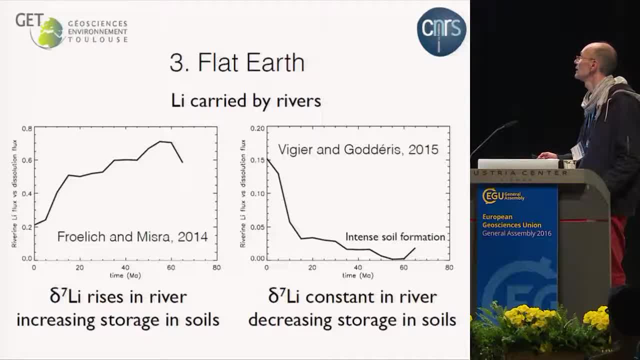 You have 20% of the lithium released in rivers That are coming from the dissolution of rocks. The rest is being stored in secondary phases. This is the Froelich and Misra paper. This is our paper. This is totally different in terms of storage of lithium. 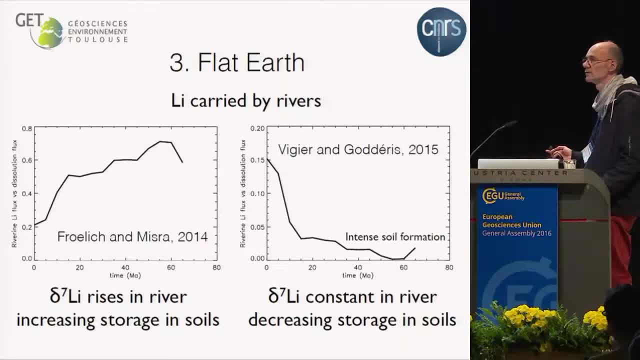 You see that there is almost no lithium In rivers, which might be extreme, But there is almost no lithium in rivers At the beginning of the Cenozoic And then it is increasing through time, Going back to the present day. So there is decreasing storage in soil. As time is running And once again I have to say that both solutions are equally possible. The question is: What are the secondary phases able to store During the weathering reactions? If you look at some data now, This is coming from a paper By Beauvais and Chardon. 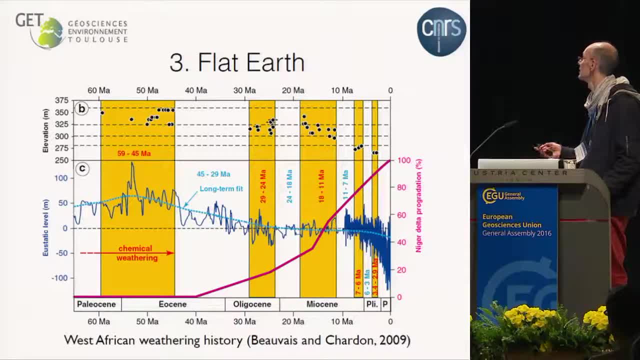 And time is running the other way. So the beginning of the Cenozoic is here And the end is here, And you see that at the beginning of the Cenozoic And several times during the Cenozoic, You have huge event of kaolinite. 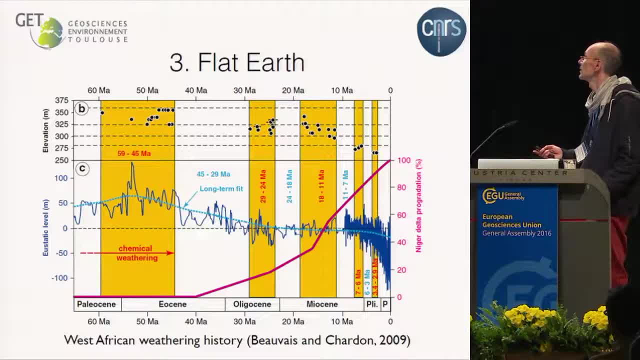 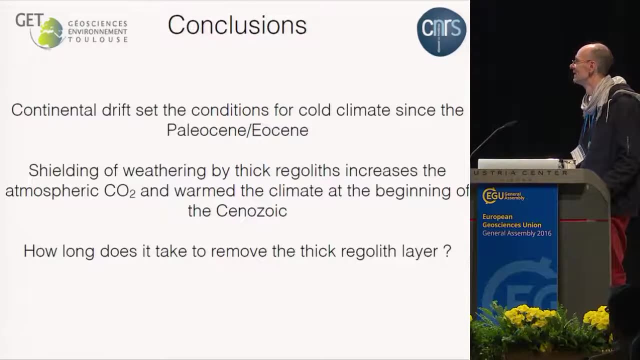 And thick weathering profile formation. That is relatively coherent with what we proposed. So there would be a big lithium storage During this episode here And I came to the conclusion And I have plenty of time to discuss it. So the idea is That maybe continental drift Set the conditions for cold climate. 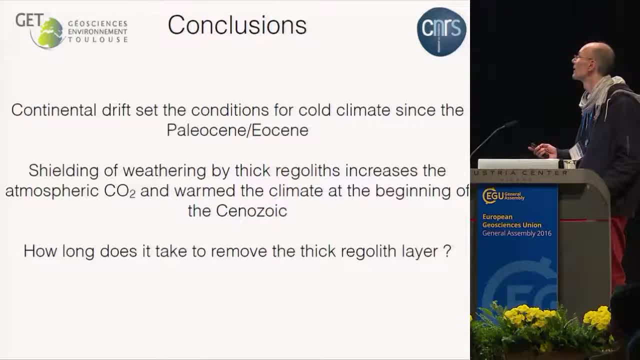 Since the Paleocene-Eocene boundary. The shielding of weathering by thick regoliths Increases the atmospheric CO2 And warm the climate at the beginning of the Cenozoic. It is not really a question of cooling it, But it is a question of warming it. 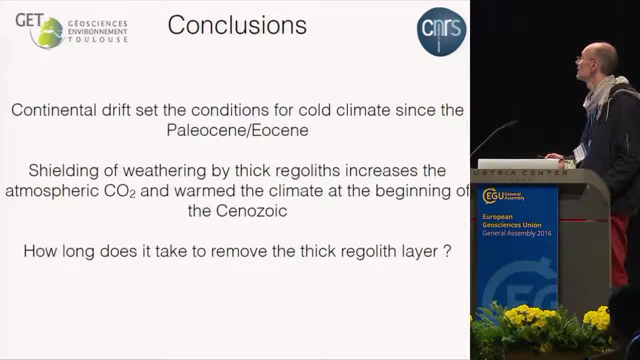 At the beginning of the Cenozoic. And finally- This is a big question And Jean has discussed this a little bit- The question of the timing. The transition between the warm world To the cold world Lasts something like 10 millions of years, Which is quite long. 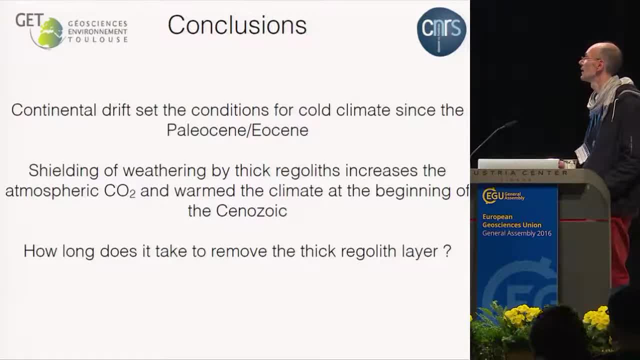 And I think we still have to understand How weathering profile Responds to the different forcing. This is exactly what Jean has shown us. At what time scale Are we just adjusting the weathering profiles To new conditions on Earth? So okay, That's it. I have 10 minutes for questions. 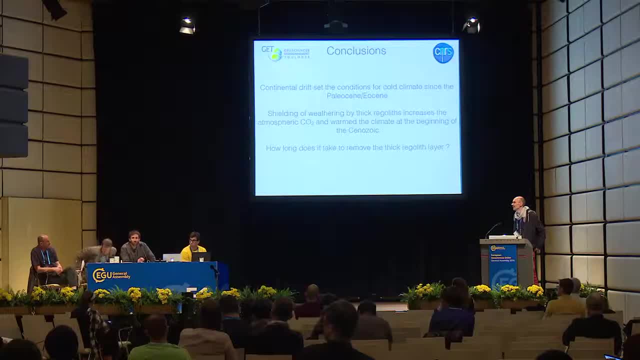 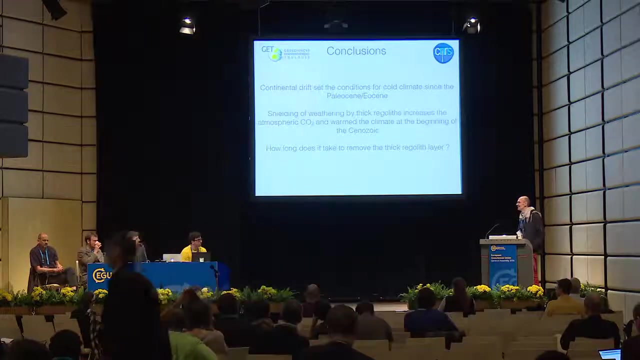 Thank you for your talk. Questions, Please. I have questions. So here you have a really global approach, Especially for the lithium, For all the lithium in the rivers. Yeah, Are there any big differences, I mean in the spatial framework, If you look at the tropical rivers Or the mid-latitude rivers? 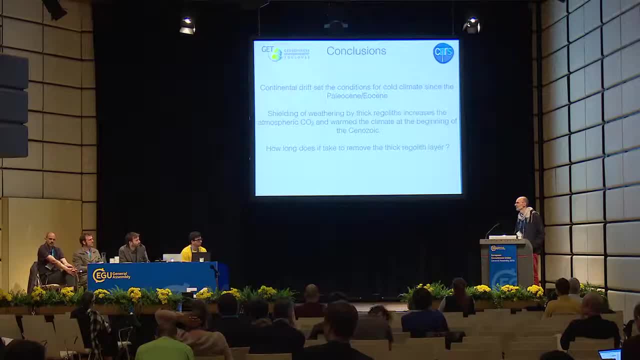 Yeah, That's a very good question. In fact, there are not so many data. There might be. They are building now Some kind of a compilation Of the lithium isotopic data in rivers, But apparently It's a big question Because there is a lot of variability. I cannot discuss this really. 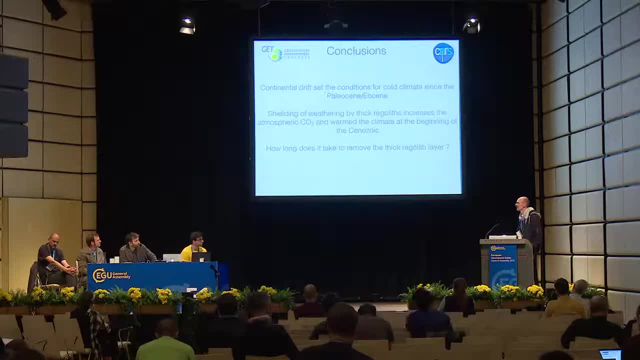 Because we would like to calibrate our model On something like the real data And the real data being compared For the moment- And it seems that all the rivers Are displaying at the same time- A system which is compatible With both hypotheses, Depending on the place And the location within the catchment. 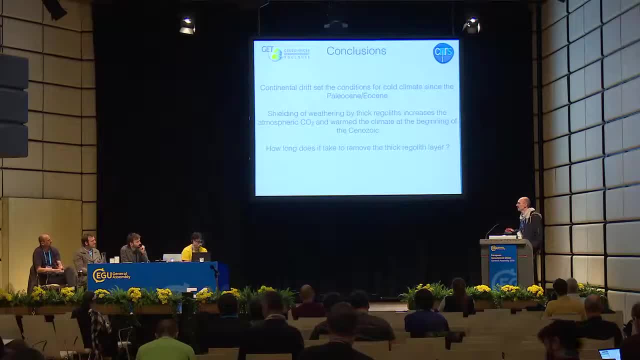 Where the data have been acquired, But this is not clear for the moment. I would really to say I'm not a data guy, I don't know how it works precisely, But I have to say That, working with Nathalie Vigier, That we do not have any compilation. 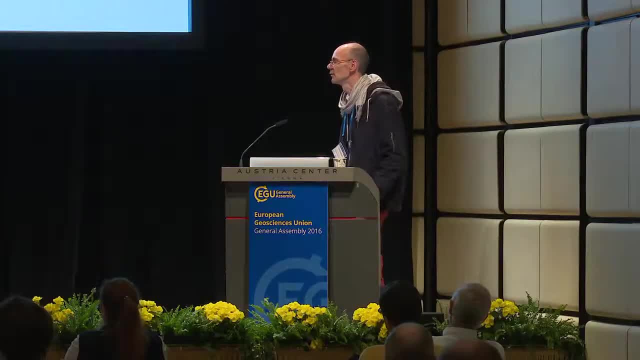 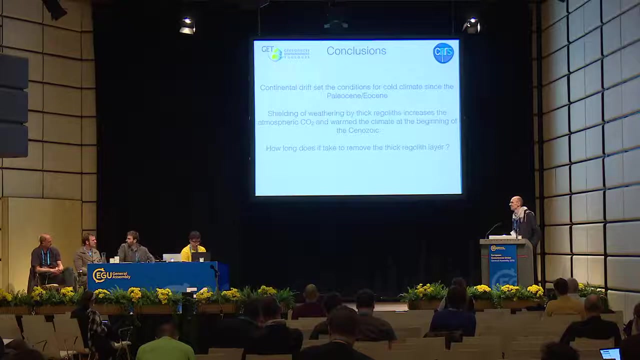 Clear compilation for that, And this will be the key point. Most of the data are just For the moment, concentrated On the lithium storage In the various clay minerals phases, On a theoretical point of view. But sorry, Yes, please. I think it's a pretty interesting story. 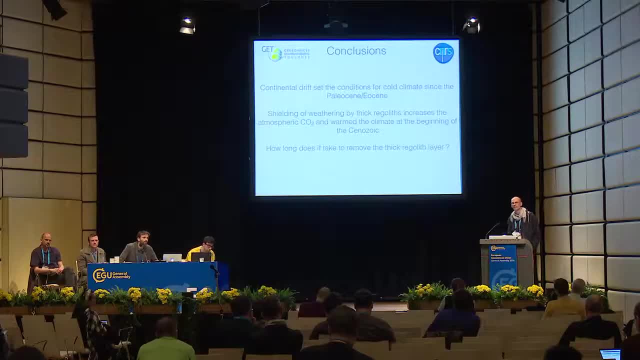 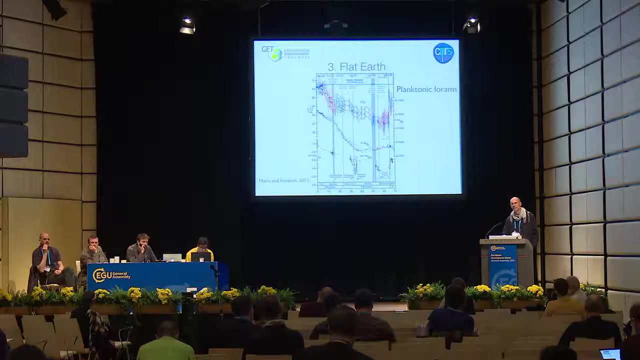 I'm having one trouble understanding, Which is that When you look at the general, The general trends Throughout the small soil- Yes, Especially out at like The long term variations In the CO2 demands, For instance, benefit, Yes, Then the big picture is that The really big fractional Of CO2 and temperatures 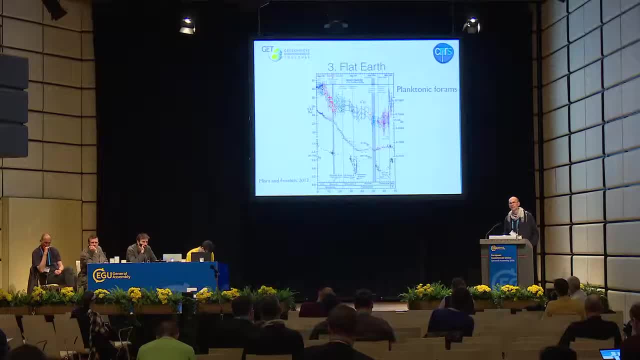 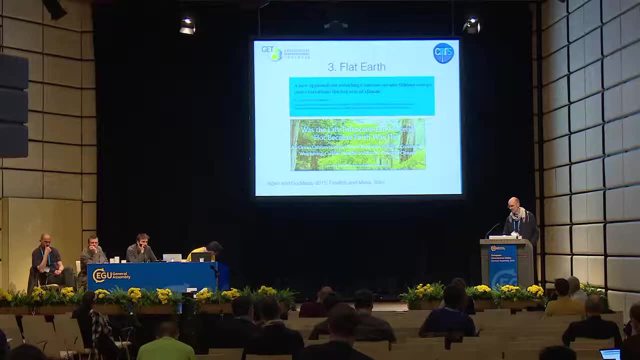 Throughout the EC And then you have the big jump At the EC position And after that You basically have A pretty long period With not too much Of changes. Of course there are changes, But they're not as big As at the start. Yeah, And if I'm correct, 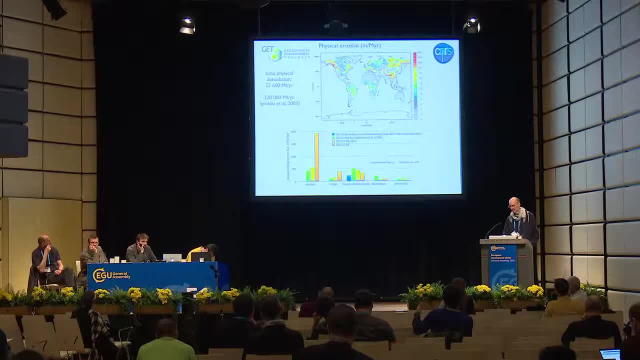 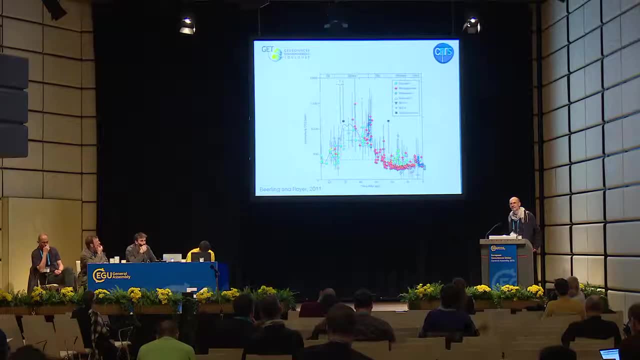 The big draw down Is actually before, When you see most Of the major uplifts That take place. Yes, Because most of those Are like between, say, 40 and 10 times 40, and then And then present, But they don't accumulate At the end. Yes, So how would you? 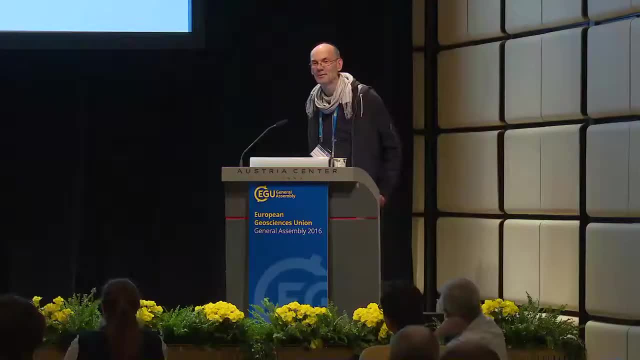 Explain that I don't know. That's, once again, A very good question. I think that First I have to apologize Because I gave my talk In 20 minutes. It was designed For 30 minutes, So I have got too fast On several points. But in terms of CO2, 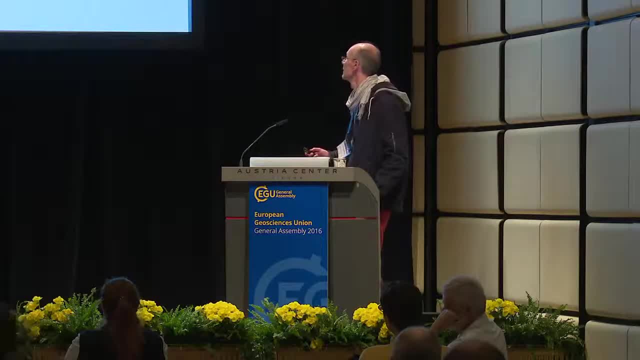 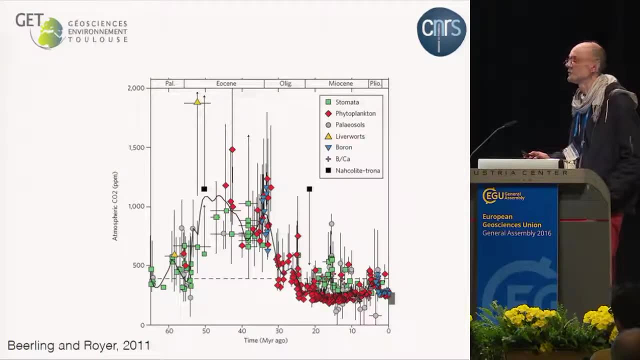 The question we have Is that Of course, we can produce High CO2 level here When shielding The continental weathering, But at What is the time scale Of the response Of the system To a change? I don't know What is happening here. CO2 is going down. 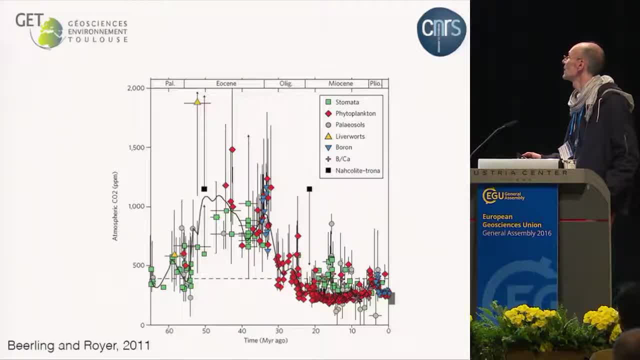 Quite rapidly Within a window Of 10 millions of years. This makes me think That the weathering system, The weathering profile, Is reacting At a quite slow rate To changes. But is the change Tectonic? I'm not so sure, Because the main Major uplift Are a little bit later. 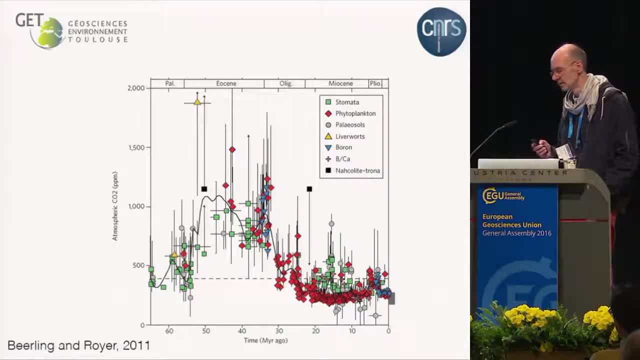 Let's say It's not totally clear. Also because You can see Some starting Of the tectonic In the literature At 40, 30 or 20 millions Of years, But I don't know What is the transition. I'm just asking The question, The transition here. 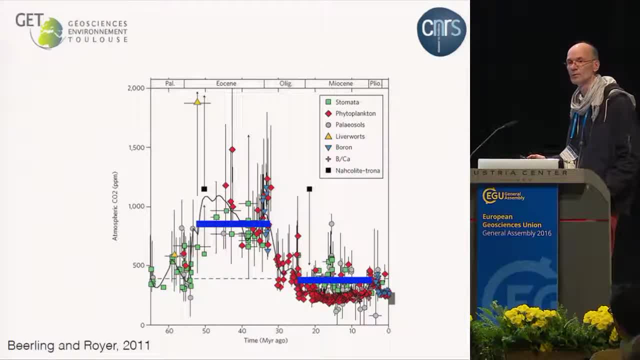 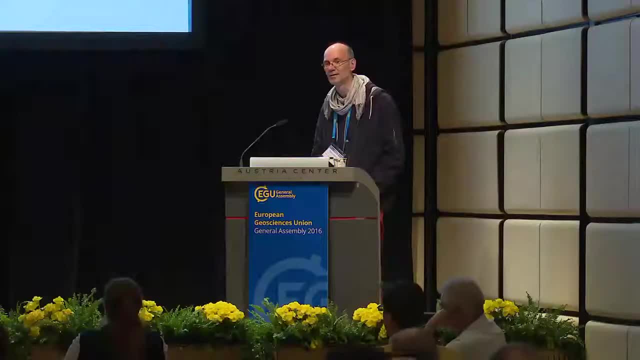 Is something That is really Totally unsolved Right now And I have no scenario For that. It's disappointing. It's just Work for the future. Just to- Oh sorry, Please Question to that: What was the role Of vegetation? That's a good point. Yeah, That's a good point. 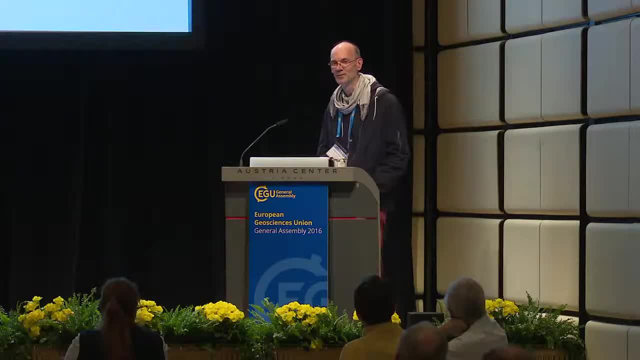 Also, Vegetation Is not impacting On lithium. As far as We know, For the moment There is no Fractionation Of lithium Within the vegetation. Regarding the story Of lithium, We can Forget about The vegetation And about CO2. I'm just asking Very good questions. You know, I don't know. 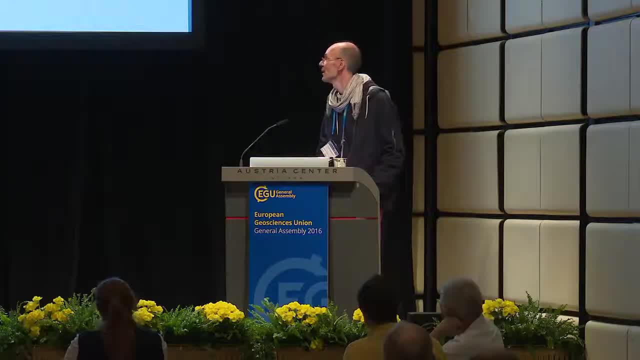 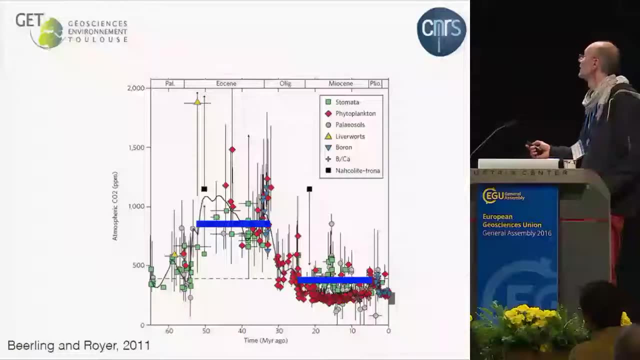 I don't know. There might be, Of course, Some impacts, Clearly Because The vegetation Here Is not The vegetation Here Is not The vegetation There. The mass Of vegetation Can fluctuate, It can have An impact On the albedo, And then We have focused Mainly On what is. 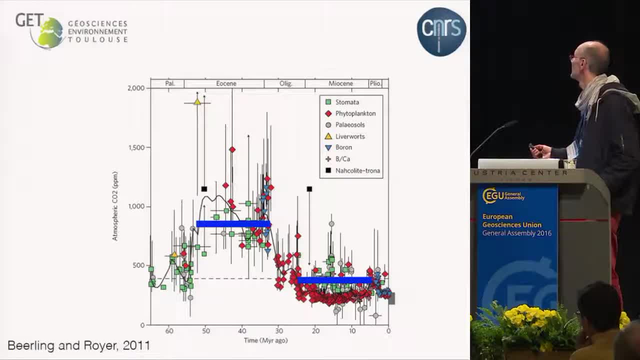 Happening here At 38 Millions of years And what is Happening here At the end Of the cynosomic. But even here For the CO2 There are Large discrepancies. I'm just Coming back To the previous Question. Here you have 500 ppm Coming from. 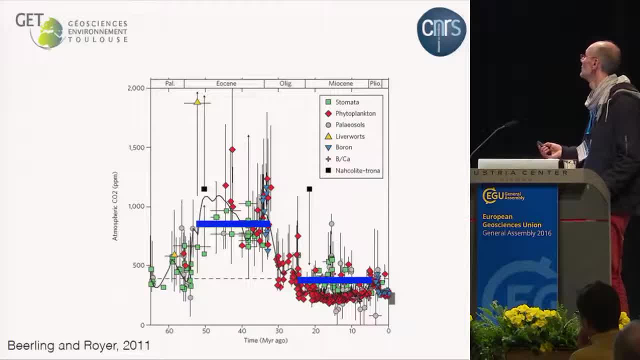 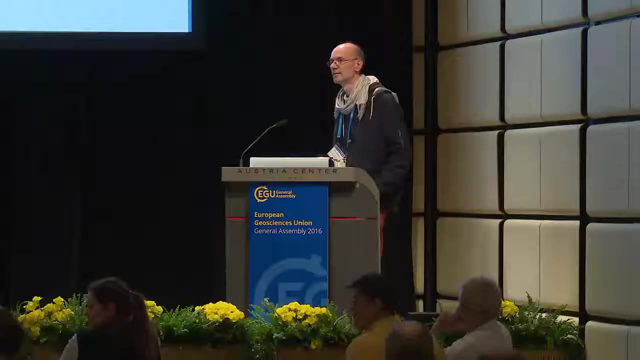 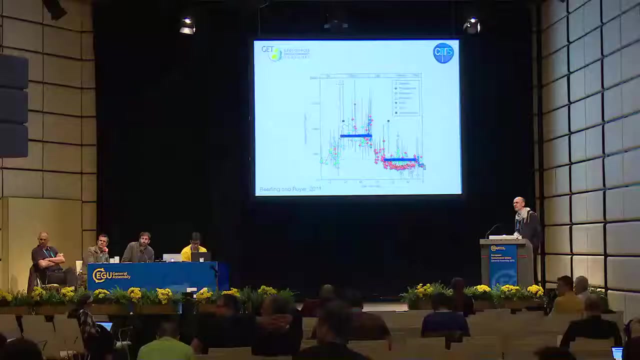 Stone metal Indexes And you have Something Less than The present Day value Coming. So the vegetation Is playing A role, But which Role Nobody Knows. Yes, Please, I would Have Said That's A good Question Prior To Your Question. Yeah, Of Course, This Is Why, Once Again, 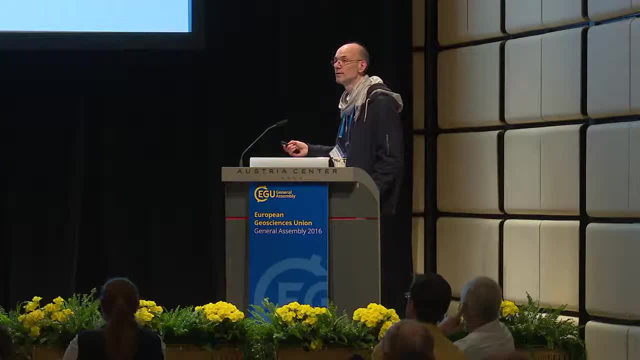 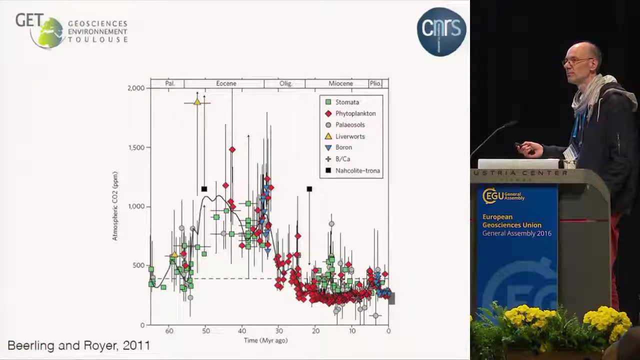 These Are Quite Low Levels Of CO2. This Is Why I Think That Proposing A Cold Baseline For The Cynosomic Is Not Totally Crazy, And This Is An Event Produced By Continental Drift. But That's All I Can Say For The Moment. But Of 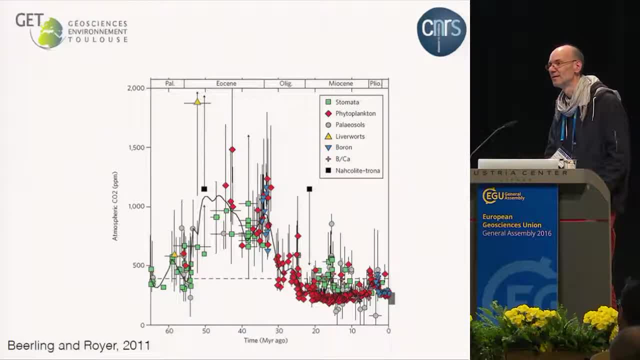 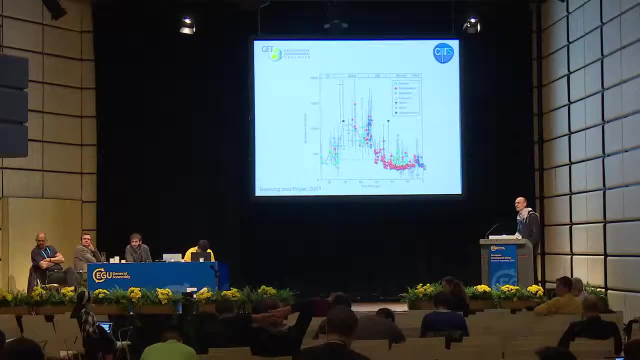 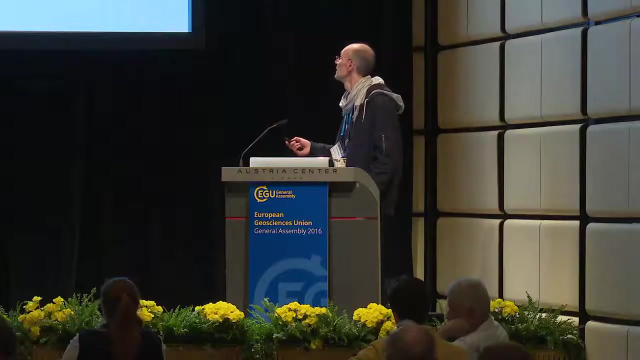 Course. This Is Maybe A Cold Baseline And This Is A Warm Event In The Cynosomic. I'm Not Clearly Answering Your Question. You Know, If You're Talking About The Rapid Decrease In Transition, It's Too Slow To React To This. But Once Again, 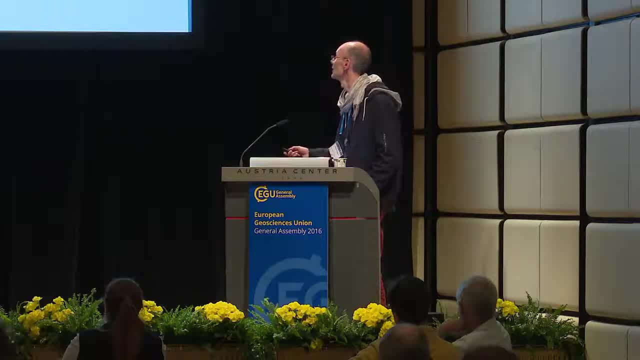 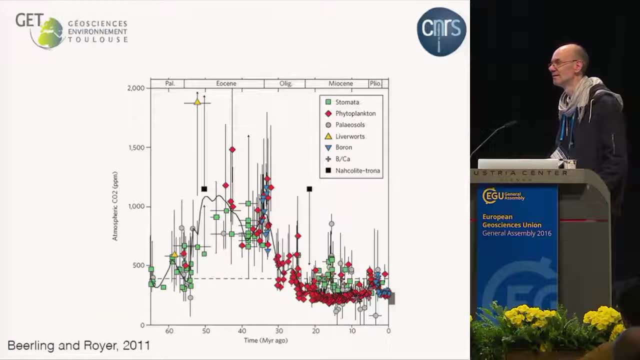 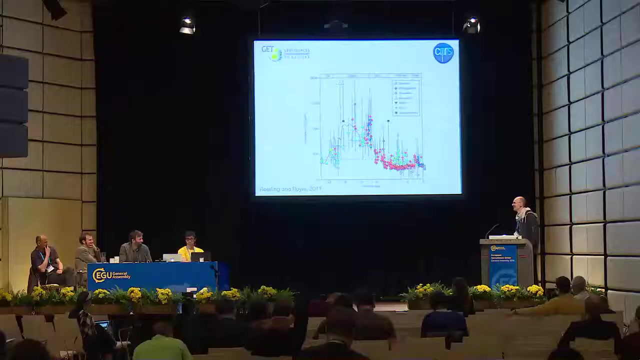 You Have Something Between This And This Level, So It's A Good Investigation. I Have One More Question. That's A Good Question, I Have Not The Answer. Question Regarding The Transition From A Flat World To A World: Yeah, Maybe You Could Imagine That At A Certain Altitude. 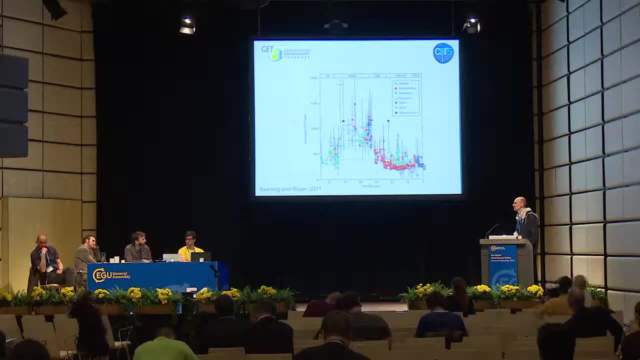 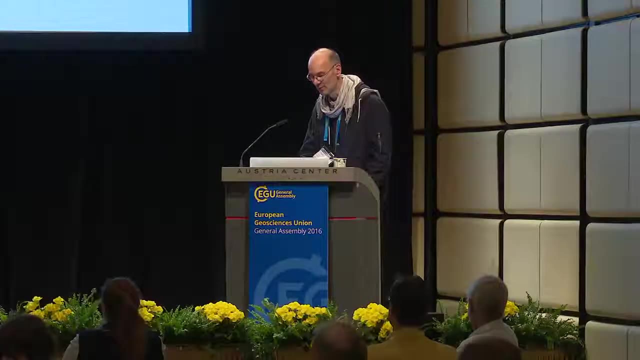 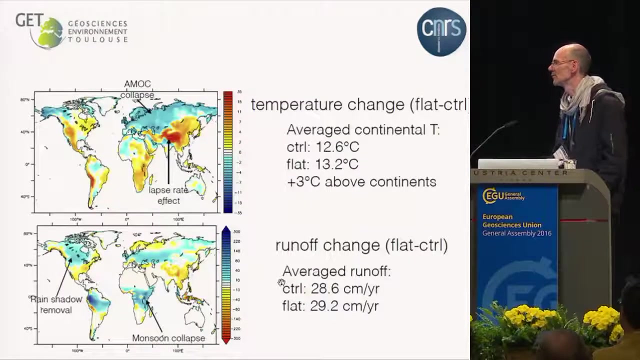 It's A Bit Of Follow-Up Of The First Question. Yeah, Maybe You Can Imagine That You Have A Different Response Of The Simulation, With A Half Altitude For Instance, Or One Third Altitude, Two Third Altitude. It's Not Done Yet, But I Would Like Just